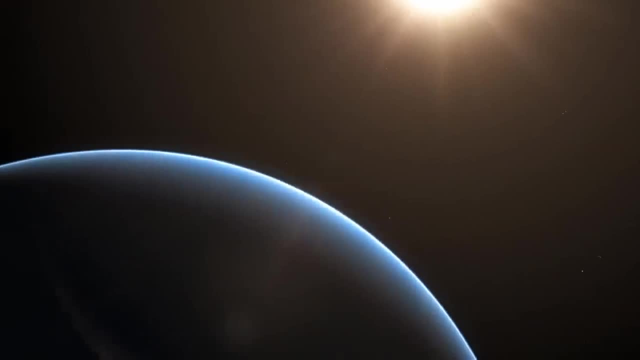 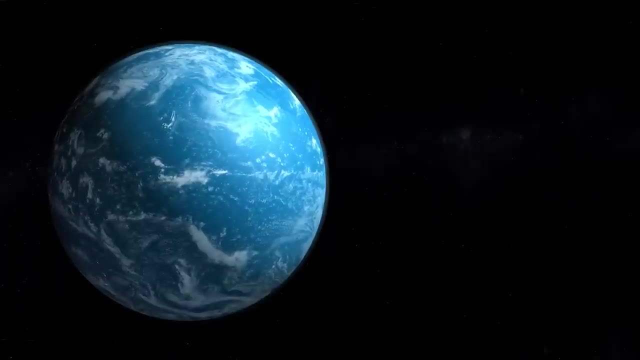 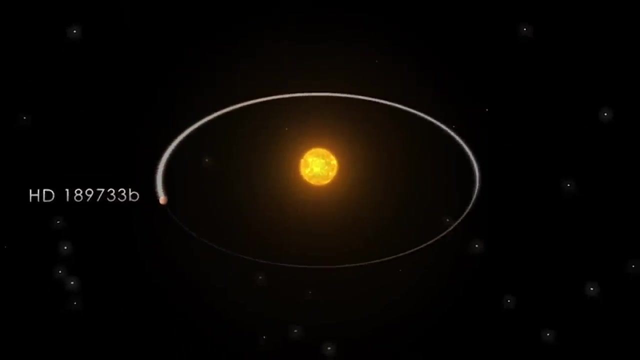 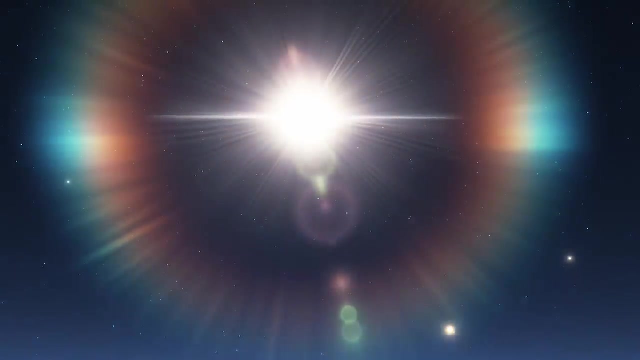 and dynamics. The atmosphere of HD 189733b is a scorching turbulent maelstrom, with temperatures soaring to over 1,000 degrees Celsius. This intense heat is a direct consequence of the planet's close orbit around its host star, which exposes it to severe stellar radiation. 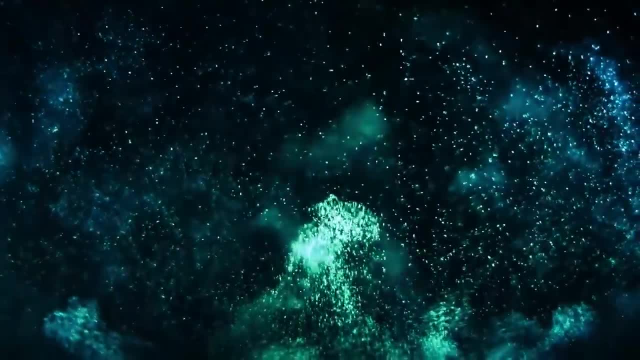 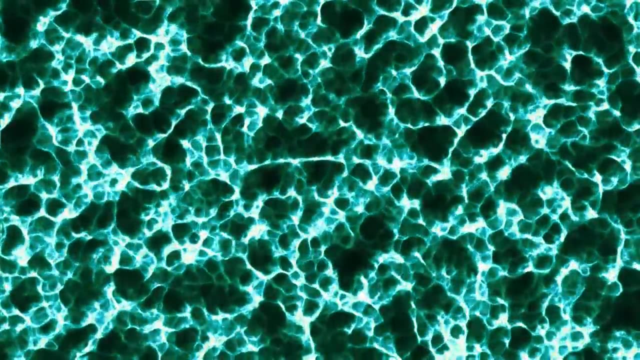 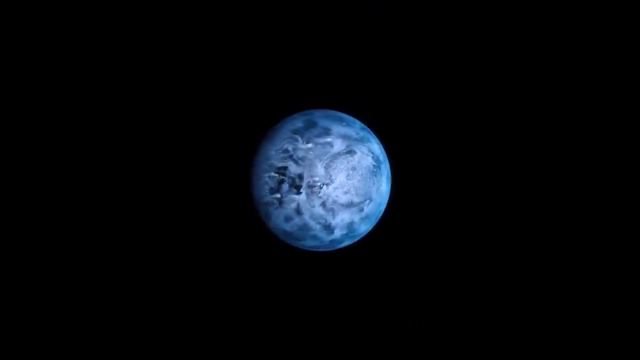 In this hellish environment, silicate particles are able to form and exist in the atmosphere. The high temperatures ensure that these silicate particles are not solid, but instead exist in a molten state floating in the atmosphere. The wind speeds on HD 189733b present a staggering contrast. 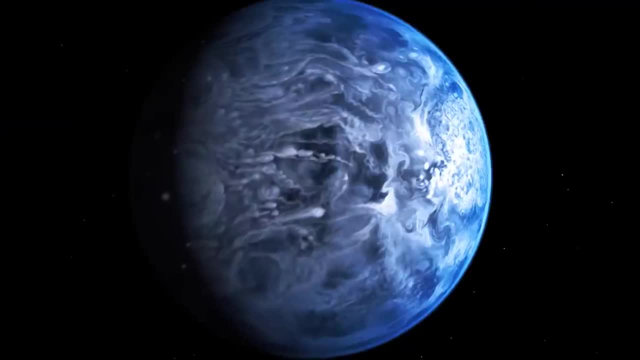 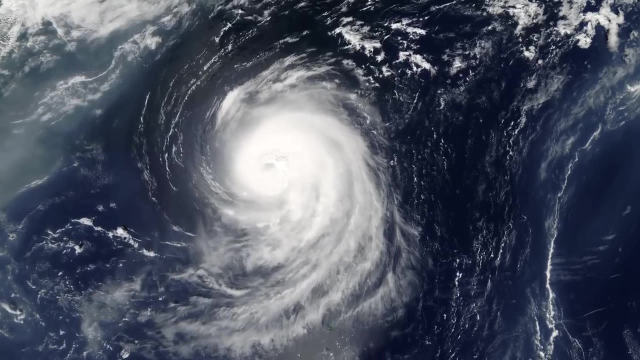 to what we're accustomed to on Earth, painting a picture of a world where the very air itself embodies forces beyond our wildest comprehension. On Earth, the most powerful hurricanes, such as those experienced by the older generation in the United States, can unleash winds reaching 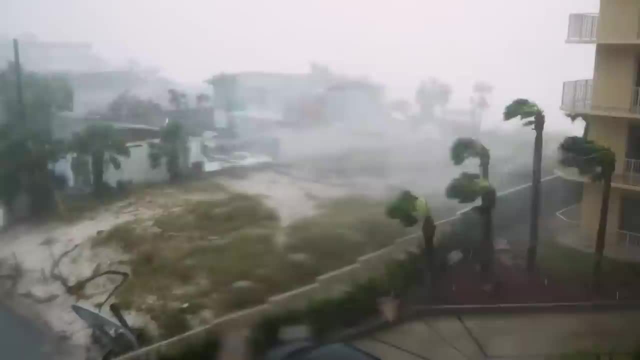 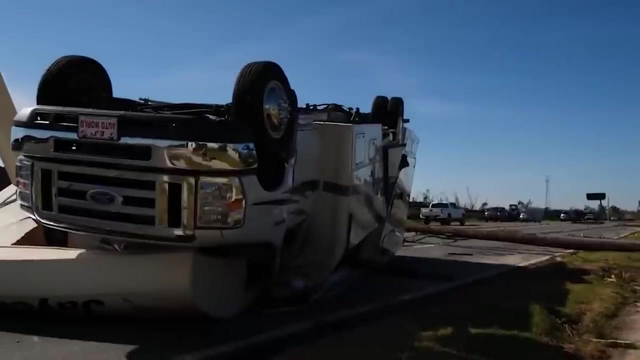 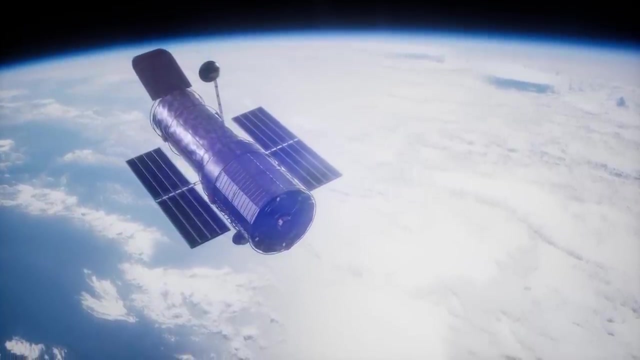 speeds of up to 250 kilometers per hour. Approximately, 150 kilometers per hour is the speed at which they can reach. These storms, while formidable and capable of causing significant destruction, pale in comparison to the atmospheric tempests that rage on HD 189733b. 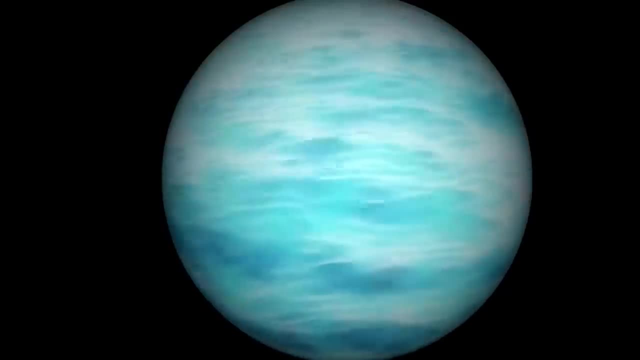 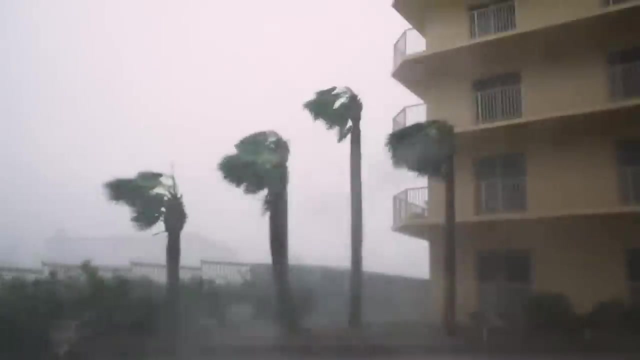 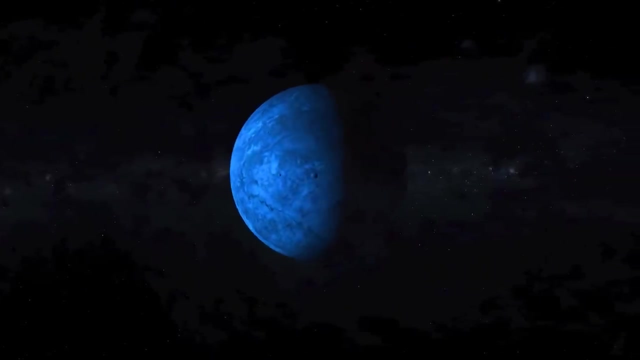 On this distant exoplanet, the winds howl at speeds exceeding 7,000 kilometers per hour, or around 4,350 miles per hour, a figure that is nearly 20 times faster than Earth's most powerful hurricanes. Imagine the air moving at such a velocity that it could traverse the continental United. 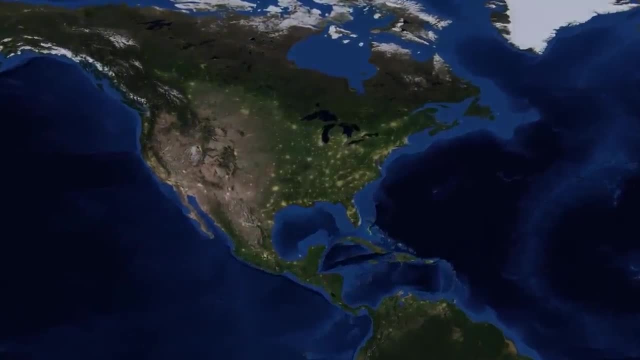 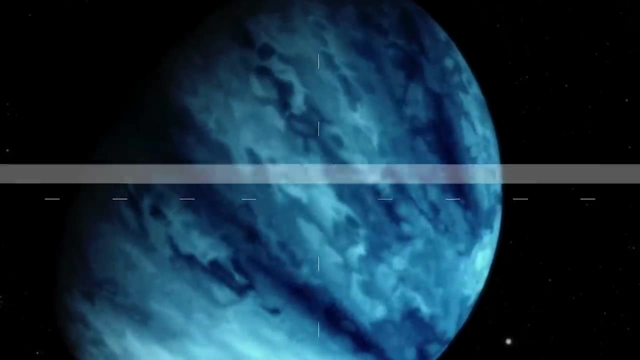 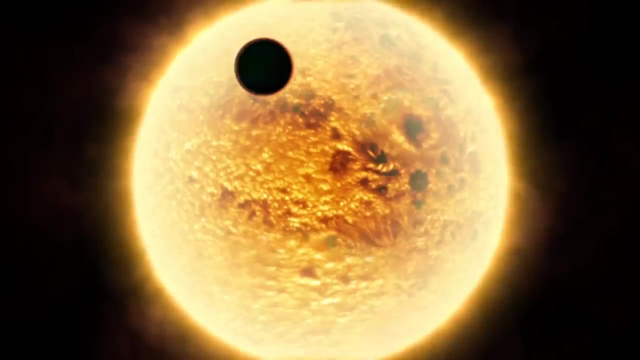 States from coast to coast in well under two hours. This comparison brings into sharp relief the sheer magnitude of HD 189733b's wind speeds and the extreme conditions that define its atmosphere. The cause of these extraordinary wind speeds lies in the planet's close proximity. 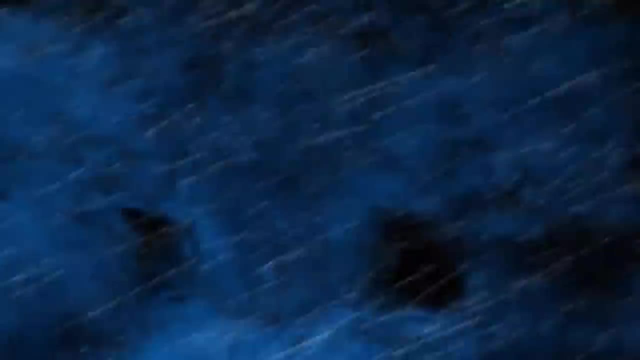 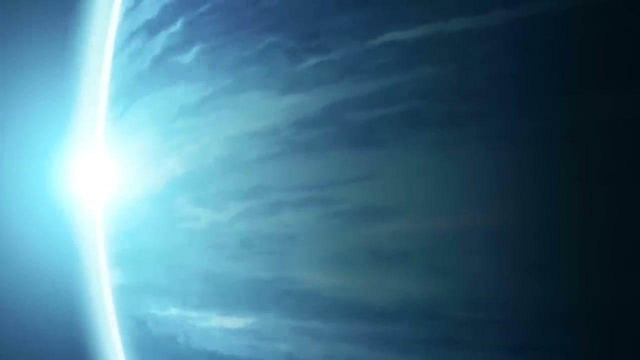 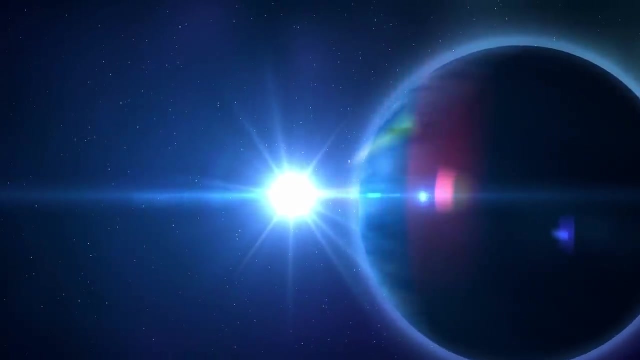 to its star, which results in dramatic temperature differences across its atmosphere. This temperature disparity drives the fierce winds, as hot air rushes toward cooler regions with such speed and force that it defies Earthly analogues. The concept of wind on HD 189733b. 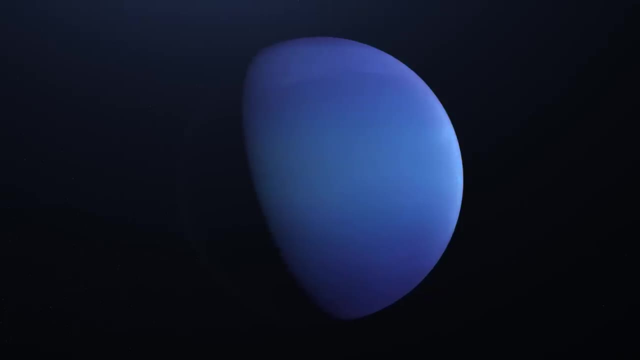 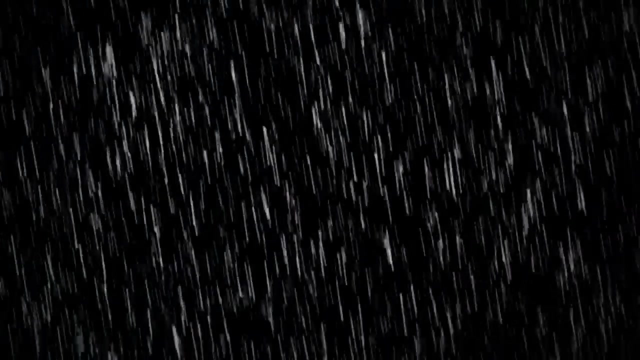 extends beyond mere atmospheric movement. It represents a fundamental aspect of the planet's identity, shaping everything from its weather patterns to the surreal phenomenon of glass rain. The presence of glass rain on any星hal you see on the moon is an pellicle of most significant weather phenomena. 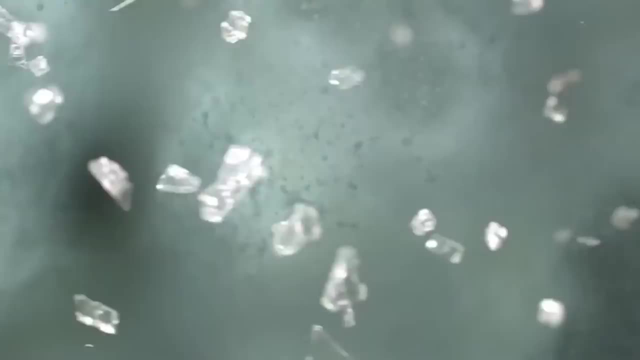 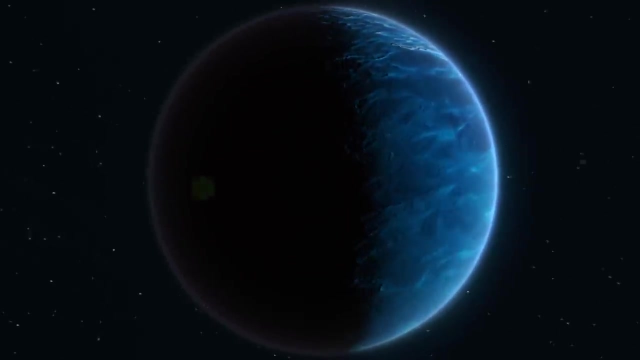 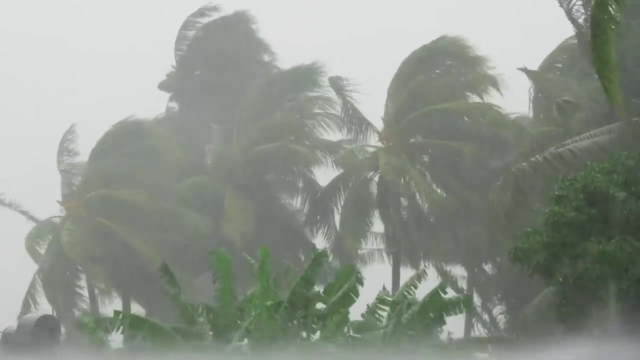 The presence of glass rain on HD 189733b, a phenomenon as intriguing as it is violent, has profound implications for the planet's surface and overall environment, Unlike the gentle rainfalls that nourish the Earth, bringing life to its many ecosystems. 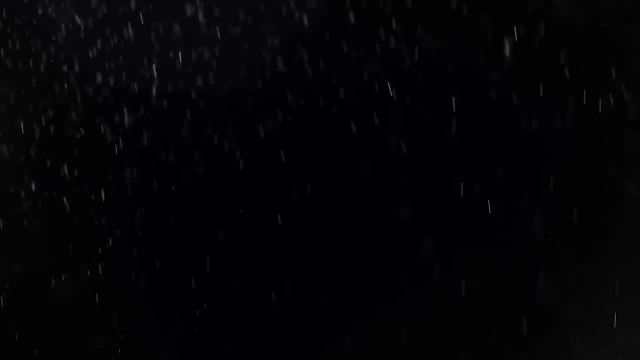 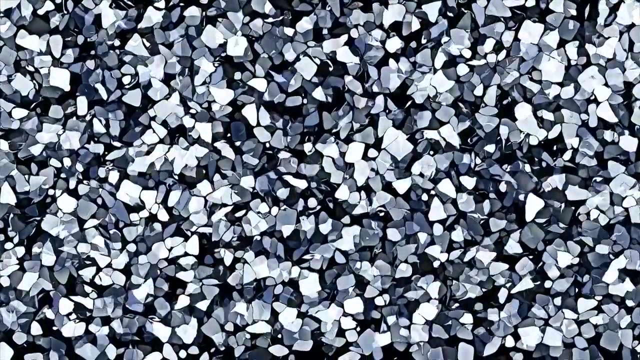 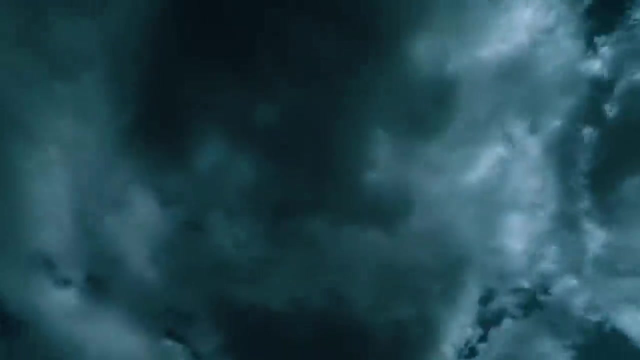 the glass rain on HD 189733b is a manifestation of the planet's extreme and hostile conditions. The shards of glass formed from molten silicate particles caught in the planet's ferocious winds and cooled into solid form, do not merely fall to the surface. 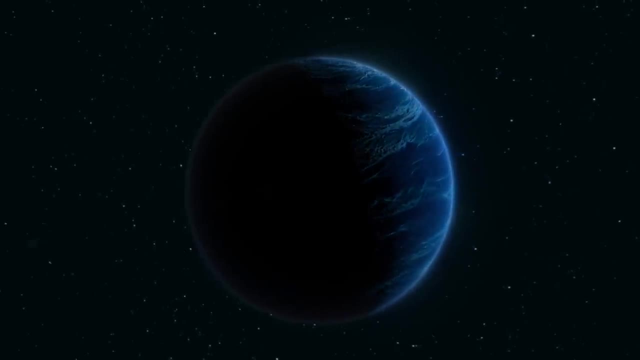 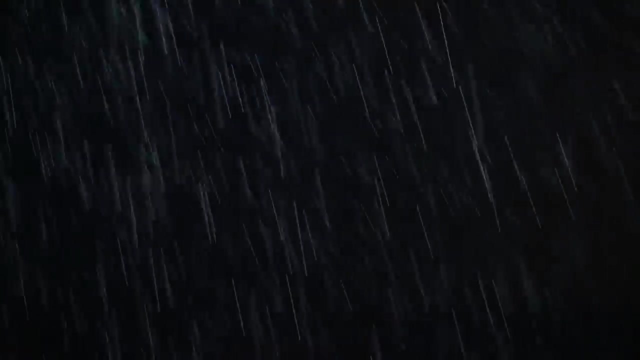 They bombard it at speeds of up to 7,000 km per hour, akin to the speeds of the winds themselves. This relentless shower of glass particles shapes the landscape of HD 189733b in ways that are difficult for us to comprehend from our vantage point on Earth. 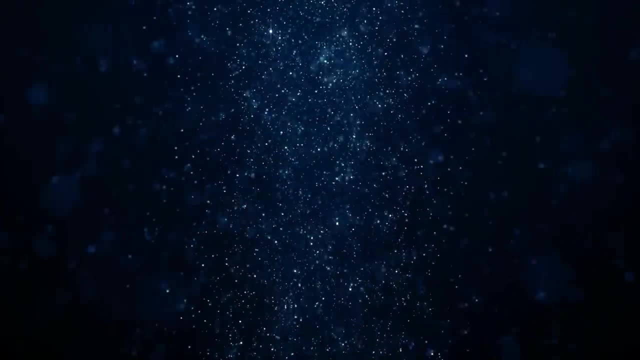 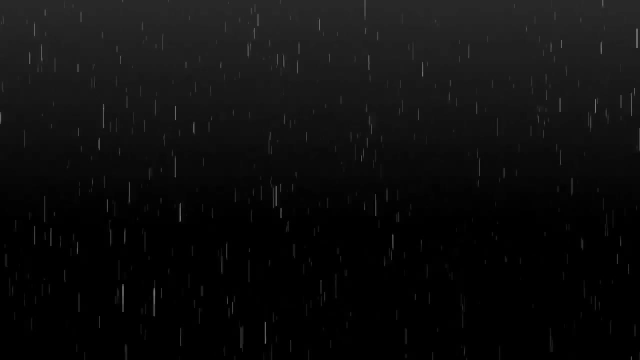 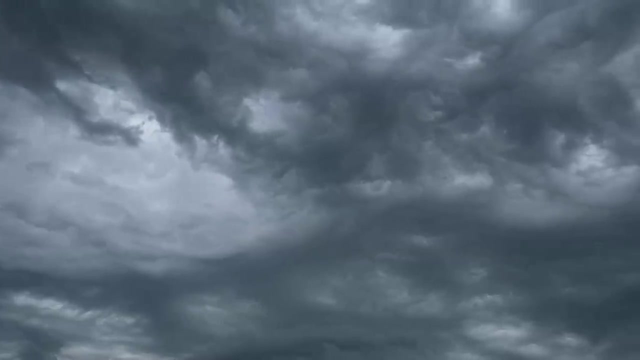 The surface Subjectivity, Subjected to constant abrasion by these high-velocity particles, is likely to be extremely rugged, with features sculpted by the ongoing assault Over geological timescales. the accumulation of glass from the sky could lead to the formation of vast reflective dunes. 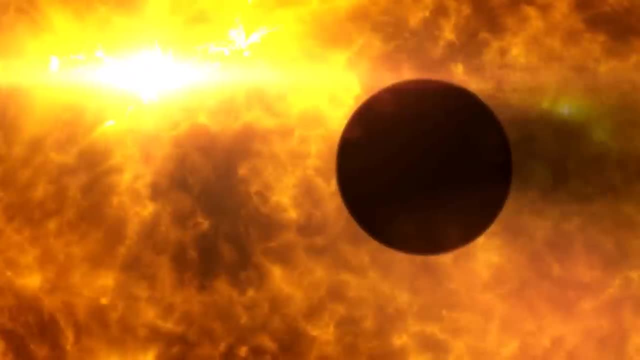 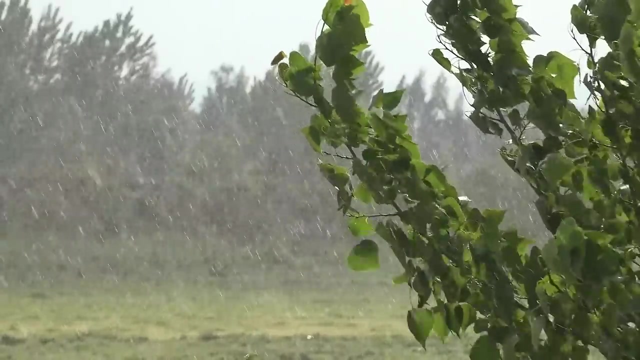 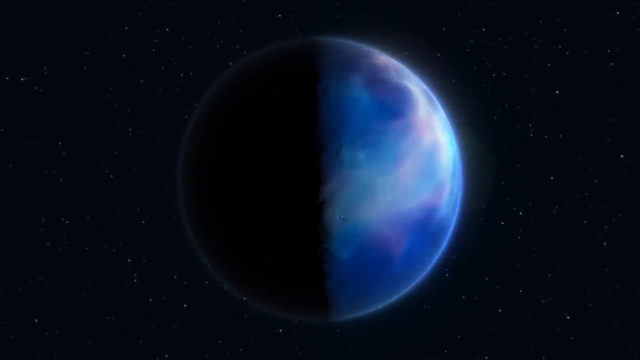 creating a landscape that sparkles ominously under the light of the planet's nearby star. The impact of glass rain extends beyond the physical alteration of the planet's surface. The energy dynamics of such an environment are unique, with the heat from the planet's close star. and the kinetic energy of the falling glass, contributing to an atmosphere that is in a perpetual state of flux. This extreme weather phenomenon likely precludes the existence of water in liquid form, a fundamental prerequisite for life as we know it, and poses significant challenges for the formation of stable habitable zones. 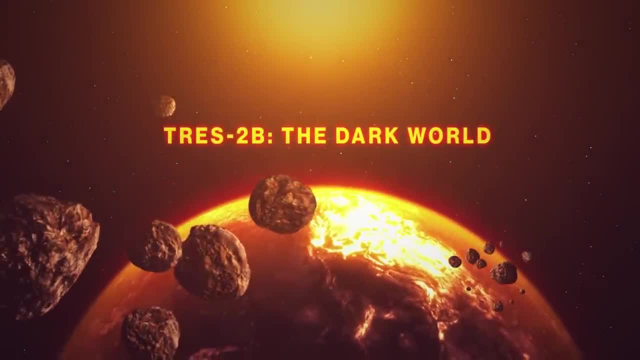 We are only beginning to understand that such enormous量er, vast gou 더� creeping about, goes so far that the planet s-ков in both謝謝 주세요- does not actually make any sense. Ahhh, yeah, that's true. 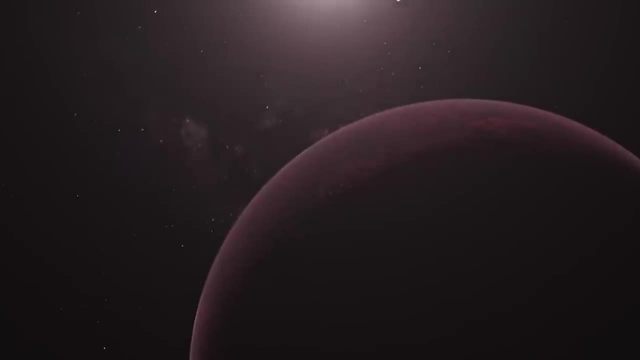 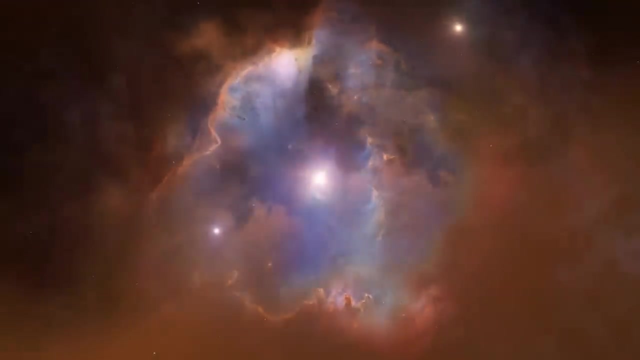 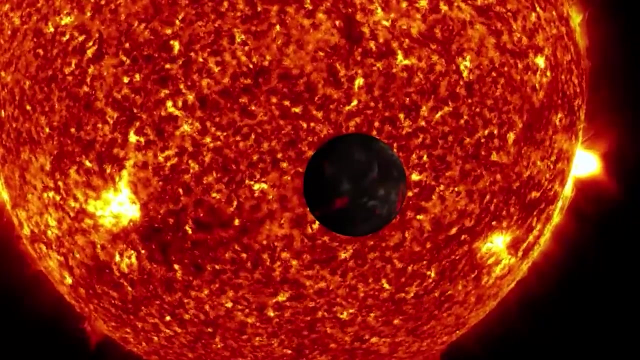 Why would it make any sense? Why would it matter? TRES 2b, another fascinating exoplanet located about 750 light-years away from Earth, holds the title of the darkest known planet discovered in the universe. This distant world reflects less than one percent of the sunlight that hits it. 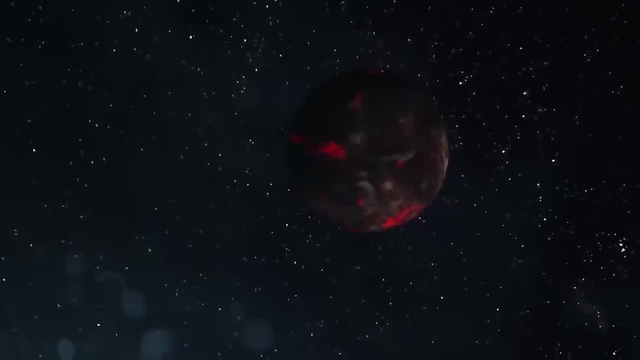 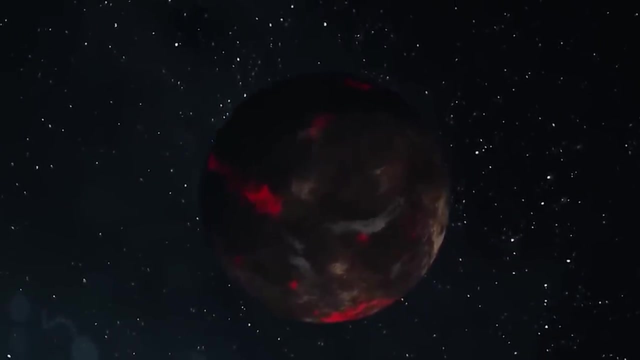 making it darker than coal and one of the most intriguing sub-ru guy details subjects for astronomers and scientists alike. The cause of TRES-2b's extreme darkness is a combination of its unique atmospheric composition and the chemical reactions that occur within it. 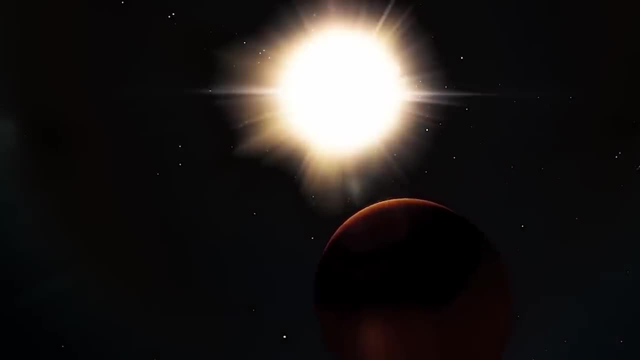 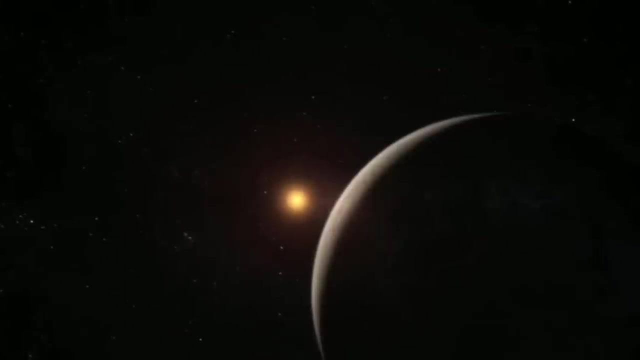 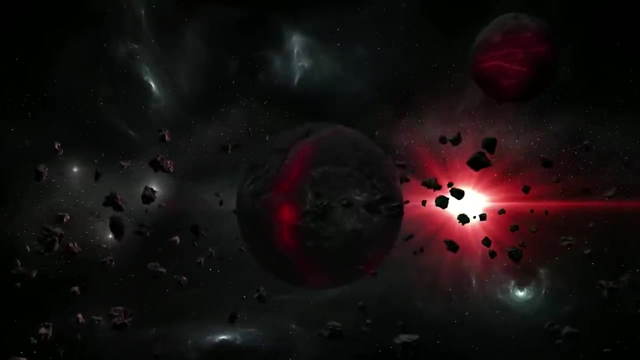 phenomena that starkly contrast with the more familiar climates and celestial bodies within our own solar system. The atmosphere of TRES-2b contains a high concentration of light-absorbing chemicals such as vaporized sodium and potassium, as well as titanium oxide. However, 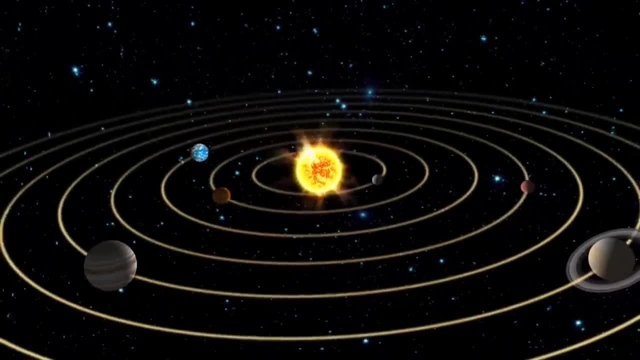 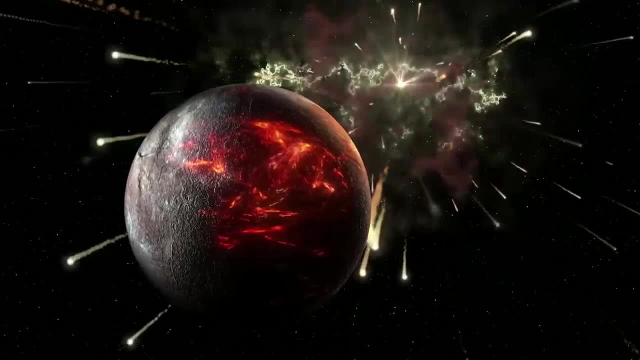 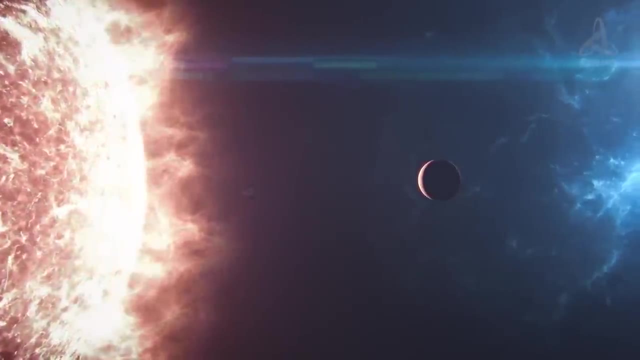 unlike planets in our solar system, where titanium oxide could reflect light and contribute to a brighter appearance, the atmospheric conditions on TRES-2b prevent such reflection. Instead, these elements absorb almost all of the sunlight that reaches the planet, trapping it as heat. This absorption is so efficient that it prevents the planet from reflecting light and light-absorbing chemicals. This is the reason why TRES-2b is so important to us, as astronomers and scientists alike. The atmosphere of TRES-2b contains a high concentration of light-absorbing chemicals, such as sodium oxide, potassium oxide and sodium oxide. 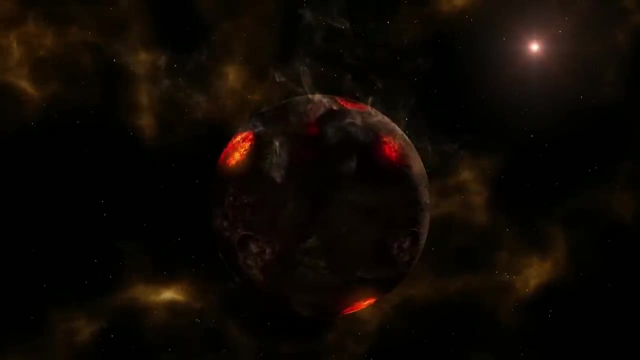 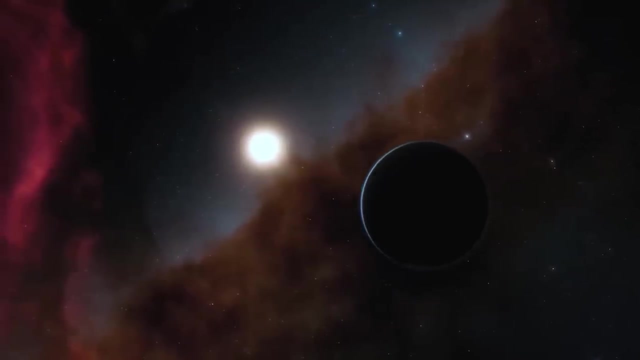 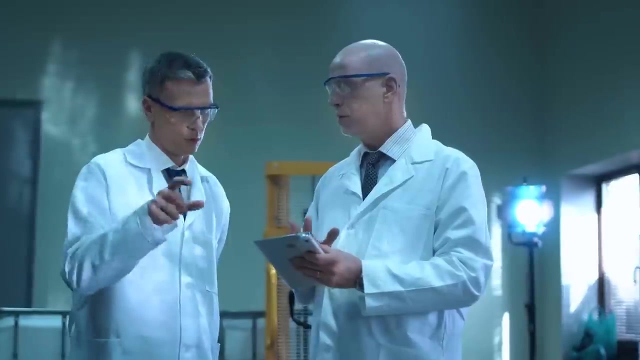 and these chemicals, when they are absorbed and absorbed back into space, account for its incredibly dark appearance. Another contributing factor to TRES-2b's darkness is the potential presence of unknown compounds in its atmosphere. Scientists speculate that these compounds could be responsible for the exceptionally 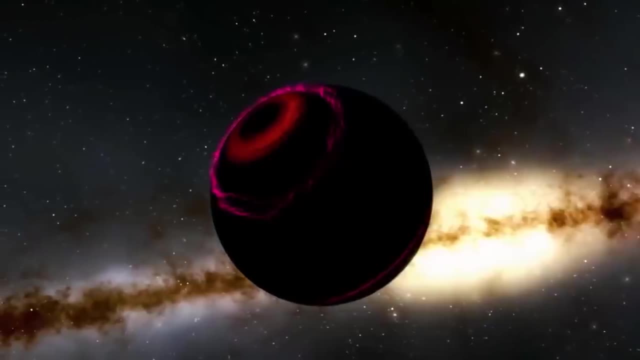 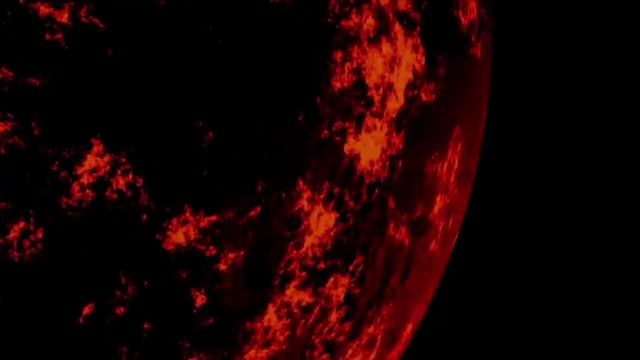 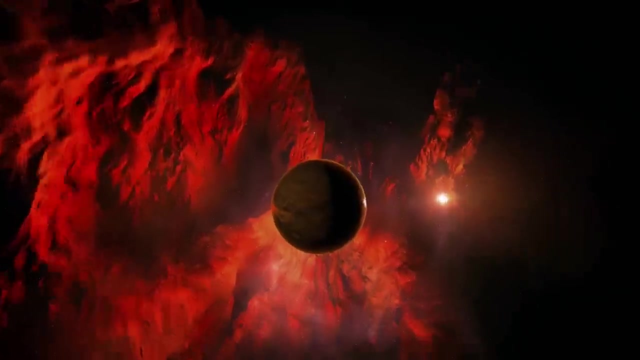 high level of light absorption, though the exact nature of these materials remains a subject of ongoing research. The high temperatures on the planet, which can reach up to 1,000 degrees Celsius, about 1832 degrees Fahrenheit, also play a significant role in maintaining its 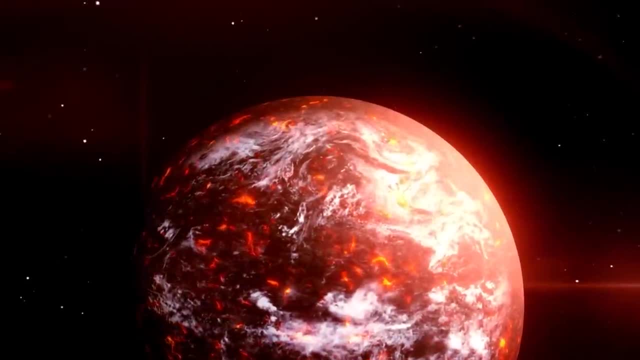 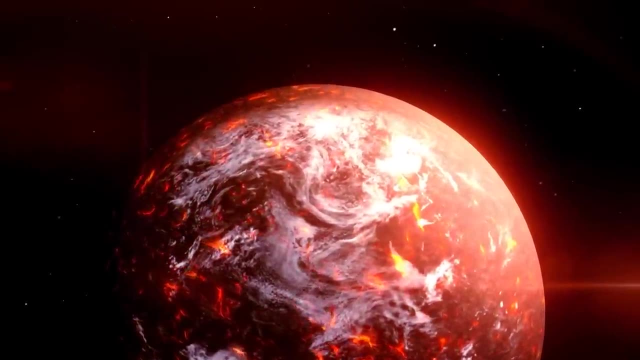 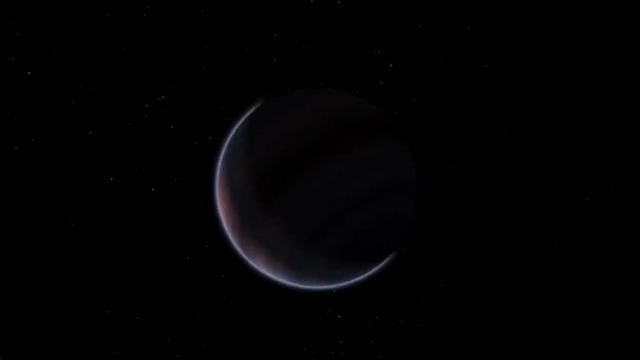 dark state. This heat further facilitates the chemical reactions that lead to the absorption of light rather than its reflection. One prevailing theory suggests that the atmosphere of TRES-2b is rich in molecules like vaporized sodium and potassium, both of which are known to absorb. 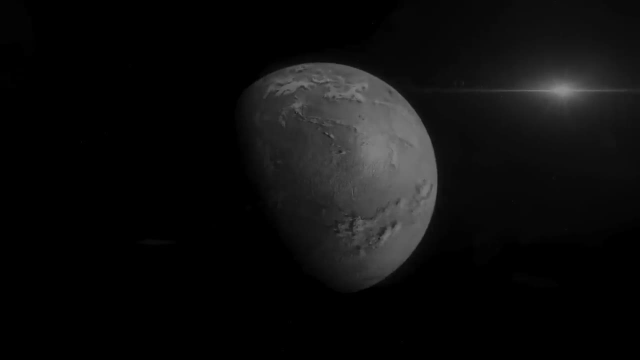 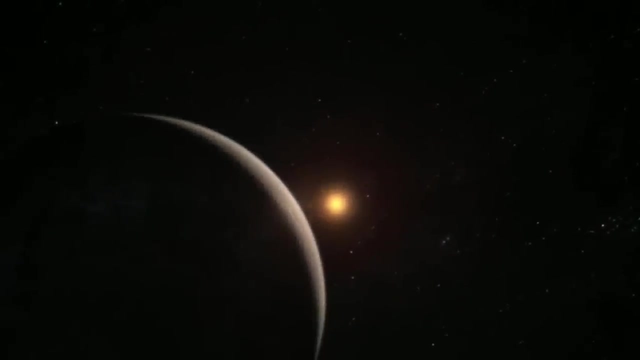 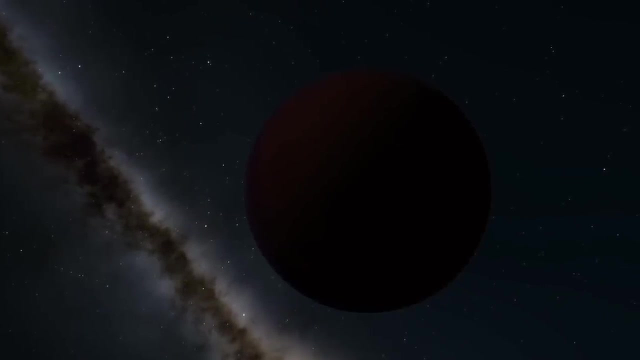 visible light. These elements in the high temperature environment of TRES-2b could contribute significantly to its dark appearance by preventing sunlight from being reflected back into space. Additionally, the presence of titanium oxide has been hypothesized In many planetary atmospheres. titanium oxide acts as a reflector of light. However, in the 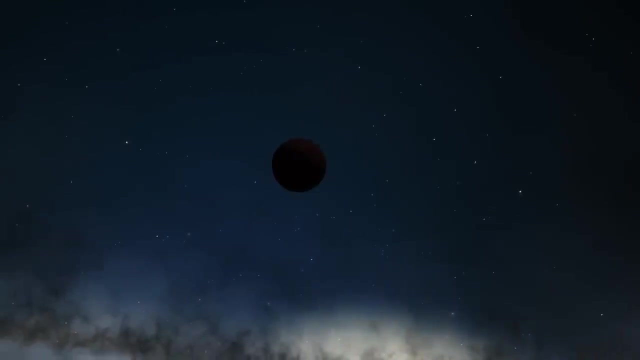 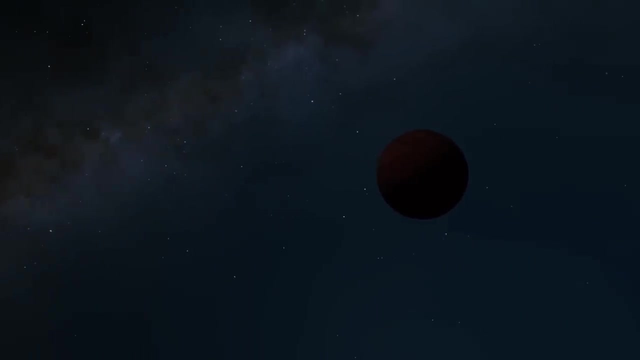 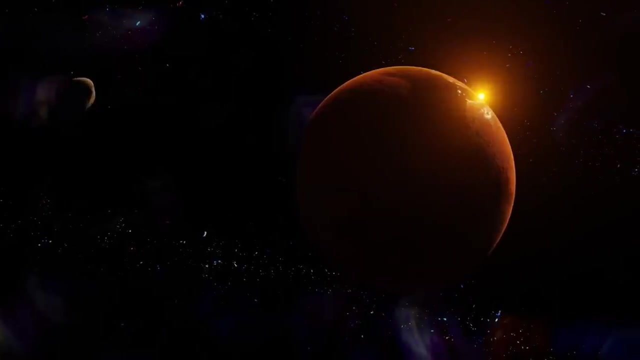 extreme conditions on TRES-2b, it may contribute to the absorption rather than the reflection. Beyond these known substances, researchers also speculate the existence of yet unidentified compounds in TRES-2b's atmosphere that could further enhance its light-absorbing capabilities. 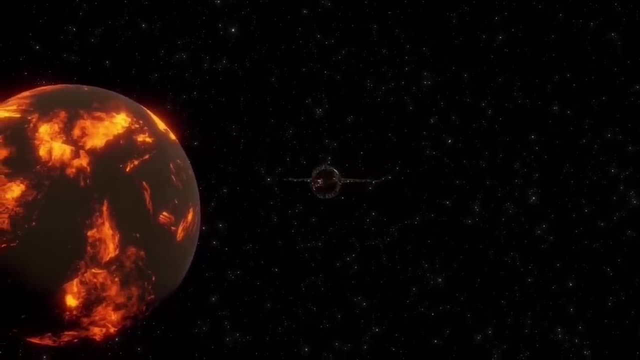 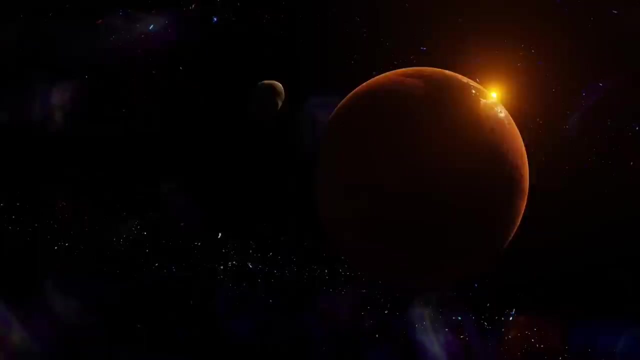 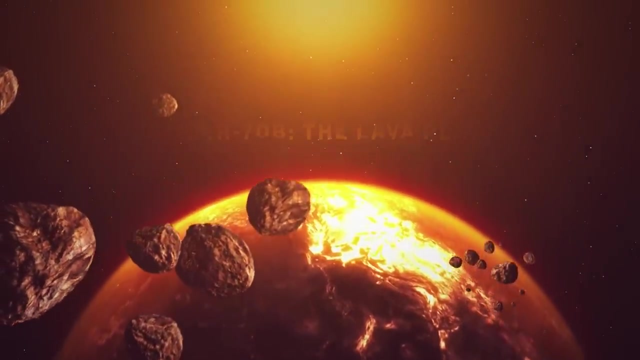 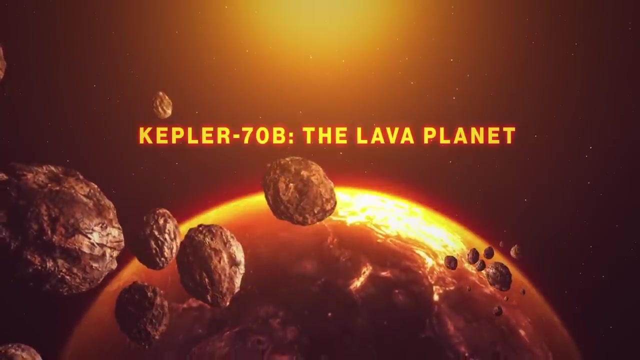 These unknown compounds are thought to play a crucial role in the planet's darkness, potentially representing new types of chemical processes that occur under the extreme temperatures and pressures found in the atmosphere. The Kepler-70b exoplanet is an exoplanet that exists in a realm of extreme heat, challenging our 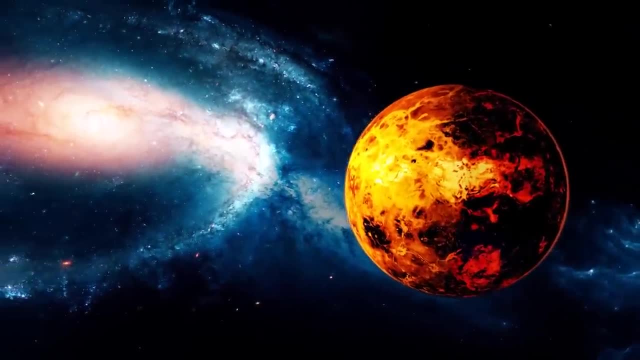 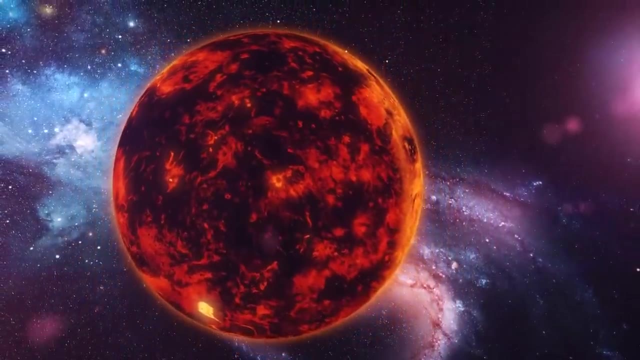 understanding of planetary climates. with its astonishing temperature range, Situated in a close orbit around its host star, Kepler-70b endures temperatures that are not even close to the temperatures that far exceed anything found on Earth or, indeed, most known planets. 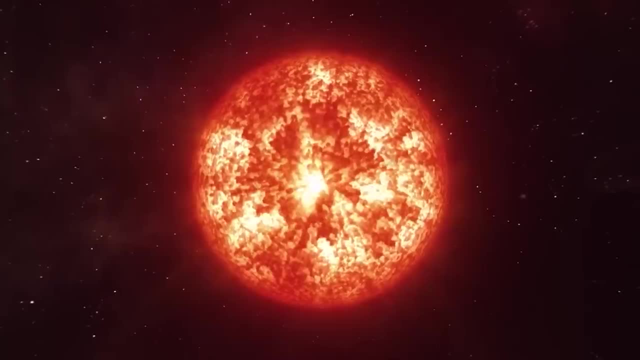 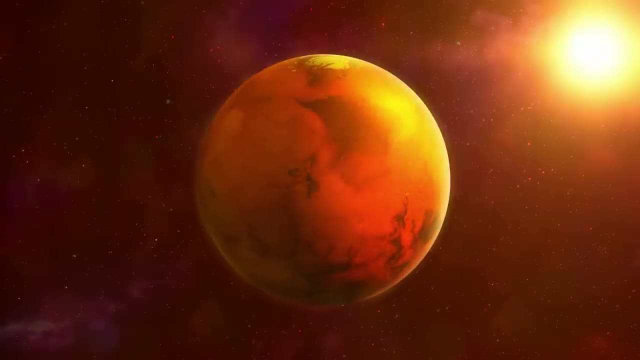 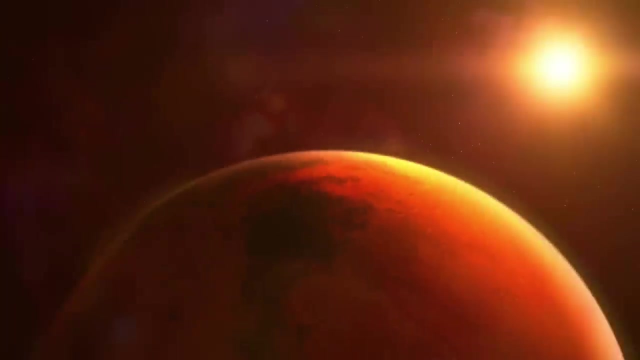 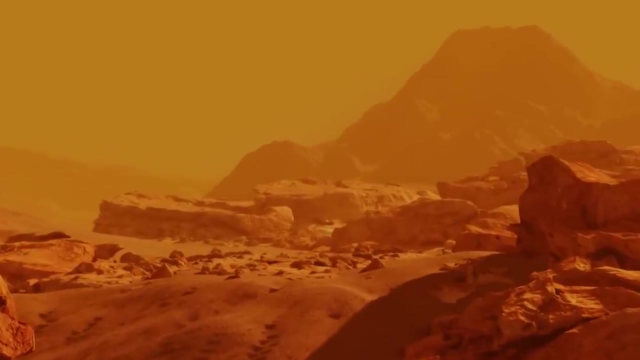 The temperature range on this celestial body can soar to between 6,700°C- approximately 12,092°F- and 7,300°C. This range places Kepler-70b among the hottest planets ever discovered, with surface conditions that resemble the outer layer of a star more than a planet's atmosphere. 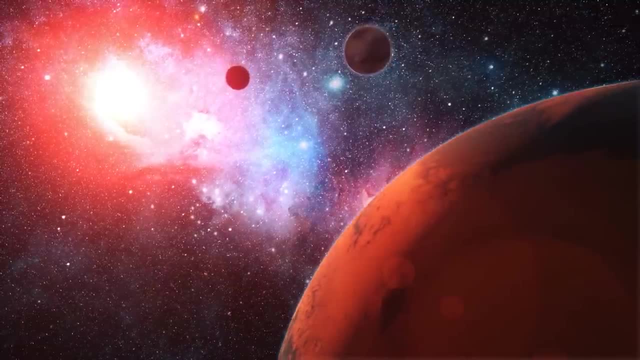 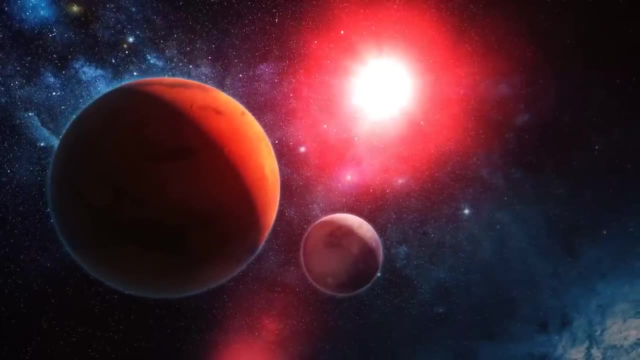 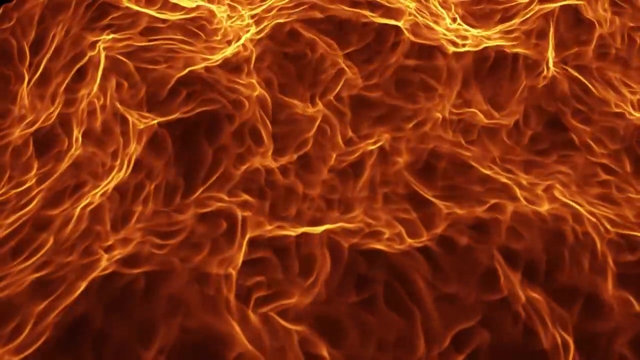 The extraordinary heat on Kepler-70b is primarily due to its proximity to its host star, Kepler-70, which it orbits at a remarkably close distance. This tight orbit results in extreme levels of stellar radiation bombarding the planet, heating its surface to temperatures that vaporize. 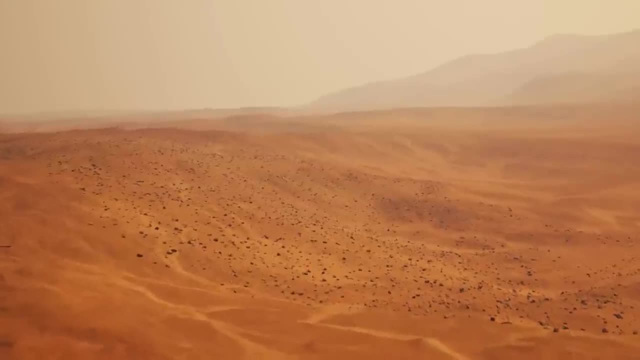 metals and rock, creating an environment that is not only inhospitable but almost unbearable. The Kepler-70b is a very powerful and highly sensitive planet, with a temperature of up to 5 degrees Celsius. The Kepler-70b is a very powerful and extremely sensitive planet, with 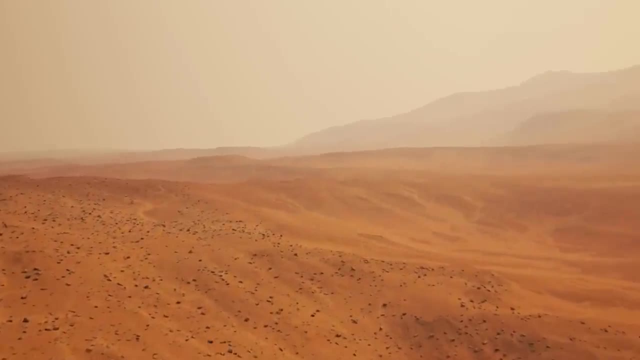 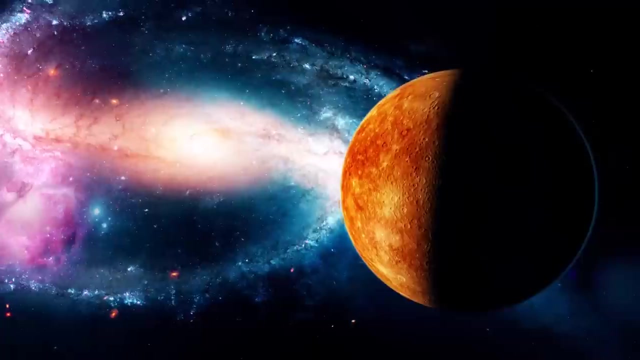 a temperature of up to 5 degrees Celsius. The Kepler-70b is a very powerful and extremely sensitive planet with a temperature of up to 5 degrees Celsius. The concept of day and night on Kepler-70b is irrelevant due to its close orbit leading. 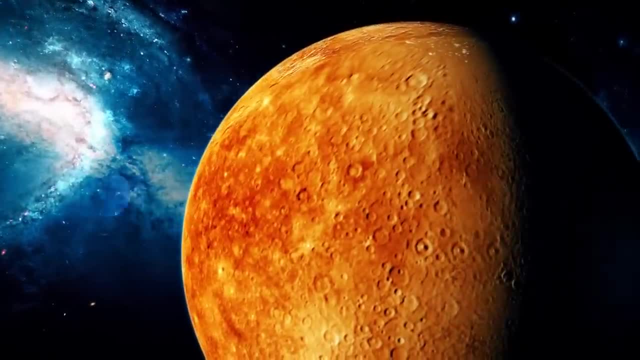 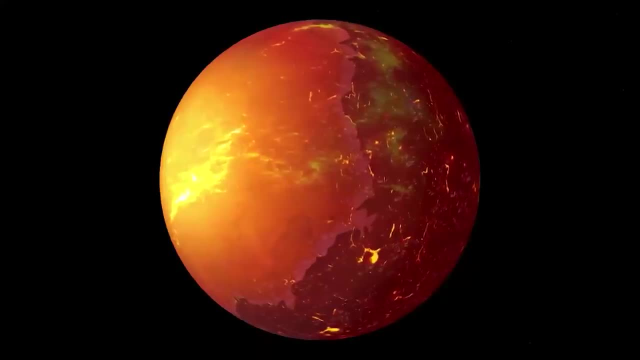 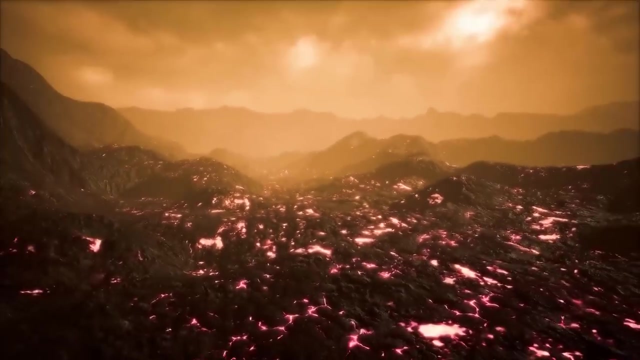 to nearly uniform temperatures across the entire surface that hover at the brink of what solid matter can endure before becoming plasma Transitioning. from the extreme temperatures of Kepler-70b, it's crucial to explore how its close proximity to its star profoundly influences the solar system. Kepler-70b is a very powerful and extremely sensitive planet. 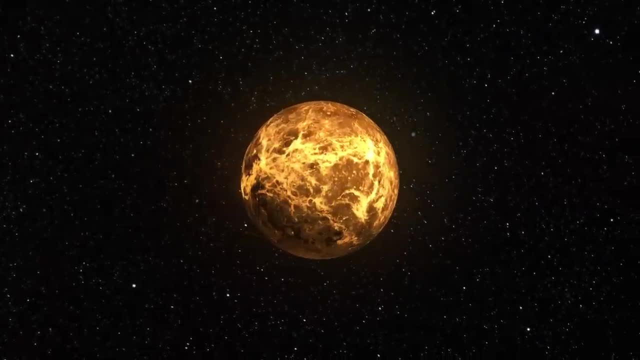 with a temperature of up to 5 degrees Celsius. Mediation hellenized the top half of its outer surface, Forging an environment that starkly contrasts with any terrestrial counterpart in planning implications. its энthris proves from any emotional result that early extraterrestrial 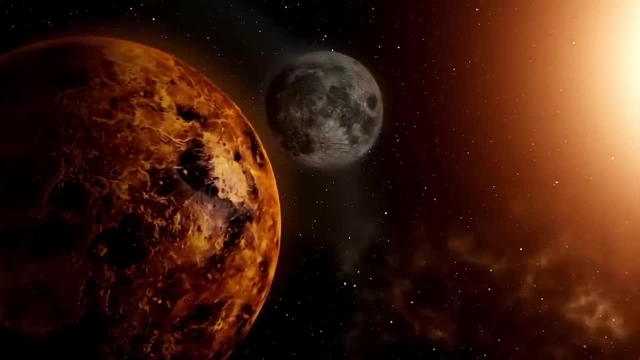 phenomena can continue to grab hold of the passing lightning in life. The intense stellar radiation that Kepler-70b receives due to its tight orbit around the host star Kepler-70 directly impacts the planet's physical characteristics, leading to a surface scenario that defies imagination. 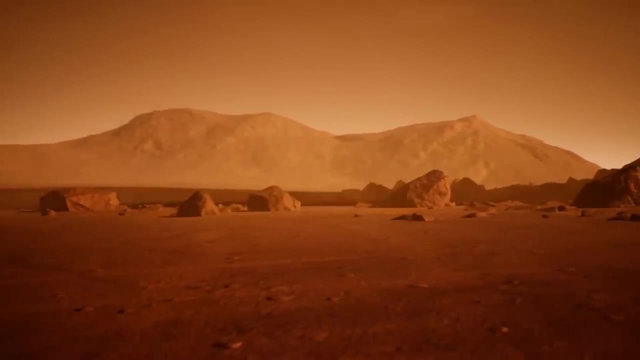 The heatingene Figad gorilla, trembling to low levels of heat from such close proximity to its star, causes the surface of Kepler-70b to reach temperaturesilos. вопрос: nuclear nor solar system's temperature, and even the temperature of its star can freezerly Deprived 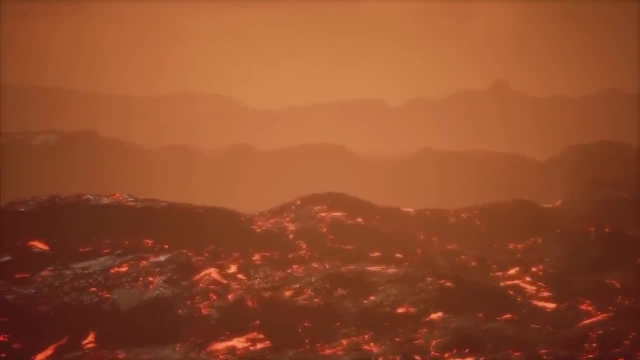 and September was 저희가's firstquaer- to concentrated, boundless temperatures of crack, live Temperatures where metals and rocks don't just melt, they vaporize. This results in a landscape that is in a constant state of flux. 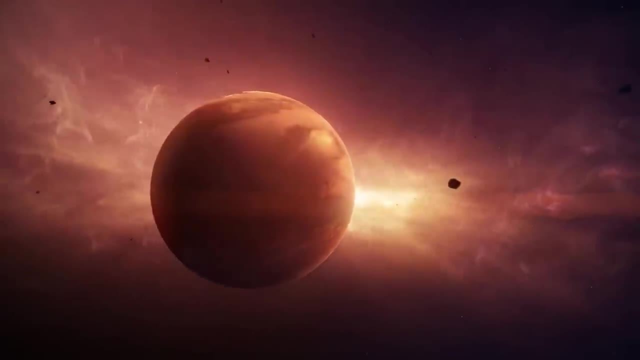 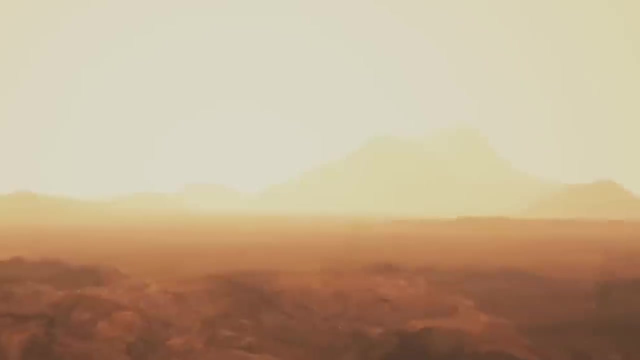 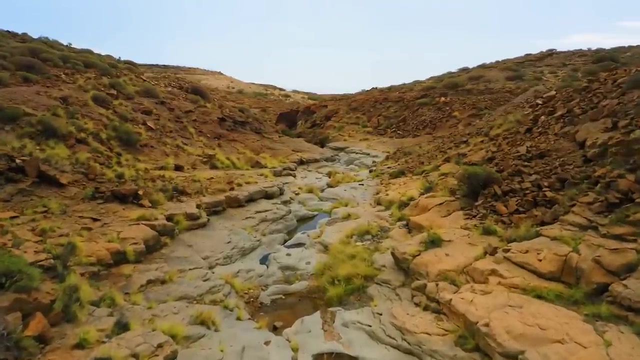 with surfaces that may be molten or partially vaporized during the planet's orbit. The extreme heat can create pools of liquid, metals and silicates, giving rise to a shimmering, reflective surface that could not be more different from the rocky or water-covered surfaces we are familiar with on Earth. 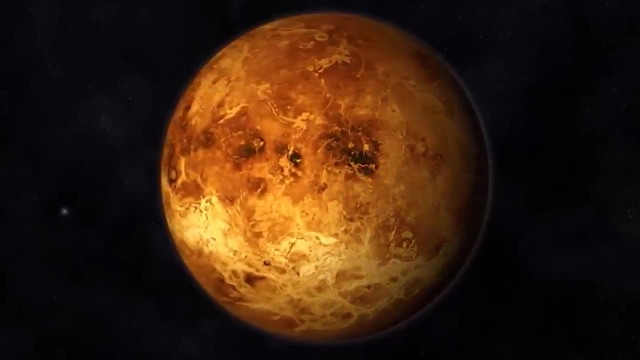 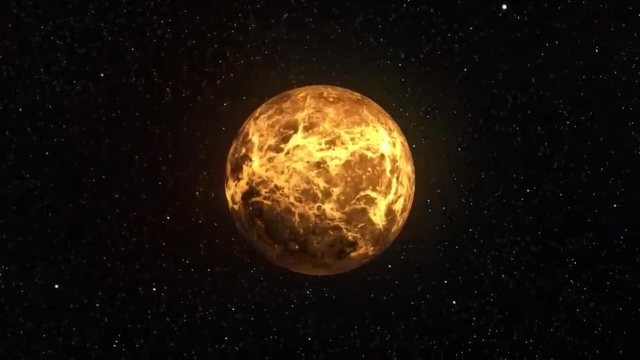 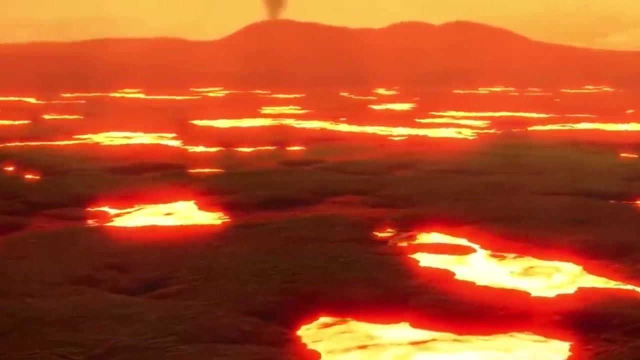 The gravitational forces at play due to the close orbit contribute to significant tidal stresses on Kepler-70b. These stresses can deform the planet, potentially causing volcanic activity or creating unusual geological formations. Such activity would further alter the surface of Kepler-70b. 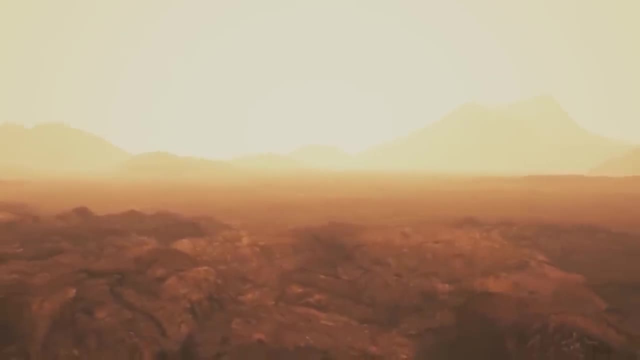 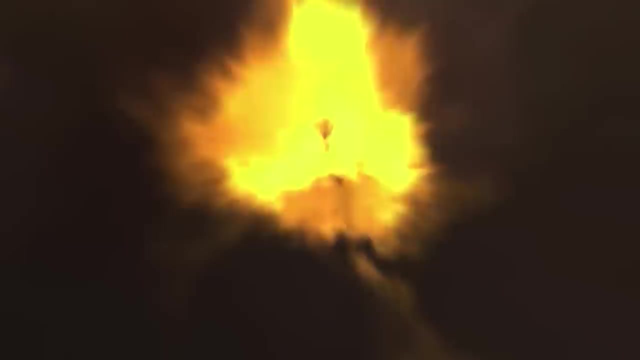 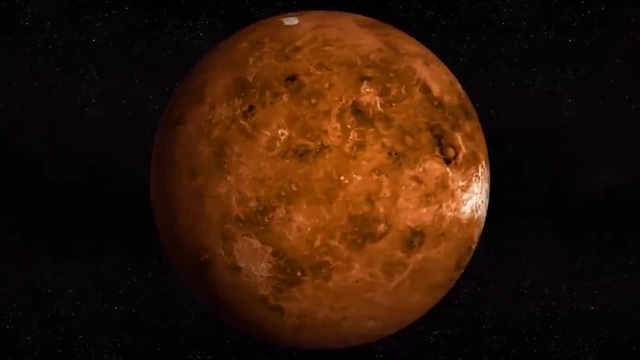 making it a dynamic and ever-changing world where the ground underfoot- if one could stand on it- is as transient as the atmosphere above. The extreme conditions found on Kepler-70b stand as a testament to the diverse environments that planets can endure. 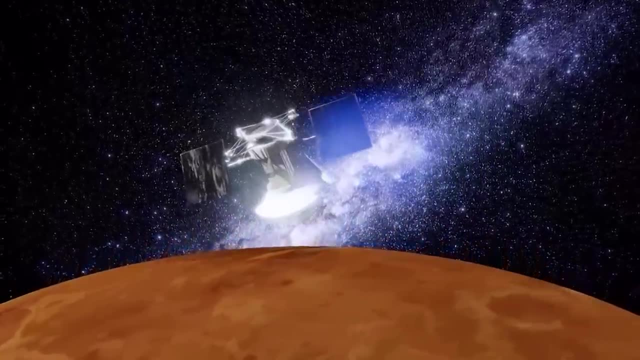 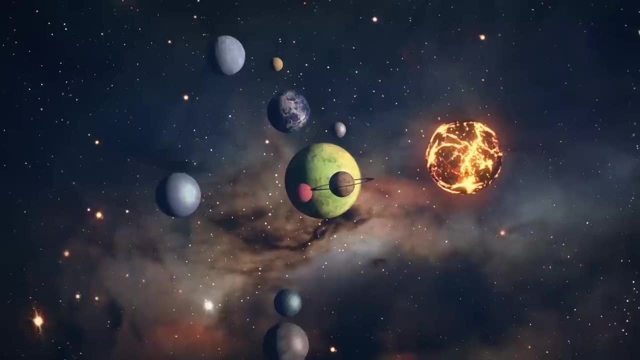 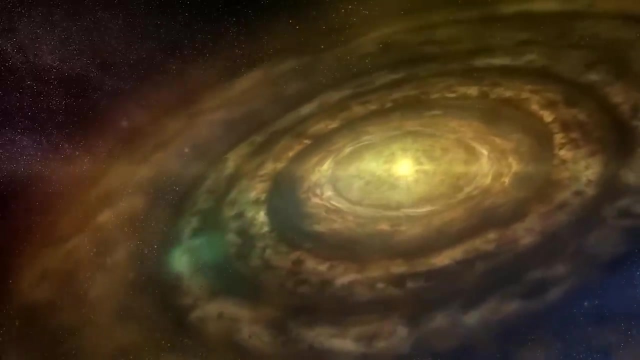 This diversity in turn offers a unique perspective on the processes that lead to planet formation and survival in the universe. The formation of planets, a process that has intrigued scientists for centuries, is influenced by a multitude of factors, including the composition of the universe. 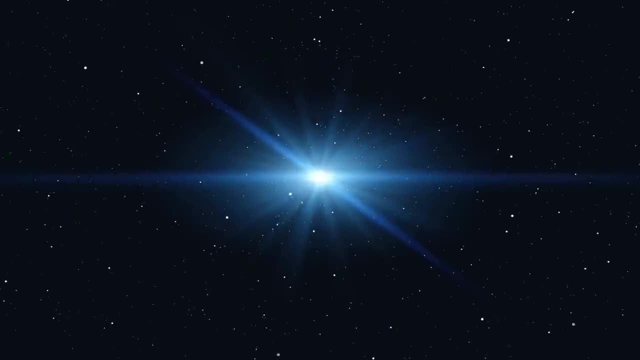 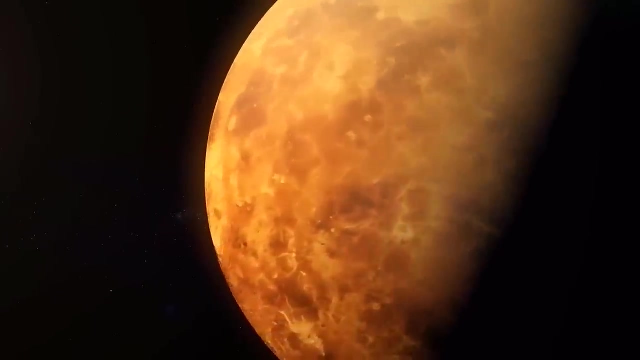 the structure of the protoplanetary disk, the distance from the host star and the star's characteristics. Kepler-70b's existence in such an inhospitable zone close to its star challenges existing models of planet formation, suggesting that planets can form and remain stable. 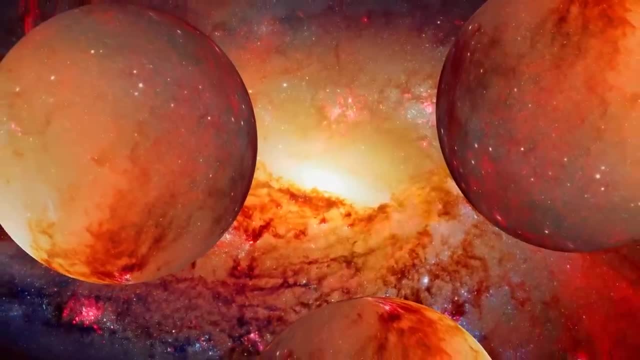 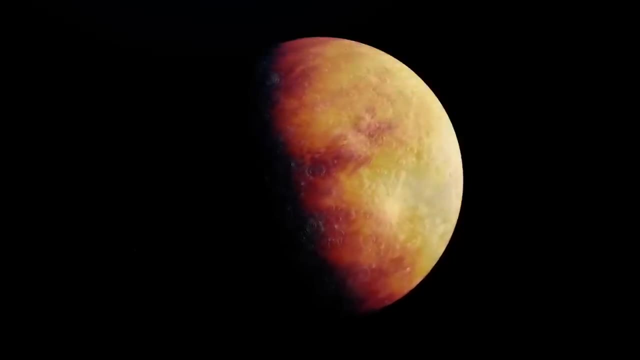 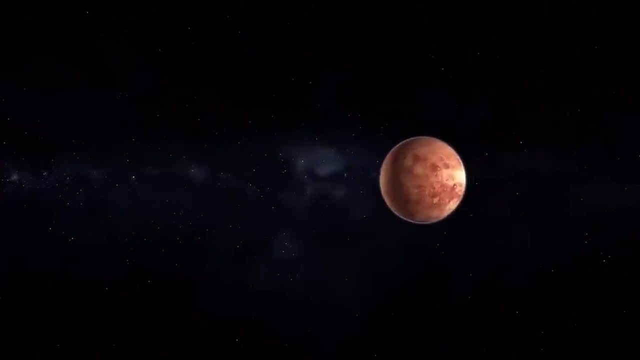 even in environments that would seem too extreme for such processes to occur. The survival of Kepler-70b in these conditions could indicate that planet formation mechanisms are more versatile and robust than previously thought, capable of resulting in stable celestial bodies even under severe thermal and gravitational stresses. 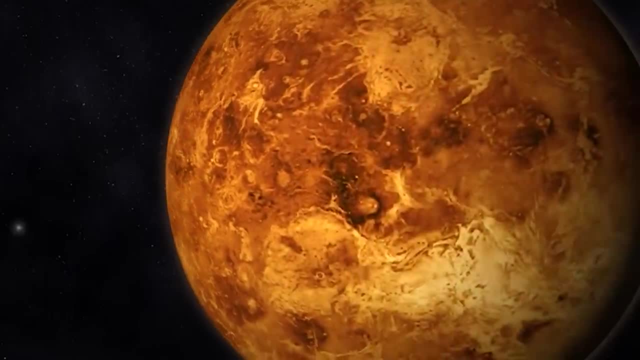 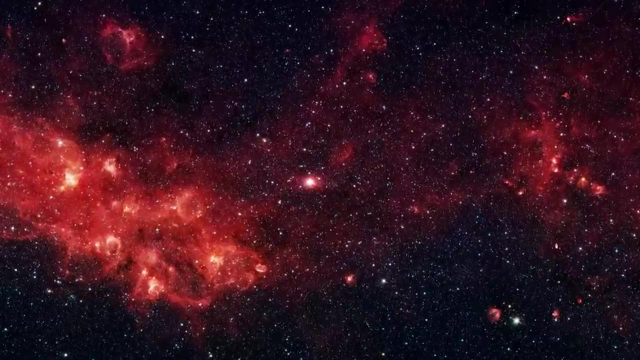 The study of Kepler-70b's extreme conditions can shed light on the end stages of planetary systems. As stars evolve and expand into their red giant phase, they can engulf the innermost planets, subjecting them to conditions similar to those experienced by Kepler-70b. 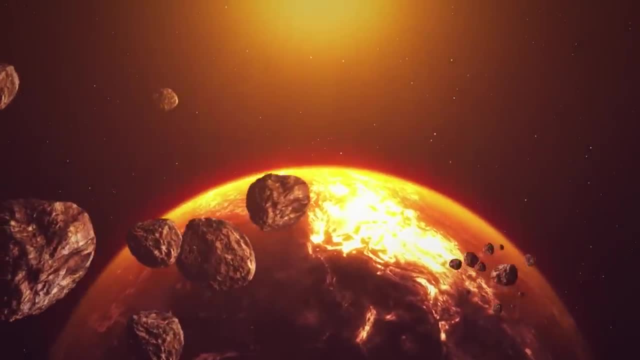 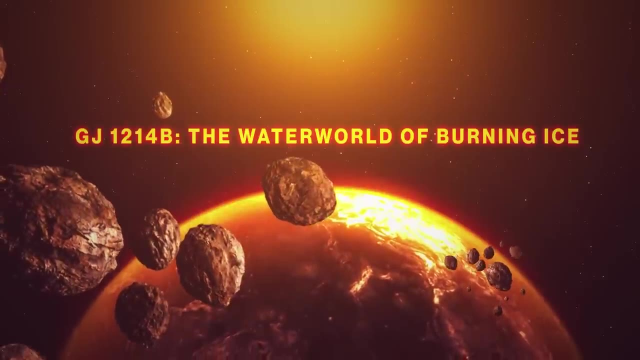 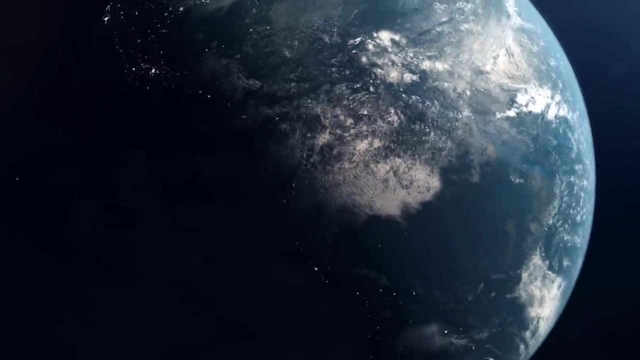 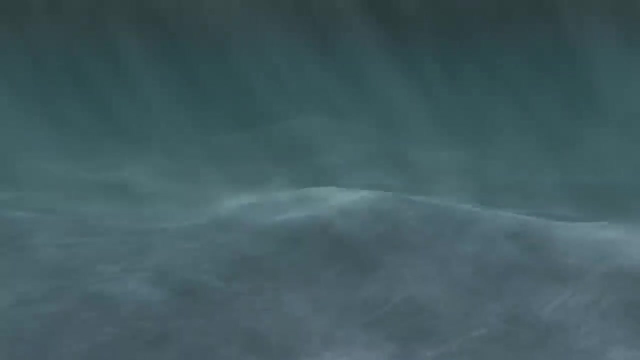 Kepler-70b, Planet GJ-1214b, an exoplanet located approximately 40 light years away from Earth, unveils a phenomenon that challenges our everyday understanding of water, Known as a super-Earth due to its size and mass, being larger than Earth's. 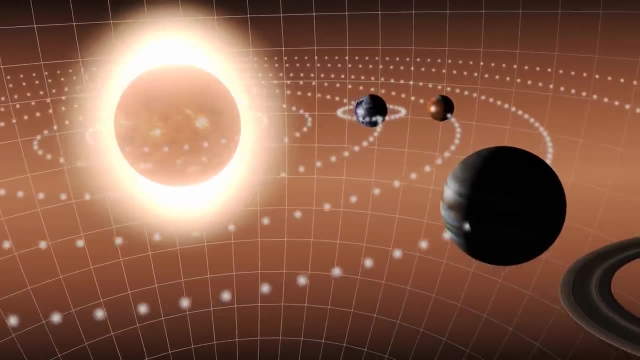 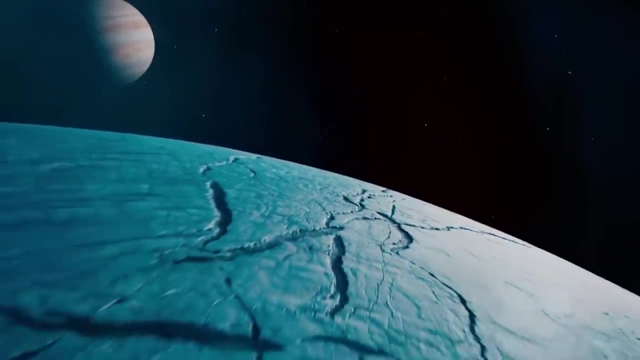 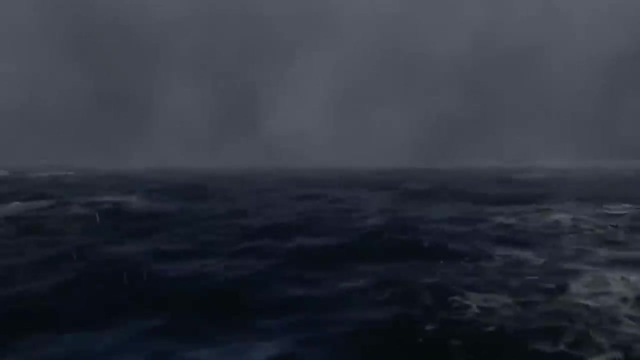 Earth's, but smaller than that of the gas giants in our solar system. GJ 1214b harbours conditions that give rise to what is colloquially referred to as burning ice. This term, while seemingly contradictory, describes a state of water that exists under the extreme pressure and temperature. 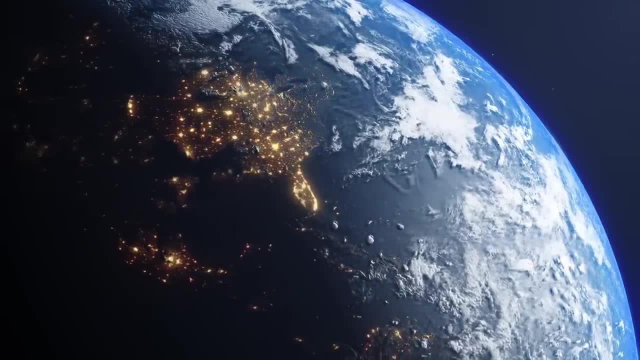 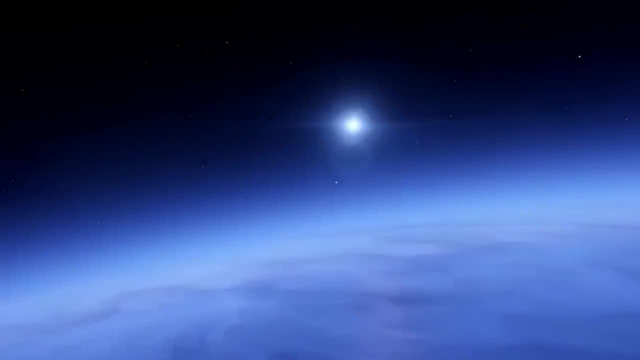 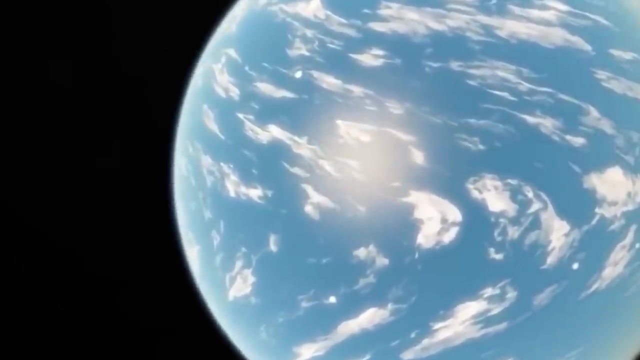 conditions found on the planet, a state that defies the familiar solid, liquid and gas phases known on Earth. The concept of burning ice on GJ 1214b stems from the planet's dense atmosphere and the profound depths of its potential oceans. Under the immense pressure exerted by the planet's 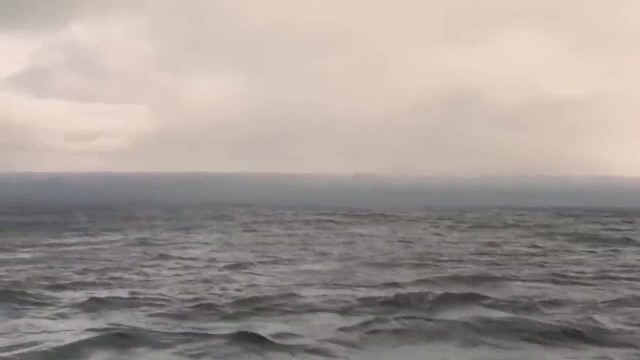 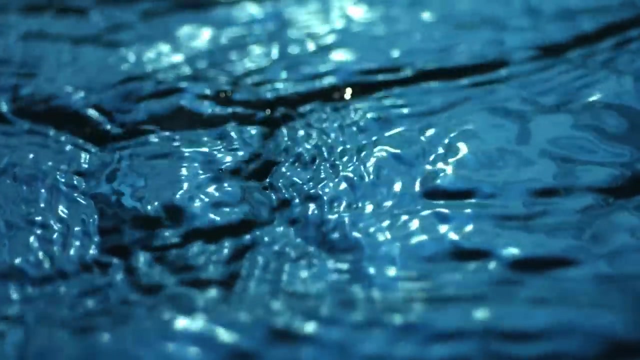 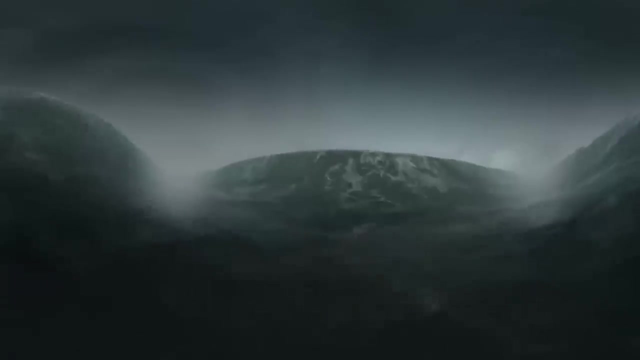 atmosphere, water assumes a form known as supercritical fluid, a phase that blurs the lines between liquid and gas. In this state, water retains some properties of a liquid, such as the ability to dissolve materials, While also acquiring characteristics typical of a gas, like filling a container to its shape. 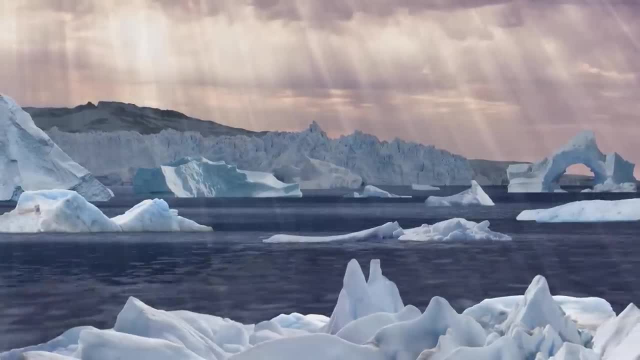 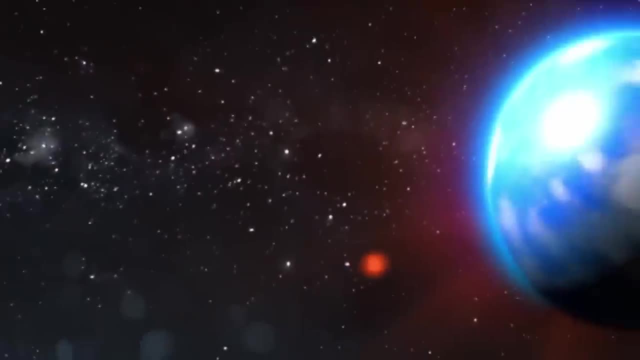 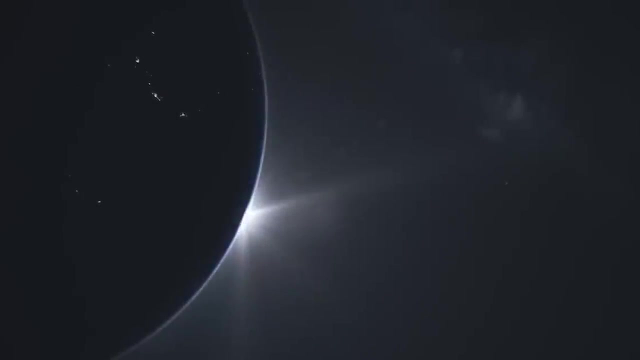 This supercritical water is not ice in the conventional sense, nor is it burning in terms of being a flame, but the extreme conditions under which it exists lead to its description as burning ice. The temperatures on GJ 1214b contribute to this phenomenon as well. 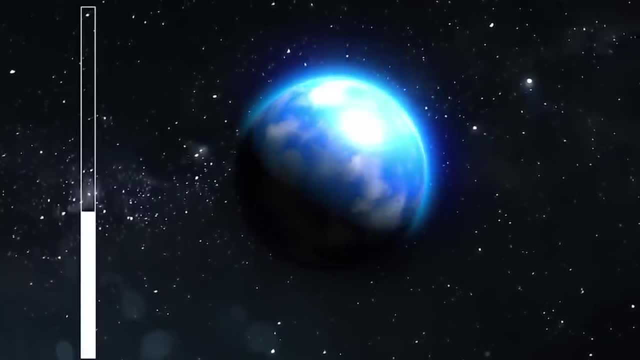 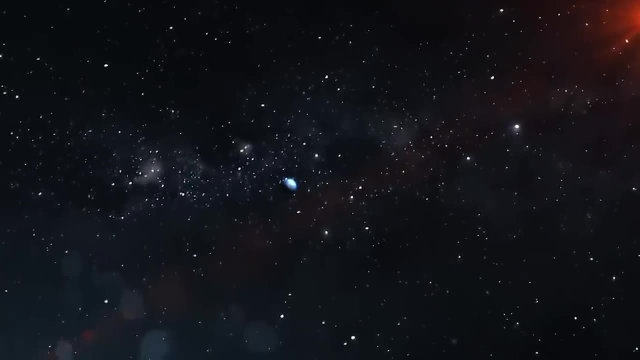 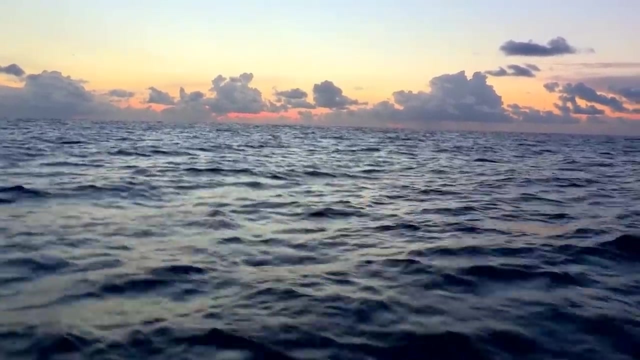 While not as scorchingly hot as some exoplanets, the temperature is sufficiently high to prevent water from existing in a familiar liquid state at the surface level. assuming instead this exotic supercritical phase, This condition creates an environment where water behaves unlike anything we experience on Earth with. 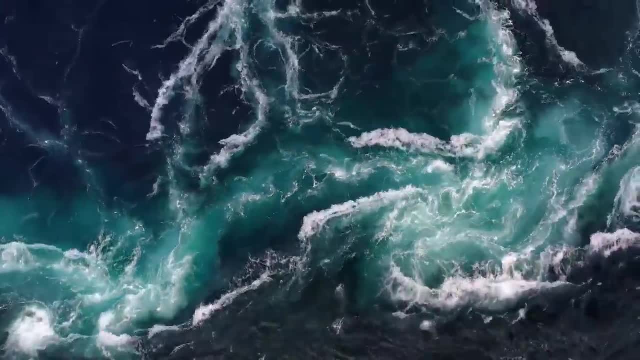 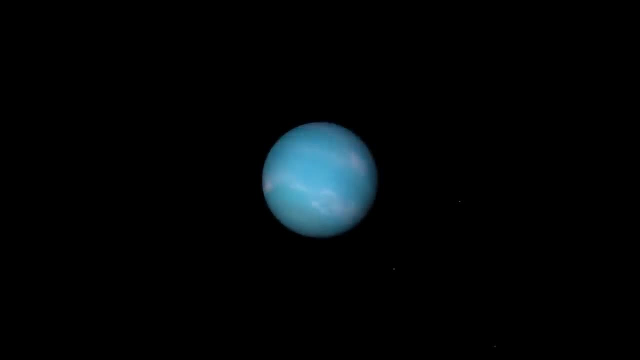 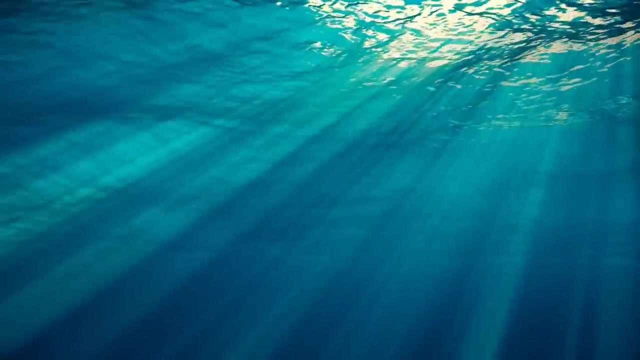 the capability of both dissolving materials like a liquid, and permeating spaces like a gas. The pressure on GJ 1214b presents a stark contrast to the pressures found in Earth's deepest oceans, pushing the limits of our understanding of extreme environments. Earth's oceans, while profound and mysterious in their 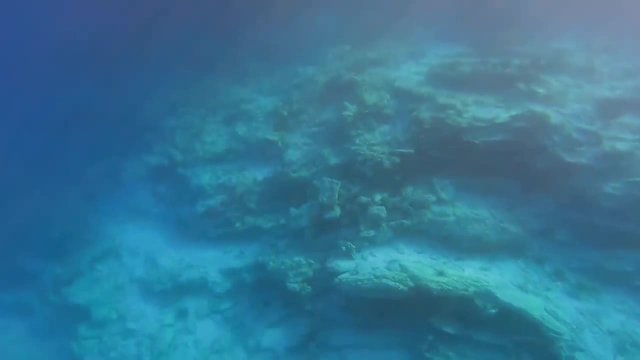 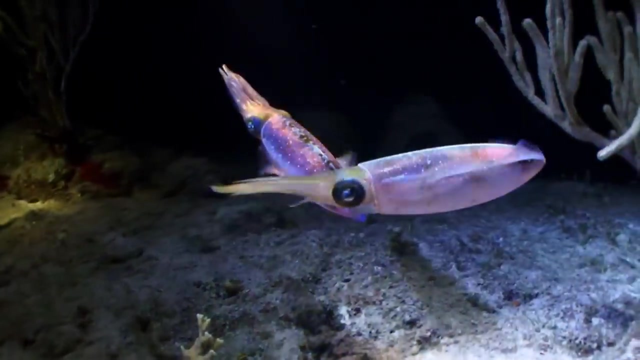 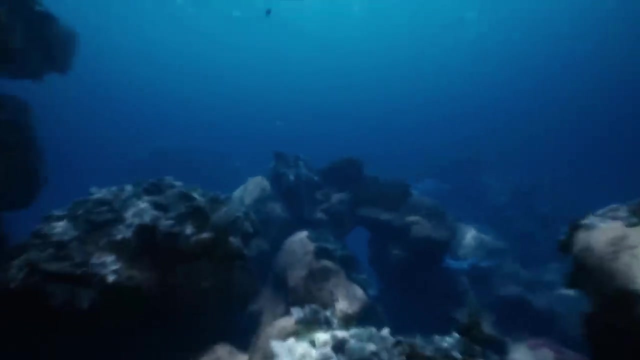 own right reach their greatest depths in the Mariana Trench, where the pressure soars to about 1,086 bars, or around 15,750 psi. This is equivalent to experiencing the weight of an elephant standing on a postage stamp, a comparison that vividly illustrates the intense pressure at such depths. However, when we turn our gaze to GJ 1214b, the concept of pressure enters a whole new realm of intensity. The atmospheric pressure on GJ 1214b is estimated to be thousands of times greater than the pressure at the deepest point of Earth's oceans. This immense pressure. 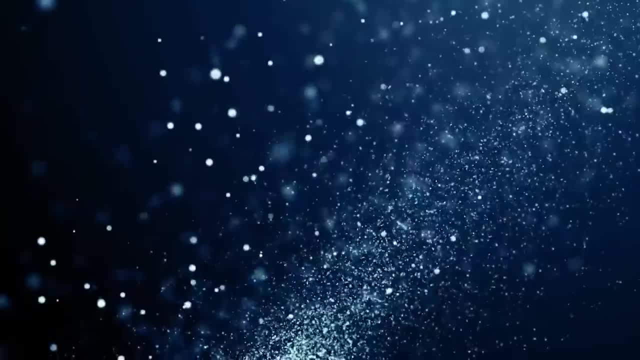 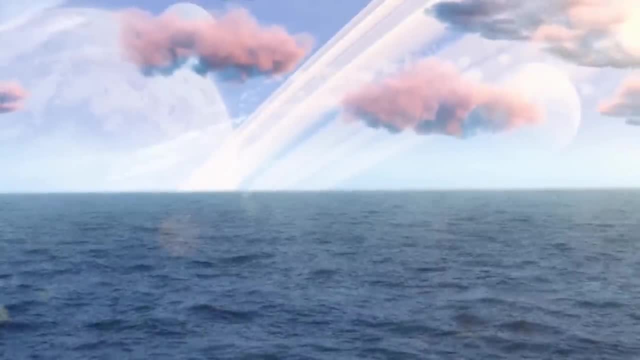 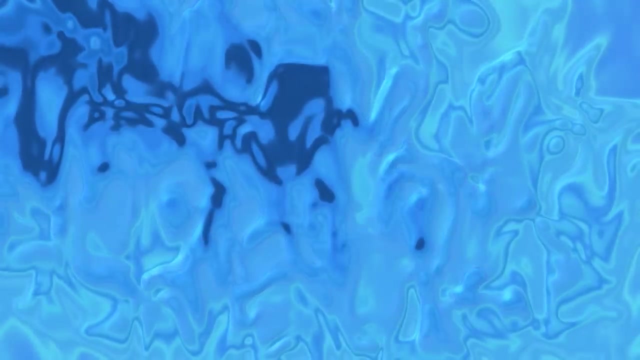 is due to the planet's larger mass and density, combined with a thick atmosphere that is like, likely composed of heavy molecules. Under such conditions, water and other substances undergo dramatic transformations, entering exotic phases, like the supercritical fluid state mentioned earlier, where traditional distinctions between gases and liquids no longer apply. 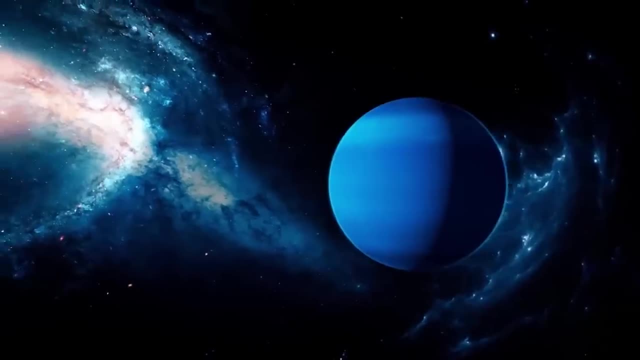 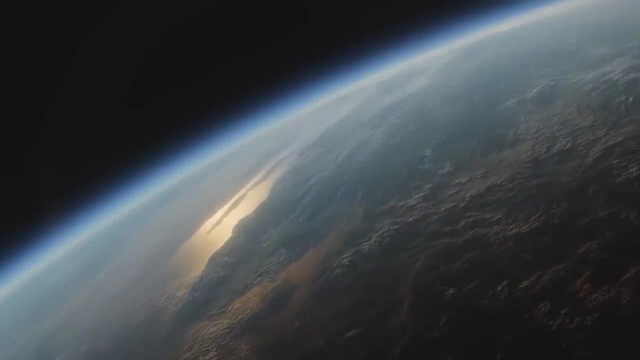 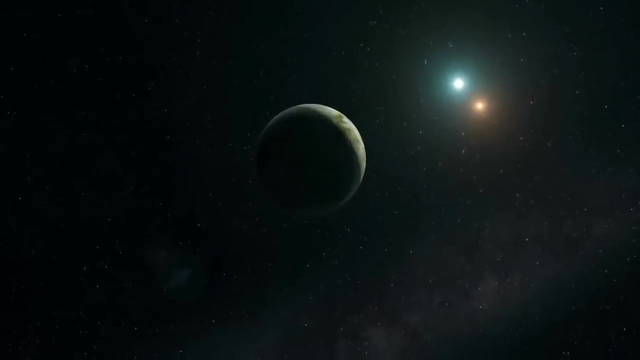 Studying GJ 1214b, with its intriguing characteristics and distant location, presents a unique set of challenges for scientists. These challenges stem from both the technological limitations of current observational tools and the inherent difficulties of interpreting data from such a remote exoplanet. 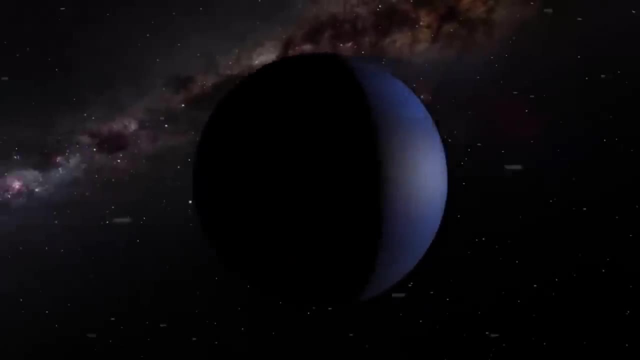 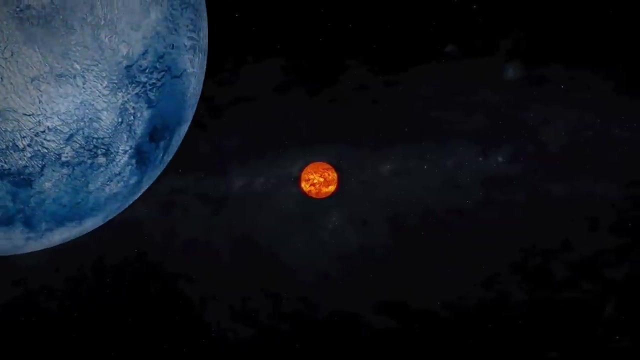 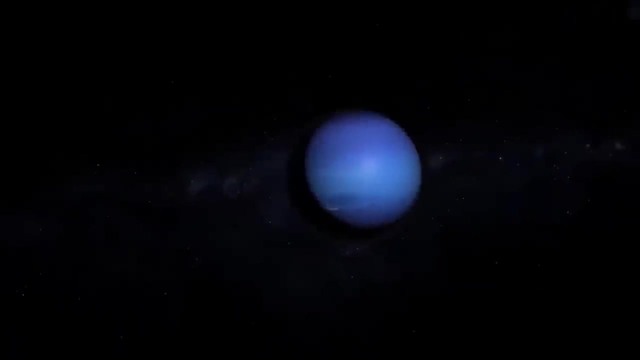 One of the primary hurdles in studying GJ 1214b or any exoplanet of similar distance and composition is the vast expanse that separates us from these celestial bodies Located approximately 40 light-years away from Earth. GJ 1214b. 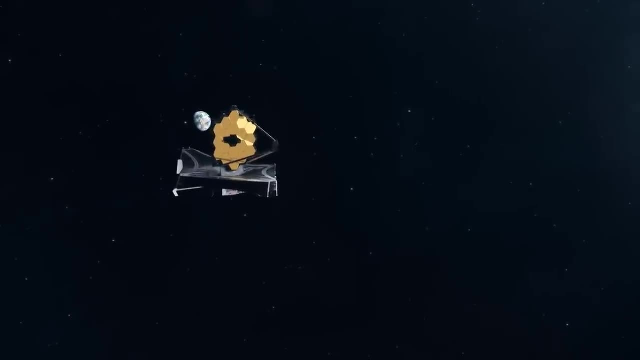 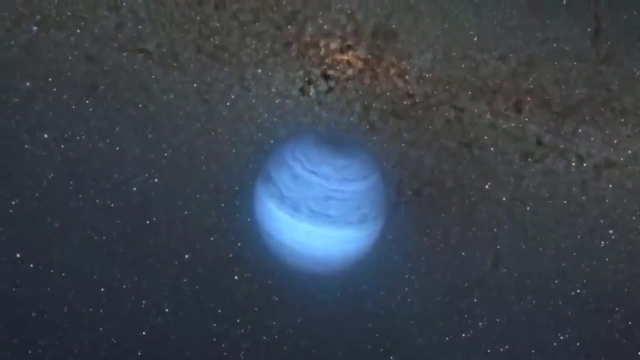 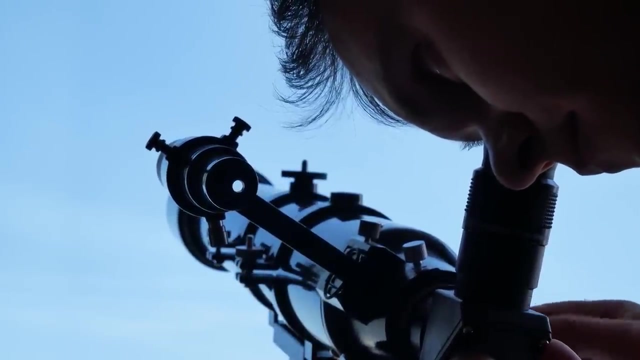 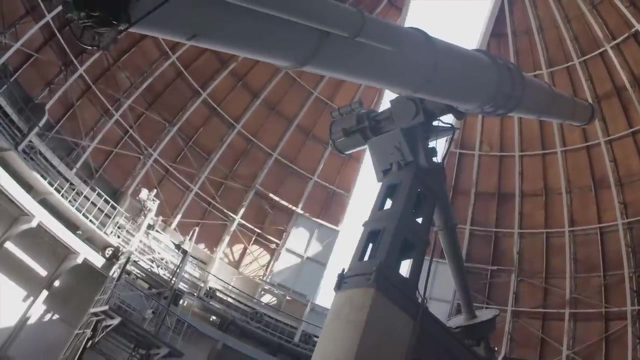 requires advanced telescopes equipped with highly sensitive instruments to detect and analyze its atmospheric composition, temperature and other vital characteristics. Another significant challenge is the resolution and sensitivity of current astronomical instruments. While technological advancements have dramatically improved our ability to observe distant planets, there are still limitations in detecting the finer details of an exoplanet's atmosphere. 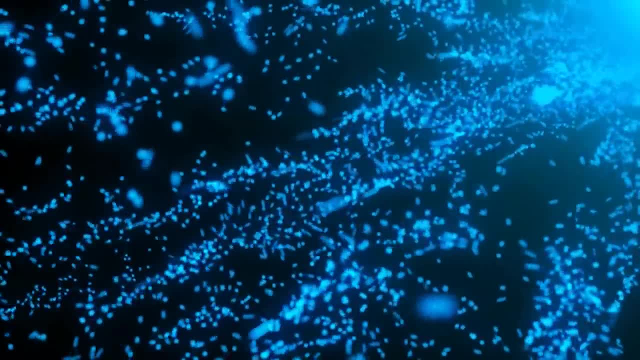 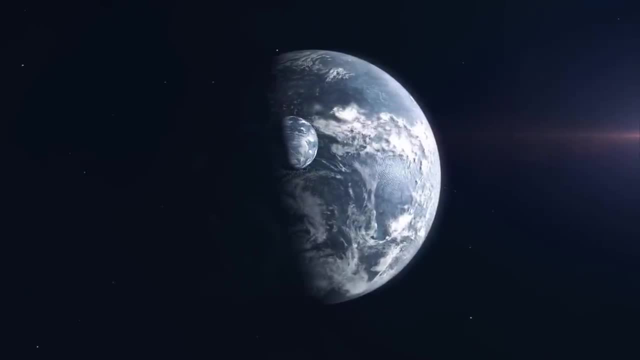 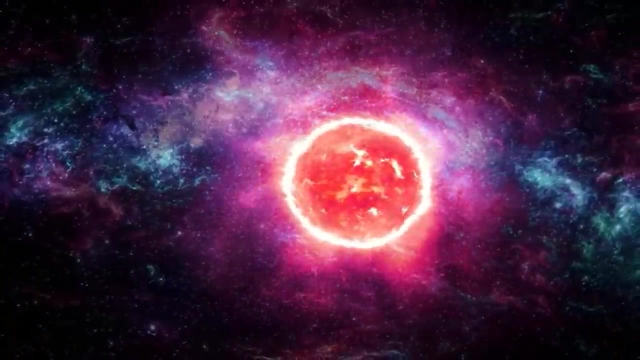 Especially when it comes to identifying specific molecules or understanding the dynamics of atmospheric conditions. This is compounded by the fact that the signals from these planets are often obscured or diluted by the overwhelming brightness of their host stars, making it difficult to isolate the specific characteristics of the planet from the light it reflects or emits. 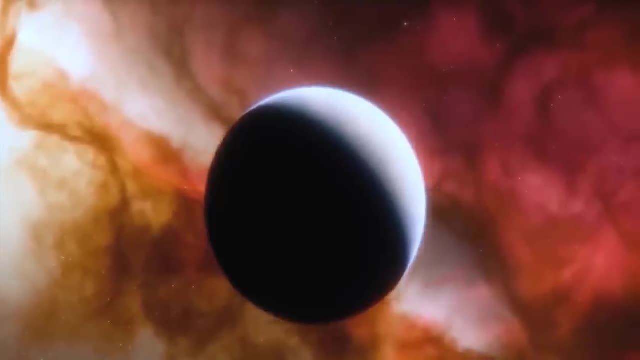 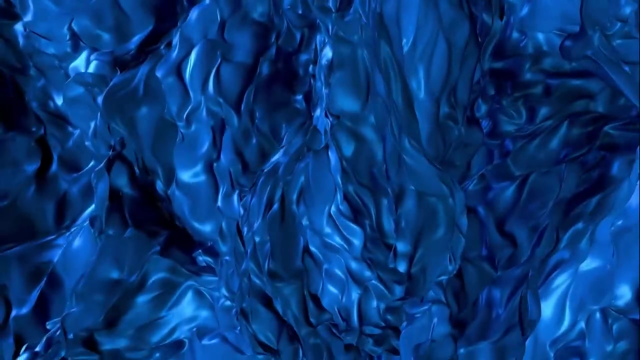 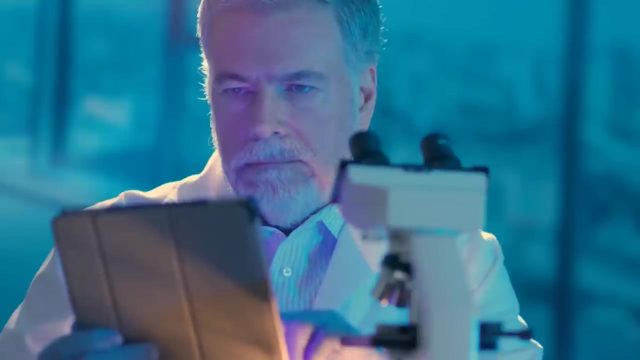 The interpretation of data from GJ 1214b is complicated by our limited understanding of how certain conditions, such as supercritical fluids, behave under the extreme pressures and temperatures found on such planets. Scientists rely on theoretical models and laboratory experiments to simulate these conditions. 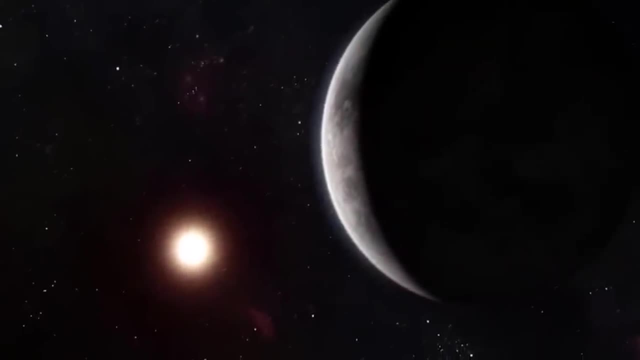 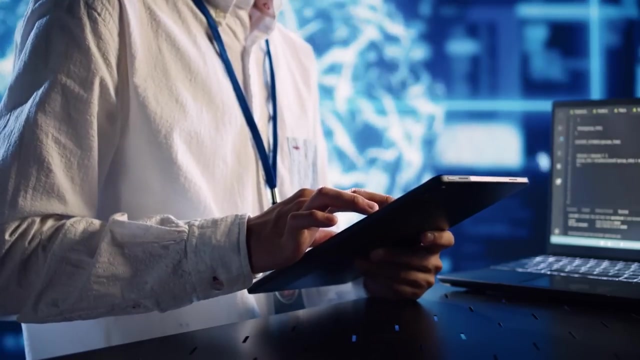 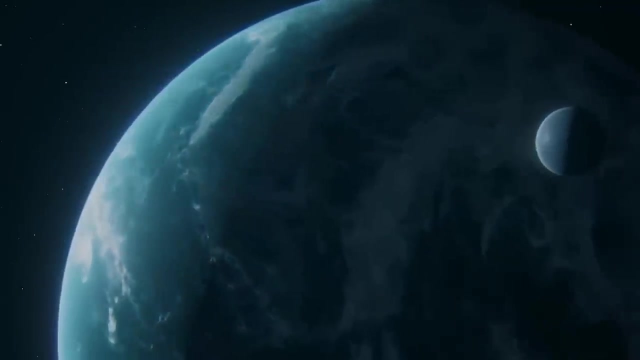 but these models have their limitations and cannot perfectly replicate the complex environments of distant exoplanets. As a result, there is an ongoing effort to refine these models and develop new techniques to better understand the data we receive from observations of GJ 1214b. 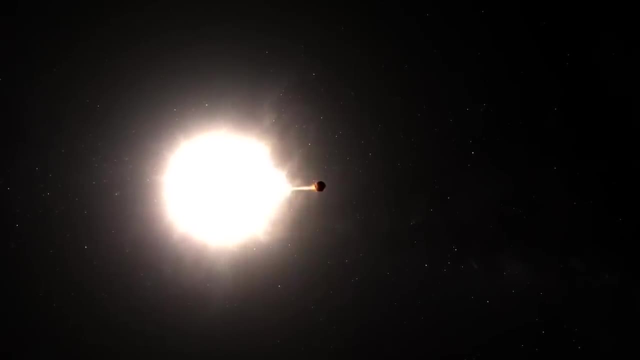 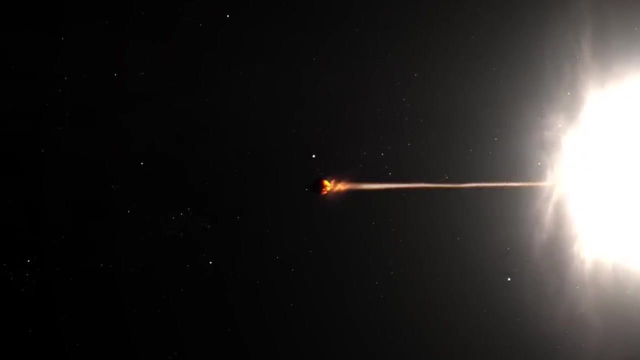 GJ 1214b, an exoplanet located approximately 600 light-years from Earth, has been dubbed a doomed planet due to its perilously close orbit around Earth, Leading to a grim fate that has captivated both scientists and the public alike. 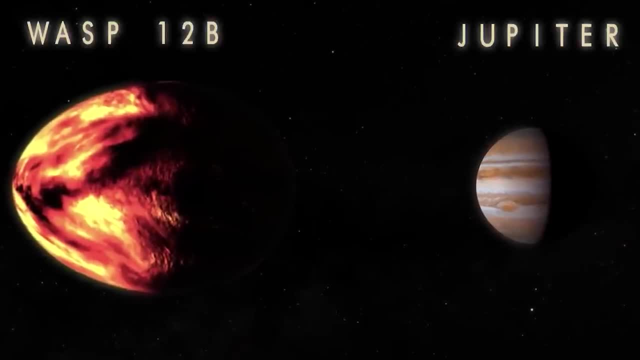 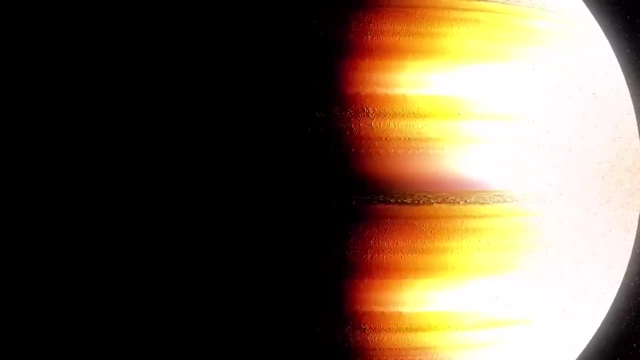 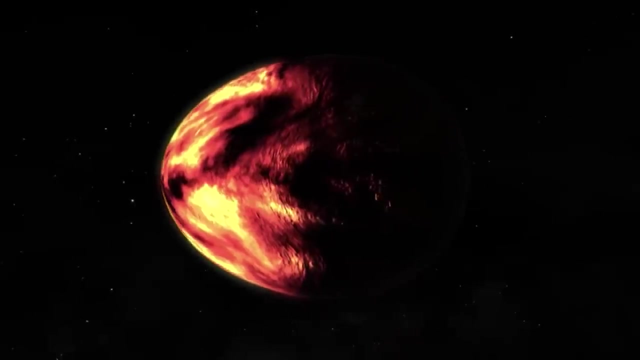 This gas giant, roughly the size of Jupiter, is being gradually consumed by its star, a process that offers a stark illustration of the destructive forces that can shape the life cycle of planets. The primary reason GJ 1214b is considered doomed lies in its incredibly close proximity to its host star, GJ 1214b. 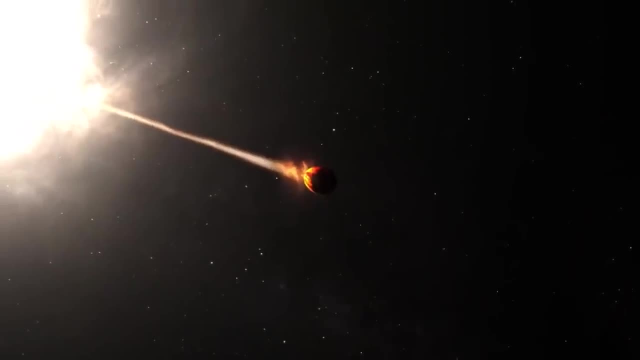 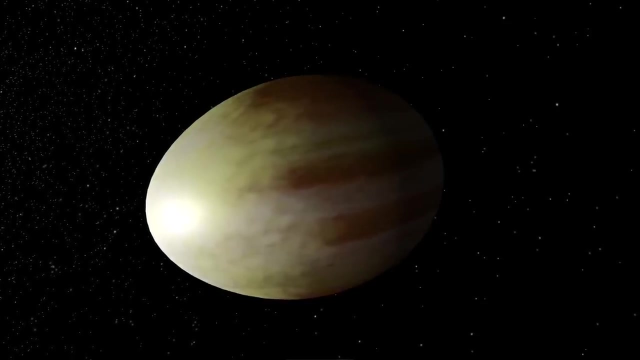 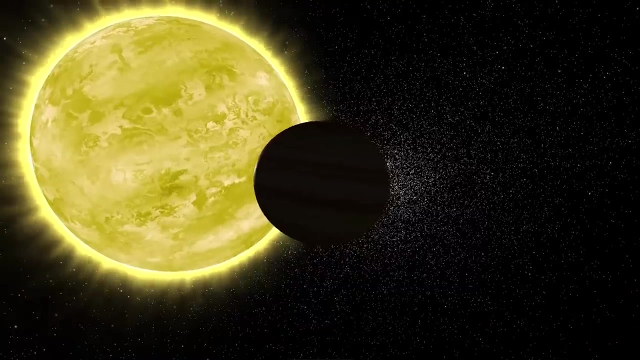 This proximity results in extreme gravitational forces exerted on the planet, causing it to become tidally locked, meaning one side of the planet always faces the star, while the other side remains in perpetual darkness. The side of GJ 1214b that faces the star experiences intense heat. 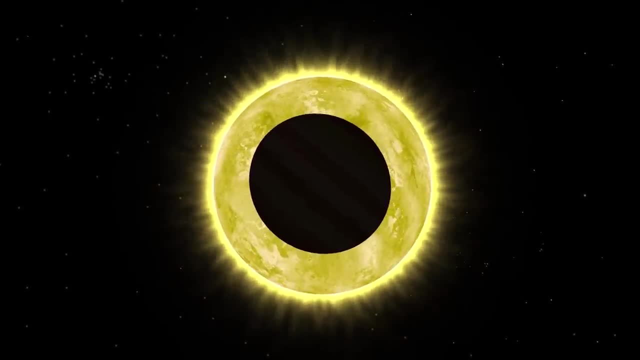 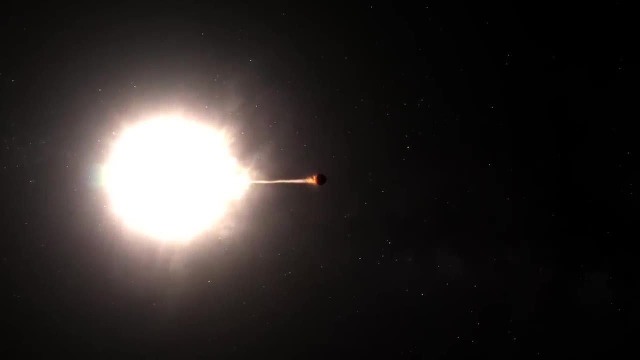 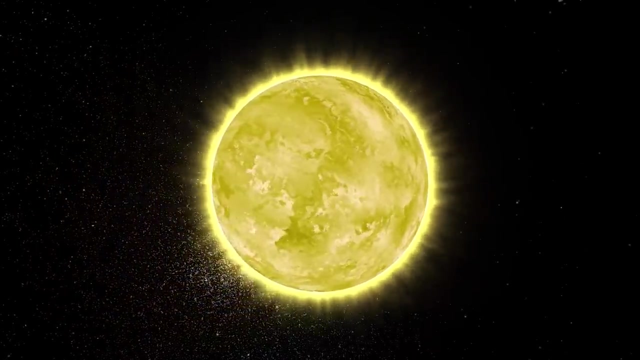 with temperatures soaring to over 2,500 degrees Celsius, about 4,532 degrees Fahrenheit, leading to the planet's atmosphere being blown away into space. The intense gravitational pull from the star has caused GJ 1214b to take on an elongated, egg-like shape. 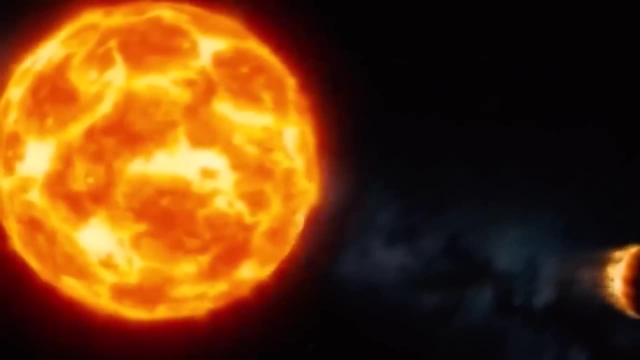 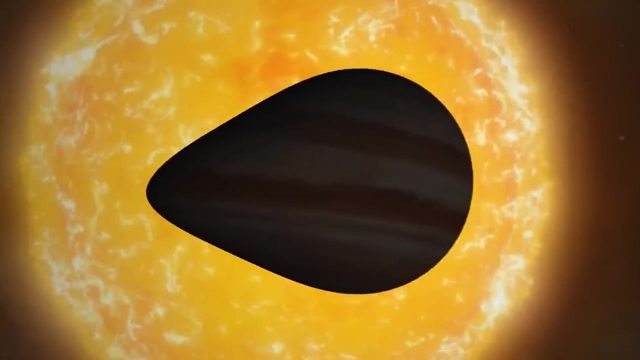 rather than the spherical shape typical of planets. This deformation is a clear indicator of the star's powerful influence on the planet. Observations have revealed that GJ 1214b is losing mass at a rate of about 189 quadrillion tons per year. 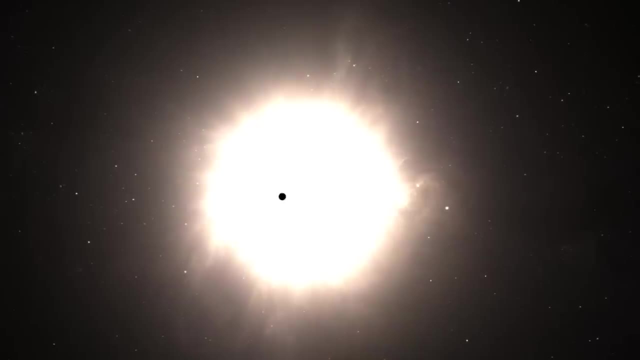 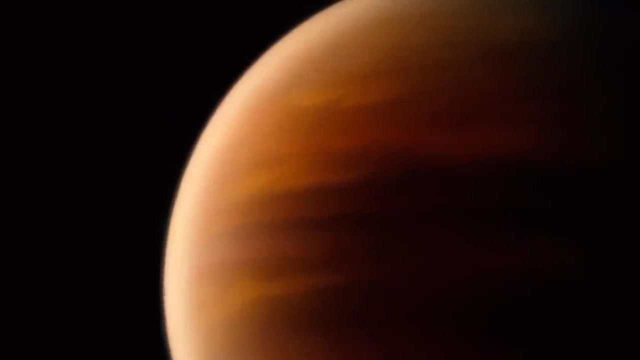 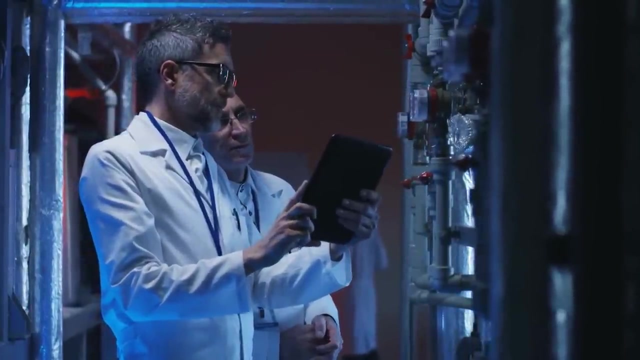 a significant portion of its total mass. This loss is due to the star's heat and gravitational pull stripping away the planet's outer layers, a process known as atmospheric escape. Scientists predict that within a relatively short astronomical timeframe, possibly as little as 10 million years- 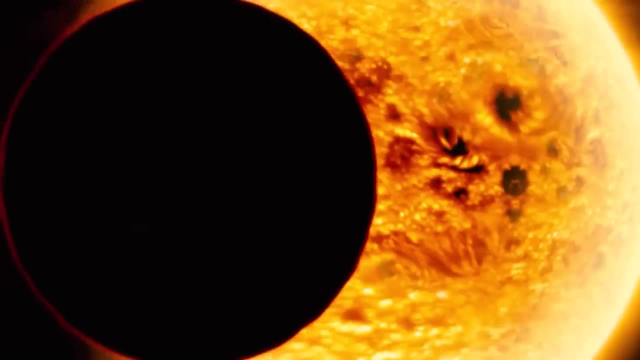 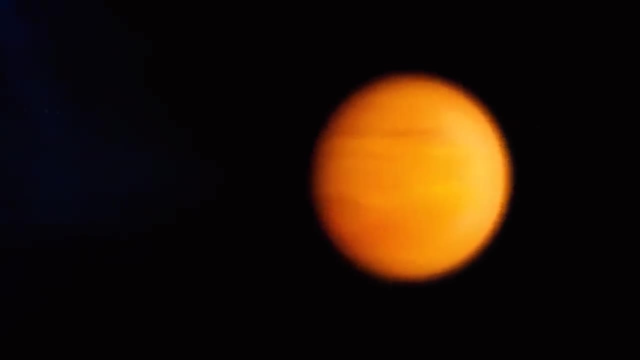 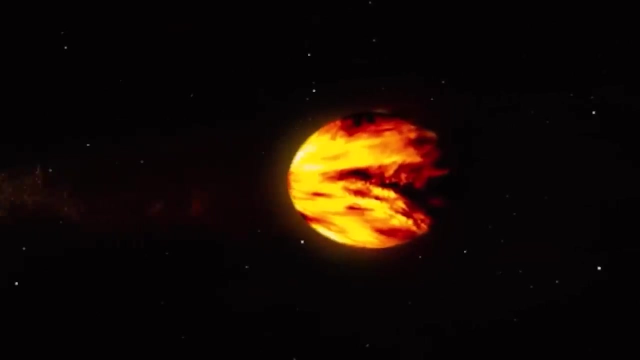 GJ 1214b may be completely devoured by its host star. This eventual consumption underscores the planet's status as doomed and highlights the dynamic and sometimes violent nature of planetary systems. The study of GJ 1214b and its inevitable demise. 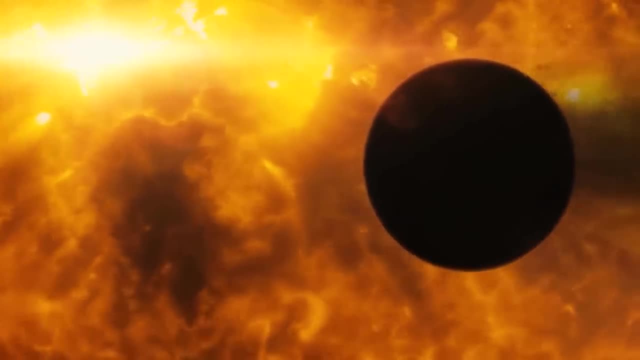 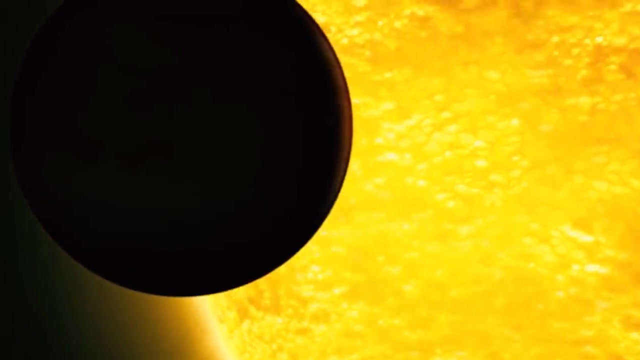 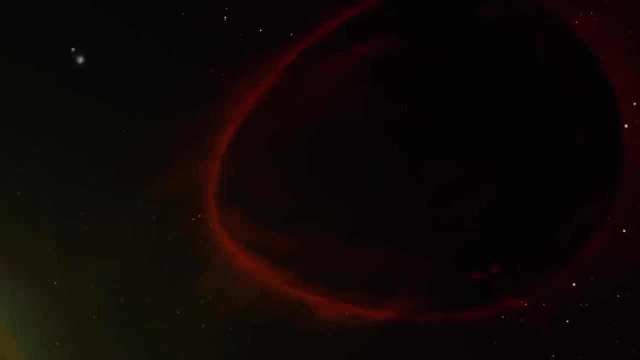 provides valuable insights into the life cycle of planets, especially those in close orbits around their stars, and serves as a reminder of the powerful forces at play within our universe. The observations of GJ 1214b's death spiral into its host star provide a fascinating and somewhat ominous glimpse. 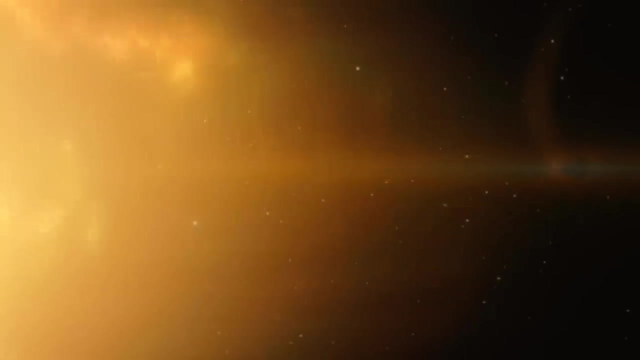 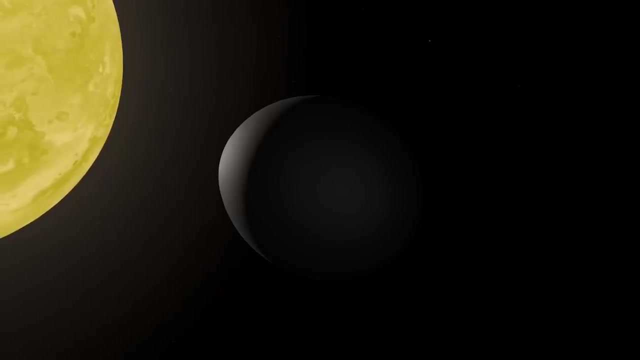 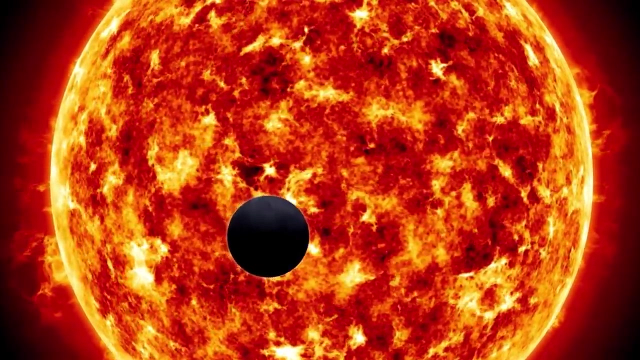 into the dynamics of celestial mechanics at their most extreme. Astronomers, using powerful telescopes and space-based observatories, have gathered critical data on this doomed planet, offering insight into the process by which it is being consumed by its star. The most compelling observations come from the detection. 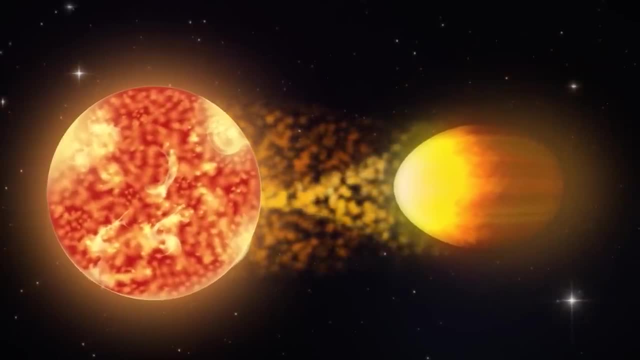 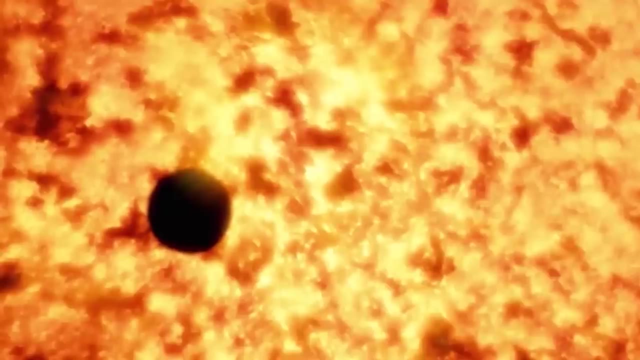 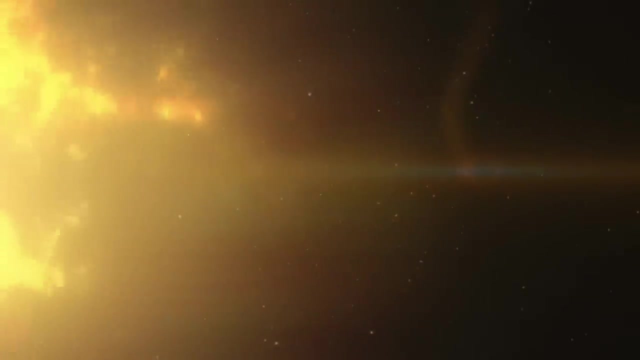 of a vast cloud of material being pulled away from GJ 1214b and toward its star, a direct consequence of the planet's close orbit and the immense gravitational forces at play. This material forms a kind of extended atmosphere or exosphere that stretches from the planet towards the star. 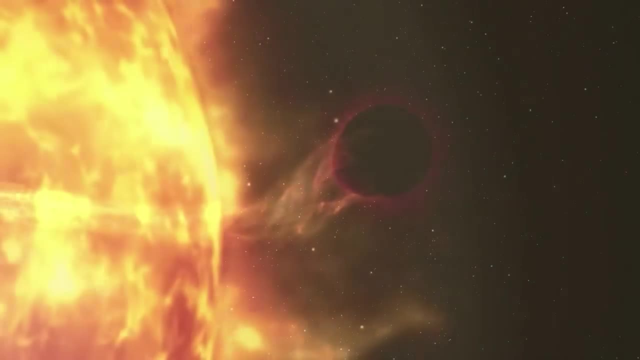 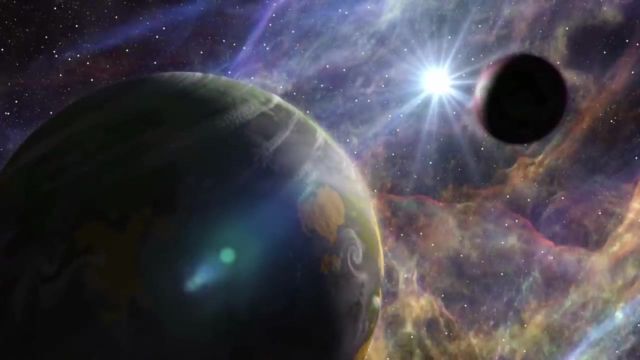 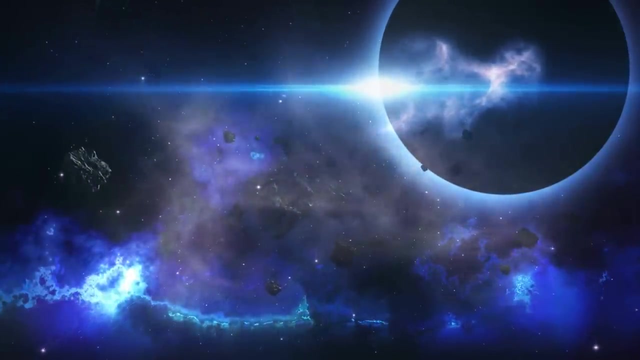 creating a bridge of gas that is slowly being siphoned off. GJ 1214b Spectroscopic analysis, a technique that allows scientists to determine the composition of celestial objects by analyzing the light they emit or absorb, has been instrumental in studying this phenomenon. 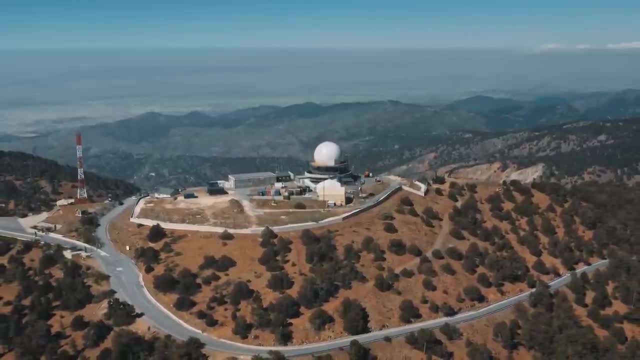 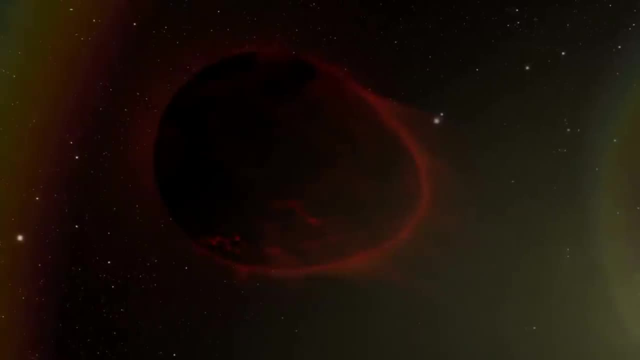 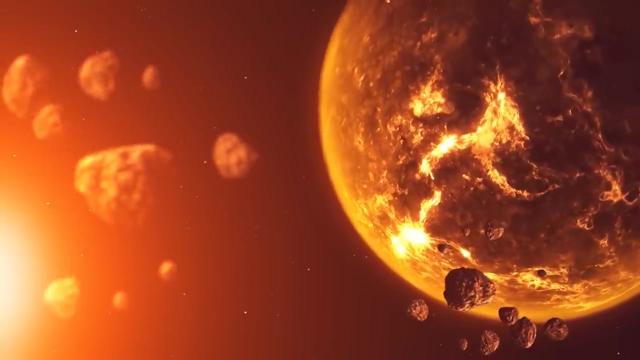 Through spectroscopy. astronomers have identified various gases in this stream, including hydrogen helium and heavier elements, which are being stripped from the planet's atmosphere and added to the star. Further observations have revealed that the rate of mass loss is so significant that the planet's shape has become distorted, elongated. 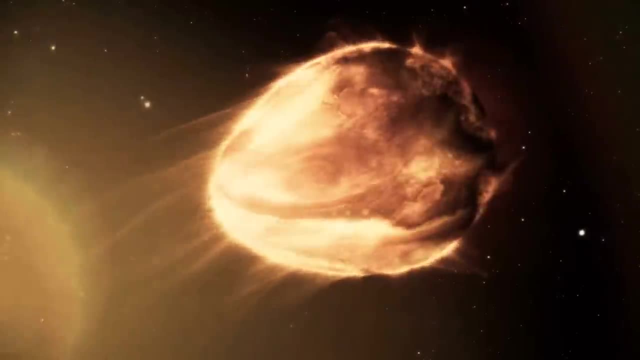 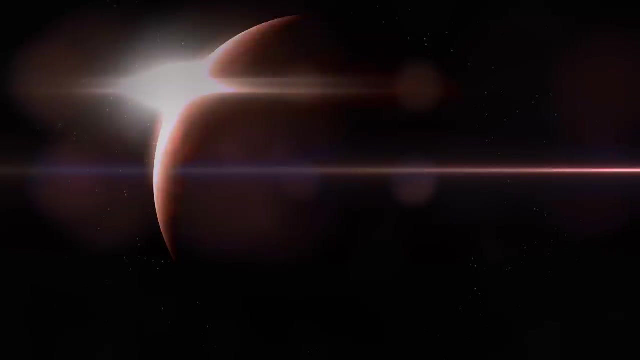 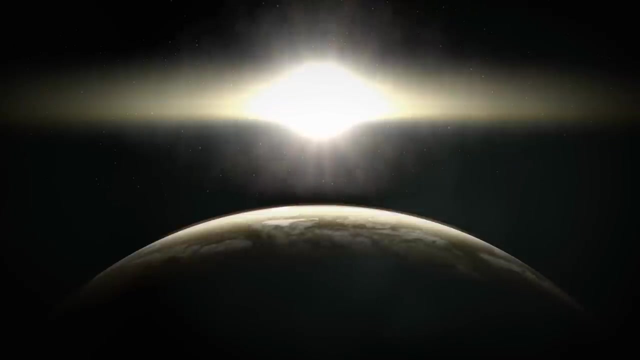 by the tidal forces exerted by the star. This distortion not only affects the planet's gravitational equilibrium, but also accelerates the process of atmospheric escape, hastening GJ 1214b's demise As the planet loses mass to its star. 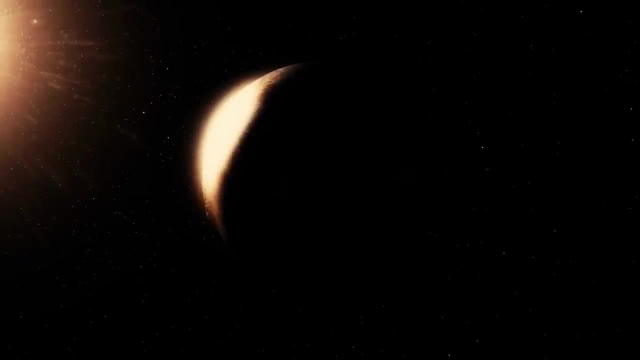 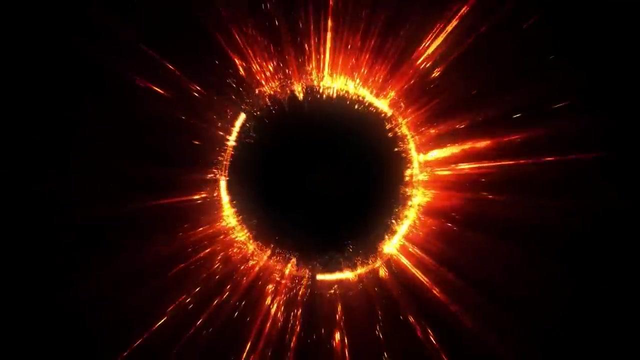 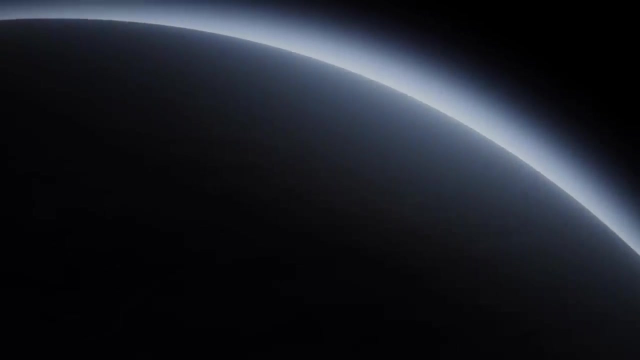 the atmosphere undergoes significant changes, with vast quantities of gas being stripped away. This loss includes not only hydrogen and helium, the most common elements in gas giants, but also heavier elements and compounds that contribute to the planet's atmospheric composition. The stripping of WASP-12b's atmosphere. 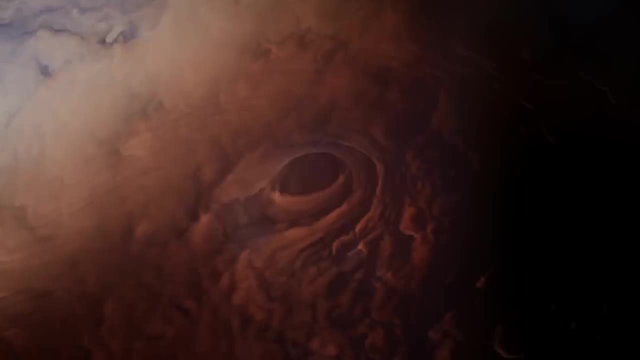 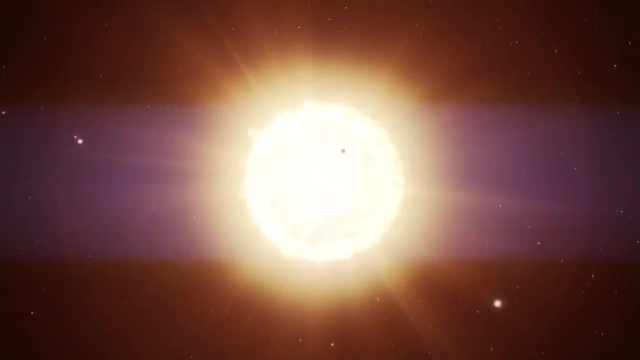 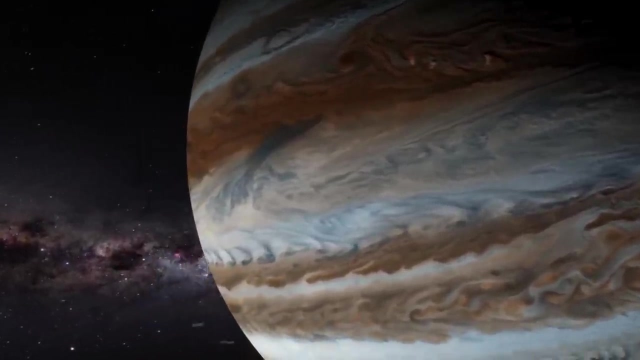 leads to a decrease in atmospheric pressure, altering the balance between the planet's surface and the vacuum of space. In addition, the intense heat from the nearby star causes the remaining atmosphere to expand and escape more readily, further accelerating the atmospheric loss. This process can cause the atmosphere to become thinner. 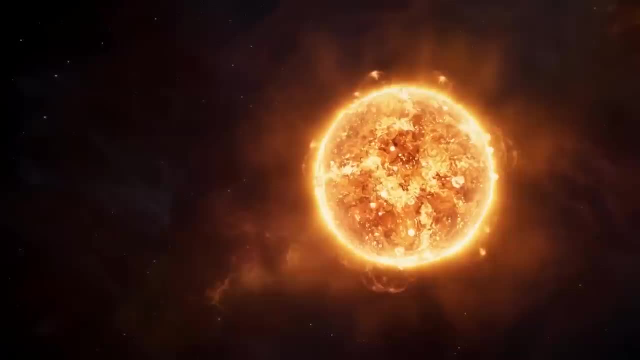 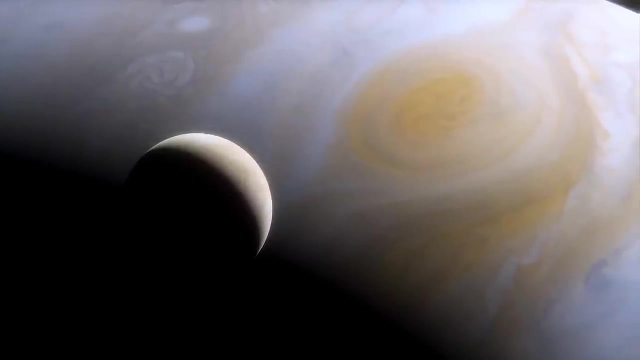 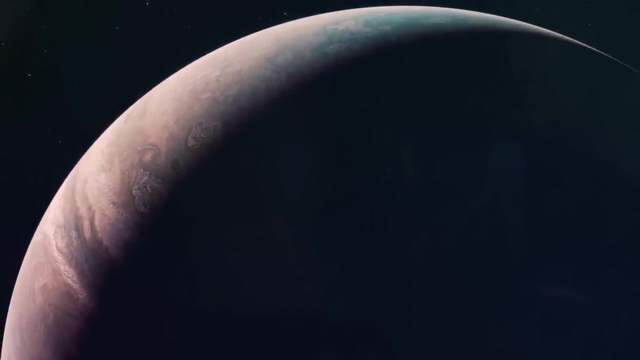 and less capable of protecting the planet's surface from harmful stellar radiation, leading to increased surface temperatures and potentially altering the chemical makeup of the surface itself. The tidal forces exerted by the star on WASP-12b not only elongate the planet. 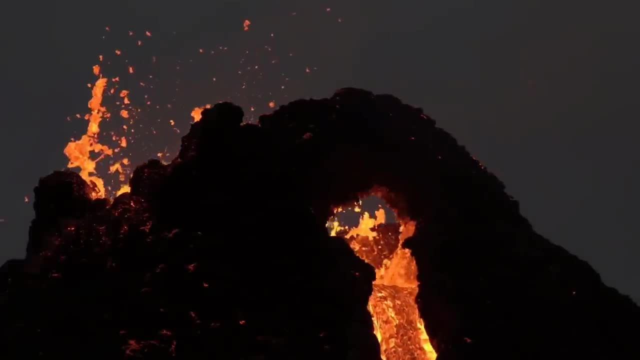 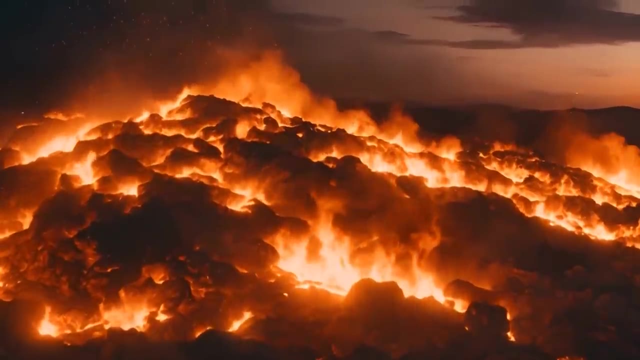 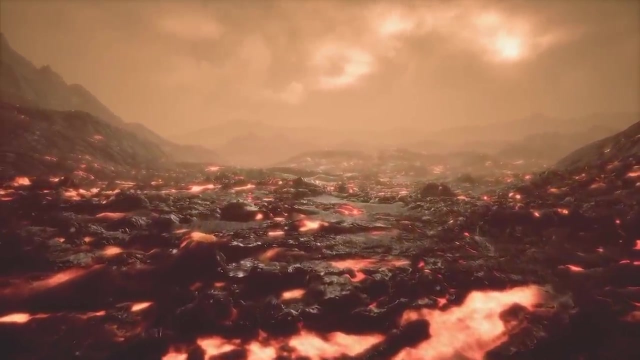 but can also induce volcanic activity or other geological processes on the surface by heating the planet's interior. This geothermal heating could reshape the planet's surface over time, creating new surface features or eroding existing ones. The study of WASP-12b's death spiral. 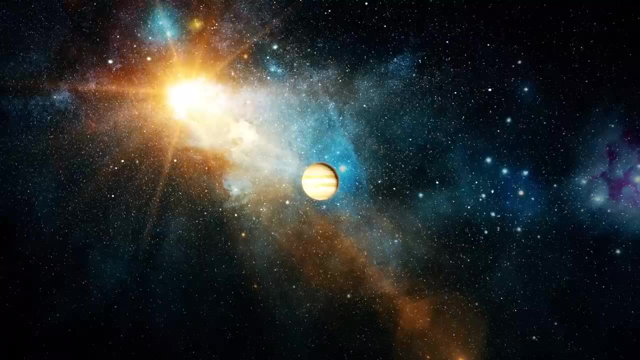 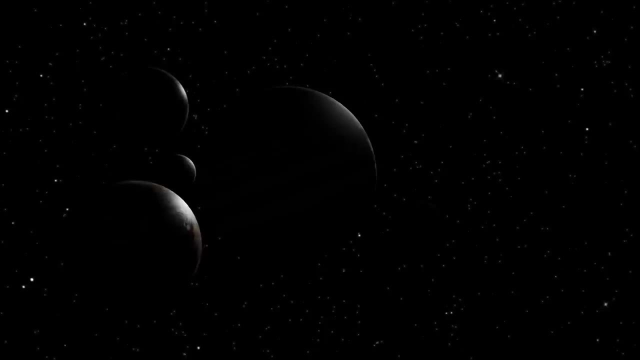 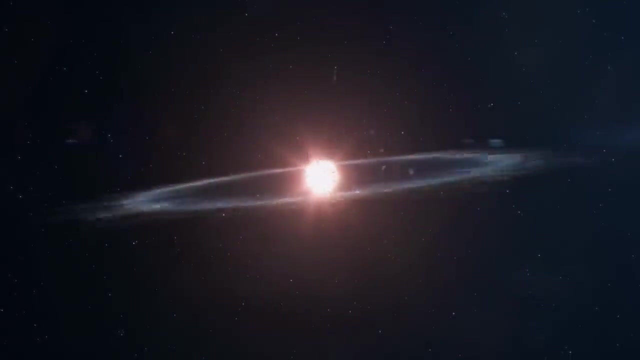 offers not only a window into the fate that awaits the planet, but also broader implications for our understanding of planetary evolution and star-planet interactions. These observations have challenged previous notions about the stability of planetary orbits and the factors that can lead to a planet's destruction. 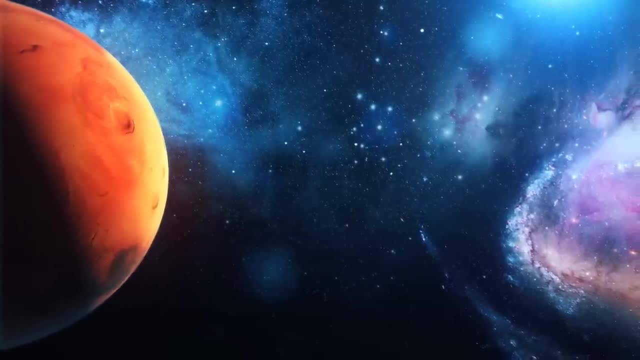 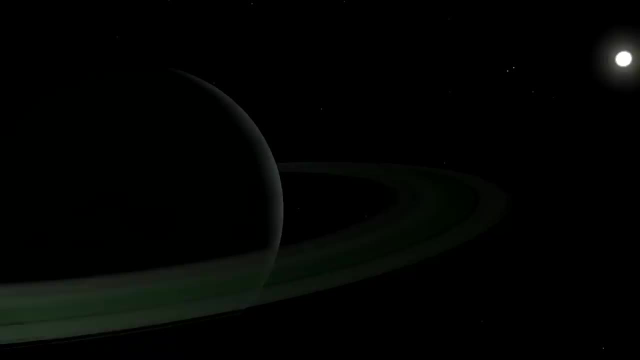 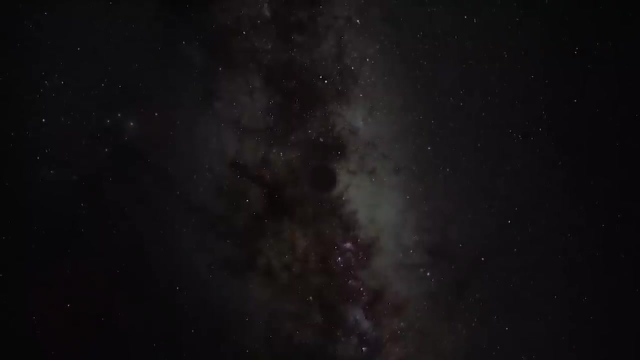 Moving from the captivating yet dire circumstances of WASP-12b, we delve into the enigmatic case of HD 106906b, a planet whose peculiar and disrupted orbit offers a stark contrast to more conventional planetary systems. HD 106906b is an exoplanet that lies about 300 light-years away from Earth. and presents a curious case for astronomers. due to its highly elliptical and distant orbit around its host star. This exoplanet is situated at a staggering distance of more than 650 times the Earth's distance from the Sun, placing it in a part of its solar system. 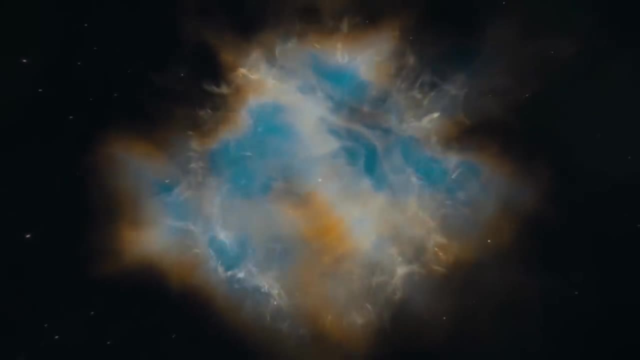 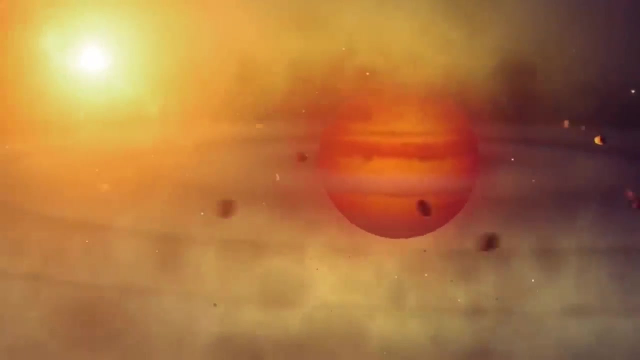 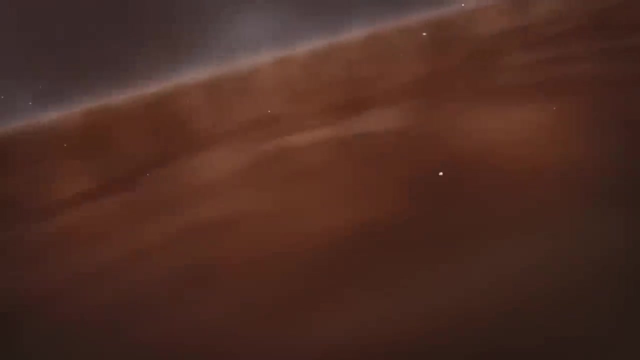 where traditional models of planet formation and orbital dynamics struggle to provide clear explanations. The disrupted orbit of HD 106906b raises intriguing questions about the processes that could lead to such an unusual arrangement. One prevailing theory suggests that its current orbit is the result of gravitational interactions with other planets. 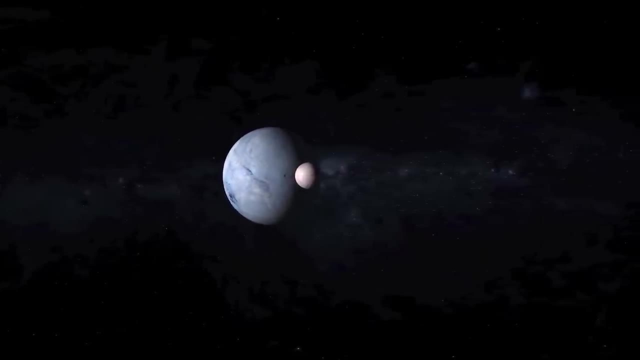 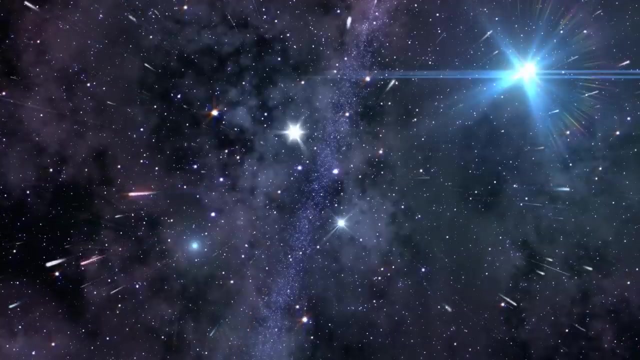 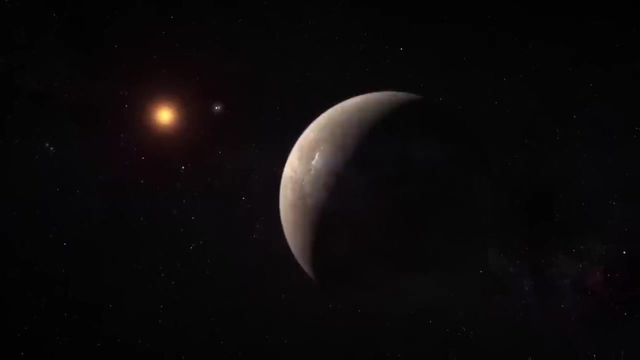 within the system or even a passing star which could have dramatically altered its trajectory. Such an encounter would need to be both powerful and precise, nudging HD 106906b into its current path without ejecting it from the system entirely or causing it to crash into its host star. 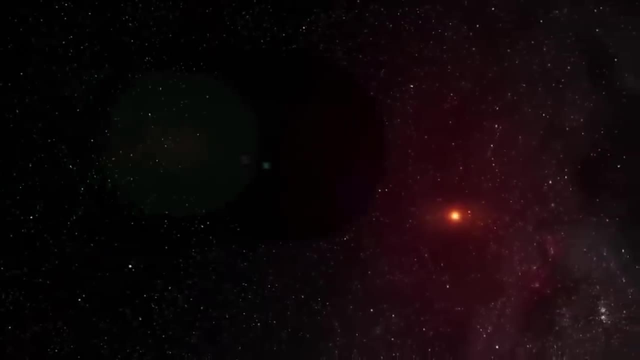 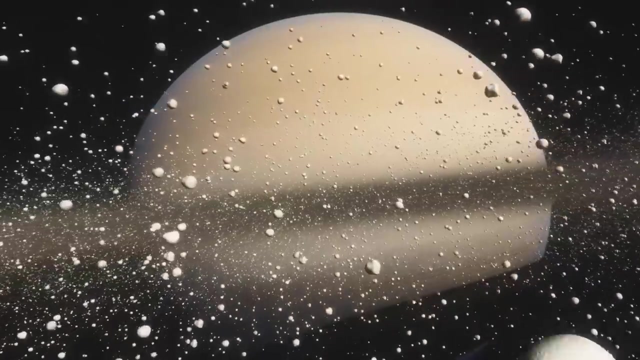 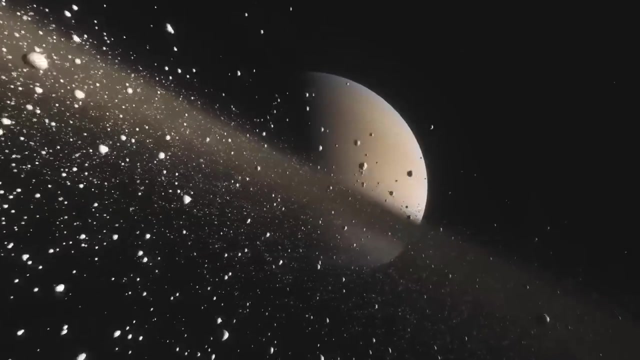 Another aspect of HD 106906b's orbit that fascinates scientists is its inclination. Observations indicate that the planet's orbit is tilted significantly in relation to the plane of its solar system, further complicating the mystery of its origin and evolution. 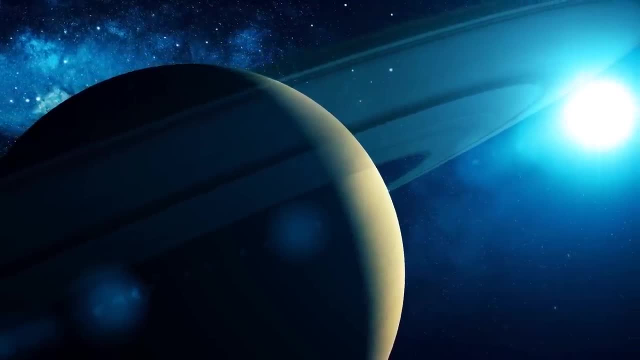 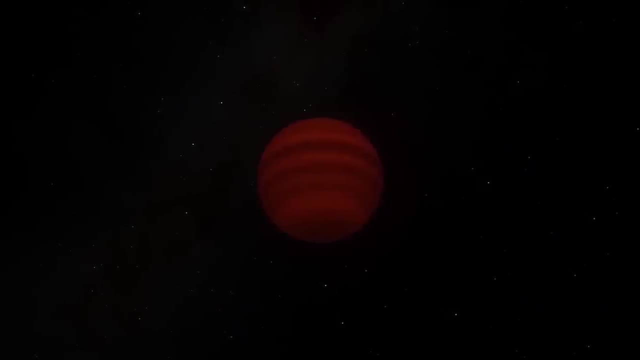 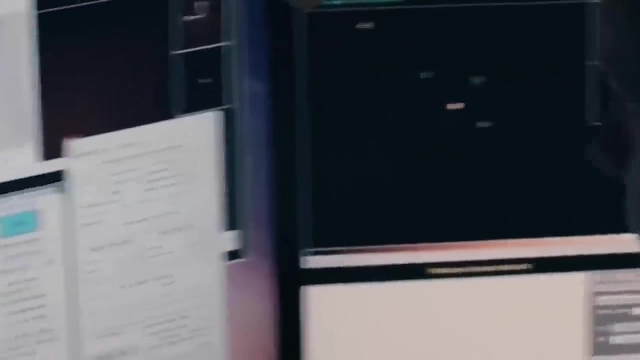 This inclination could be evidence of a dynamic and possibly turbulent past within its solar system, involving interactions that are not yet fully understood. The unusual orbit of HD 106906b not only captivates the curiosity of astronomers, but also poses a significant challenge. 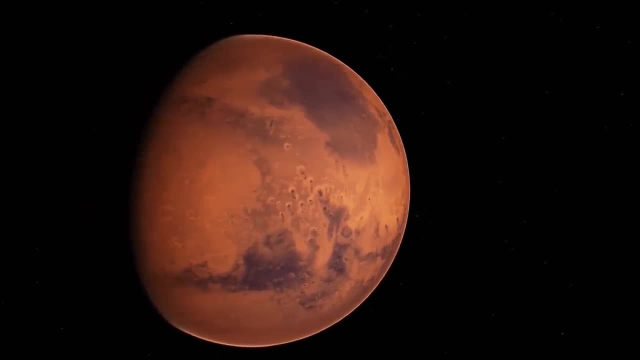 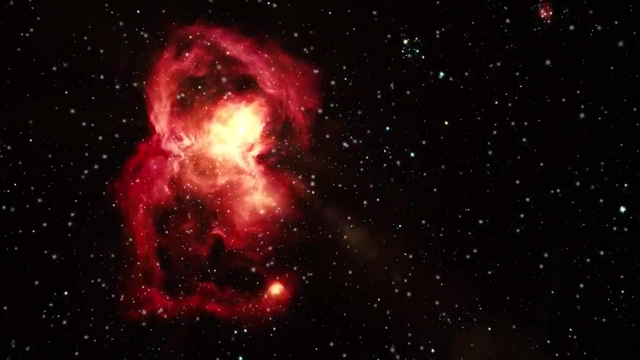 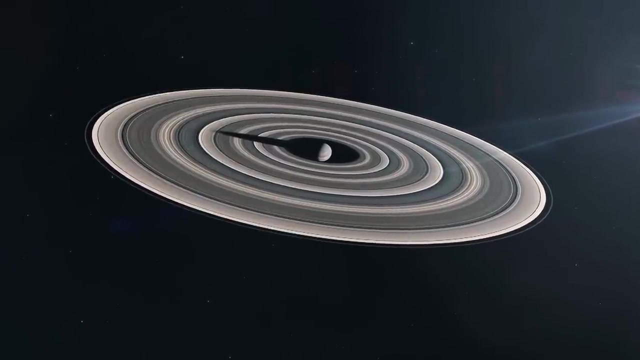 to our existing theories of planetary system formation. Traditionally, models of planetary formation have centered around the concept of a protoplanetary disk, a rotating circumstellar disk of dense gas and dust surrounding a newly formed star where planets form through the accretion of disk material. 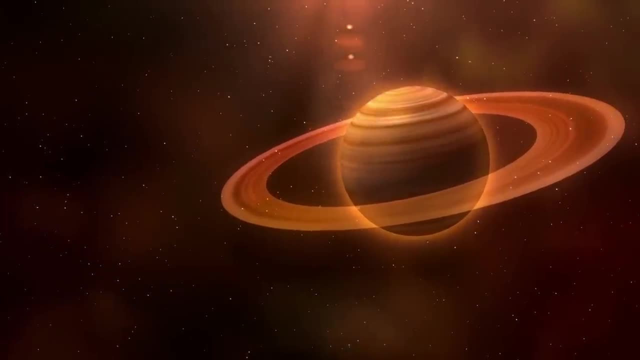 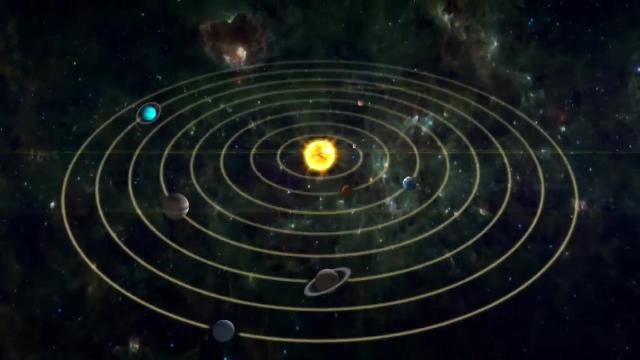 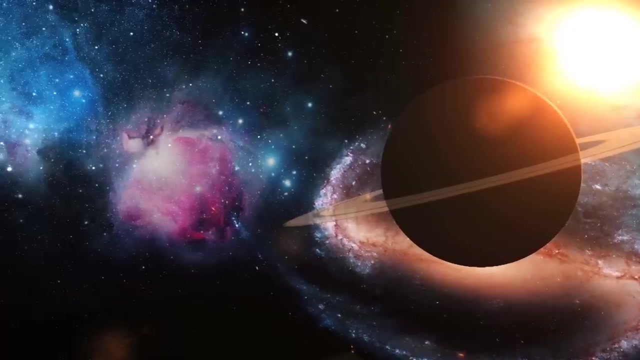 These models predict that planets should form within the disk and maintain orbits relatively close to the plane in which the disk lies, similar to the configuration of our solar system. However, the extraordinary orbit of HD 106906b, with its significant distance from its host star. 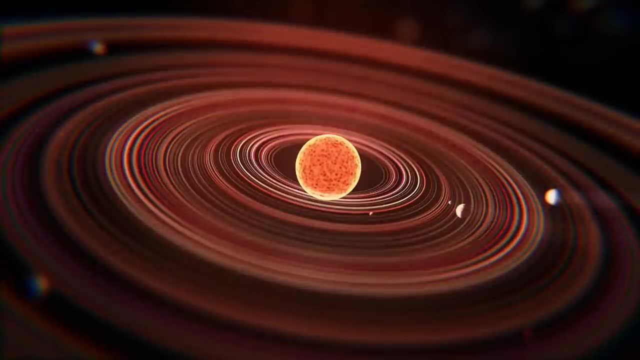 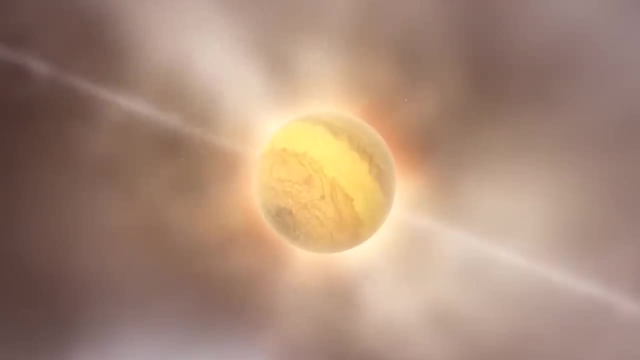 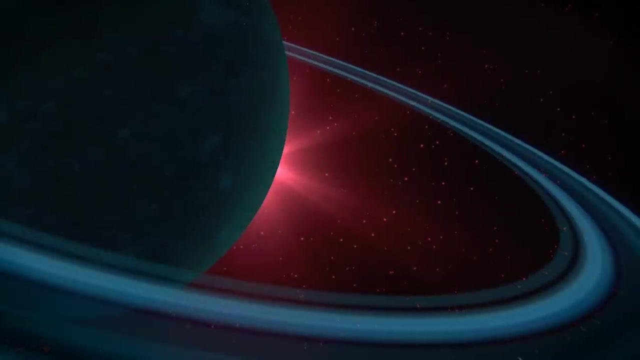 and its inclined orbital path suggests that other processes may be at play in the formation and evolution of planetary systems. One of the key challenges presented by HD 106906b's orbit is understanding how a planet can end up in such a wide and inclined orbit. 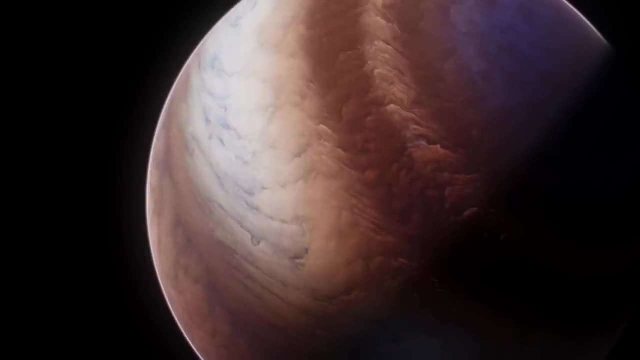 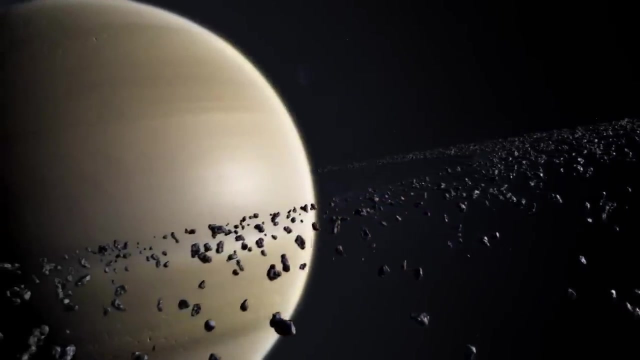 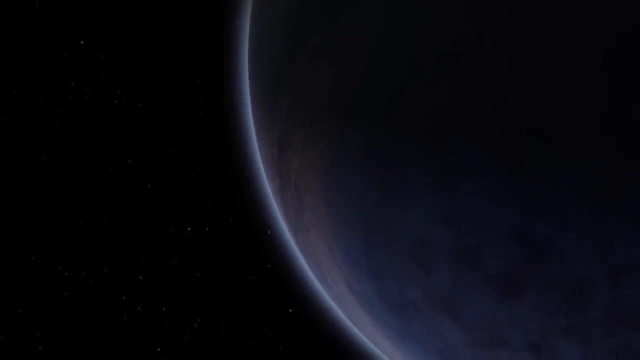 when traditional formation mechanisms would not predict such outcomes. This discrepancy suggests that interactions beyond simple accretion and disk dynamics are involved. Theories have been proposed that include gravitational disturbances from other massive bodies within the planetary system, such as other giant planets, or even close encounters with passing stars. 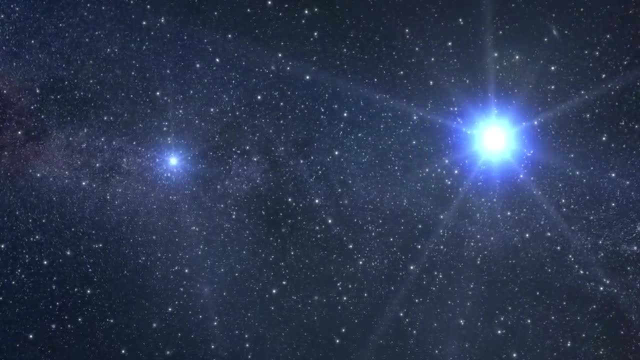 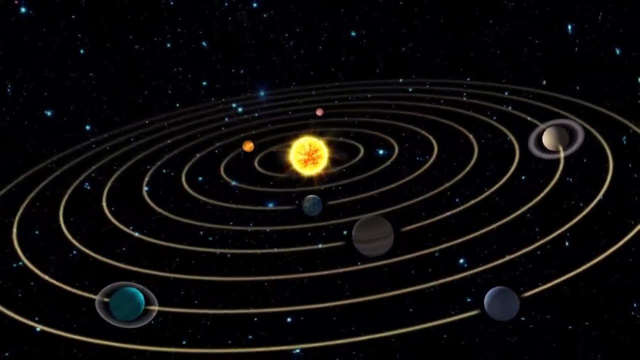 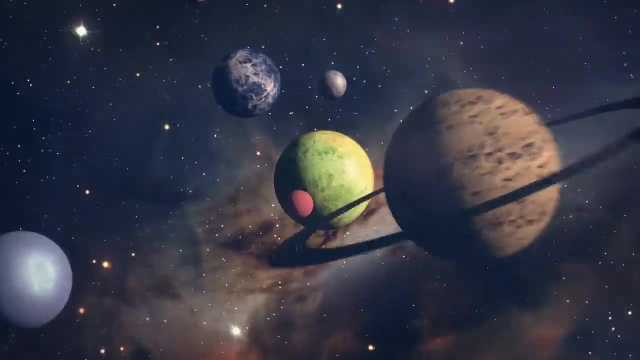 that could dramatically alter a planet's trajectory. These scenarios imply a more chaotic and dynamic early solar system environment than previously assumed. Furthermore, the existence of HD 106906b challenges the notion of how stable planetary orbits are achieved and maintained. The planet's current orbit suggests that it may have been. 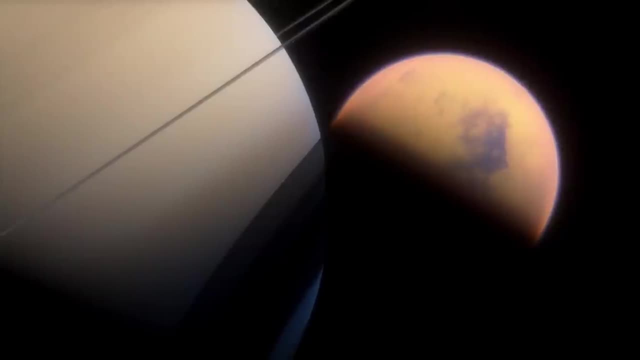 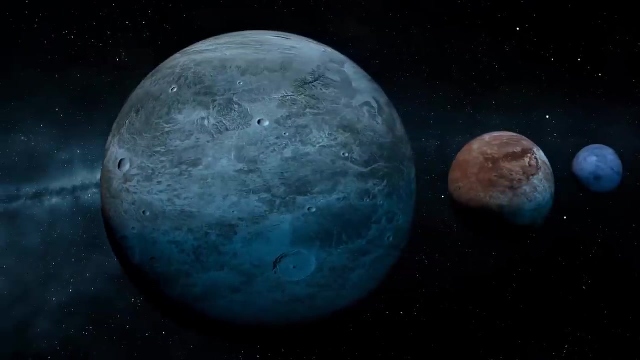 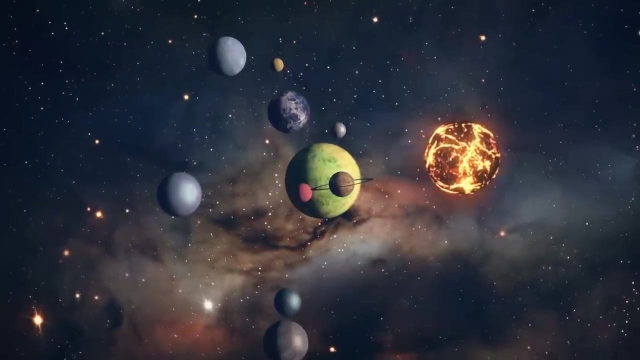 through a complex migratory history, potentially involving mechanisms like planet-planet scattering or capture from another system. such processes could lead to the wide variety of exoplanetary systems observed by astronomers, far beyond the relatively orderly configuration seen in our solar system. Building on the exploration of the challenges, 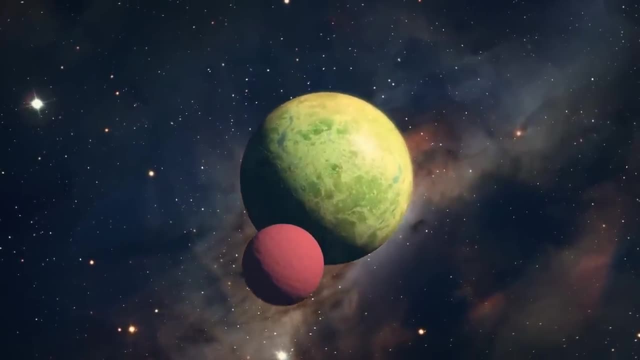 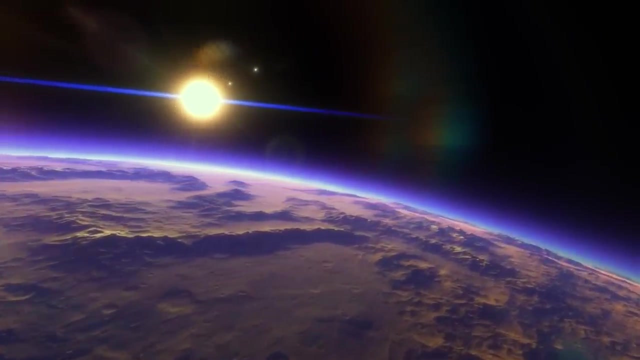 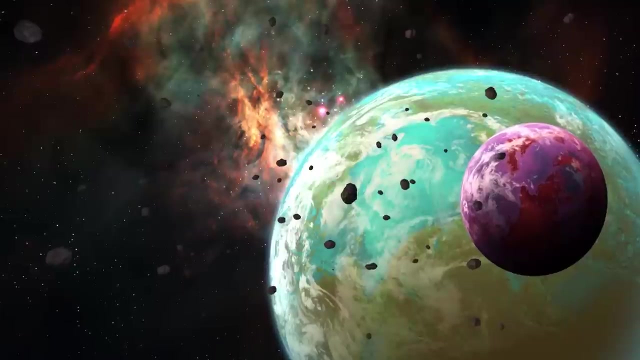 HD 106906b's unusual orbit presents to traditional theories of planetary system formation the possibility of a planetary orbit in the form of a single orbit or a planetary orbit in the form of a single orbit In this series of planetary system formation. let's delve into the speculative yet intriguing possibilities. 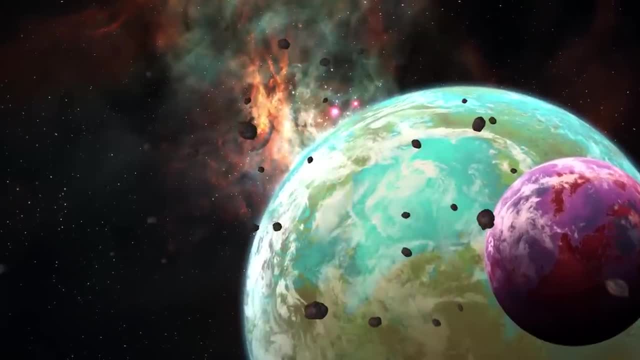 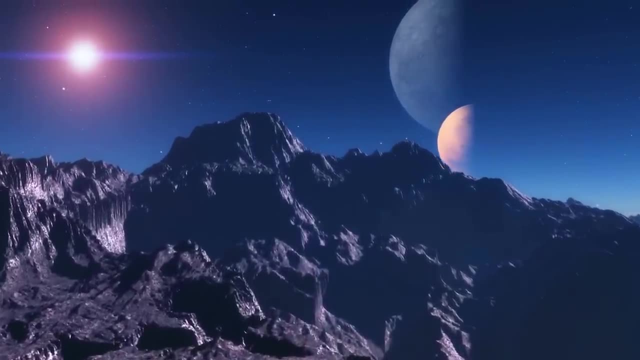 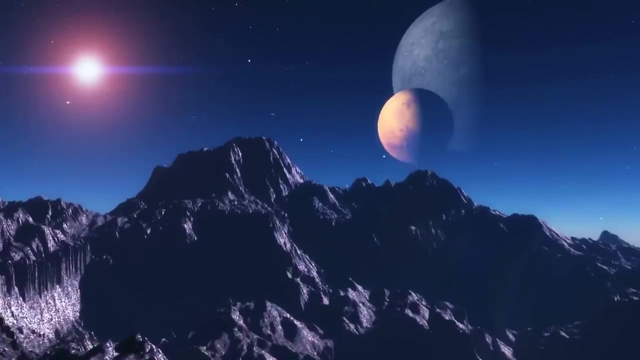 of what might have caused this exoplanet's extraordinary orbital characteristics. The orbit of HD 106906b, markedly different from the more familiar patterns observed within our own solar system, suggests an origin story filled with celestial dynamics that push the boundaries of our understanding. 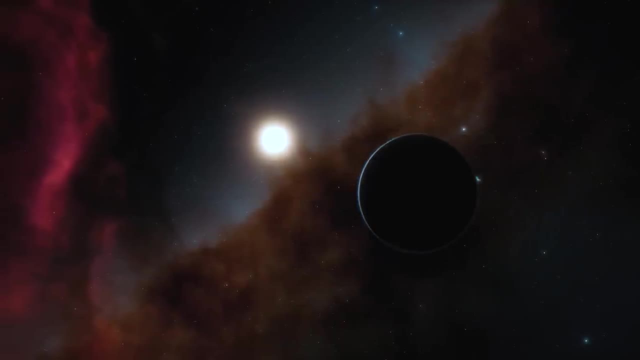 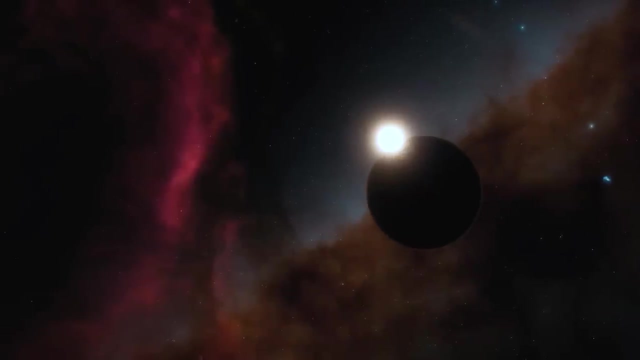 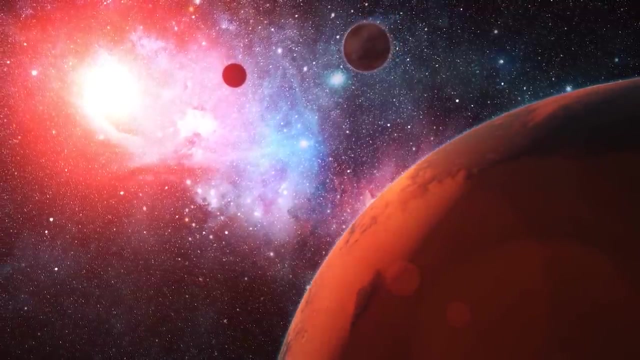 One compelling theory posits that HD 106906b is the result of gravitational interactions with another unseen companion in the system, possibly another planet or a brown dwarf. These interactions could have dramatically altered HD 106906b's trajectory early in the system's history. 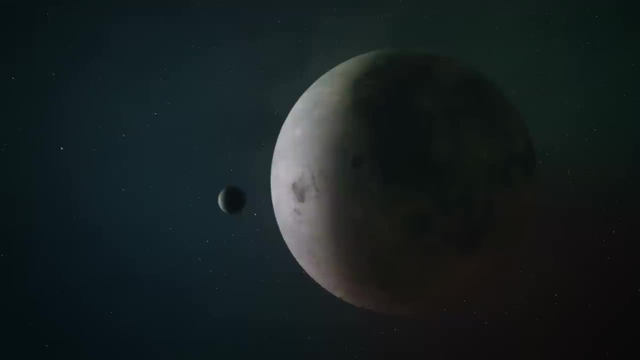 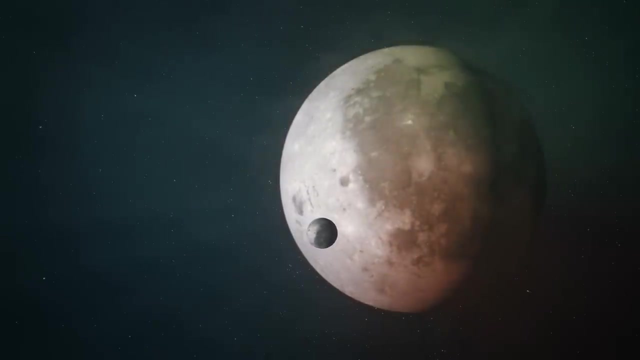 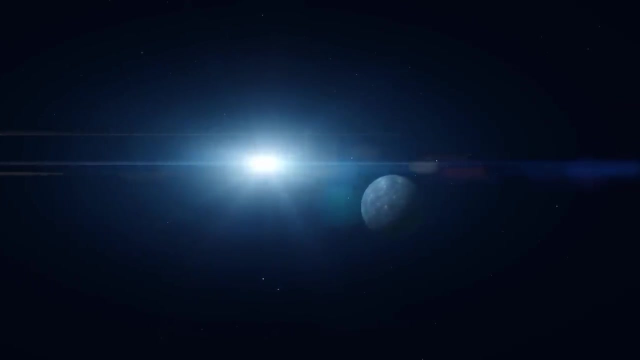 ejecting it into a distant and inclined orbit. This scenario would require a delicate balance of forces, ensuring that HD 106906b was not completely flung out of the system, but instead settled into its current wide orbit. Another hypothesis suggests that a close encounter with a passing star 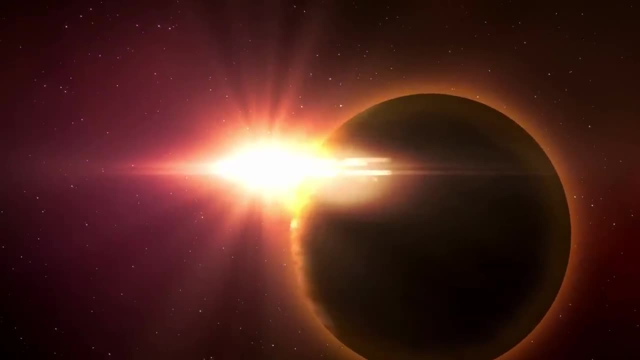 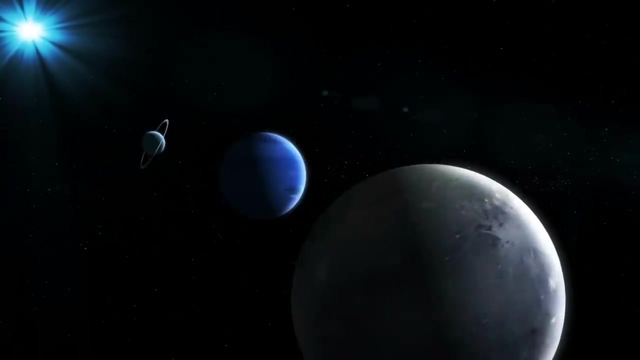 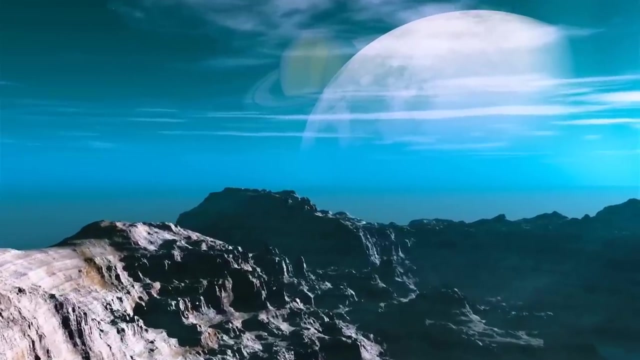 might have disrupted the young planetary system, influencing HD 106906b's path. Such an event could have occurred in the dense environment of a star cluster where close stellar encounters are more common. The gravitational tug from a nearby star could have significantly altered the velocity and direction. 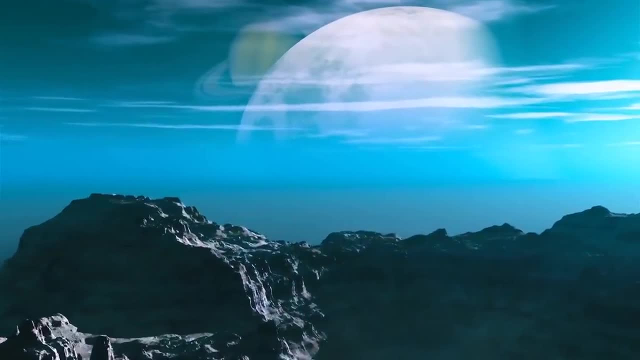 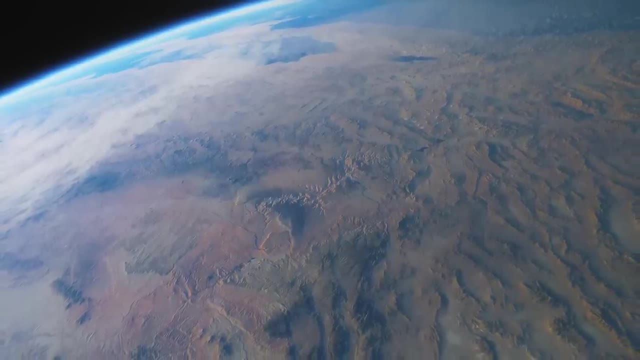 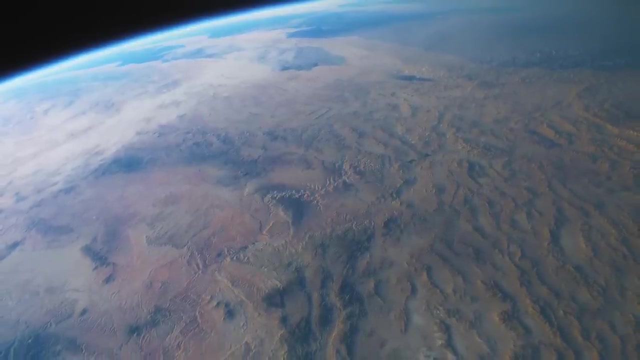 of HD 106906b, placing it on its unusual course. Additionally, the early dynamical evolution of the HD 106906 system itself may hold clues to the planet's odd orbit, The process of planet-planet scattering, where young planets in forming systems interact. 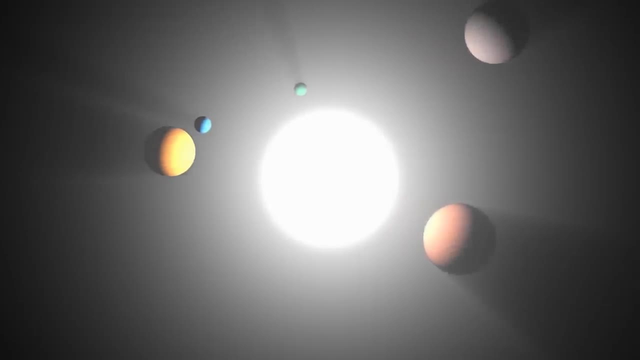 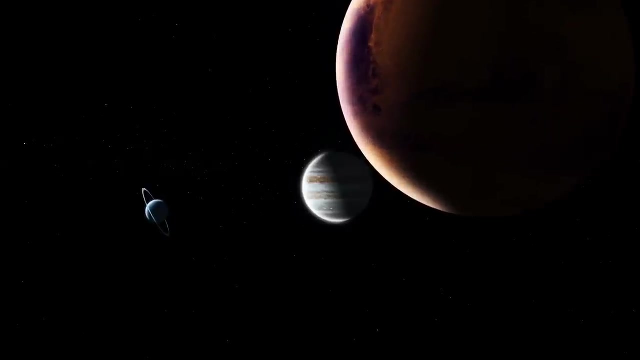 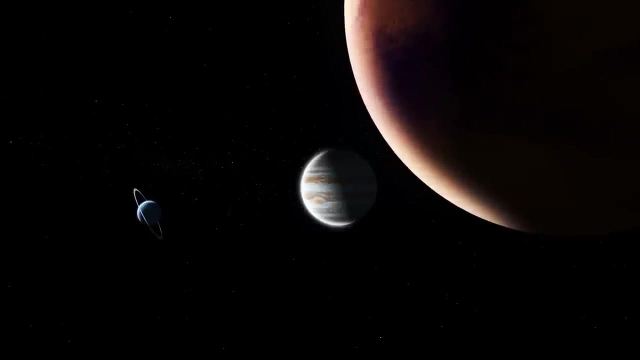 and gravitationally sling each other into different orbits could explain HD 106906b's current position. This mechanism often results in one or more planets being moved to wider, more eccentric orbits and could potentially result in the highly inclined orbit observed for HD 106906b. 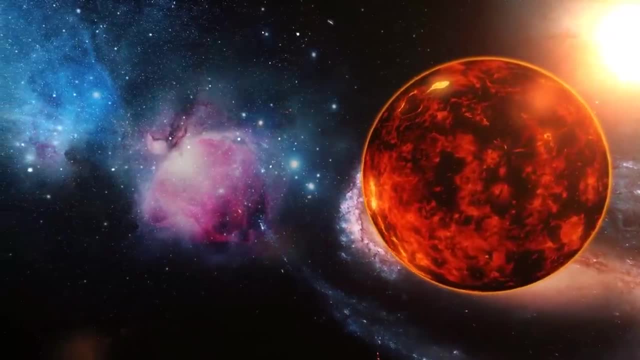 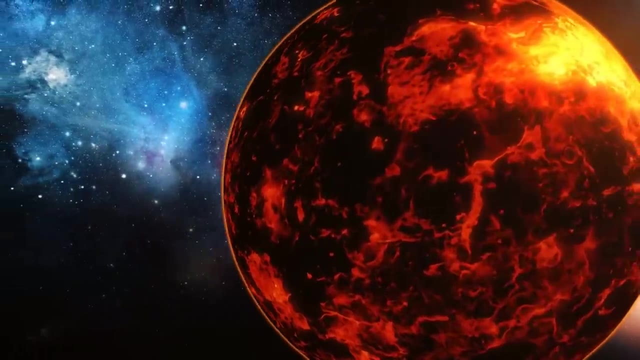 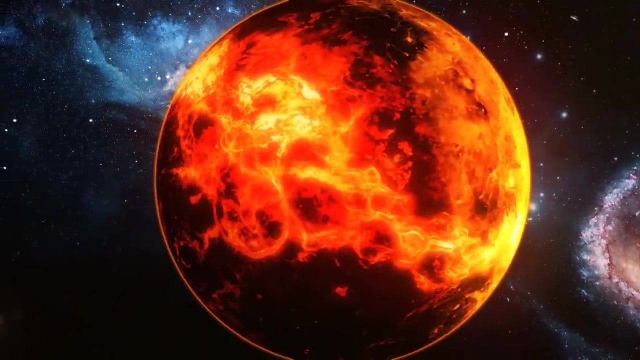 On the intriguing exoplanet Koro 7b, located a distant 489 light-years away from Earth in the constellation of Monoceros. a phenomenon as fascinating as rock showers occurs due to its extreme environmental conditions. This planet presents an extraordinary case. 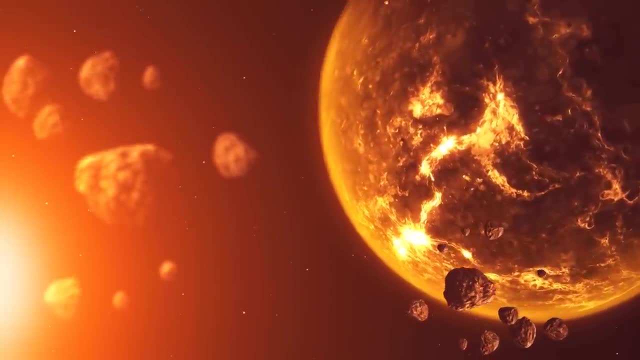 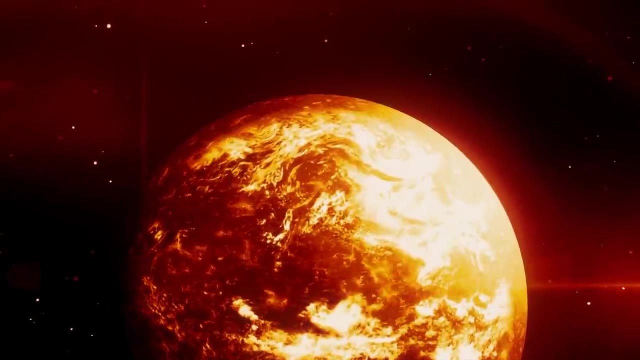 in the study of exoplanetary weather patterns, primarily because of its proximity to its host star. Koro 7b orbits its star at a distance 23 times closer than Mercury's orbit around the Sun, leading to surface temperatures on its dayside. 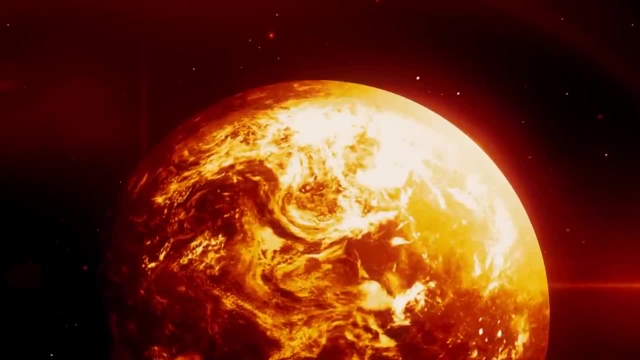 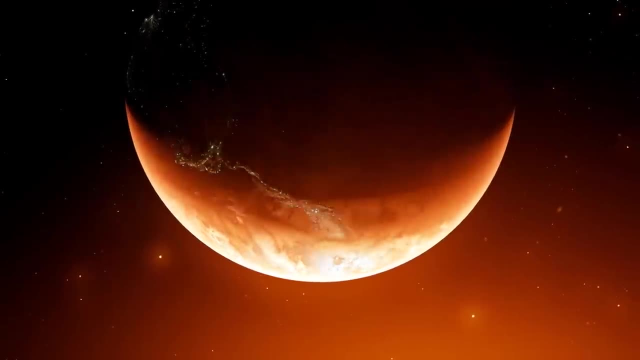 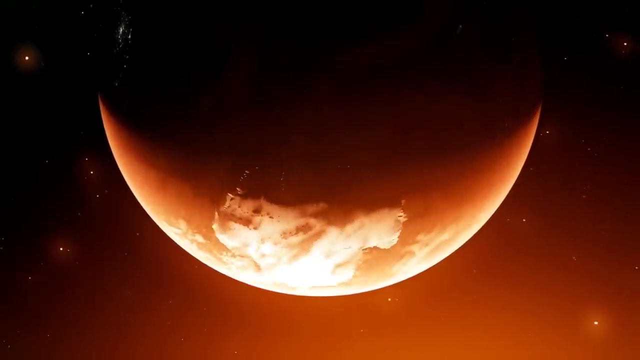 reaching up to 2,500 degrees Celsius. At such high temperatures, the rock on the surface of Koro 7b doesn't just melt, it vaporizes. This creates an environment where minerals and rocks turn into gas, a scenario vastly different from anything we experience on Earth. 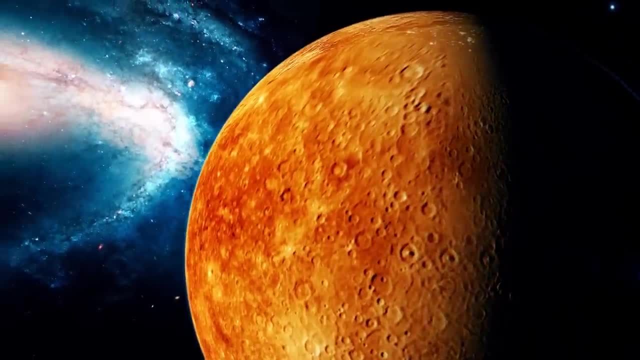 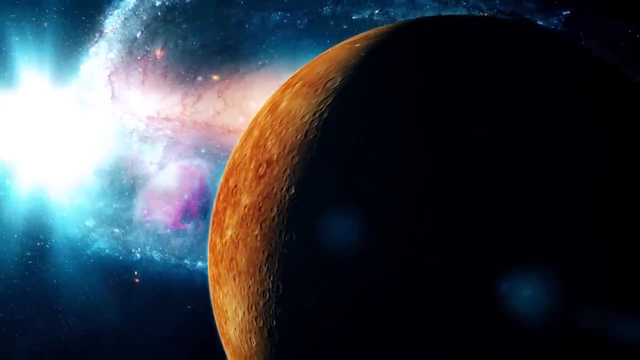 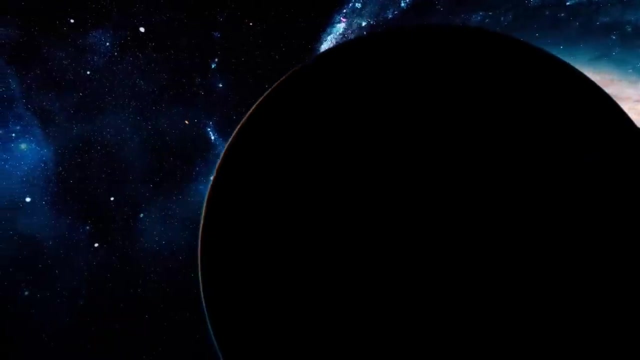 the intense heat on the planet's dayside causes the rock to vaporize, and this rock vapor is then carried by the planet's atmosphere to the cooler night side. On the night side, temperatures drop significantly, allowing the vaporized rock to condense. 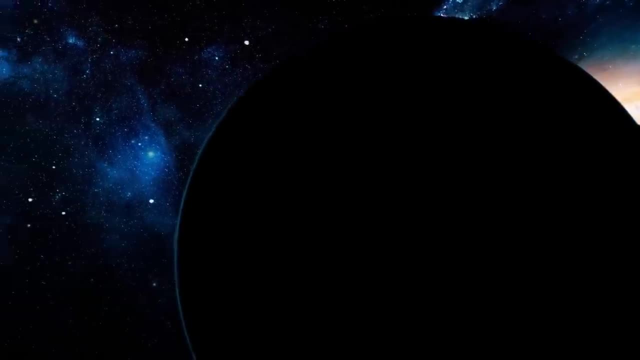 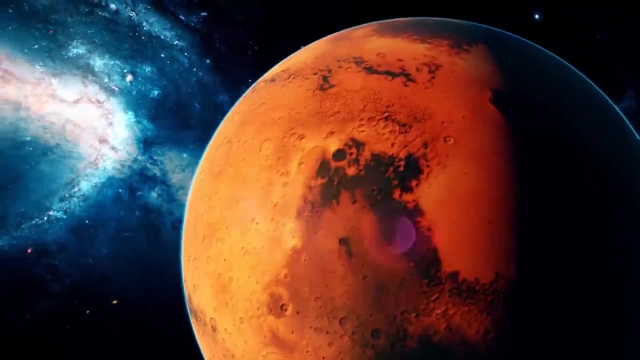 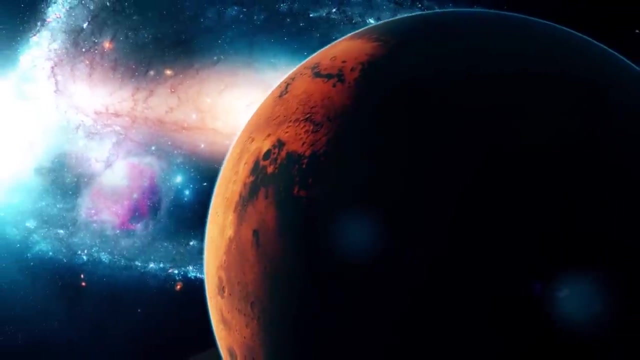 and form particles that eventually fall as precipitation, not unlike rain on Earth, but instead of water, these are literally showers of rocks. This cycle of vaporization and precipitation is a constant feature of Koro 7b's atmosphere, driven by the extreme temperature difference. 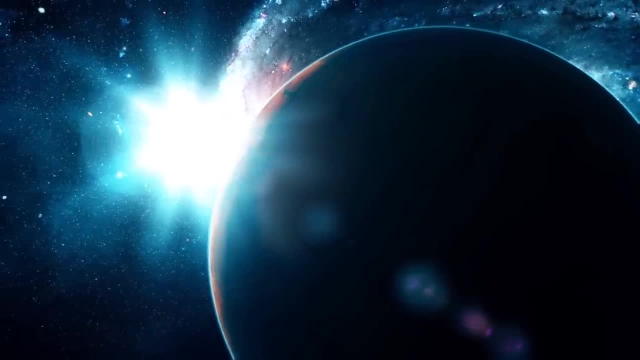 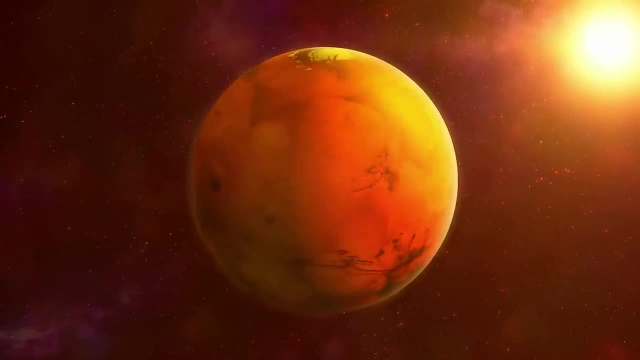 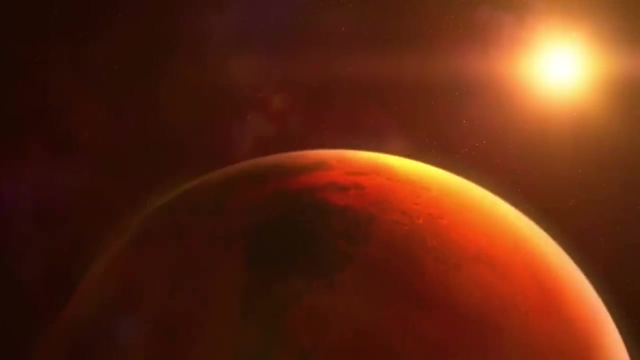 between the planet's dayside and night side. Furthermore, the gravitational forces at play between Koro 7b and its star contribute to the planet's distorted shape, which affects how the atmosphere circulates these rock vapors. The tidal forces are so strong. 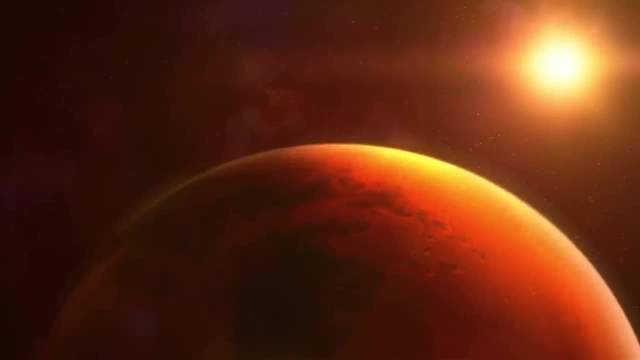 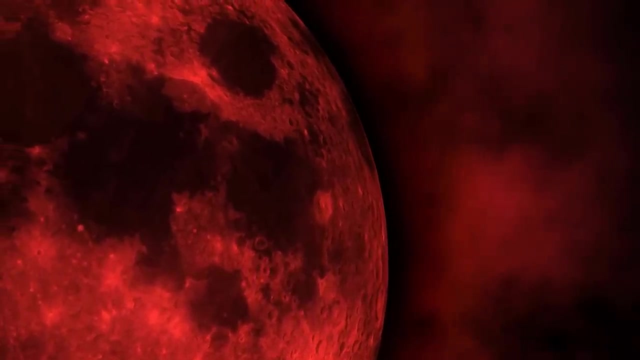 that they not only influence the planet's shape but also its internal heating, adding another layer of complexity to the weather patterns observed The unique atmospheric phenomena on Koro 7b, where temperatures can soar to 2,500 degrees Celsius on the dayside. 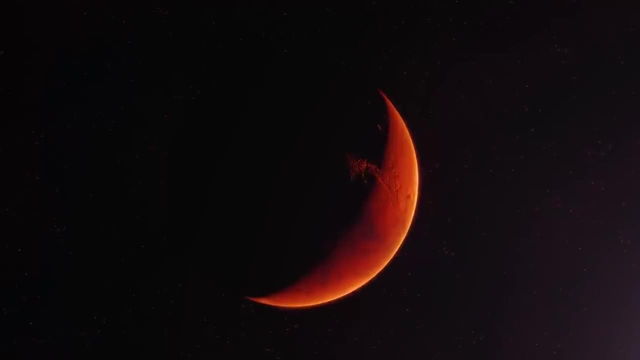 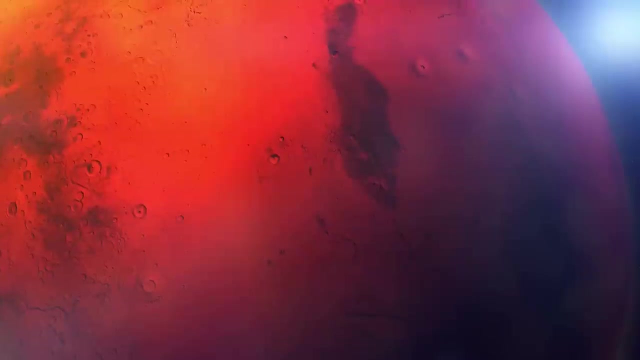 turning rocks into vapor and then see these vapors cool and condense into rock rain on the cooler night side, offer a live laboratory for studying processes that are simply not possible to observe on Earth or within our solar system. This intense cycle of vaporization and precipitation on Koro 7b. 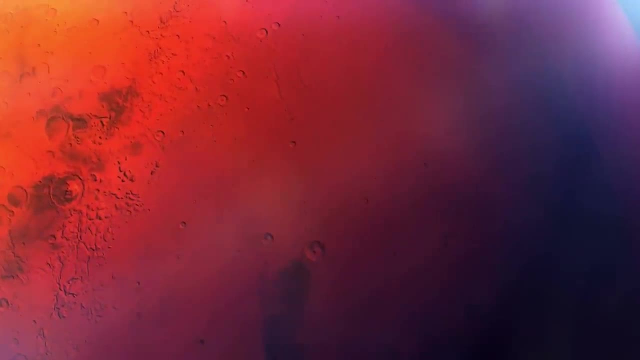 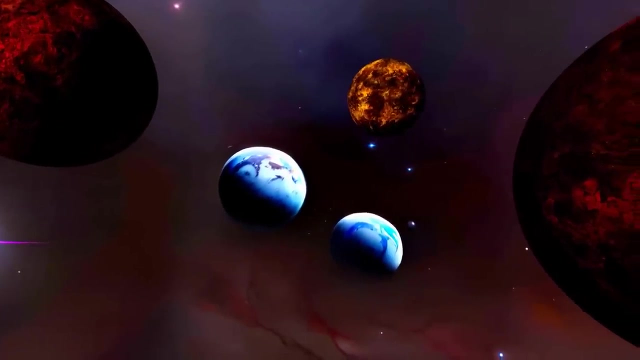 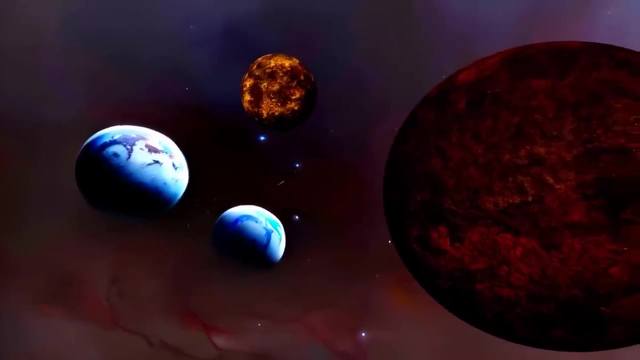 provides invaluable insights into the behavior of minerals and rocks under conditions that are extreme by Earth standards. For instance, understanding how different materials vaporize and condense can help scientists refine models of planetary formation and evolution, not just for exoplanets, but also for the early Earth. 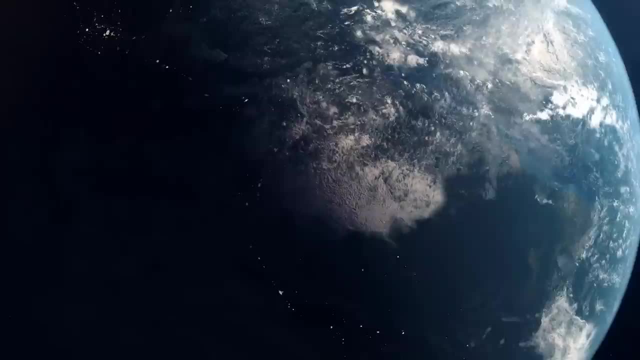 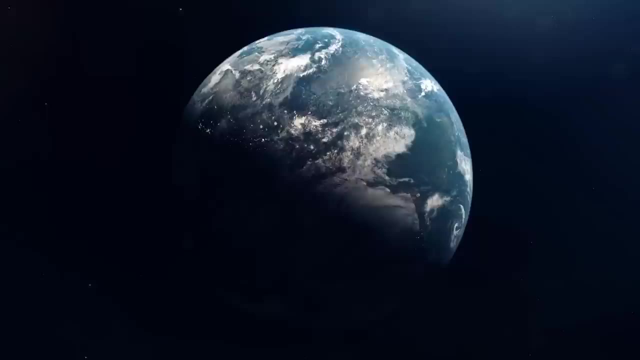 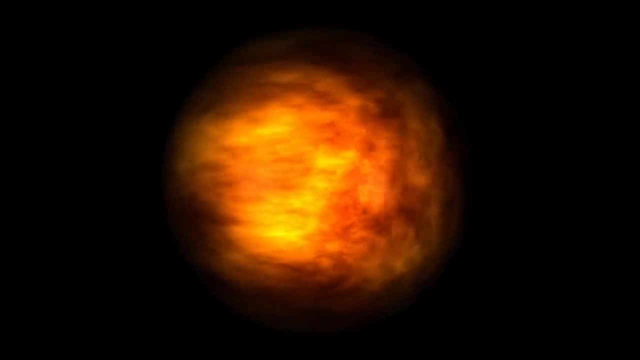 and other bodies within our own solar system. This could shed light on the mysteries of our planet's geological history, including the formation of its atmosphere and the development of its crust. Additionally, studying the atmospheric dynamics on Koro 7b allows researchers to explore the effects of extreme temperature gradients. 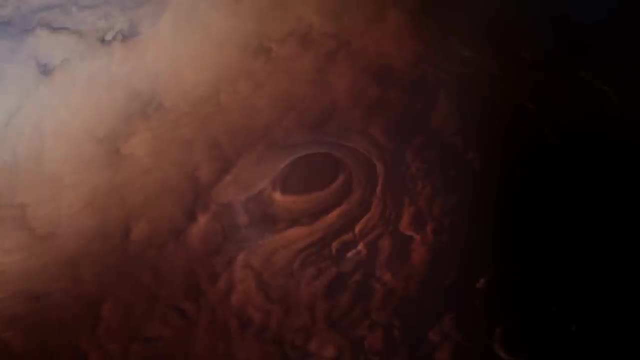 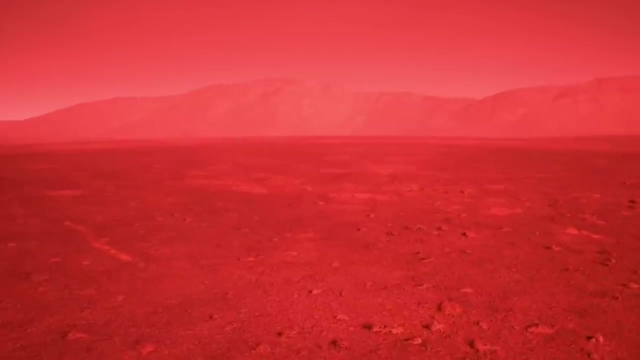 on atmospheric circulation. These insights could improve our understanding of atmospheric science, including weather patterns and climate across a range of planetary environments, from the hottest exoplanets to more Earth-like worlds. The extreme conditions on Koro 7b challenge our existing theories. 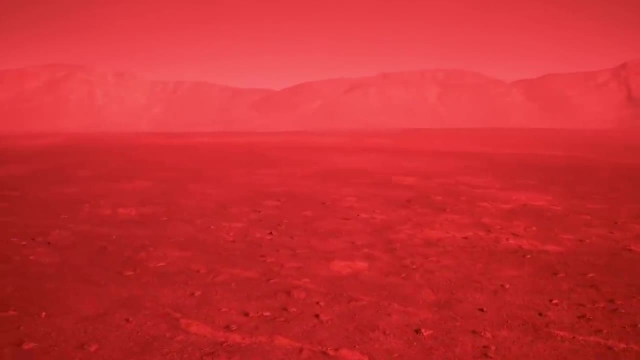 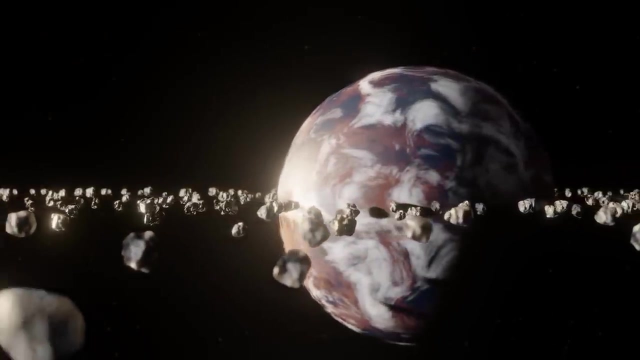 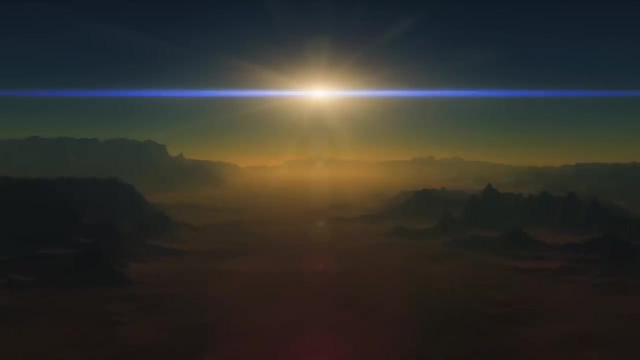 about the habitability of planets and the conditions necessary for life. By expanding our knowledge of how planets can form and evolve under a wide variety of conditions, we can better assess the potential for life elsewhere in the universe. This knowledge also aids in the search for exoplanets. 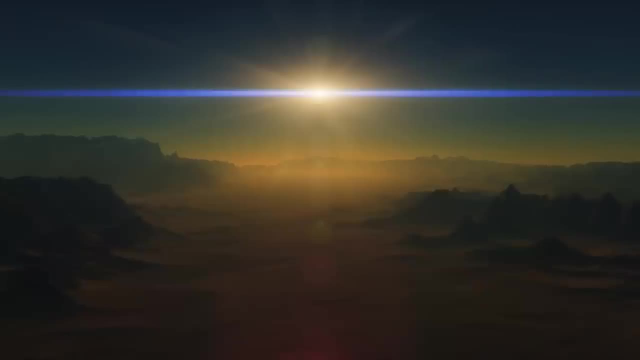 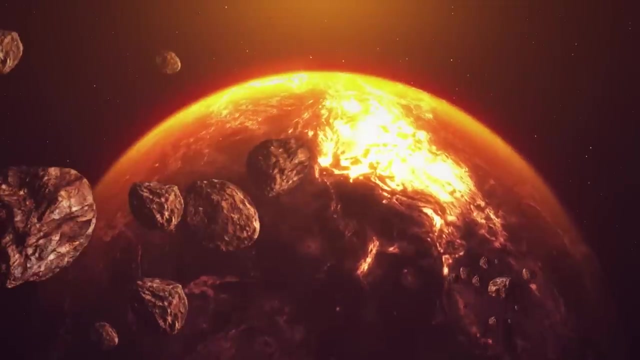 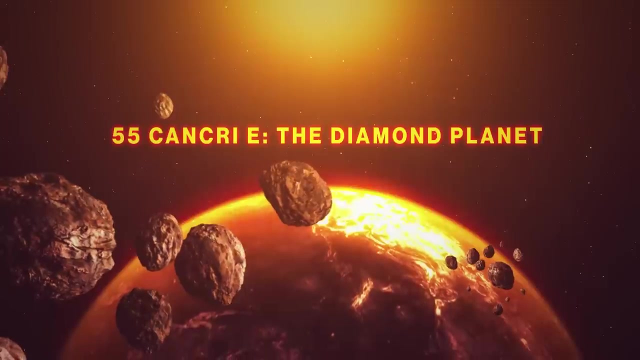 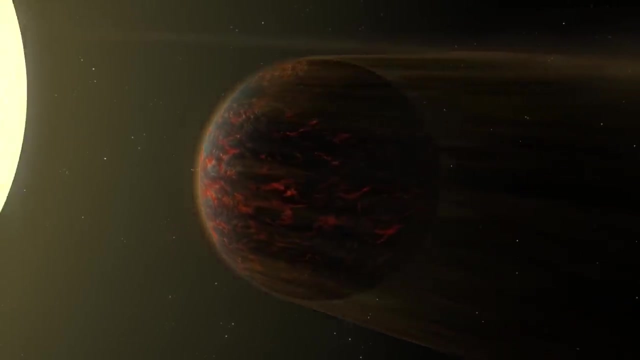 by helping to identify which characteristics might indicate a planet is more likely to be habitable or at least interesting for further study. Scientists have been captivated by 55 Cancri e, an exoplanet twice the size of Earth and located about 40 light-years away in the Cancer constellation. due to its extraordinary characteristic, It's believed to have a surface rich in diamonds. This hypothesis stems from the planet's unique composition and the extreme pressure conditions it harbours. 55 Cancri e is primarily made up of carbon, in the form of graphite and diamond. 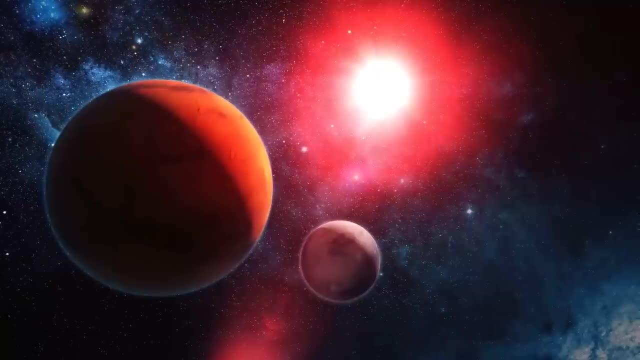 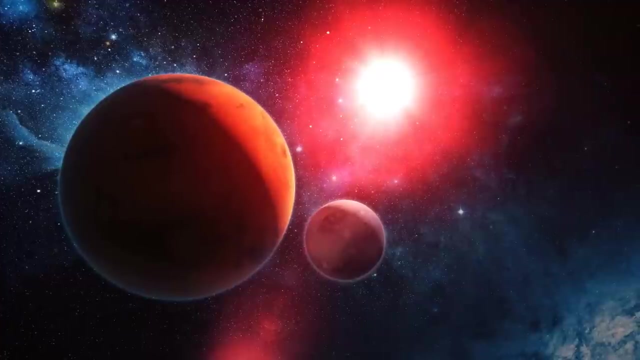 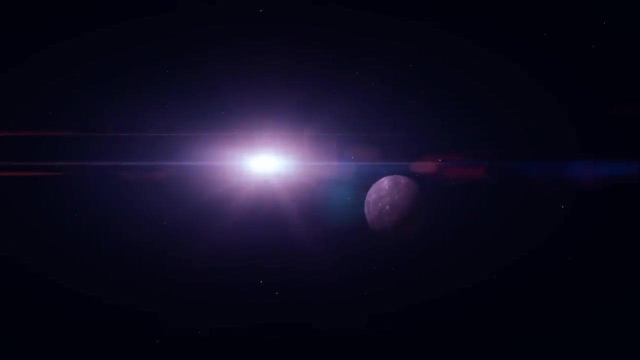 unlike Earth, which has a rocky surface, The immense heat and pressure found on this planet are the key factors that contribute to the transformation of carbon into diamond. The process begins deep within the planet, where temperatures are high enough to melt carbon. This molten carbon under the intense pressure of the planet's gravity. 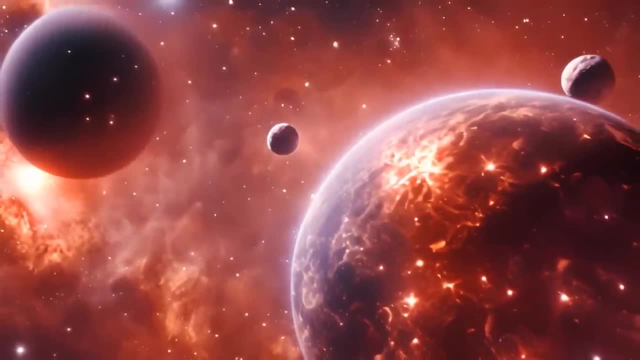 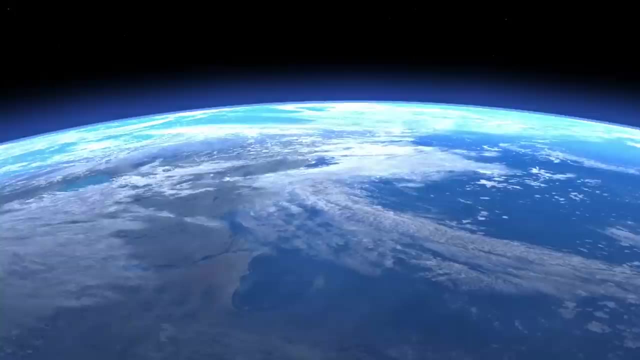 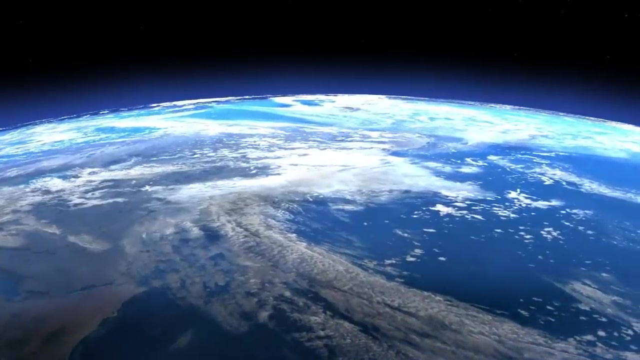 gradually crystallises into diamond. It's a similar process to how diamonds are formed on Earth, but on a much larger scale and at much higher temperatures. On Earth, diamonds form about 150 kilometres below the surface, under high temperatures and pressure over billions of years. 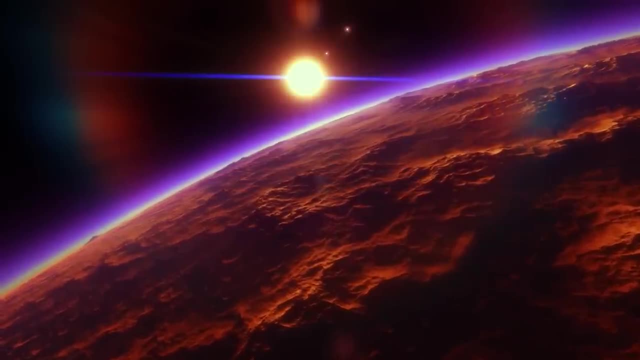 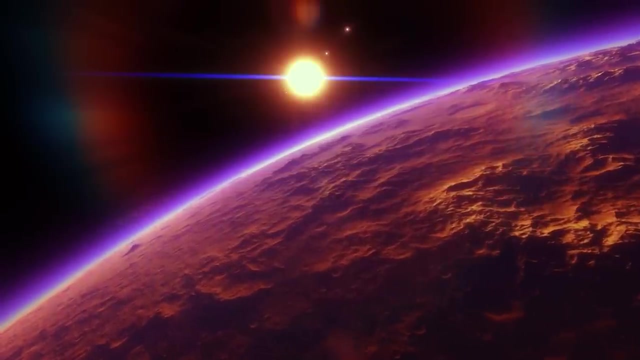 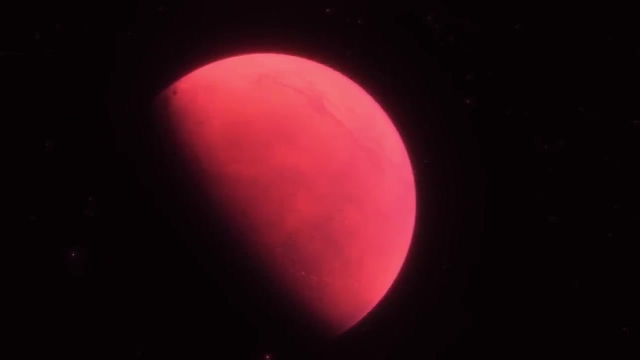 In contrast on 55 Cancri e. this process is supercharged by the planet's extreme conditions, potentially leading to a surface layer composed largely of diamond. This diamond formation is supported by observations of 55 Cancri e's density and the star's carbon-rich composition. 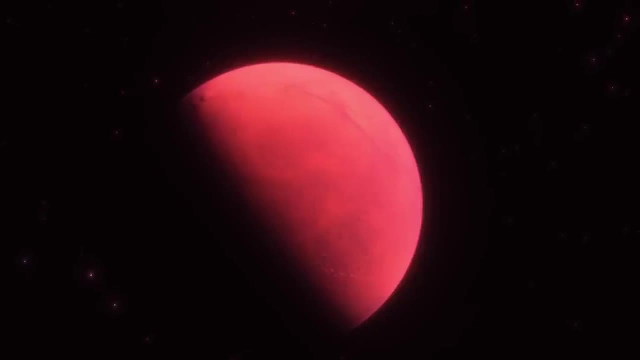 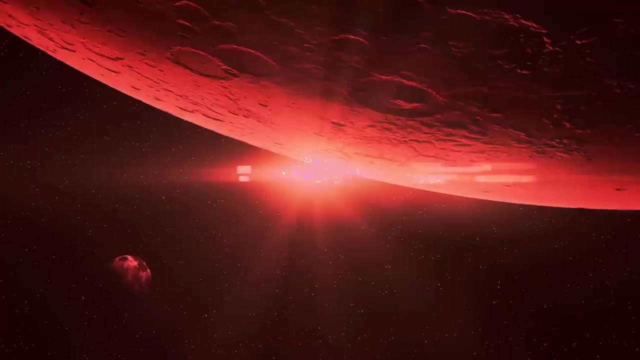 The planet's incredibly high density suggests that it is not composed of light elements like hydrogen and helium, like many gas giants, but heavier elements like carbon. Combined with the carbon-rich nature of its parent star, this leads scientists to conclude that 55 Cancri e could indeed be a diamond world. 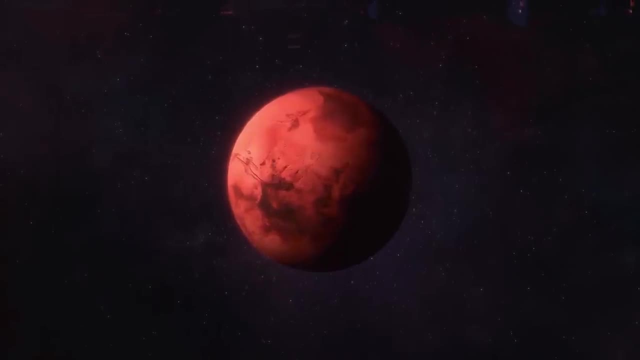 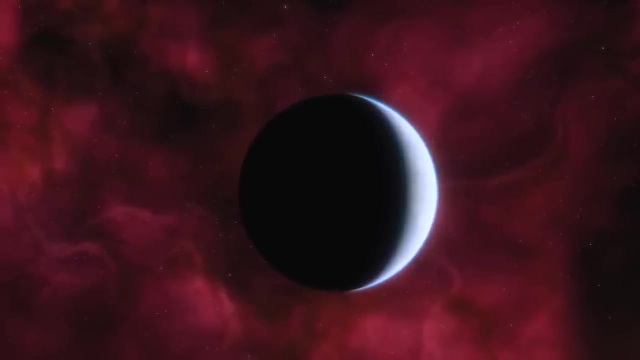 The presence of valuable materials like diamonds on planets such as 55 Cancri e offers profound insights into the diverse processes of planet formation and the conditions that prevail in different parts of our Universe. This revelation underscores the fact that planets can form under a vast array of conditions. 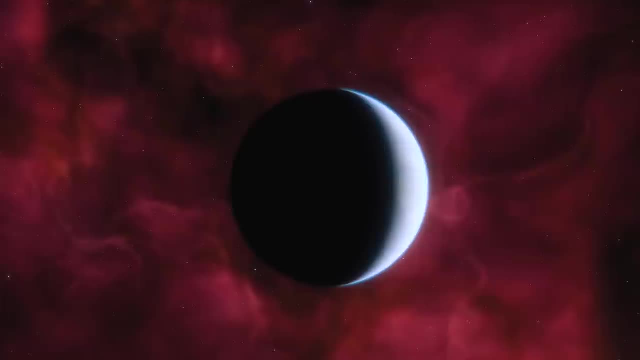 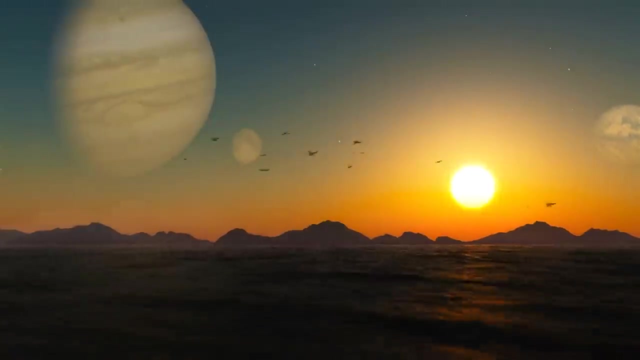 leading to a wide variety of compositions and characteristics. When we observe a planet rich in diamonds, it tells us that the cosmic neighbourhood is filled with worlds that are not only vastly different from our own, but also from each other, highlighting the incredible diversity of planetary systems. This diversity is largely due to the materials that were available in the planet-forming regions around their host stars. In the case of 55 Cancri e, the high concentration of carbon relative to other elements suggests that its formation region was rich in carbon-based materials. 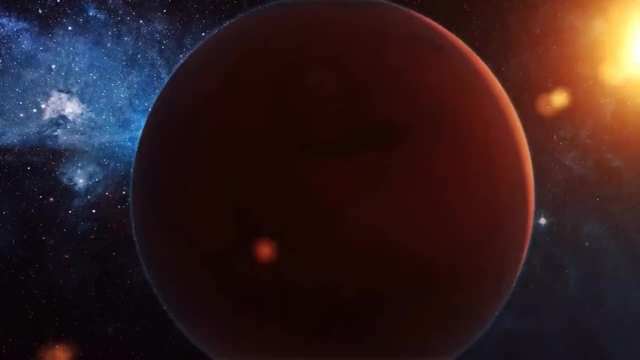 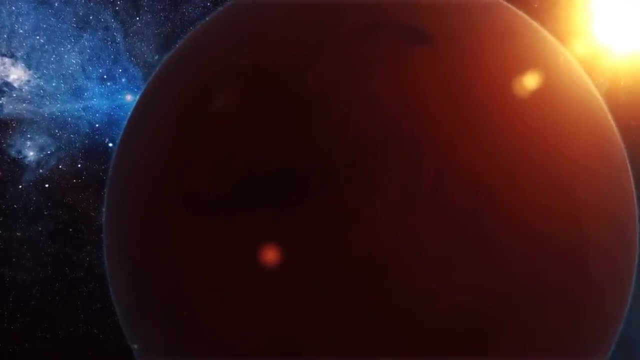 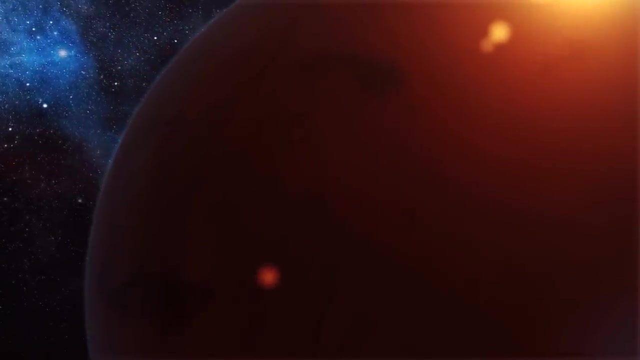 This contrasts with the Earth, where silicon and oxygen are more abundant, leading to a rocky surface. The formation of a diamond planet indicates that the protoplanetary disk from which it formed had a unique chemical composition, emphasising the role of stellar and molecular cloud environments. 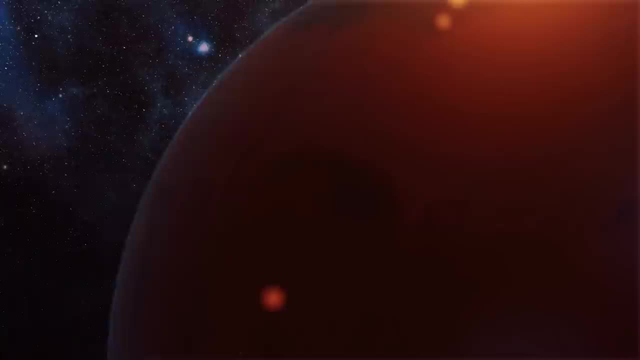 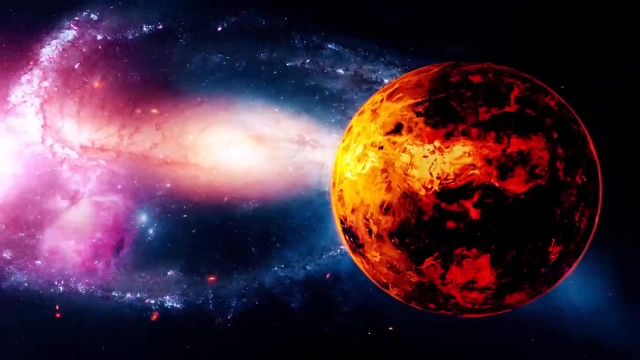 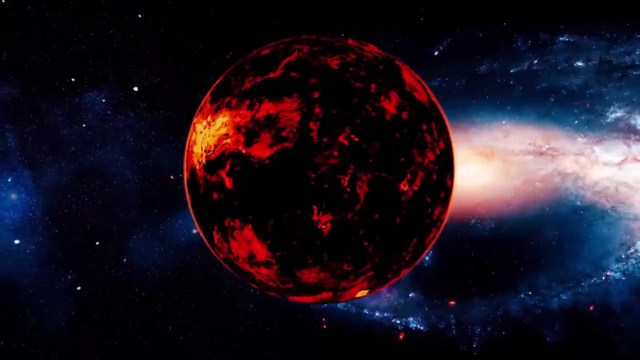 in determining the make-up of emerging planets. The process through which these materials transform under extreme conditions, such as the high pressure and temperature leading to the formation of diamonds, provides valuable clues about the internal processes and heat dynamics of these distant worlds. It suggests that there are planets. 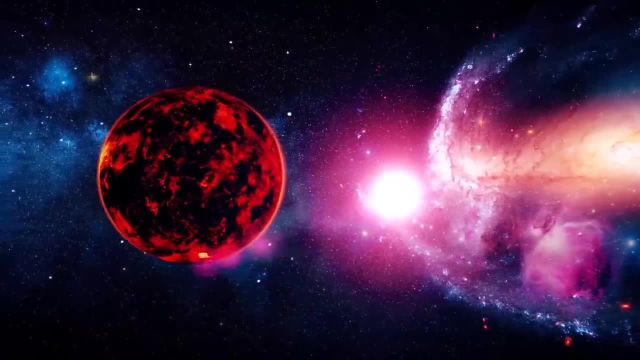 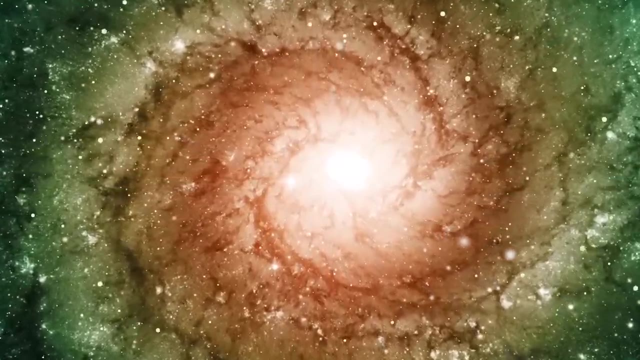 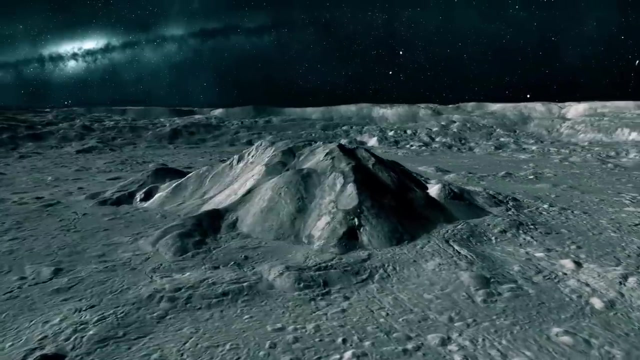 with internal heat and pressure mechanisms vastly different from those found on Earth, offering new avenues for research into planetary geophysics and chemistry. Understanding the formation of planets with surfaces rich in valuable materials also has implications for our knowledge of the life cycle of stars and planetary systems. 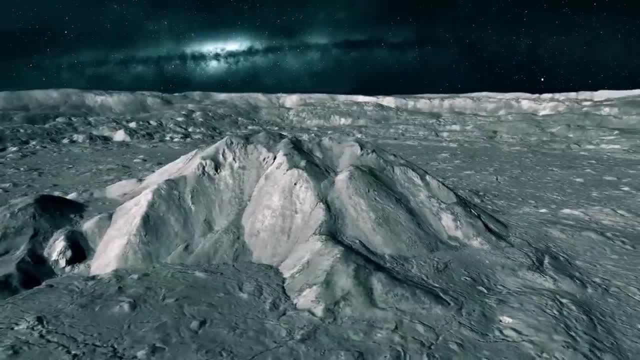 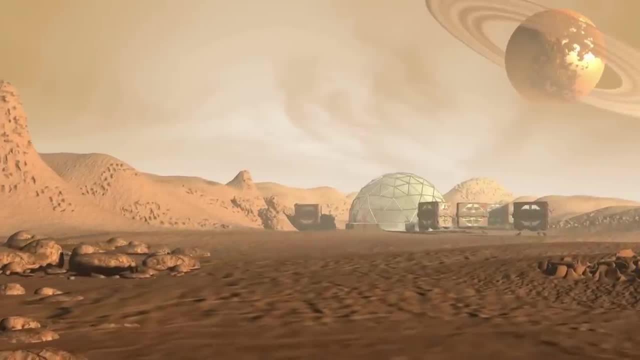 It hints at the evolution of stationary paths that planetary systems can take and the fate of planets over billions of years. For example, a carbon-rich planet might evolve differently over time compared to a water-rich planet or a gas giant affecting its surface conditions. 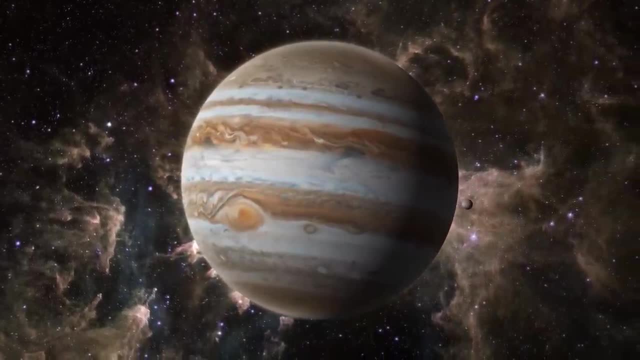 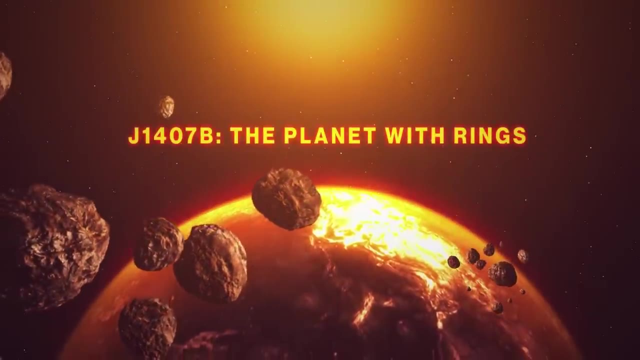 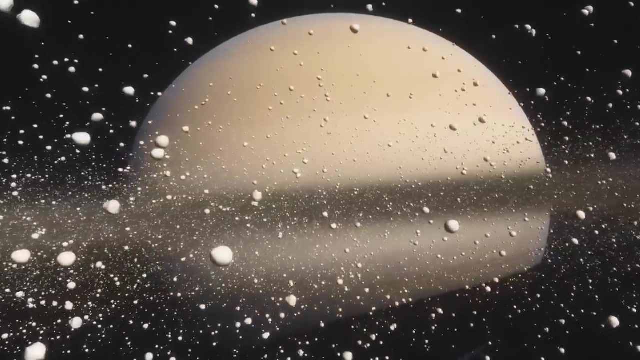 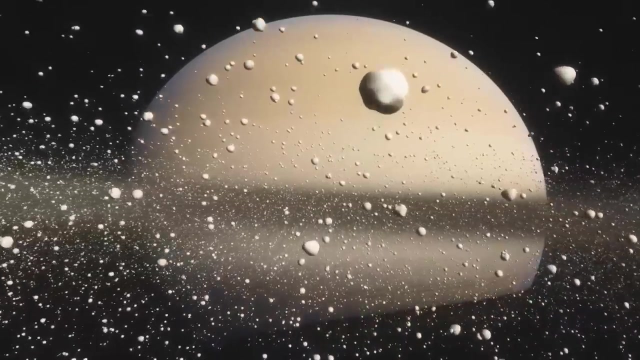 atmosphere and potential for supporting various forms of matter. The rings of J1407b, an exoplanet located hundreds of light-years away from Earth, represent one of the most spectacular phenomena discovered in the realm of exoplanetary science. These rings are not only vast, 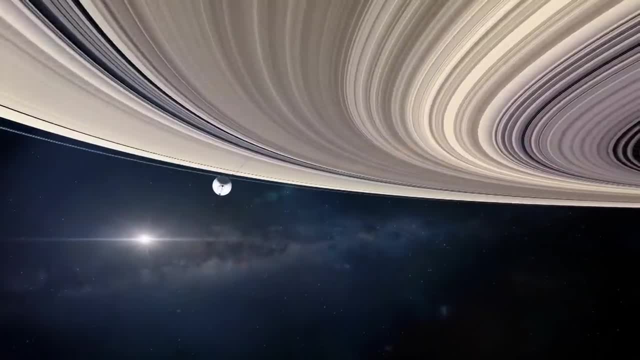 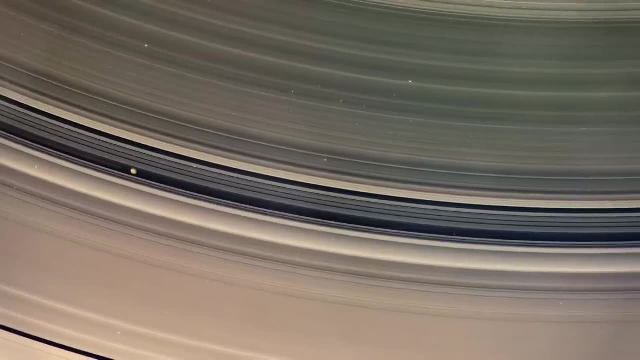 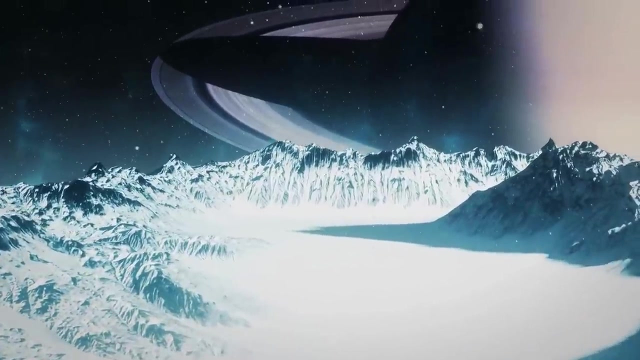 but also incredibly extensive, far surpassing anything found within our own solar system. To put their scale into perspective, the rings of J1407b are so large that they dwarf the ring system of Saturn, the jewel of our solar system, by an astonishing margin. 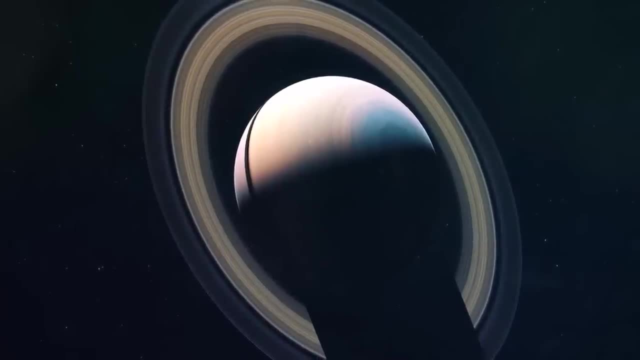 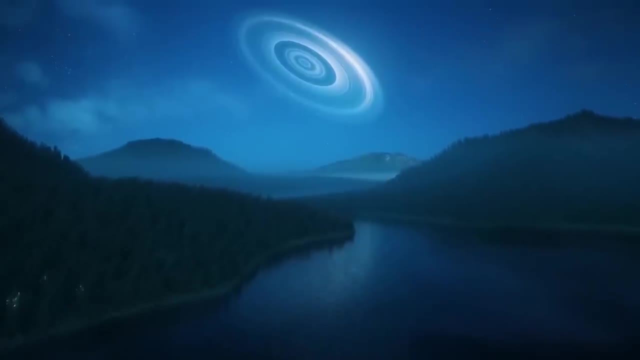 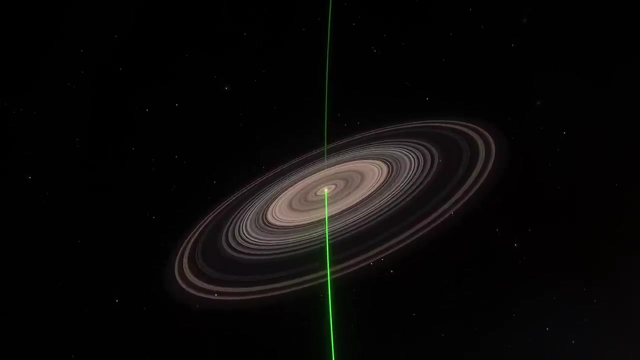 Imagine Saturn's rings, which are already a marvel to behold from Earth, and then picture a ring system that could fit Saturn's rings inside them over 200 times. That's the scale we're talking about. with J1407b, The exoplanet's rings span nearly 90 million kilometres. 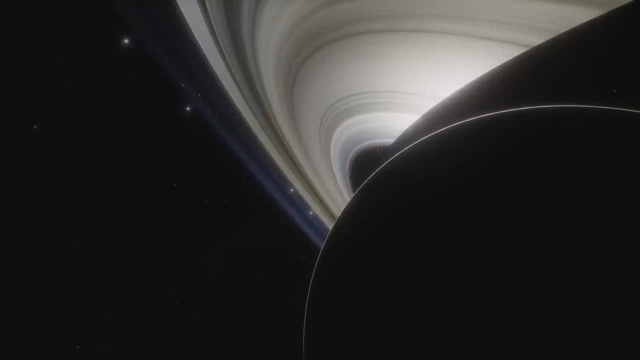 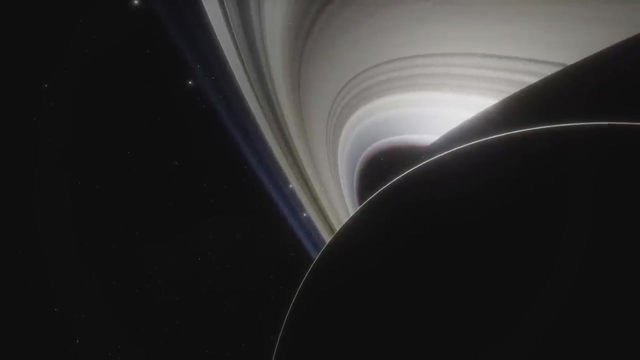 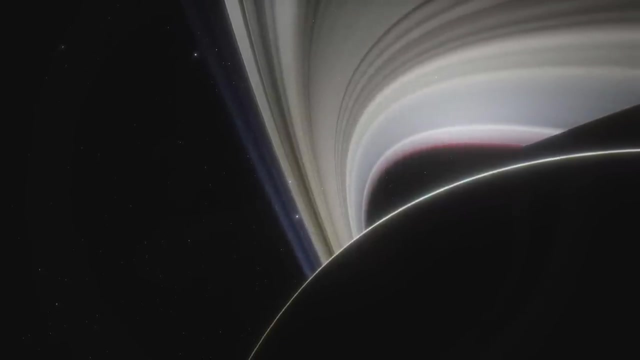 about 56 million miles in diameter. This is about 200 times the size of Saturn's rings, offering a stark illustration of the incredible diversity of planetary systems in the Universe. The discovery of J1407b's rings has provided astronomers and scientists. 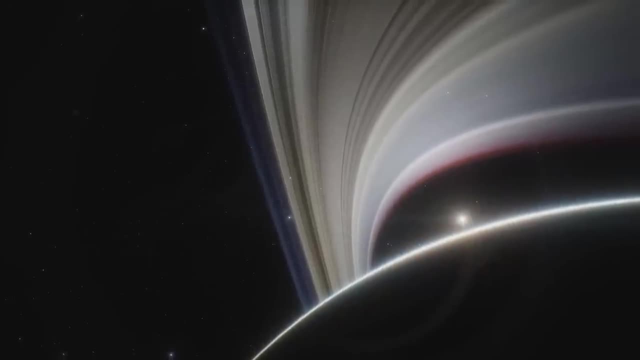 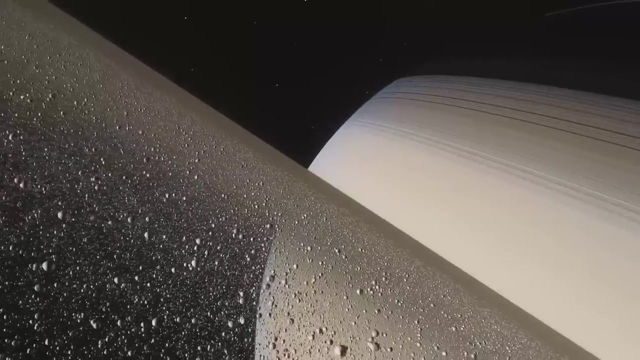 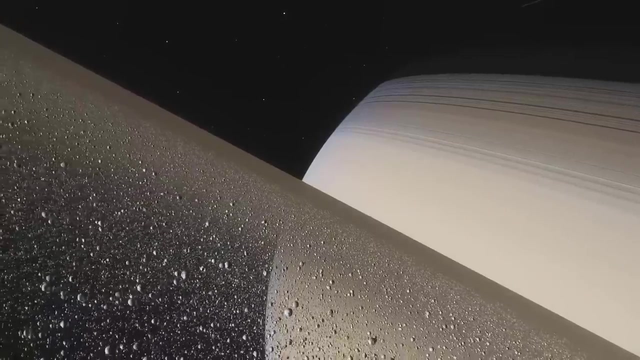 with a fascinating glimpse into the possibilities of planetary formation and the dynamics of ring systems. These rings likely contain ice, rock particles and possibly even moonlets or smaller bodies that orbit J1407b, similar to the shepherd moons found in Saturn's rings. 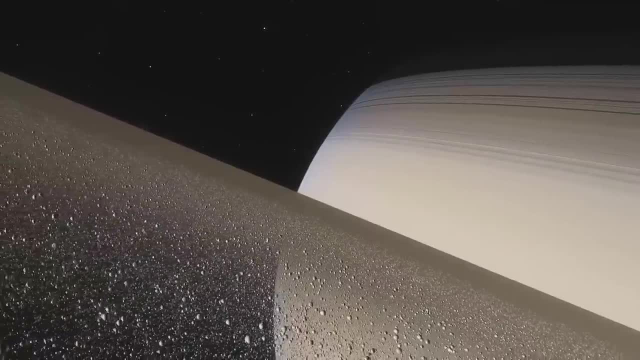 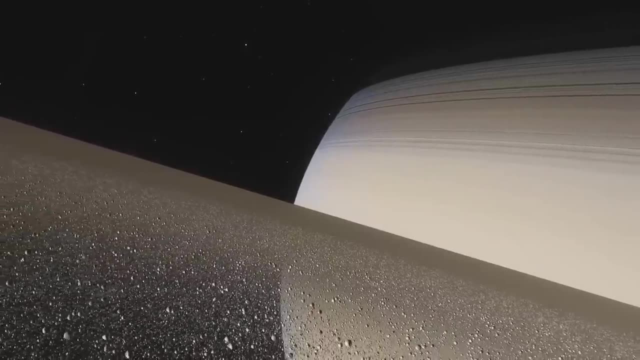 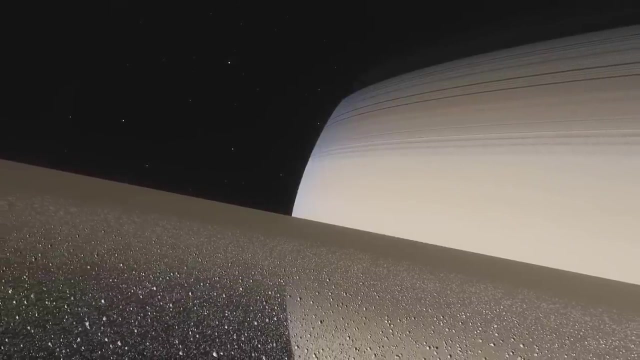 The sheer extent of J1407b's rings suggests that they could be the remnants of a massive collision or the early stages of moon formation, shedding light on processes that could have occurred in the early solar system, but on a much grander scale. 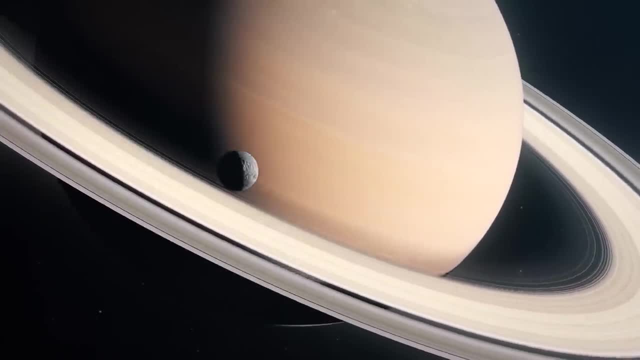 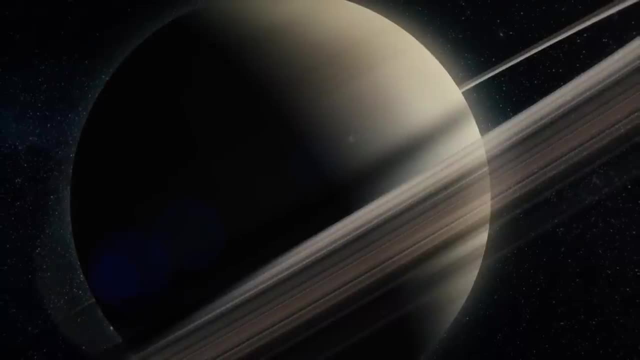 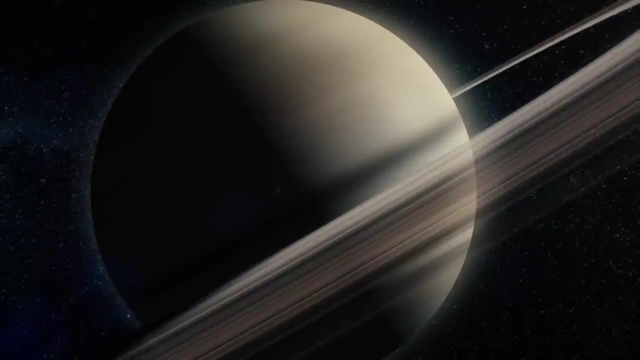 Drawing parallels from our own solar system. the rings of Saturn have shown us how moons can form within a planet's ring system. In Saturn's case, the ice and rock particles within its rings interact under the planet's gravitational influence, sometimes coalescing to form moonlets. 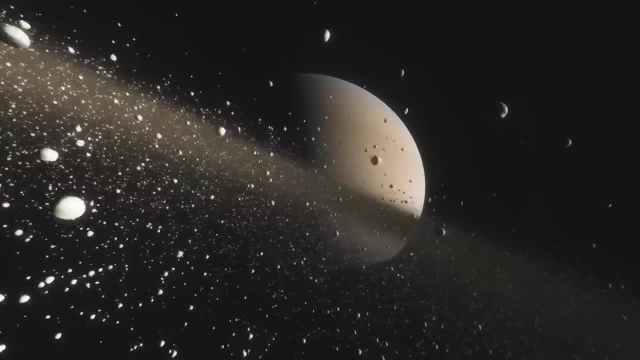 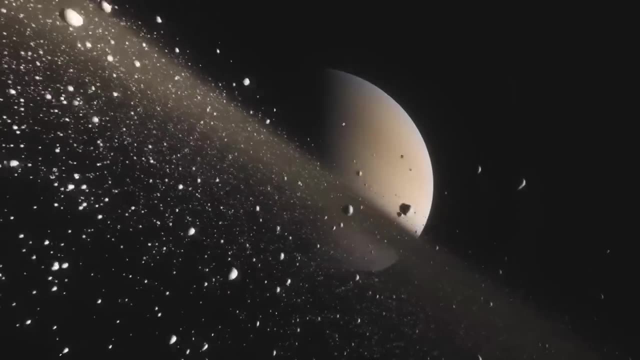 and, over time, potentially larger moons. Given the sheer size and mass of J1407b's rings, which far exceed those of Saturn, it's plausible to suggest that, within this grander scale, similar processes of accretion and moonlet formation. 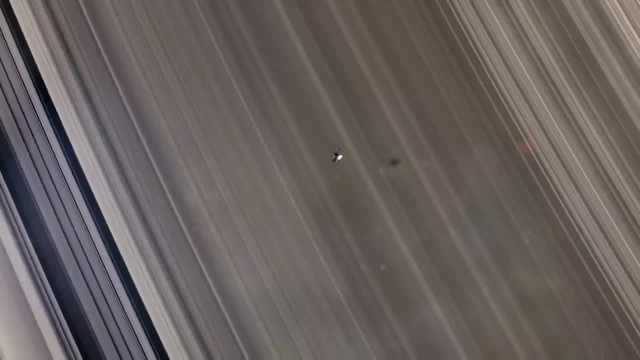 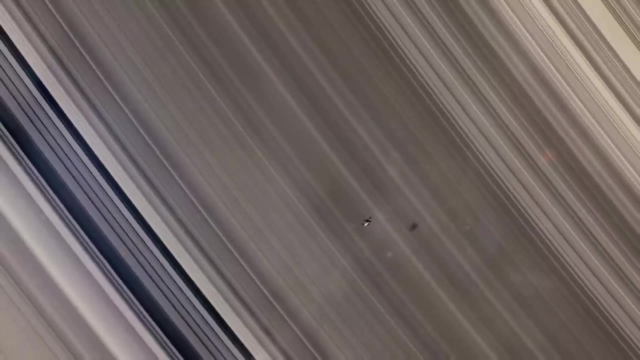 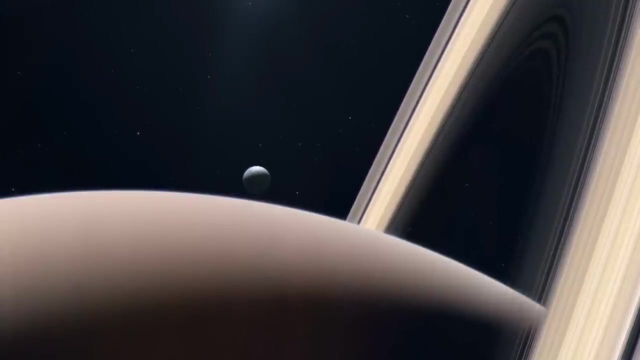 could be taking place. The theory posits that as particles within the rings collide and stick together, they gradually build up to form larger objects. Over time, these objects could accumulate enough mass to clear their orbits within the ring, a critical step towards becoming fully-fledged moons. 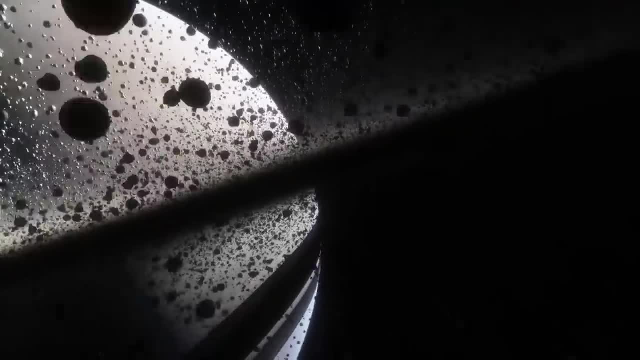 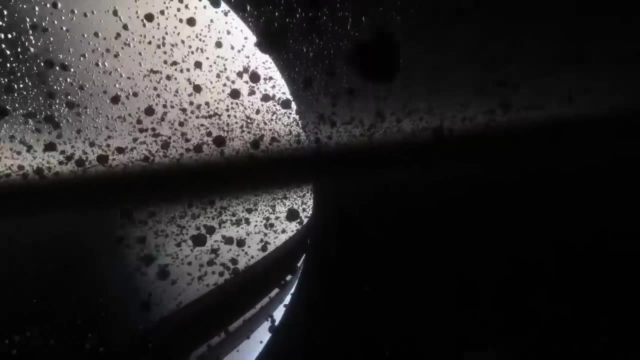 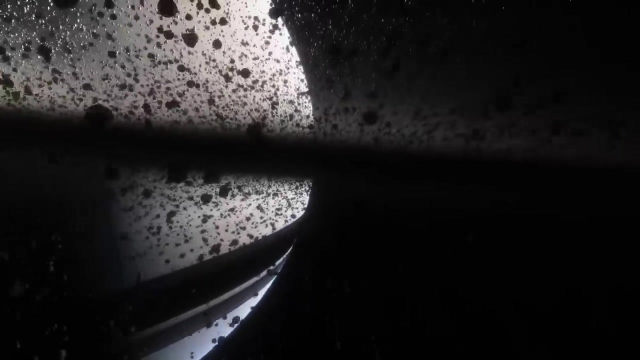 This process, while slow and complex, is a fascinating aspect of planetary science that provides insights into how moons and other small bodies in the solar system might have formed. The formation of moons within J1407b's rings could have significant implications for our understanding of planetary systems. 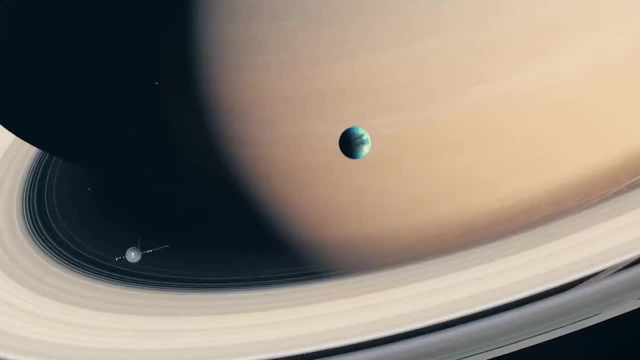 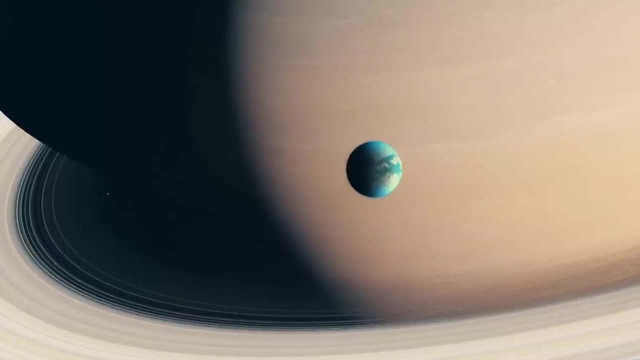 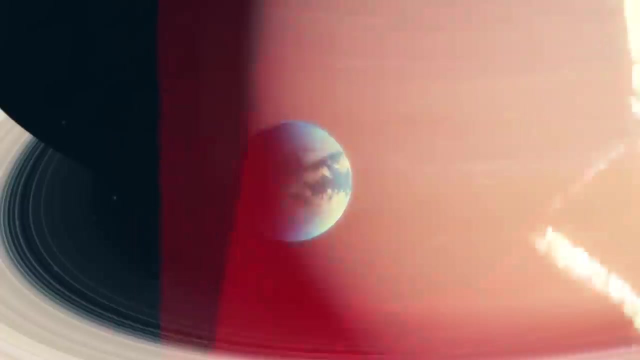 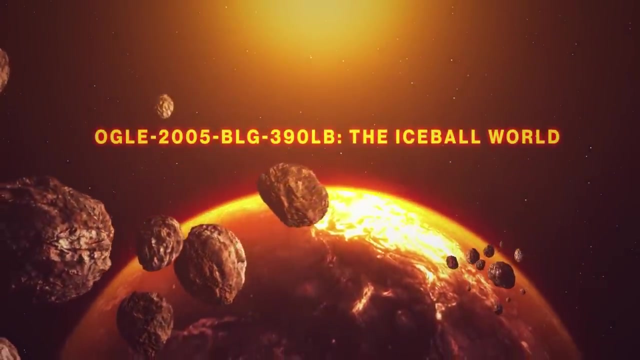 and the dynamics of rings. Observing and studying such a process would offer valuable data on the conditions necessary for moon formation, the timescales involved and how newly formed moons can affect the structure and stability of the rings themselves. OIL-2000-5-BLG-390-LB. 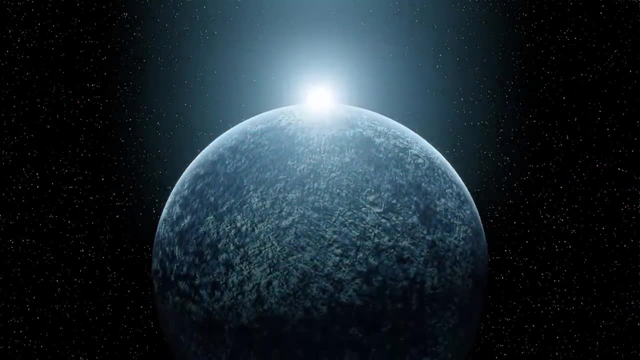 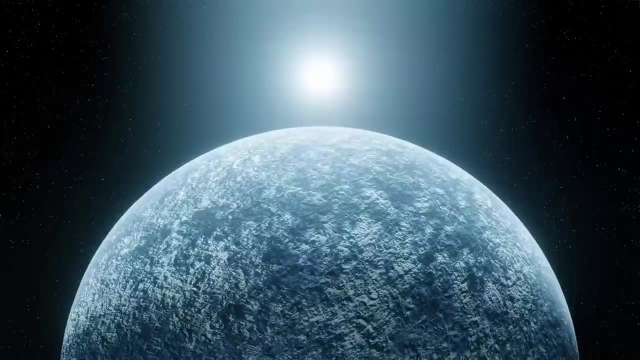 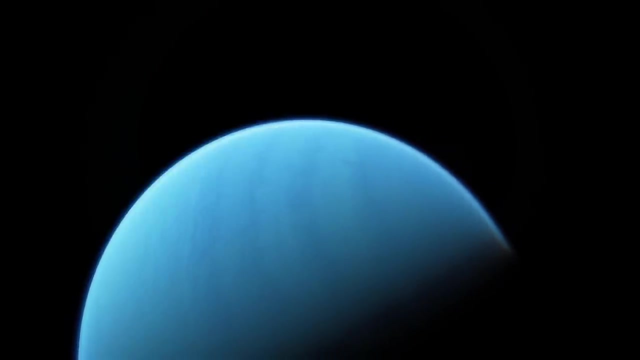 has been categorised as an iceball planet due to its extremely cold surface temperatures and its location in a distant orbit from its parent star, which makes it one of the chilliest exoplanets discovered to date, Situated about 21,500 light-years away from Earth. 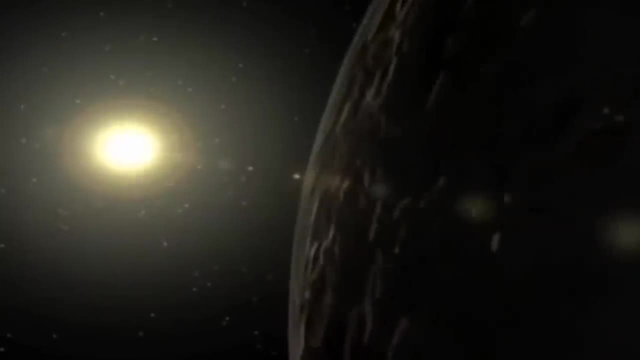 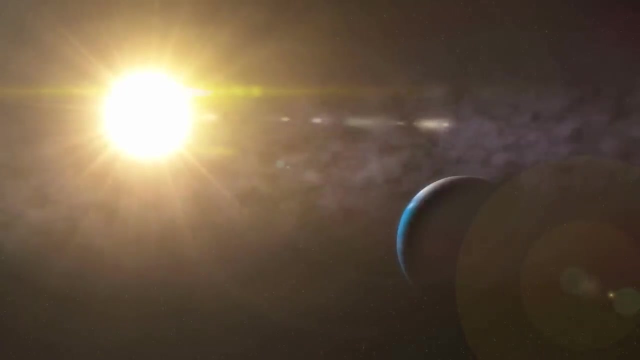 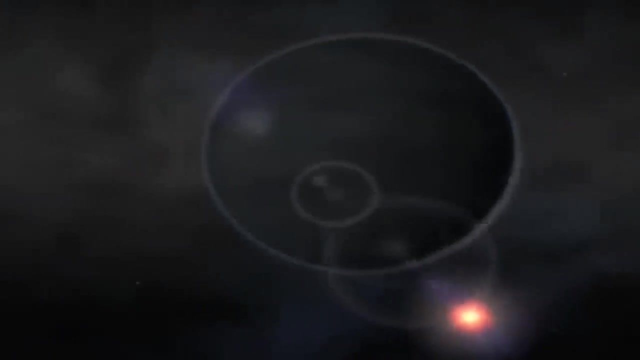 in the constellation of Sagittarius. this remote world orbits its star at a considerable distance, far greater than the Earth's distance from the Sun, resulting in minimal warmth reaching the planet. The term iceball aptly describes OGL-2000-5-BLG-390-LB. 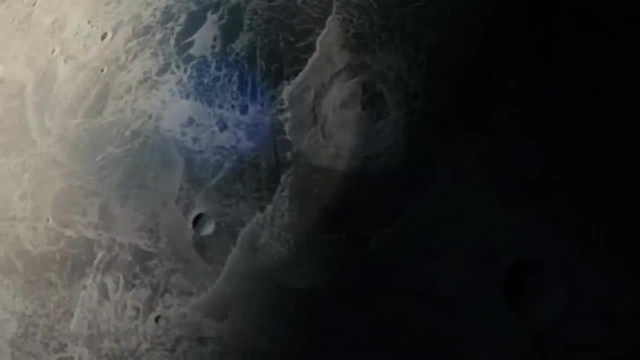 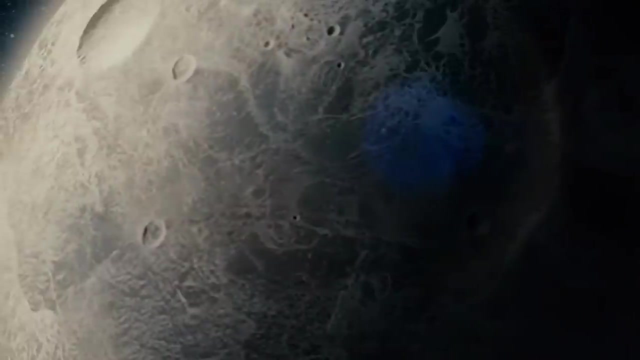 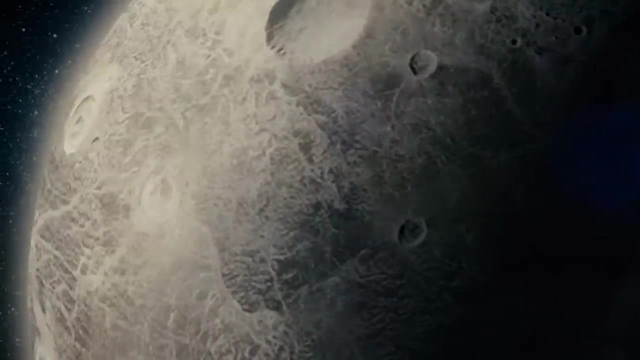 because its surface temperature is estimated to be around minus 220 degrees Celsius, minus 364 degrees Fahrenheit, making it so cold that water on its surface would be permanently frozen, creating a planet-wide icy landscape. The categorisation is based on the planet's 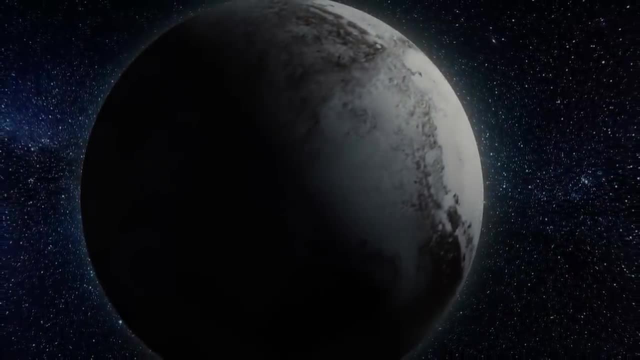 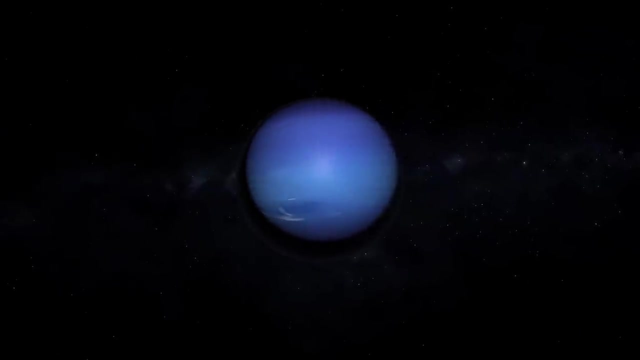 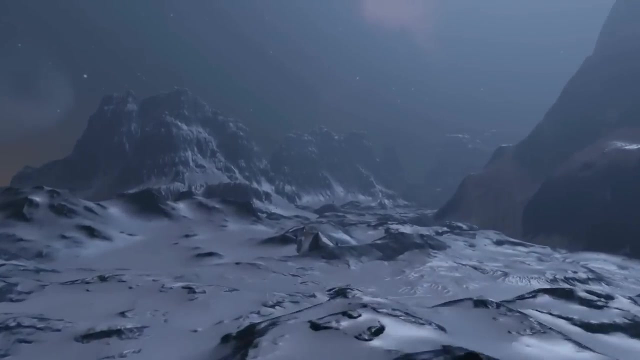 thermal characteristics and its environment. Unlike ice giants in our solar system such as Uranus and Neptune, which have significant atmospheres containing gases like hydrogen and helium, an iceball planet like OGL-2000-5-BLG-390-LB. 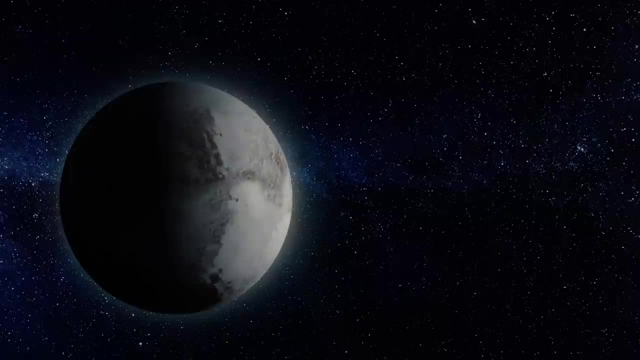 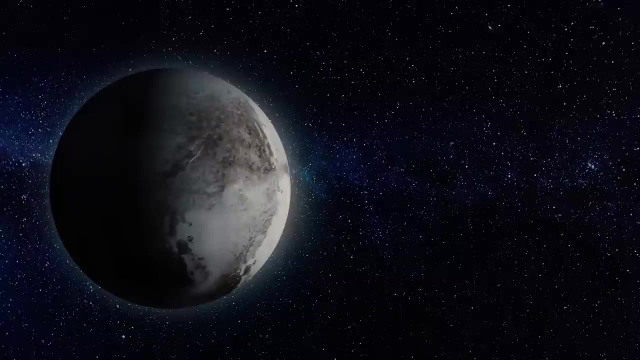 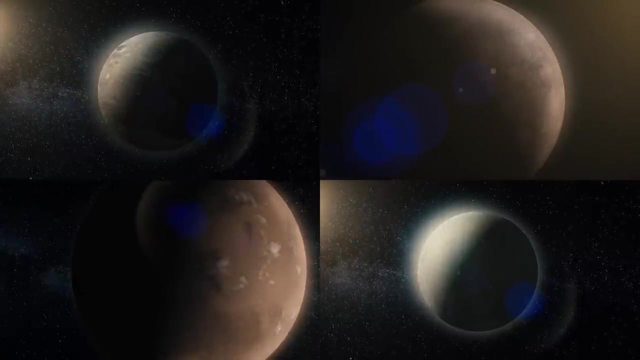 is thought to have a solid surface covered with ice. The extreme cold is attributed to its distant orbit, which prevents it from receiving sufficient solar energy to warm its surface above the freezing point of water. This classification provides insights into the diversity of planetary environments that exist in our universe. 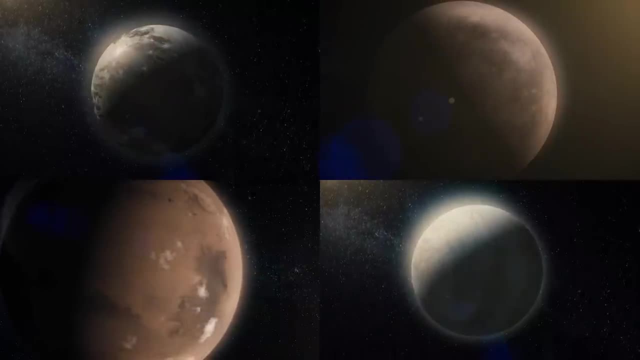 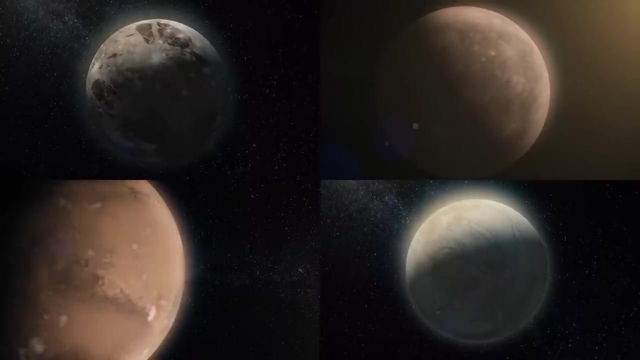 Iceball planets like OGL-2000-5-BLG-390-LB challenge our understanding of habitability and the conditions necessary for life, While the harsh, frigid conditions on such a planet would seem inhospitable to life as we know it. 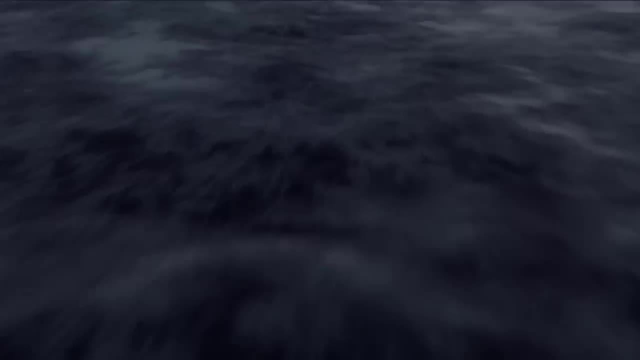 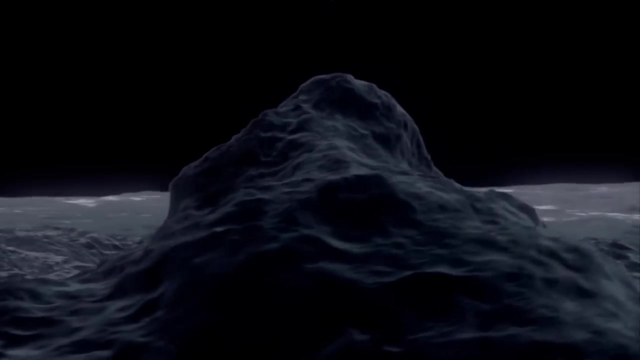 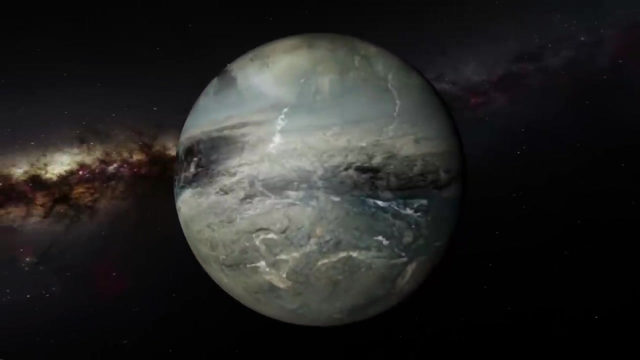 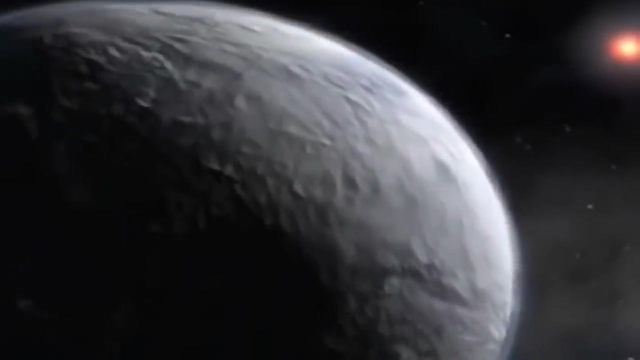 studying these worlds helps scientists understand the outer limits of planetary climates and the potential for water in its various states across different celestial bodies. In planetary science, the temperature of a planet plays a crucial role in determining its atmospheric composition. For a planet as cold as OGL-2000-5-BLG-390-LB, 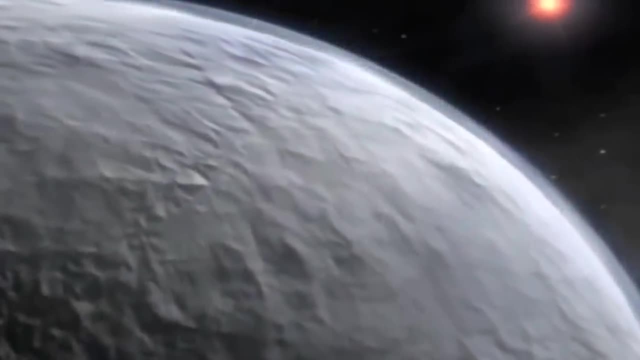 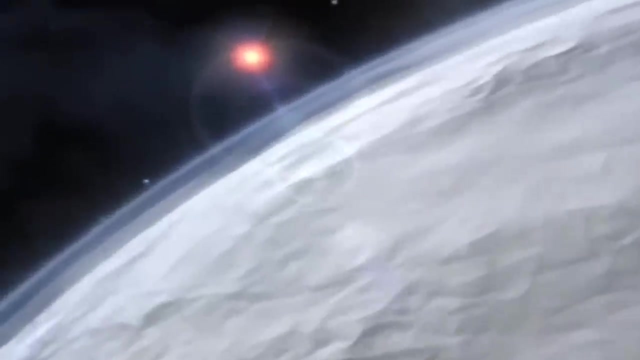 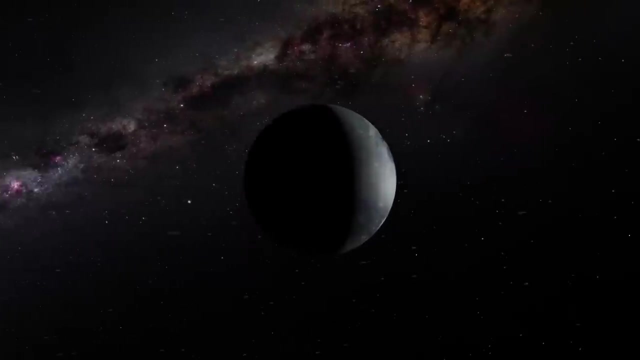 volatile compounds, which are gases at warmer temperatures such as water vapor, carbon dioxide and methane, could freeze out, settling on the surface as snow or ice. This process significantly reduces the thickness and density of the atmosphere, as fewer gases remain in a vaporous state. 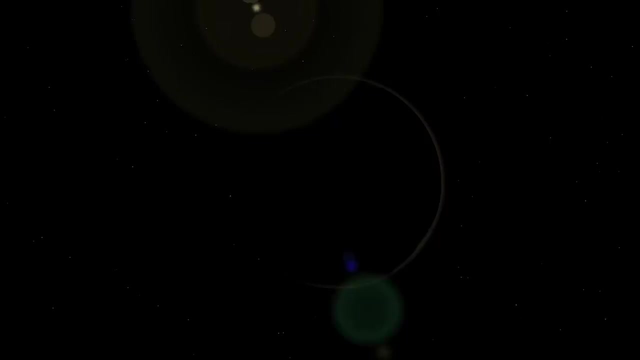 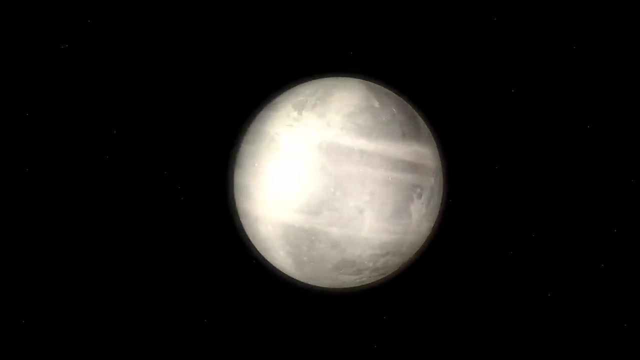 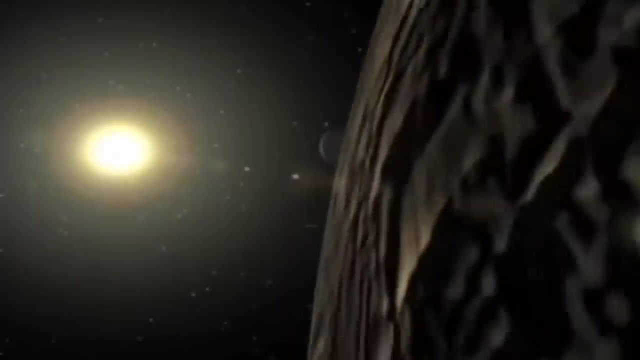 to form an extensive atmospheric layer. The lack of a substantial atmosphere on an iceball planet like OGL-2000-5-BLG-390-LB also means that any heat from its star or internal heat generated by the planet itself would not be efficiently trapped. 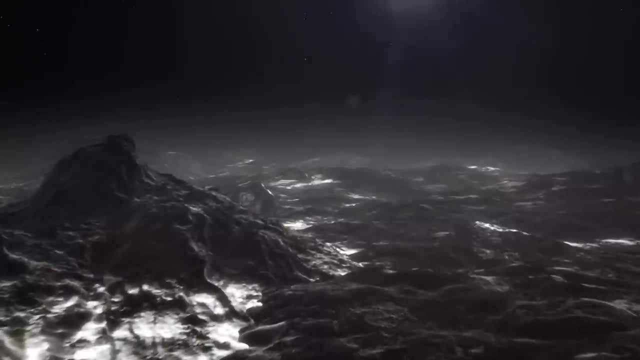 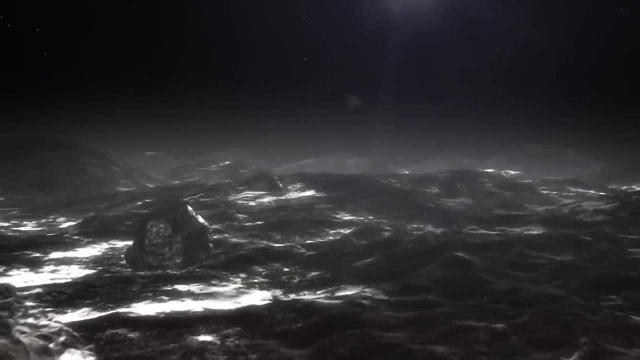 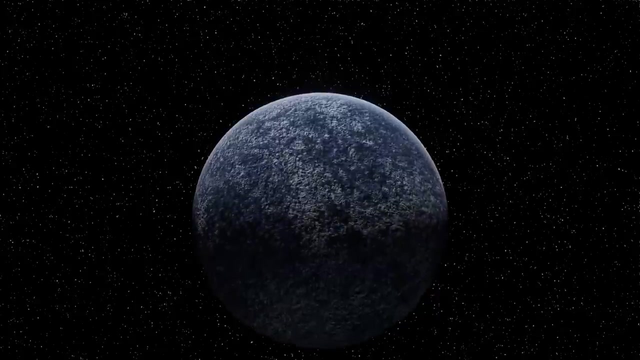 exacerbating the cold conditions. This contrasts with planets that have thick atmospheres, where greenhouse gases can trap heat and maintain a relatively warm environment, even at significant distances from their stars. The temperature and potential atmospheric conditions. on OGL-2000-5-BLG-390-LB. 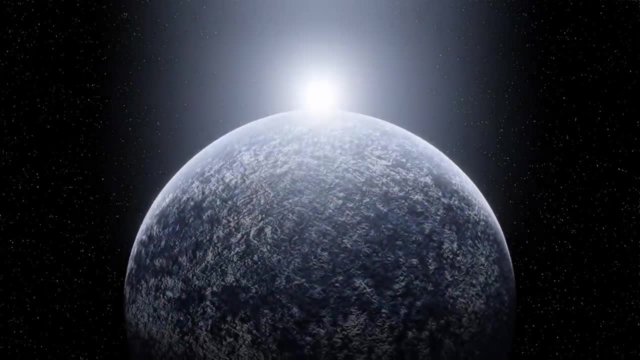 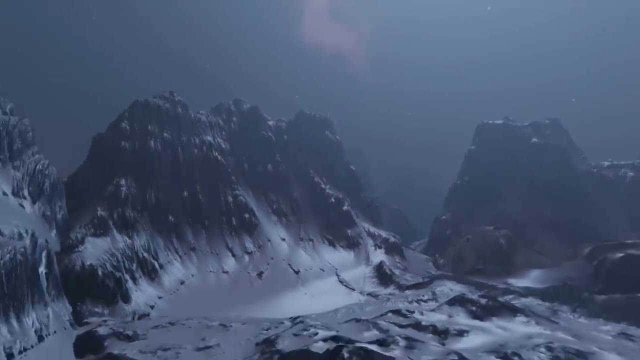 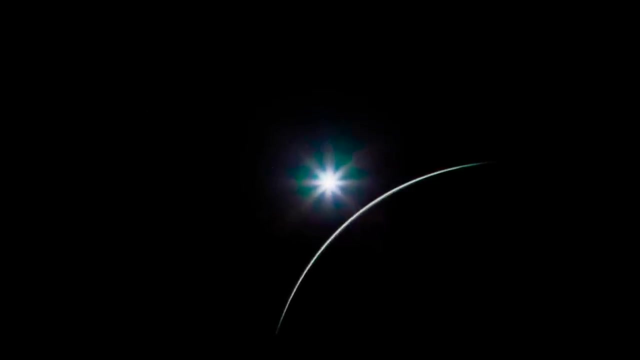 offer insights into the planet's capacity to host life as we know it. The absence of a substantial atmosphere and the extreme cold greatly diminished the likelihood of liquid water existing on the surface, a key ingredient for life on Earth. However, these conditions also open up intriguing questions. 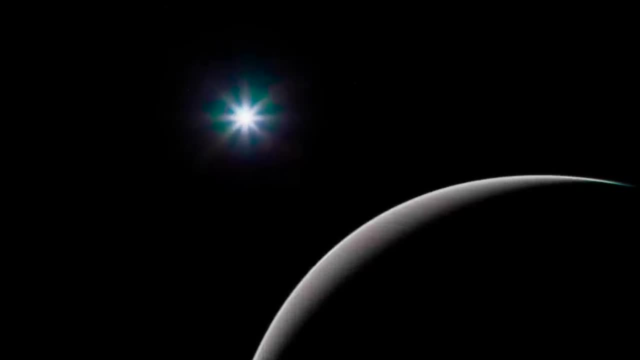 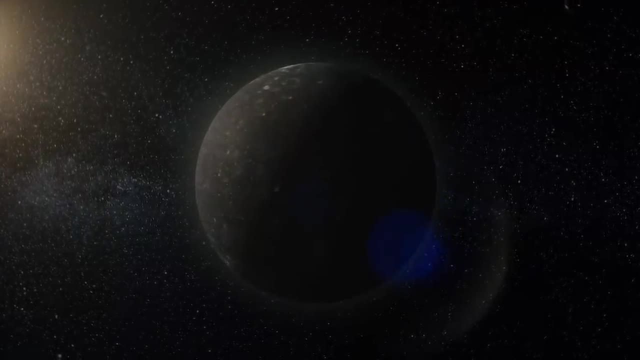 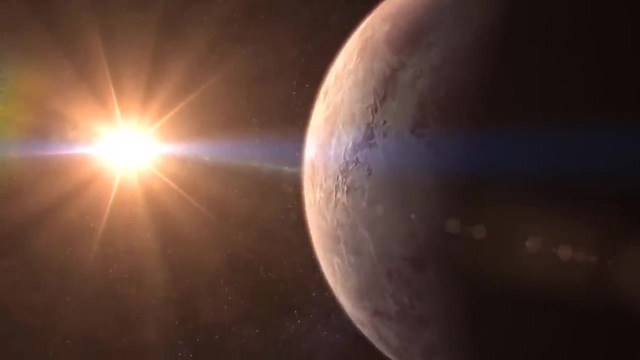 about the types of life that could potentially exist in extreme environments, or what scientists call extremophiles. pushing the boundaries of our understanding of habitability in the universe: Studying distant and cold planets like OGL-2005-BLG-390-LB. 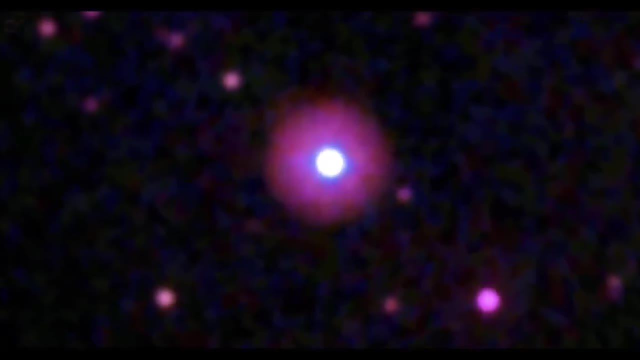 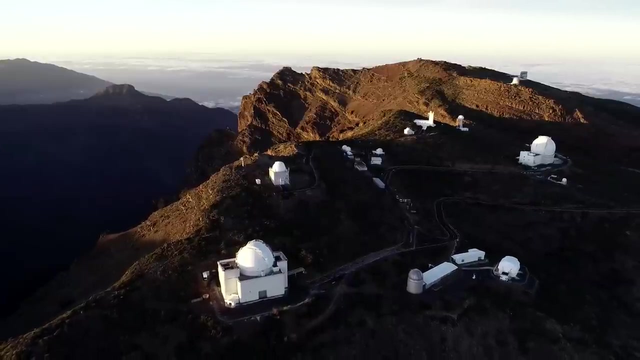 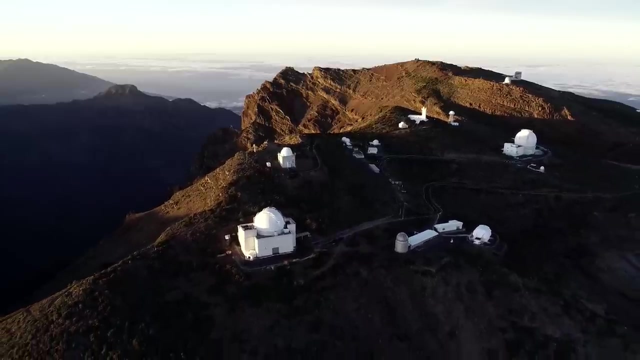 located thousands of light-years away from Earth involves the utilization of advanced astronomical techniques and technologies. Scientists rely on a combination of observational strategies and theoretical models to uncover the secrets of such remote worlds, despite the vast distances and their faint visibility. One of the key methods used in the discovery and study 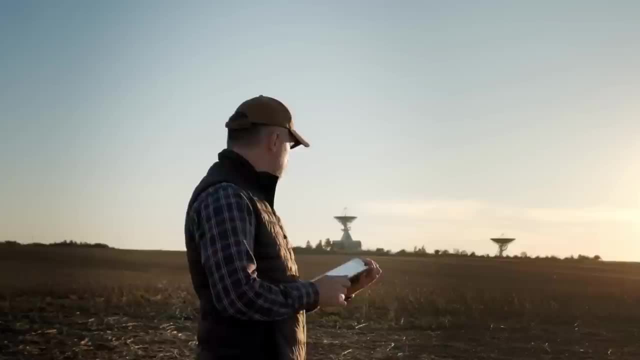 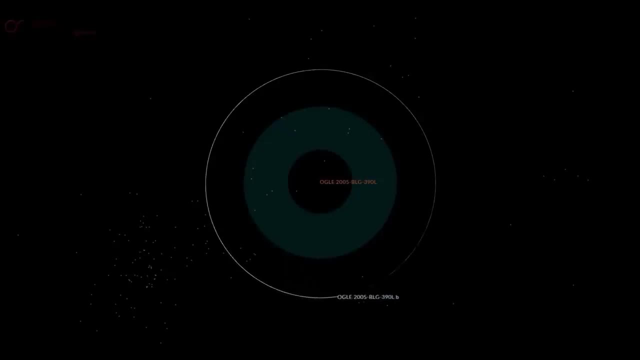 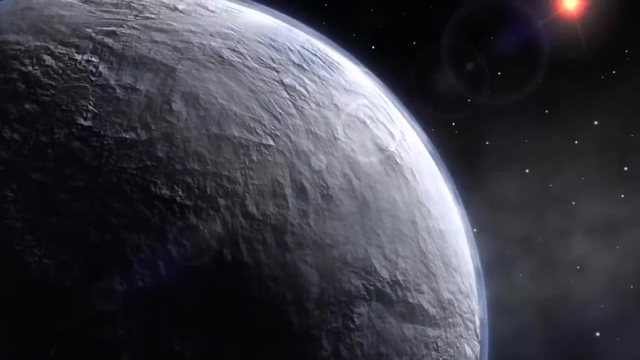 of OGL-2005-BLG-390-LB is gravitational microlensing. This phenomenon occurs when the gravity of a star or planet bends and magnifies the light of a background star as it passes in front of it. from our point of view, 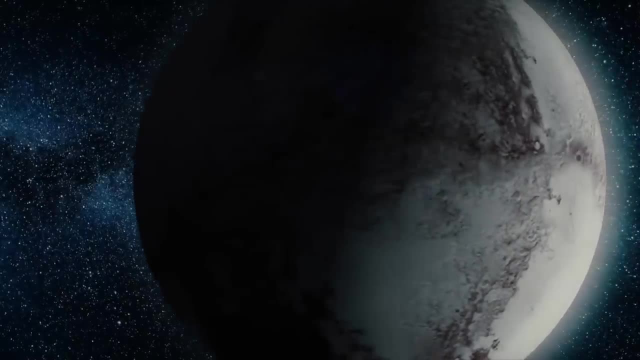 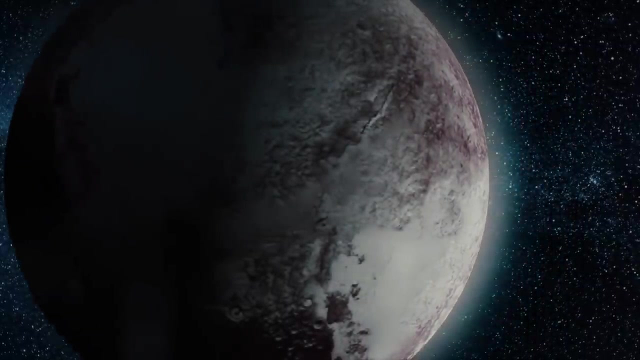 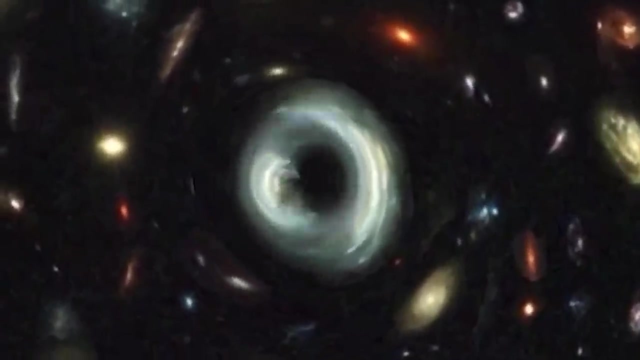 This effect can reveal the presence of planets around the foreground star, including details about their mass and distance from the host star. Gravitational microlensing is particularly powerful for detecting exoplanets that are too distant or too faint to be observed through more conventional methods. 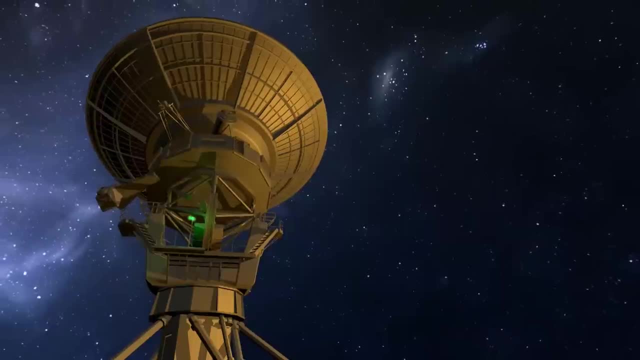 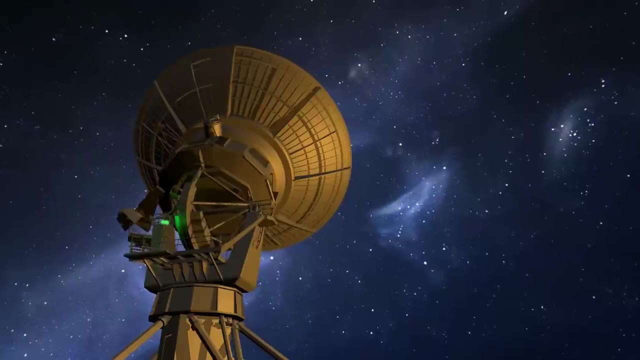 such as the transit method or direct imaging. It allows astronomers to detect planets that do not emit light on their own and are far from their host stars, making it ideal for discovering cold iceball planets like OGL-2005-BLG-390-LB. 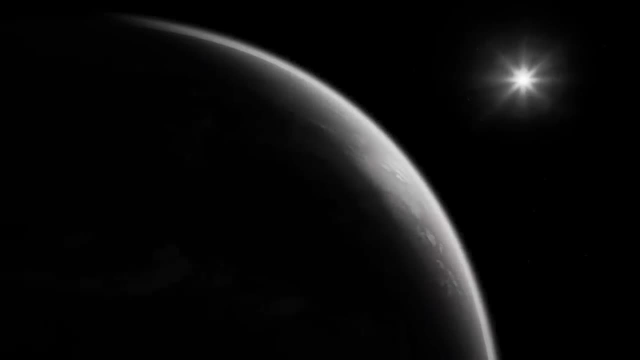 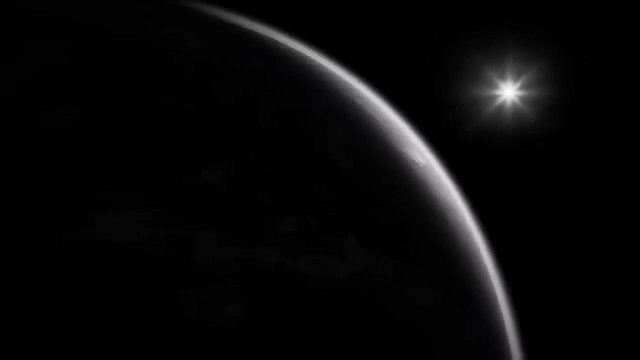 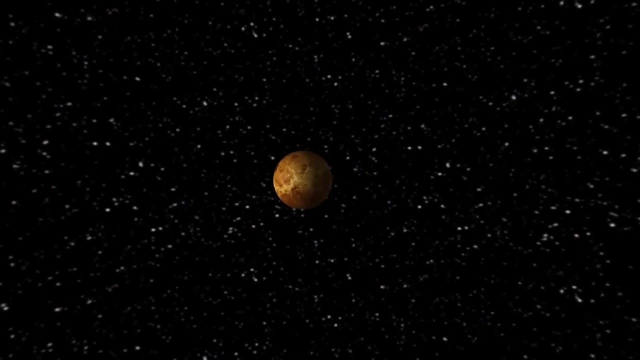 The technique does not rely on the light from the host star or the planet itself, But rather on the way the gravity of the planet affects the light of a more distant star. This method has the unique advantage of being sensitive to low-mass planets and can detect them at a wide range of distances. 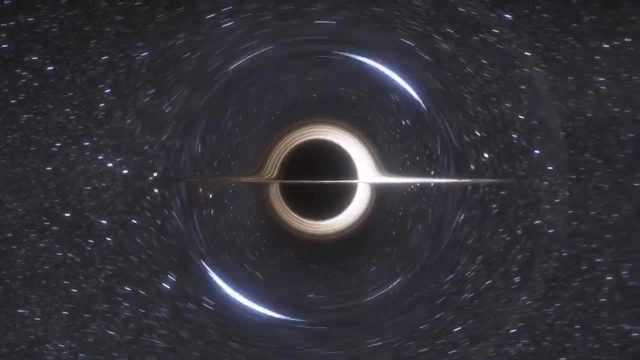 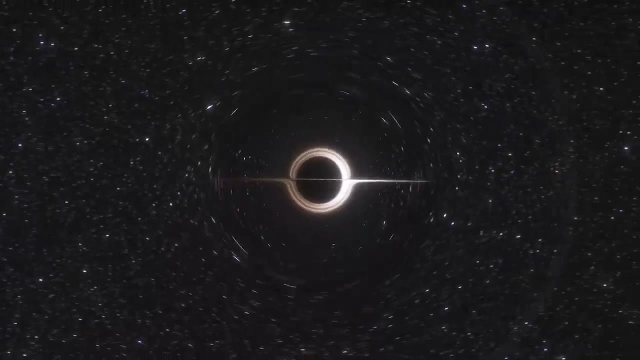 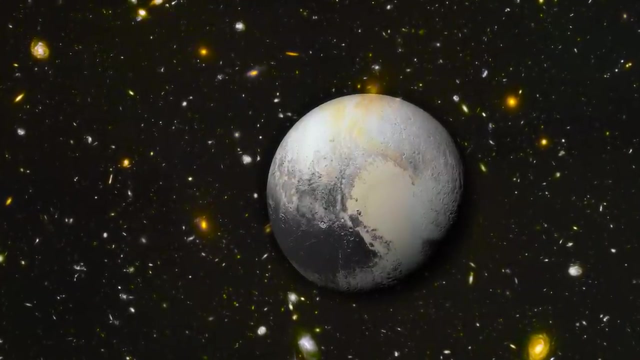 from their host stars. In addition to gravitational microlensing, scientists use computer models and simulations to predict and understand the conditions on such planets By inputting the known physical characteristics of the planet, such as its mass, distance from its star and orbital period. 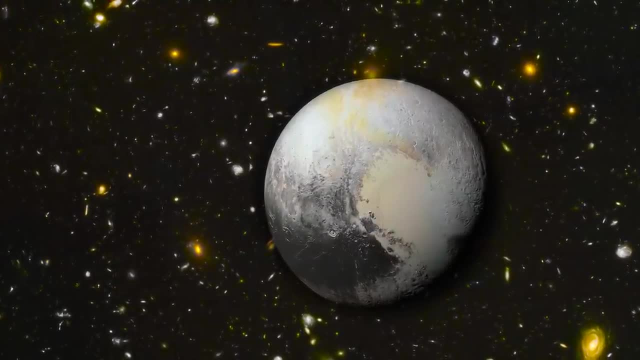 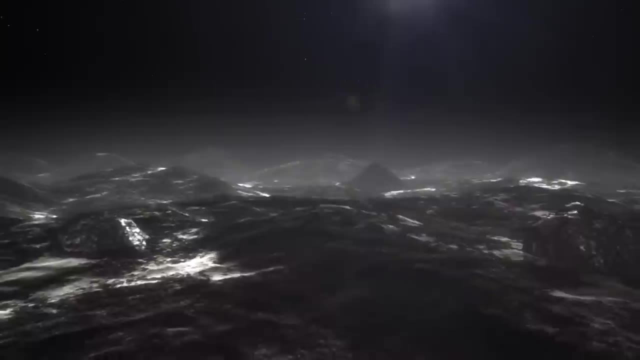 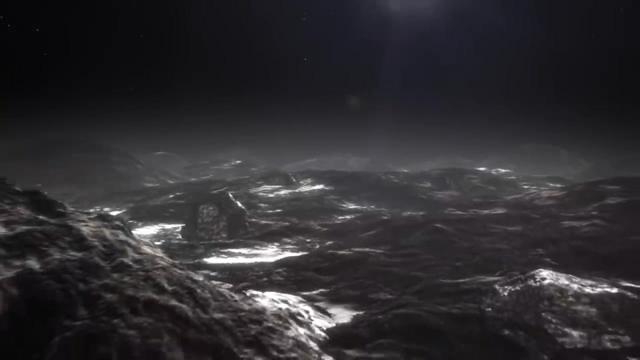 into these models, scientists can make educated guesses about the planet's atmosphere, surface conditions and potential for hosting water or ice. These models help astronomers to infer the planet's temperature, atmospheric composition and potential for having a solid surface. Telescopes equipped with sensitive instruments. 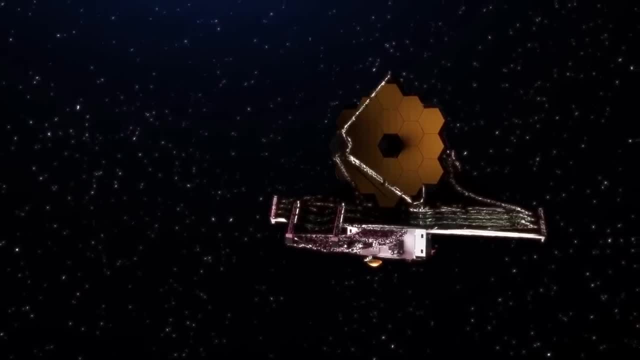 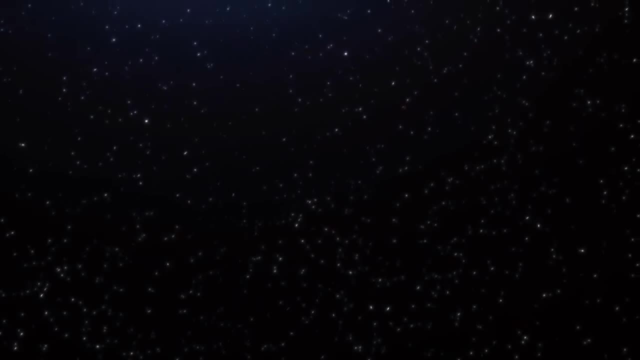 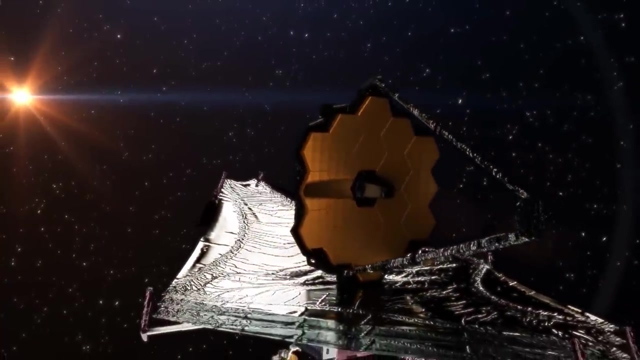 both ground-based and in space, play a crucial role in following up on discoveries made through microlensing. They can provide additional data on the star system's characteristics, helping to refine measurements and confirm the presence of the planet, Although direct observations of the planet's atmosphere or surface 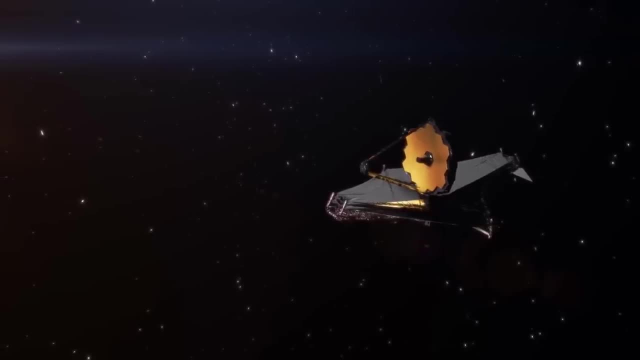 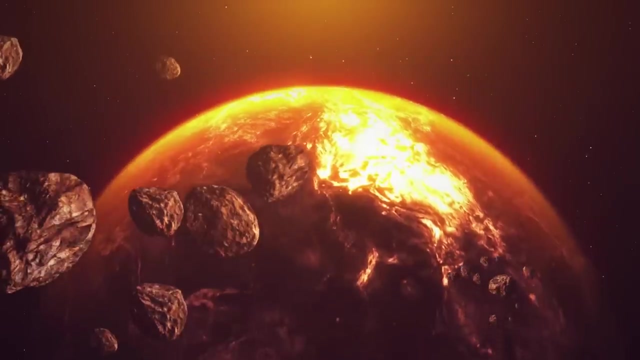 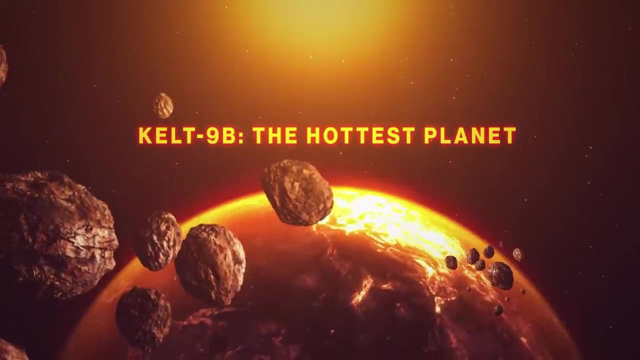 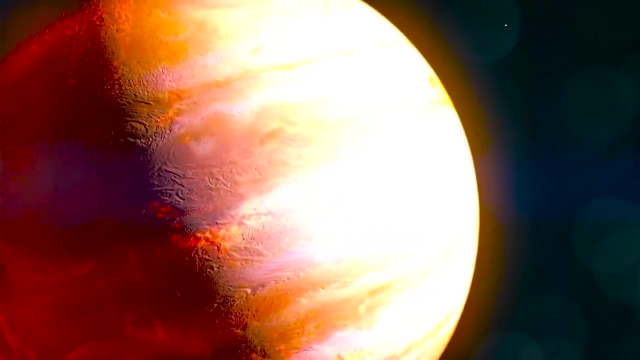 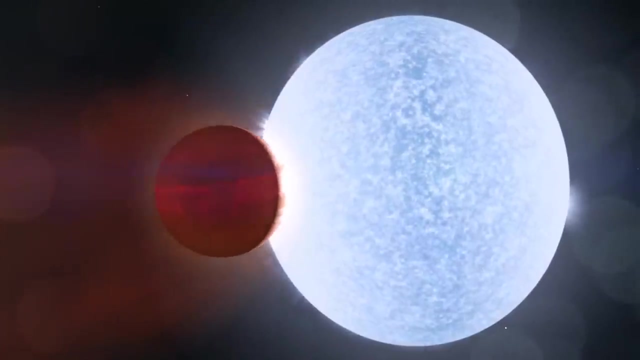 are challenging at such great distances. the combination of these techniques gives scientists valuable insights into the nature of these distant worlds. Counter-Belt motif: Pvid- Reddit Limited. Keld 9b: Keld 9b's status as the hottest known exoplanet. 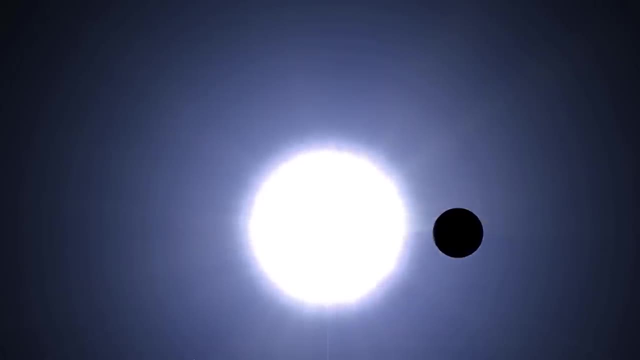 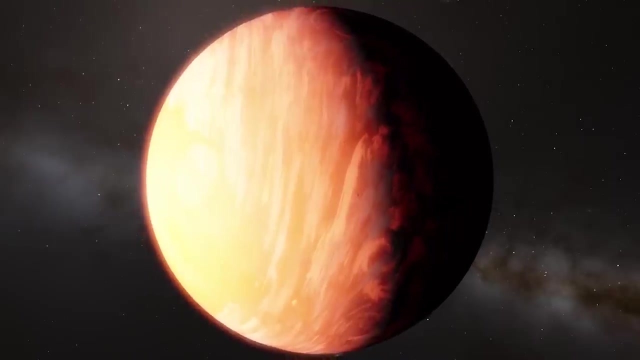 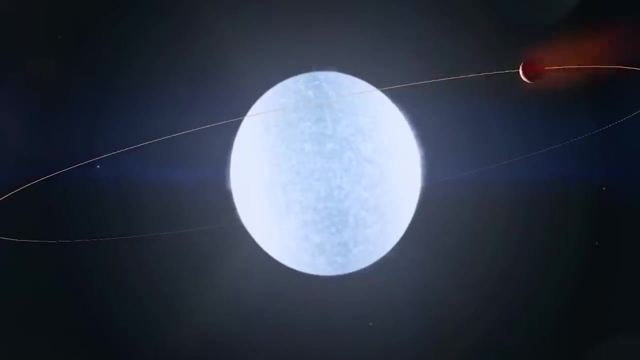 is a direct result of several extreme factors contributing to its high temperatures. This star is almost twice as hot as our Sun, making it one of the hottest stars known to host a planet. The proximity of KELT-9b to its star is astonishingly close, with an orbital period of just. 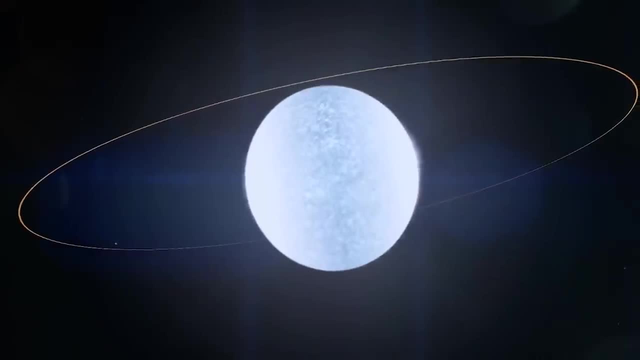 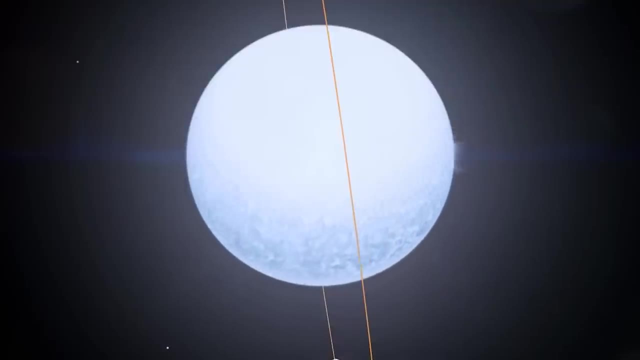 about 1.5 Earth days. This tight orbit places KELT-9b in an intense stellar environment, receiving a colossal amount of radiation from its host star. The star's high temperature and the planet's close orbit mean that KELT-9b is. 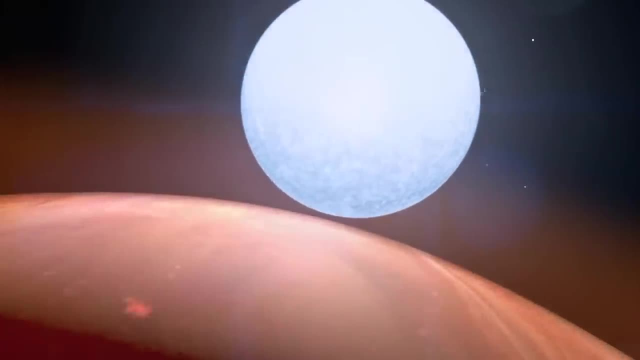 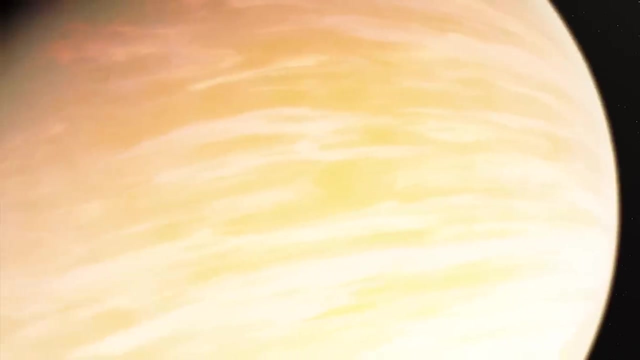 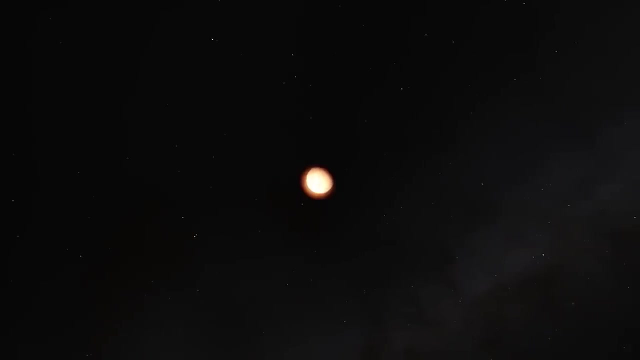 subjected to thousands of times the radiation that planets in our solar system receive from the Sun. This exposure heats the atmosphere of KELT-9b to more than 4,300 degrees Celsius, about 7,800 degrees Fahrenheit hotter than many stars and well above the melting points of most materials. 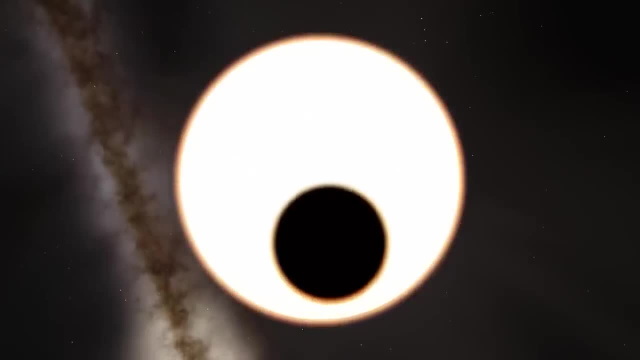 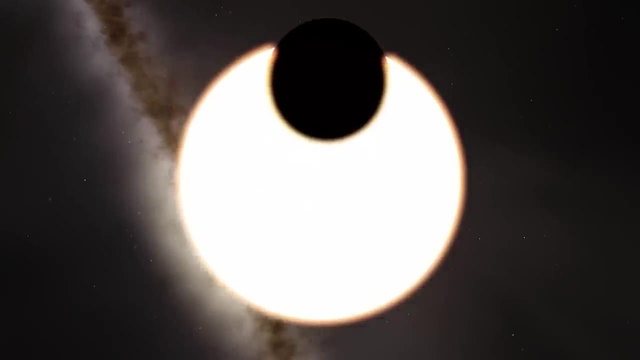 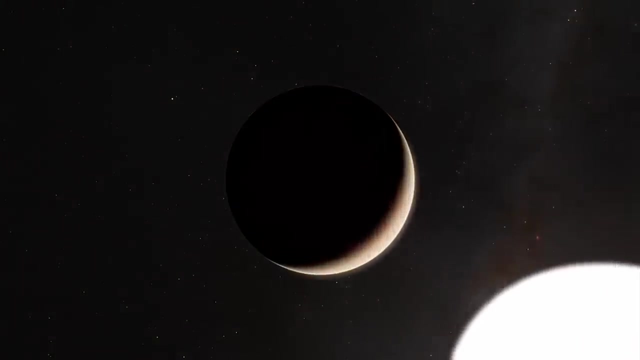 found on Earth. Such extreme temperatures are responsible for some truly exhausting and devastating effects: Exotic atmospheric chemistry and physics, including the possibility of vaporized metals and a completely obliterated molecular hydrogen, which is typically abundant in other gas giants' atmospheres, Another factor contributing to KELT-9b's. 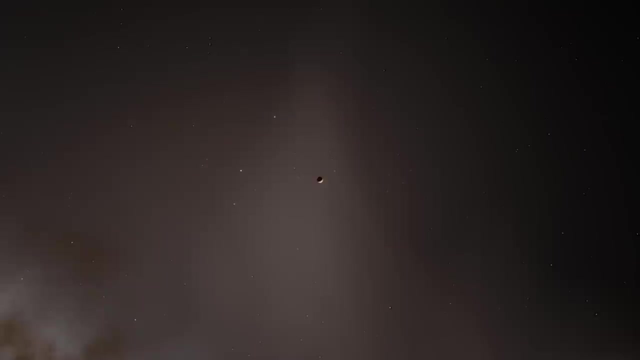 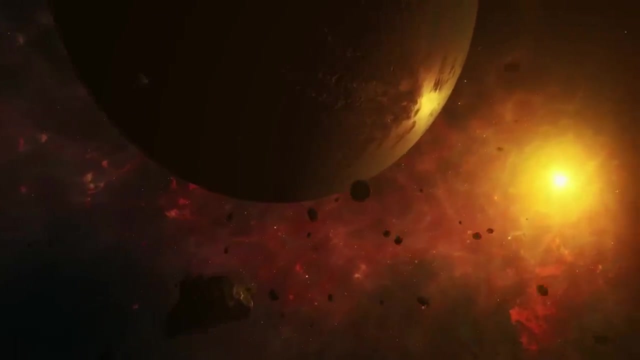 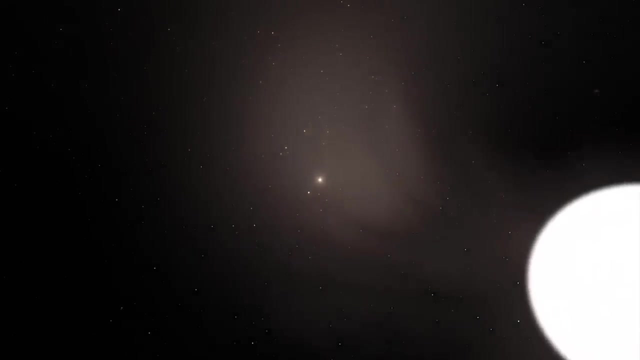 high temperatures is the lack of a significant reflective atmosphere. Planets that can reflect a portion of their star's light back into space can moderate their temperatures to some degree. However, the intense heat on KELT-9b likely prevents the formation of reflective clouds or ice, allowing the 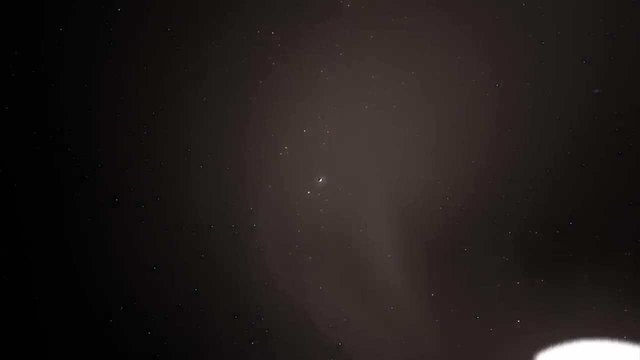 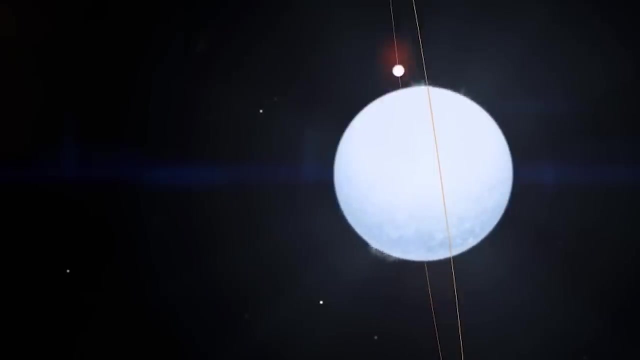 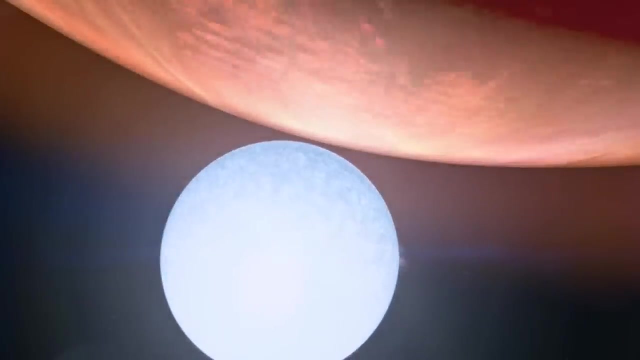 planet to absorb a maximum amount of stellar radiation. The planet's tidally locked nature, where one side always faces the star while the other remains in perpetual darkness, could exacerbate the temperature extremes, However, even with potential heat distribution by atmospheric winds. the day side of KELT-9b. 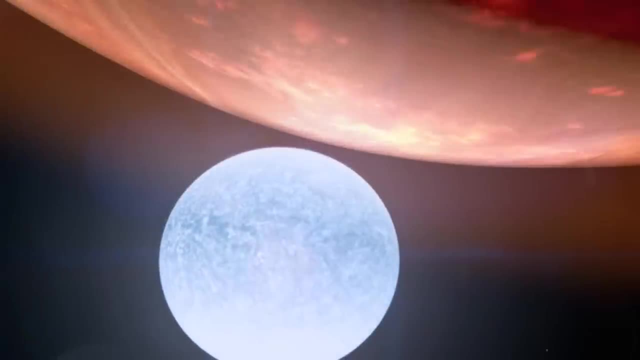 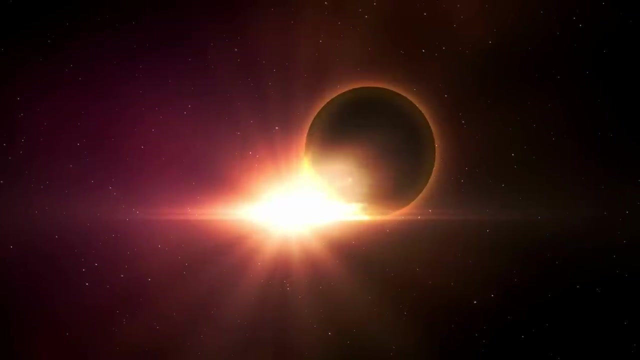 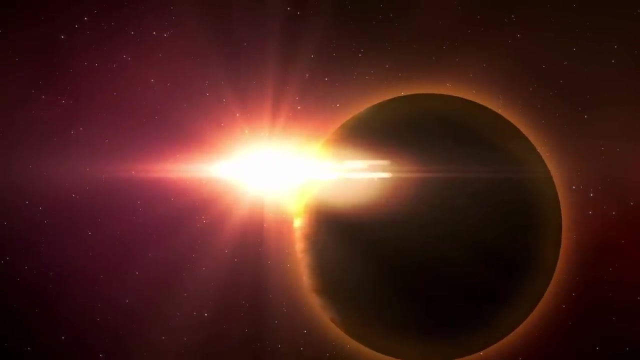 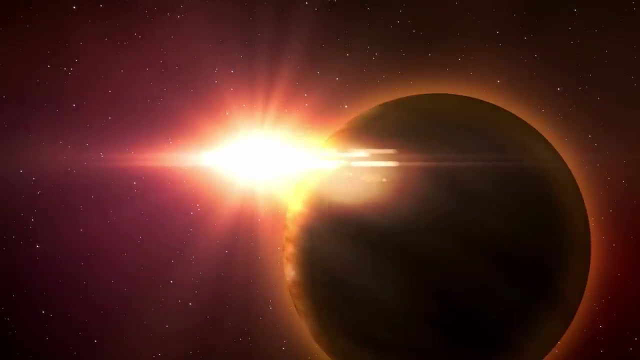 remains infernally hot, showcasing the extreme conditions of the planet's atmosphere For KELT-9b, the hottest known exoplanet. future observations aim to delve deeper into its extraordinary atmosphere and the extreme conditions resulting from its proximity to its host star, KELT-9.. Astronomers are particularly interested in utilizing the 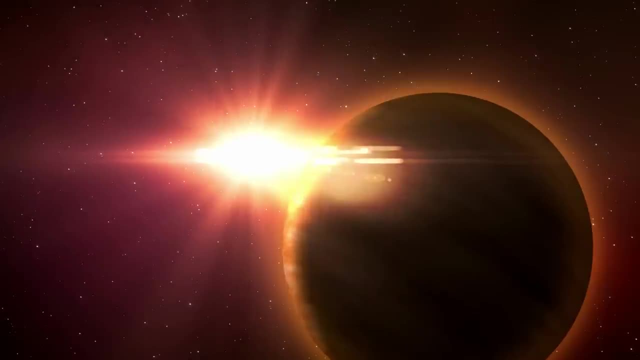 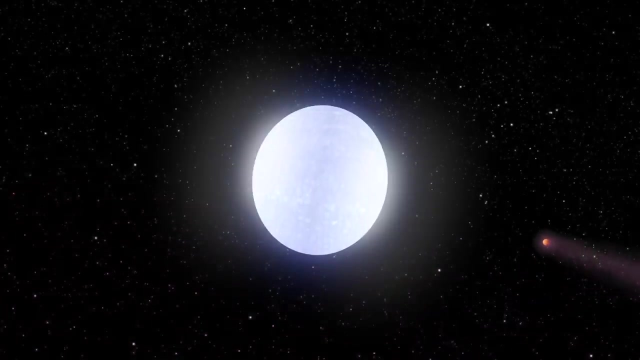 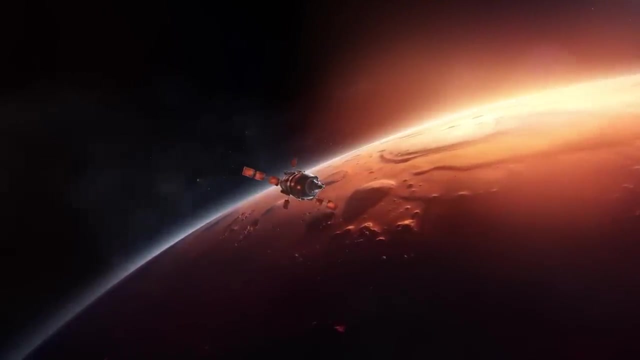 next generation of space- and ground-based telescopes to further explore this intriguing world. One of the primary goals is to study the atmospheric composition of KELT-9b in greater detail. This involves identifying the presence of exotic molecules and elements that can exist in vapor form due to the planet's high temperatures. 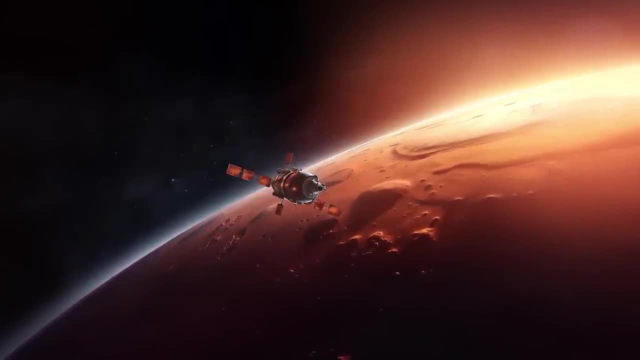 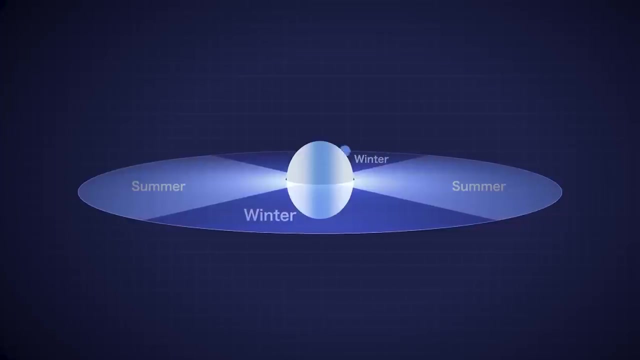 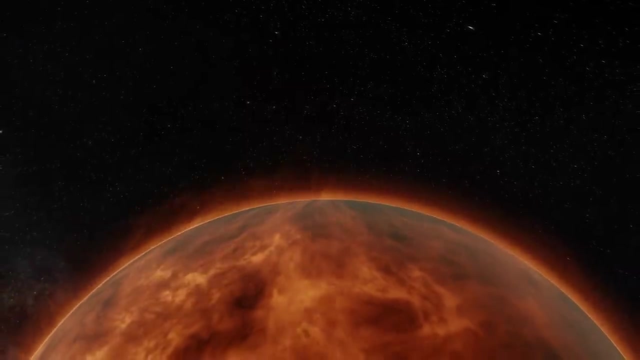 such as vaporized metals and possibly even molecules that are unknown or rare in cooler planetary atmospheres. Another focal point for future observations is the investigation of KELT-9b's atmospheric dynamics and weather patterns. Given the extreme temperatures differences between the planet's day side and night side, scientists are keen to understand. 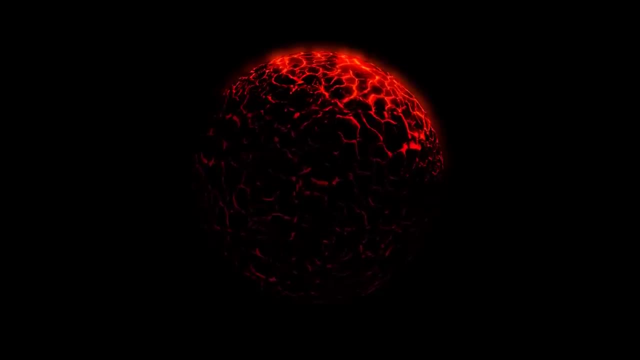 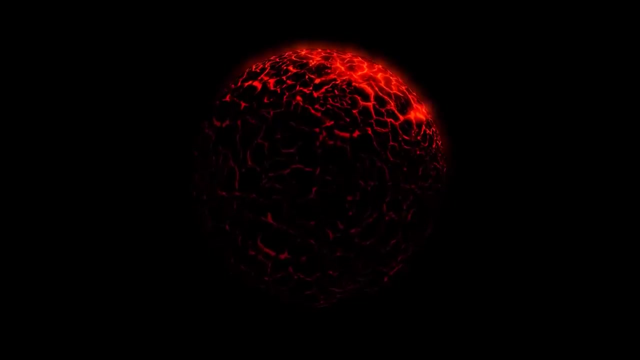 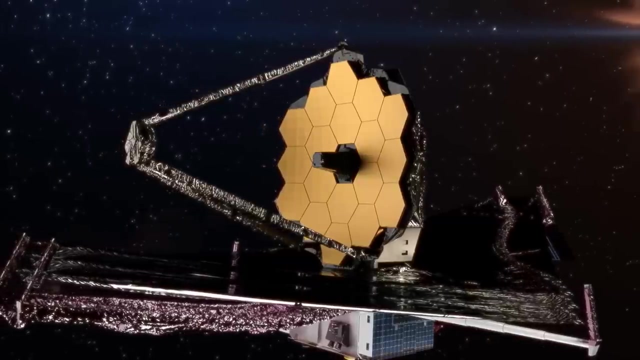 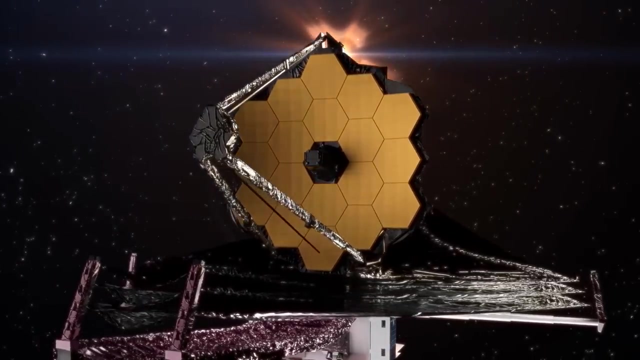 how heat is distributed across the planet. Scientists are keen to understand how heat is distributed across the planet. This could reveal insights into the potential for extreme weather phenomena. unlike anything seen in our solar system, Advanced telescopes like the James Webb Space Telescope and the Extremely Large Telescope are 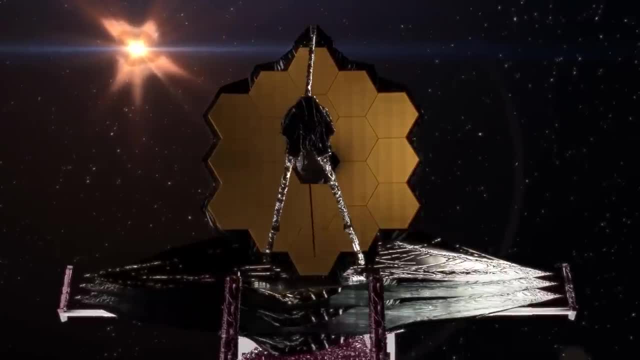 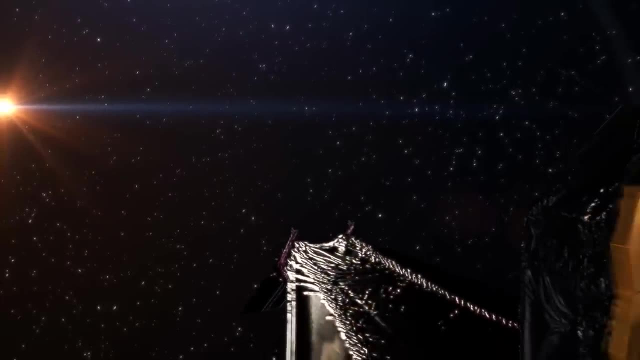 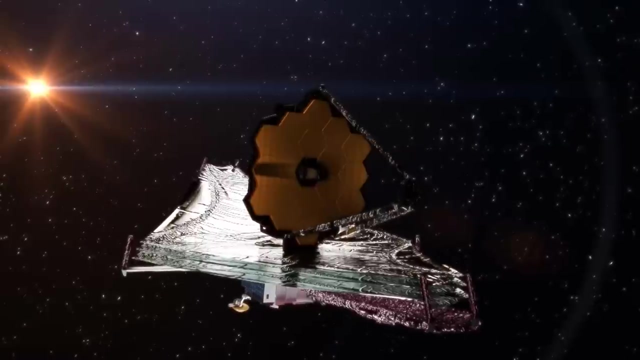 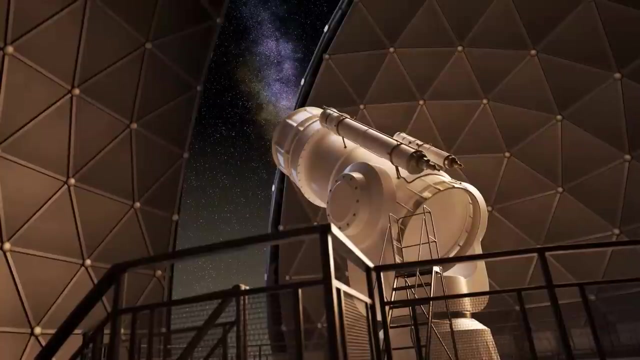 expected to play crucial roles in these observations. The JWST, with its unparalleled sensitivity to infrared light, will be able to detect the thermal emission from KELT-9b, providing detailed data on the planet's temperature distribution and atmospheric composition. The ELT, with its enormous mirror size, will offer unprecedented resolution, allowing astronomers 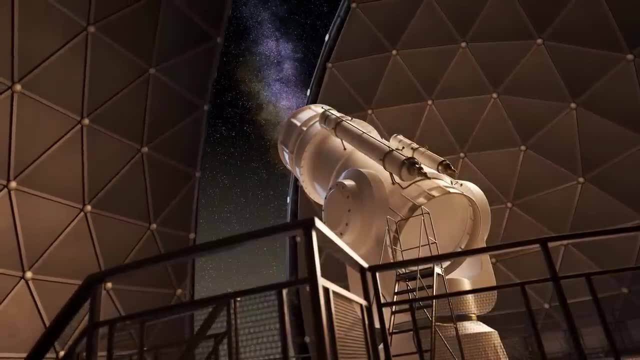 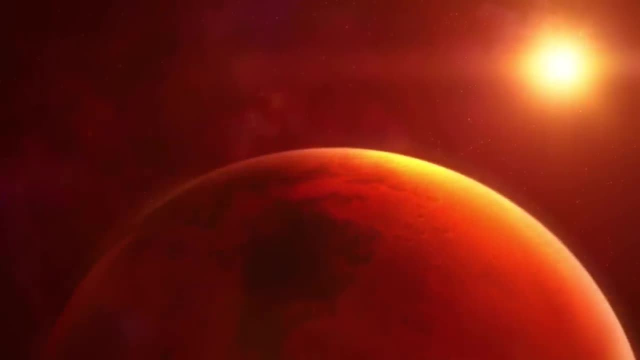 to study the atmospheric chemistry of KELT-9b with greater precision than ever before. Additionally, future observations will seek to understand the magnetic field of KELT-9b and its interaction with the stellar wind from KELT-9.. This interaction is crucial for 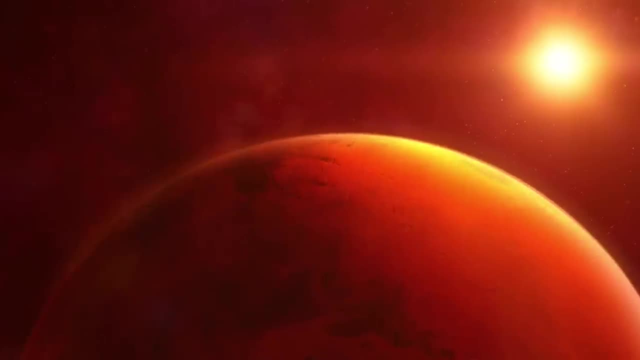 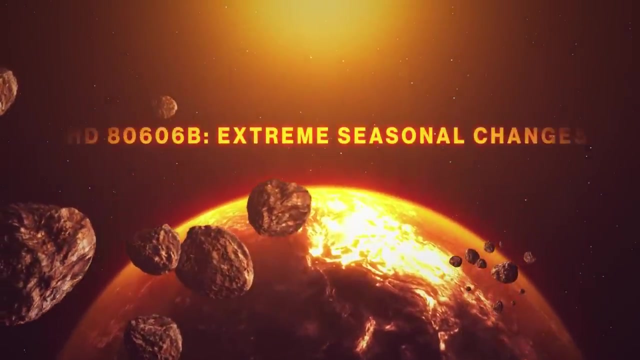 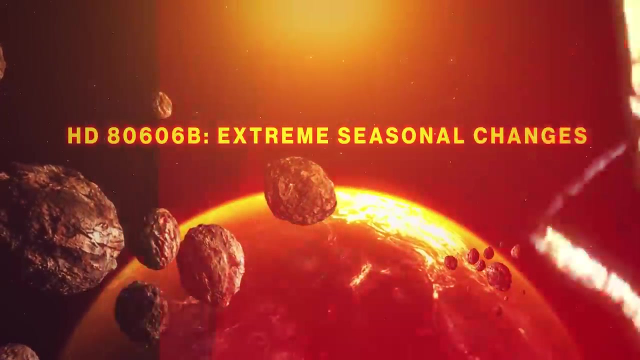 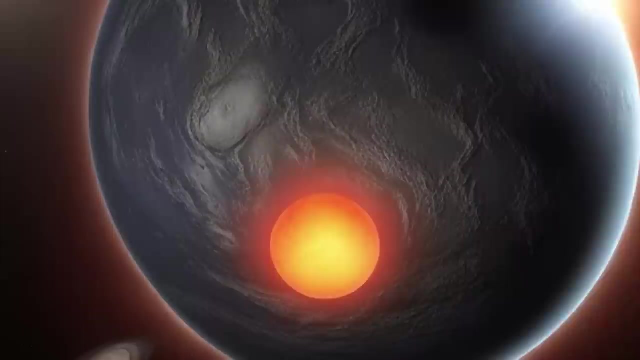 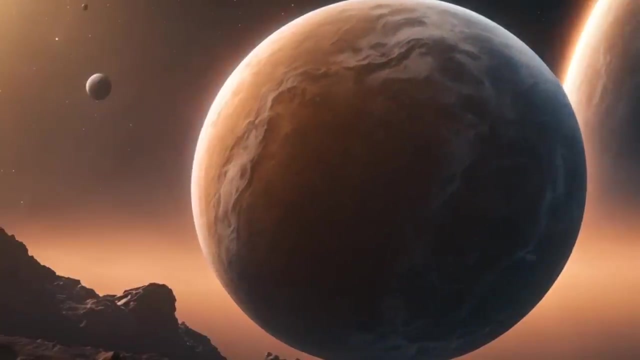 understanding the planet's atmospheric loss and how it affects the planet's long-term evolution and stability. The extreme seasonal changes on HD 80606b, a gas giant exoplanet located about 190 light years away in the constellation Ursa Major, are primarily caused by its highly eccentric 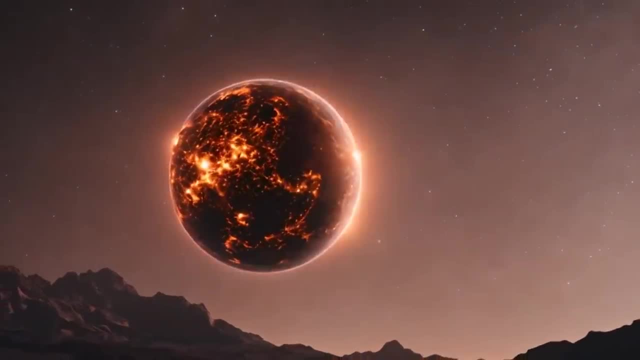 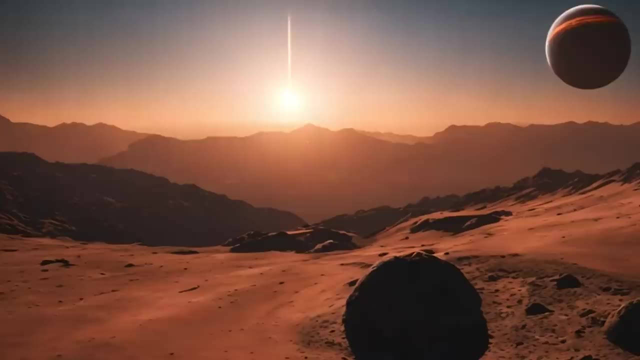 orbit around its host star. Unlike the nearly circular orbits of planets in our solar system, HD 80606b follows an elongated path that brings it extremely close to its star at perihelion. This is the first time that a solar system has ever been so close to its star at perihelion. 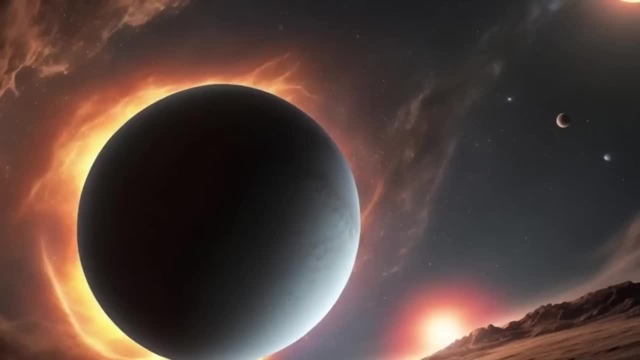 This is the first time that a solar system has ever been so close to its star, at perihelion. The first thing that happens when an orbiter reaches a perihelion is to reach perihastron, the closest point in its orbit, and then takes it far away at a pastron, the farthest point. 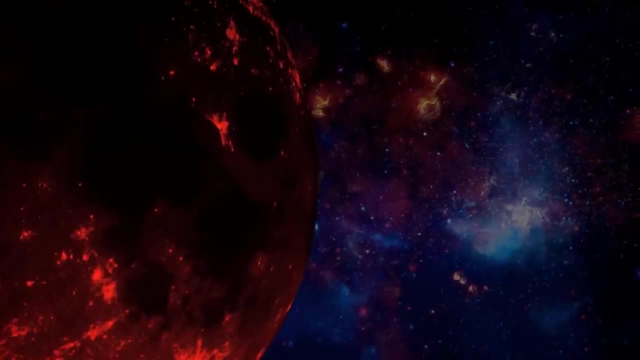 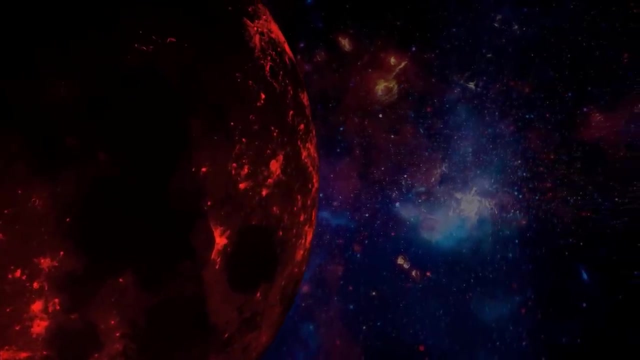 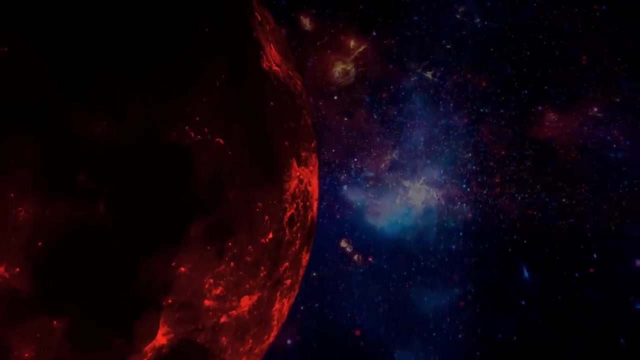 in its orbit. This unique orbital characteristic leads to dramatic variations in temperature and weather conditions on the planet over its orbit, which lasts about 111 days, As HD 80606b approaches its perihastron, it experiences a rapid increase in temperature. 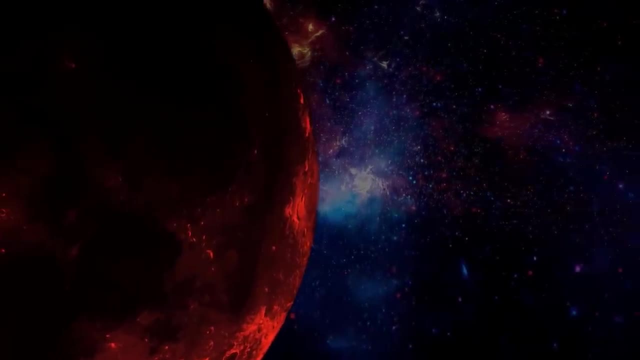 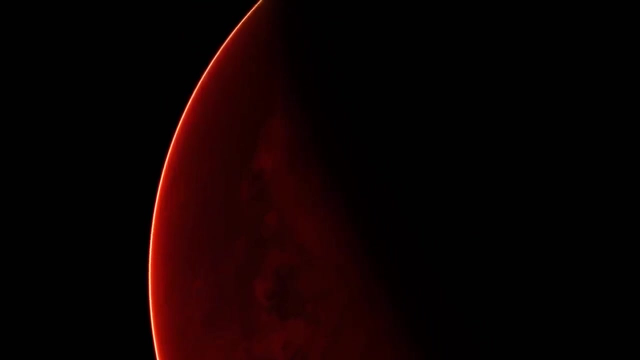 due to the intense solar radiation radiation from its nearby star. This can cause the planet's atmosphere to heat up by hundreds of degrees in just a few hours, a phenomenon that is unparalleled in our solar system. The sudden increase in temperature is believed to drive extreme weather events. 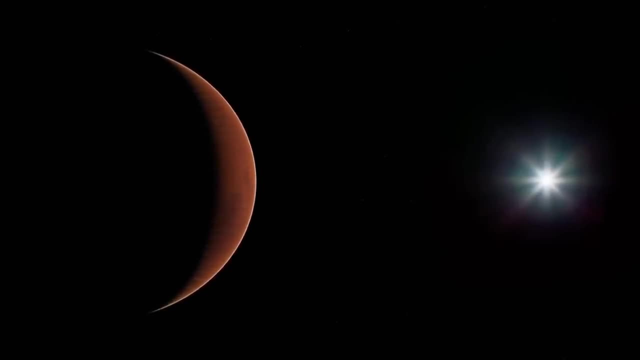 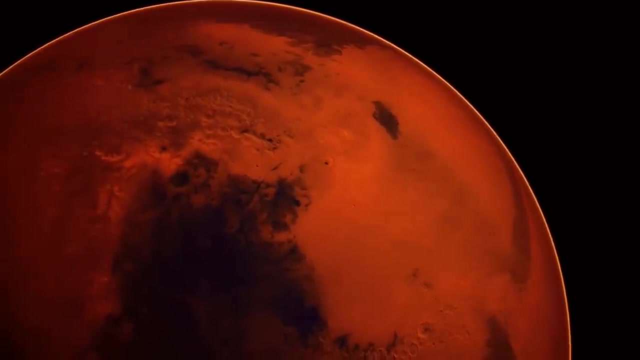 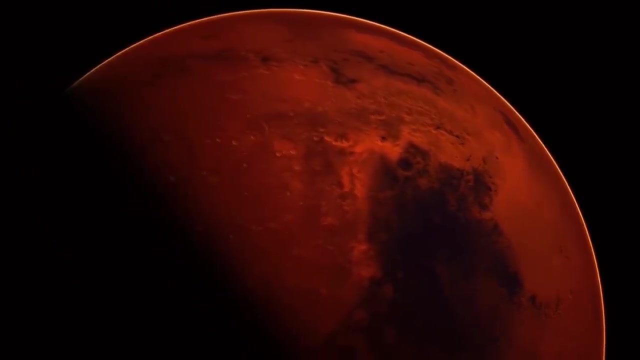 such as supersonic winds and storm systems that can span the entire planet. These conditions are a stark contrast to the much cooler and calmer weather experienced when the planet is at a far from the star. The extent of these seasonal changes is further influenced by the planet's 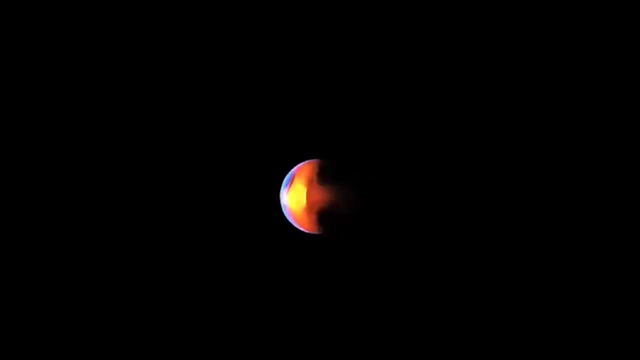 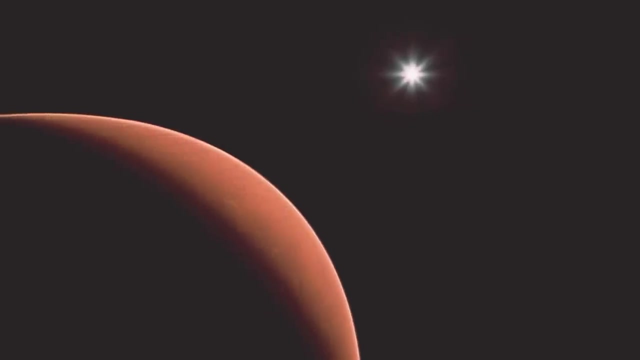 rotation and the angle of its orbital tilt. If HD 80606b is tidally locked, with one side always facing the star, the temperature contrast between its day side and night side would be even more pronounced. However, even if the planet rotates, the rapid heating and cooling as it moves along 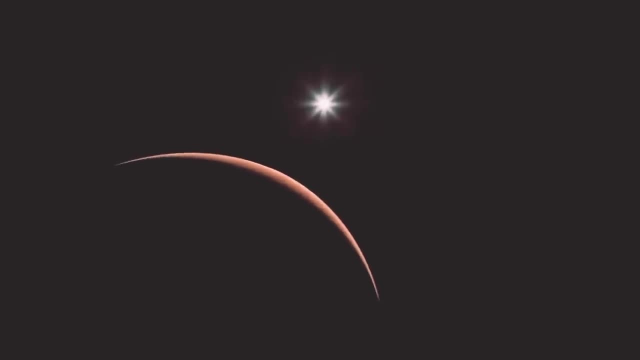 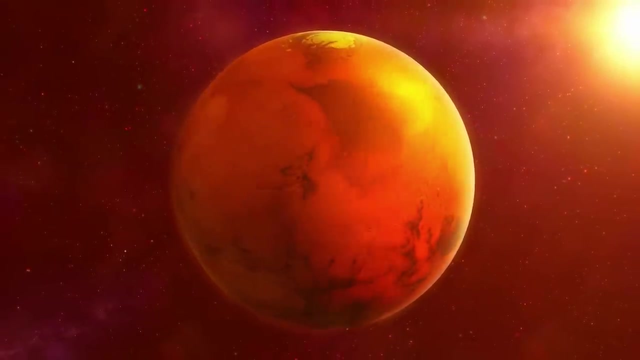 its eccentric orbit will be even more pronounced. The rapid heating and cooling as it moves along its eccentric orbit would still result in significant seasonal shifts. Astronomers study these extreme seasonal changes using various methods, including transit observations when the planet passes in front of its star from our perspective, 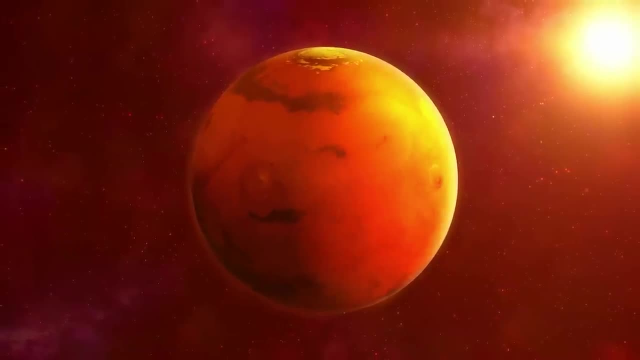 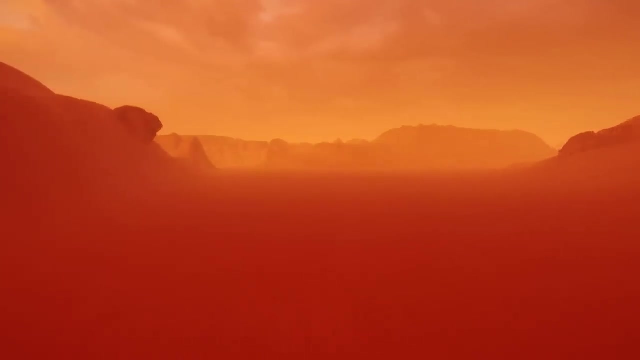 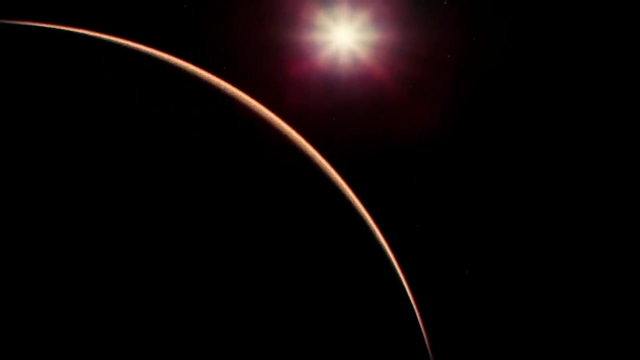 and radial velocity measurements that track the star's motion in response to the planet's gravitational pull. These observations help scientists understand the dynamics of HD 80,000.. 606 b's atmosphere and the effects of its eccentric orbit on its climate. the extreme seasonal changes on hd 80 606 b, driven by its highly eccentric orbit, have significant implications for the planet's potential for habitability. the intense fluctuations in temperature and weather conditions, ranging from scorching heat to relatively cooler periods, create an environment that is challenging for the development and sustainability of life as we understand it. the rapid increase in temperature when the planet approaches its 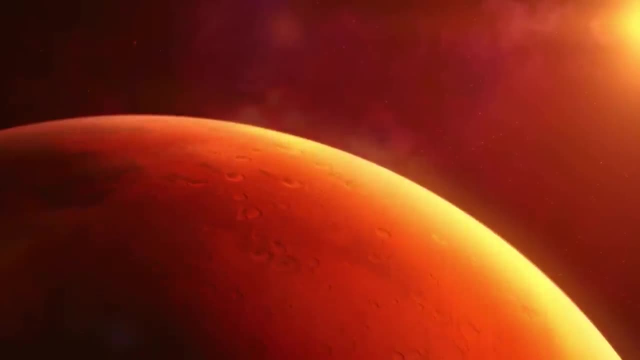 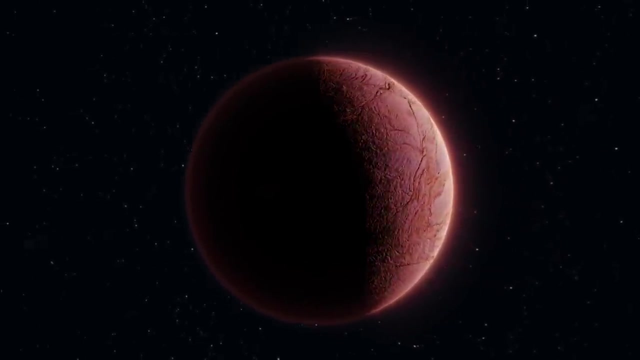 periastron can cause the atmosphere to heat up by hundreds of degrees in just a few hours, leading to harsh conditions unlikely to support life. the concept of habitability usually involves a stable environment where liquid water can exist on the planet's surface, a condition believed to be. 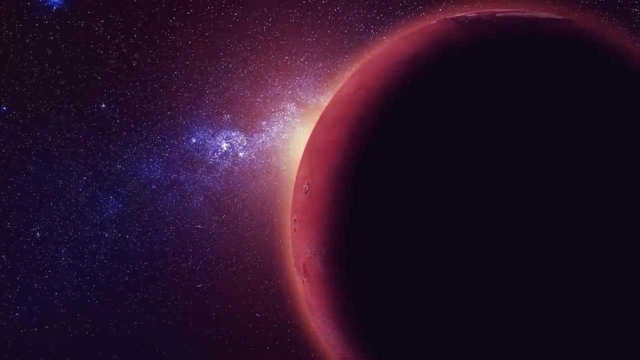 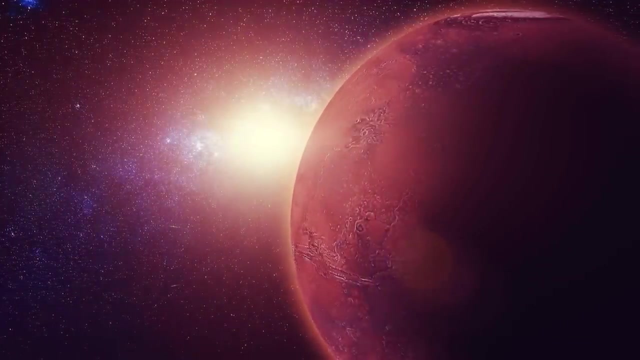 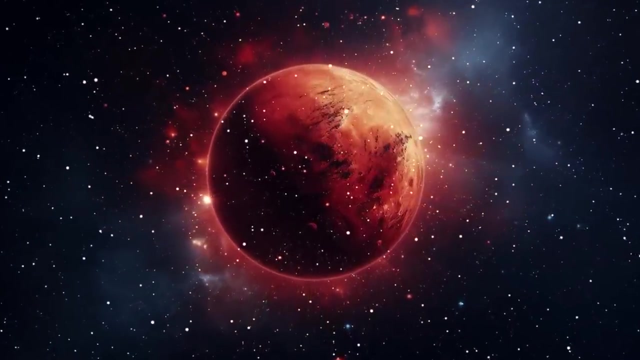 necessary for life. however, the drastic temperature changes on hd 80 606 b would make it difficult for liquid water to maintain a stable presence. during the planet's close approach to its star, any surface water would likely vaporize due to the extreme heat, while at the farthest points in its orbit, any remaining water could freeze. 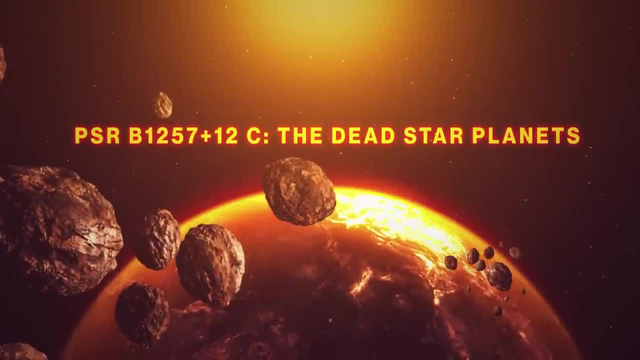 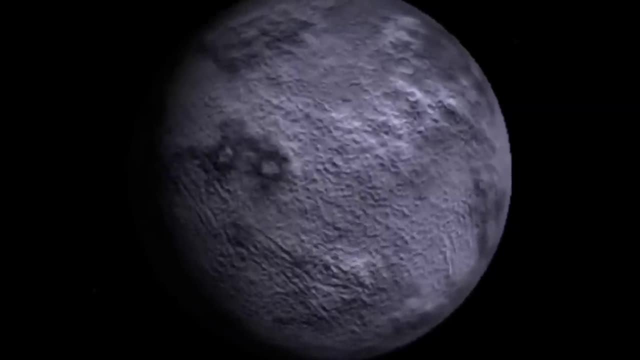 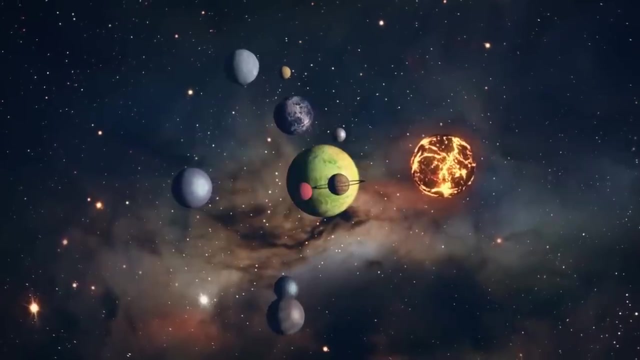 the planet's orbit and the pulsar psrb 1257 plus 12 represent one of the most intriguing and unexpected discoveries in the field of astronomy, challenging our understanding of where and how planets can form. pulsars are highly magnetized, rotating neutron stars that emit beams of 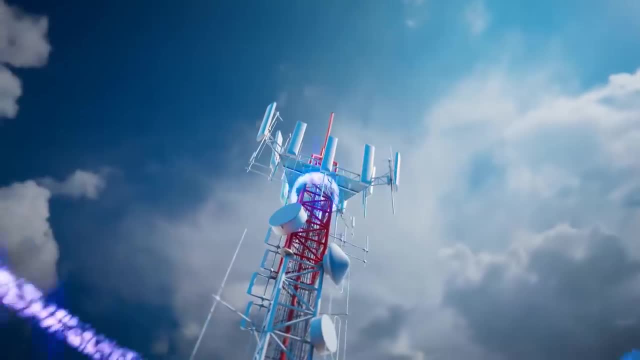 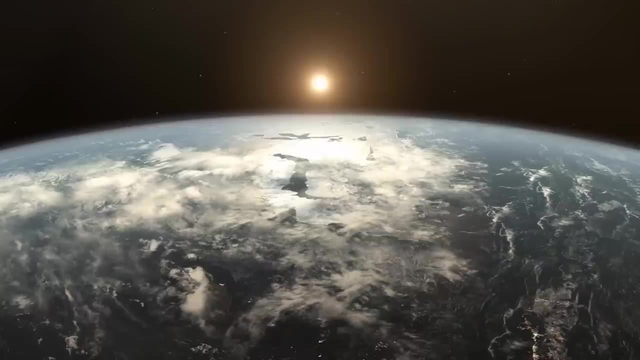 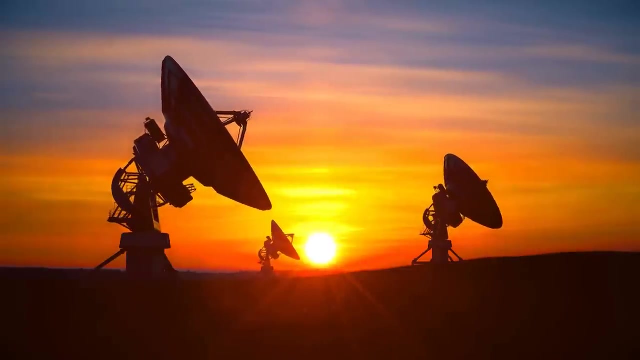 electromagnetic radiation out of their magnetic poles. as these neutron stars are highly magnetized, they can also be used to generate electromagnetic radiation. the pulsar psrb 1257 plus 12 is a pulsar approximately 2300 light years away from earth in the constellation of virgo- was groundbreaking because it demonstrated for the first time that planets could exist in environments vastly different from the solar system. the pulsar psrb 1257 plus 12 was first discovered in the solar system in the early 19th century and was the first to have a pulsar pulsar that could rotate around the earth. 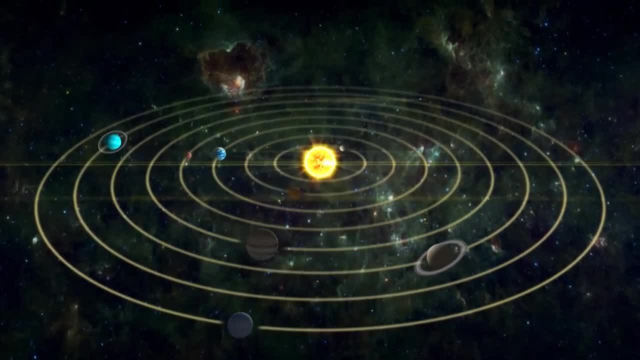 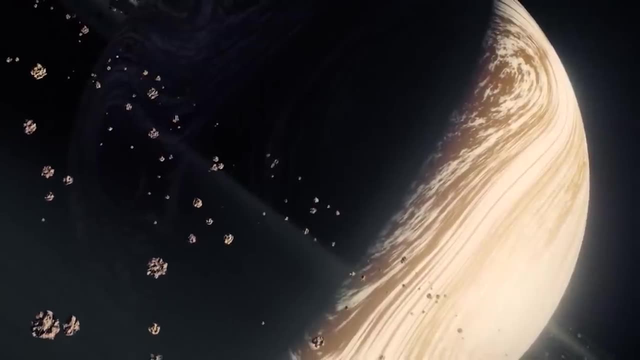 the pulsar psrb 1257 plus 12 is the first to have a pulsar pulsar. pulsar, pulsar, pulsar, pulsar. what makes these planets unique is not just their existence around a pulsar, but the conditions under which they exist. pulses are the remnants of massive stars that exploded. 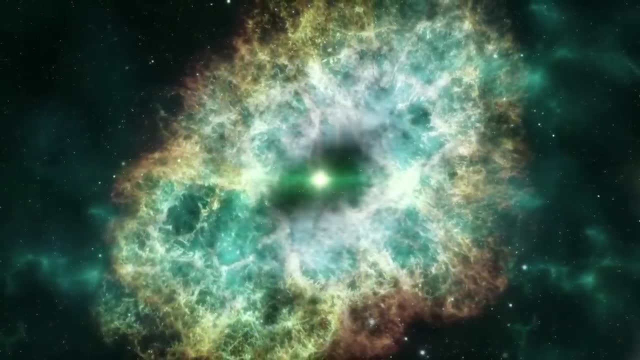 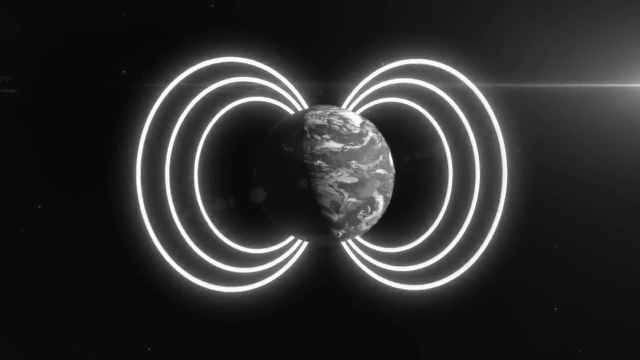 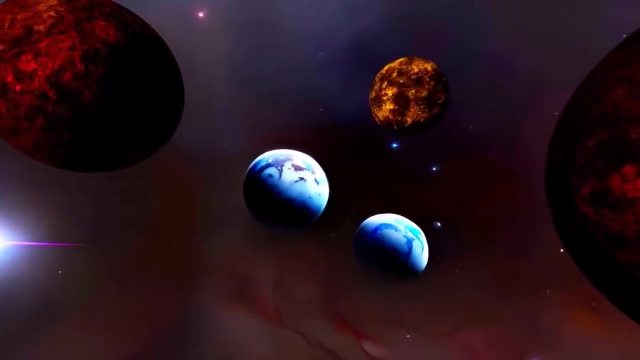 in supernovae, leaving behind a core so dense that atoms are crushed, leaving a sea of neutrons. the environment around a pulsar is extremely harsh, with intense magnetic fields and radiation levels that would be inhospitable to life as we know it. the presence of planets in such a setting? 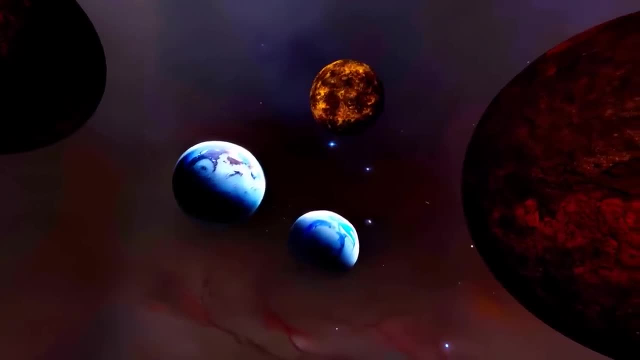 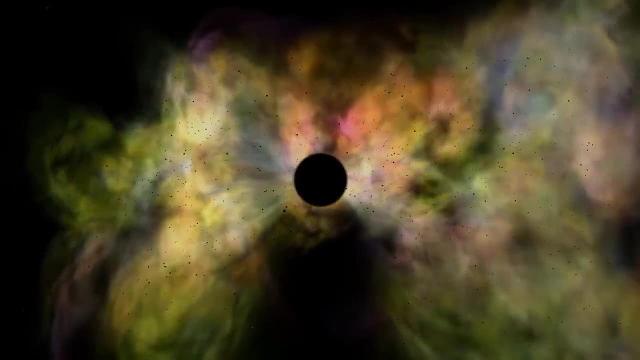 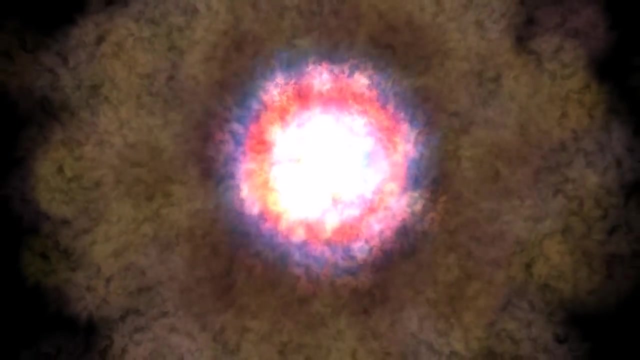 raises fascinating questions about their formation and survival. traditional theories of planet formation, which involve the accretion of dust and gas in a protoplanetary disk around a young star, do not easily apply to the environment around a neutron star, which should have been cleared of such material by the star's supernova explosion. 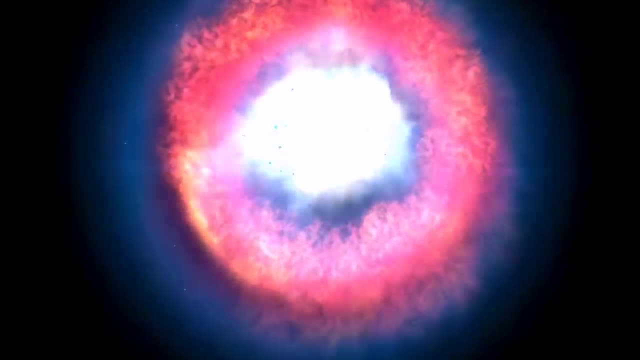 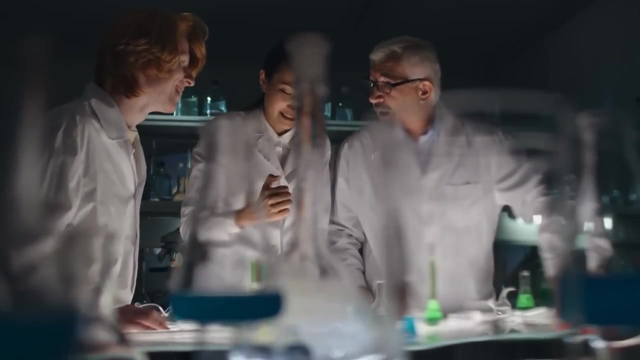 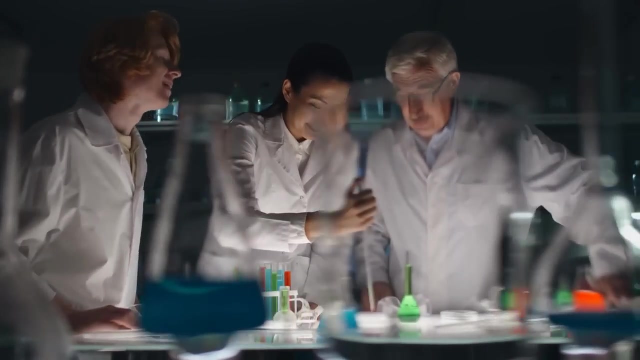 the planets orbiting. psrb 1257 plus 12 discovered in the early 1990s include several terrestrial mass bodies and their detection was a milestone in the field of exoplanetary science. their discovery was made through precise measurements of the pulsar's. 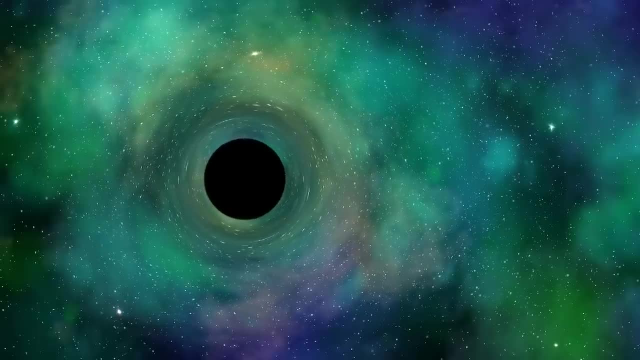 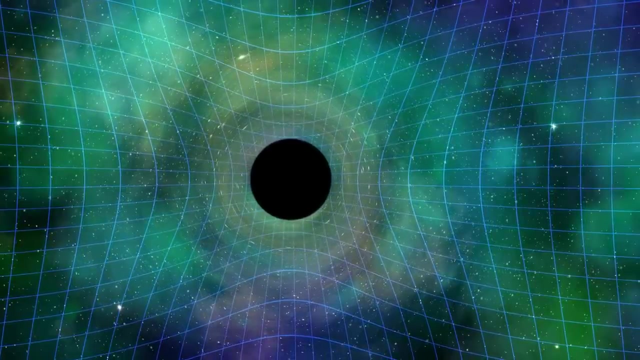 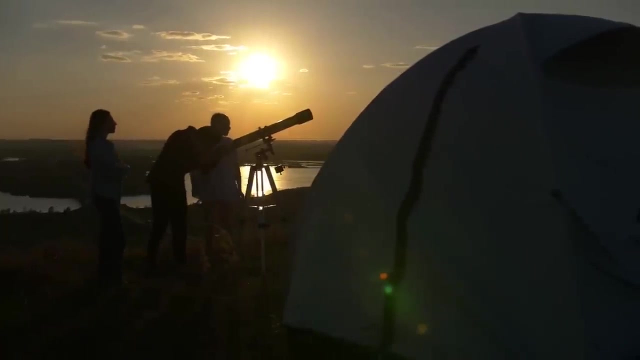 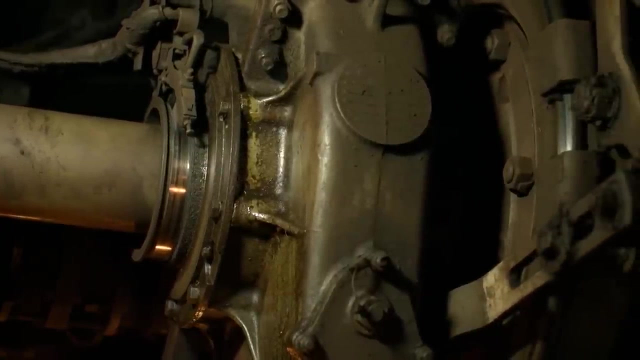 pulse timing. as planets orbit a pulsar, they cause it to wobble slightly due to their gravitational pull, leading to tiny but measurable variations in the timing of its pulses. this method of detection is unique to pulsar planets and showcases the diversity of techniques astronomers use to uncover exoplanets. another remarkable aspect of these pulsar planets is their potential. 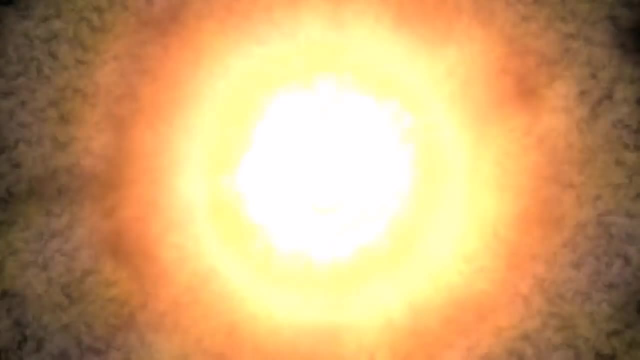 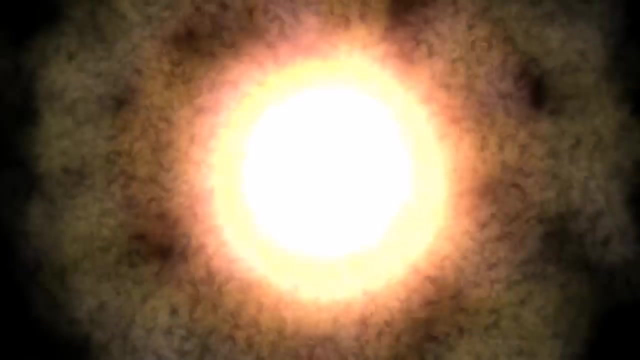 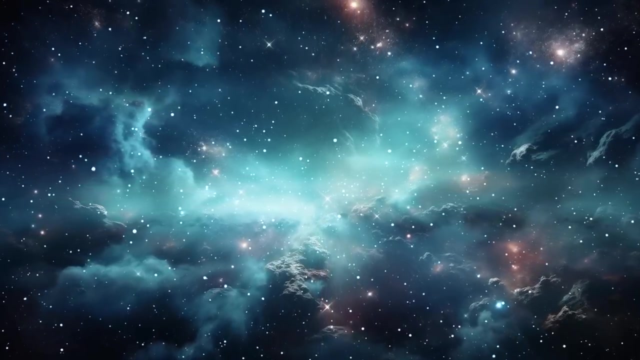 formation mechanisms. one theory suggests that these planets could have formed from the debris left over from the supernova that created the pulsar, representing a second generation of planet formation. alternatively, they might have been existing bodies captured by the pulsar's gravity, or remnants of a star system that survived the supernova explosion. 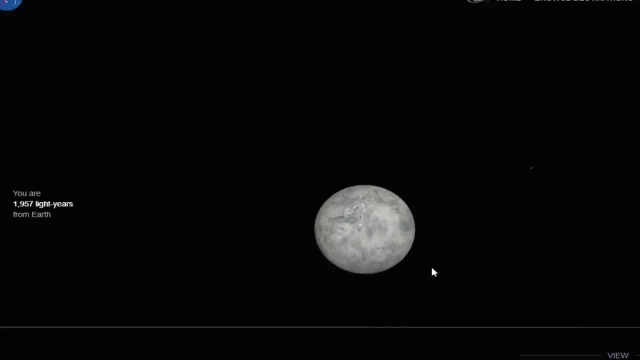 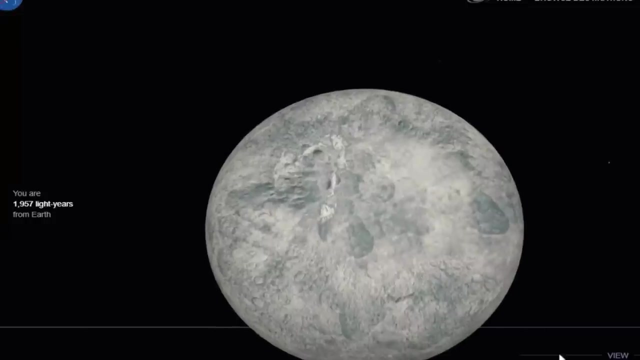 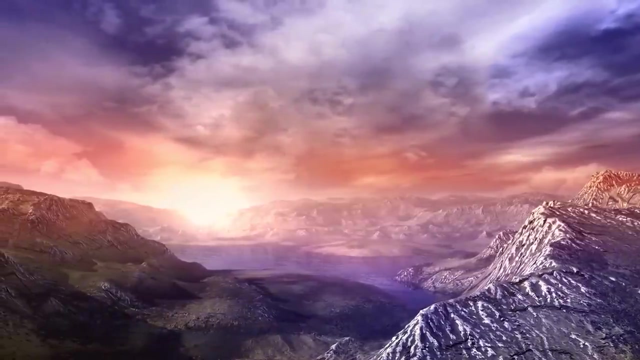 all things considered, the discovery of planets orbiting psrb 1257 plus 12 opened up a new avenue of exoplanet research, showing that planets could form in or survive extreme conditions and environments previously thought to be uninhabitable. the conditions on the planets: orbiting the pulsar psrb 1257 plus 12 are starkly different from the original ations of these planets. the time claim as follows: after the discovery of the planets orbiting the pulsar psrb 1257 plus 12 opened up a new avenue of exoplanet research, 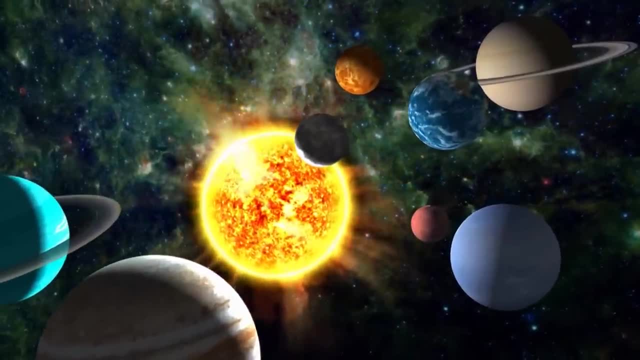 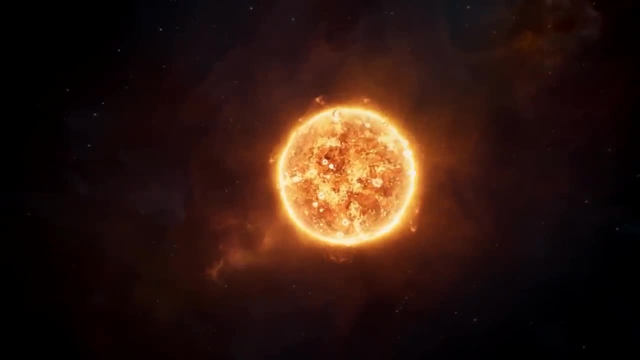 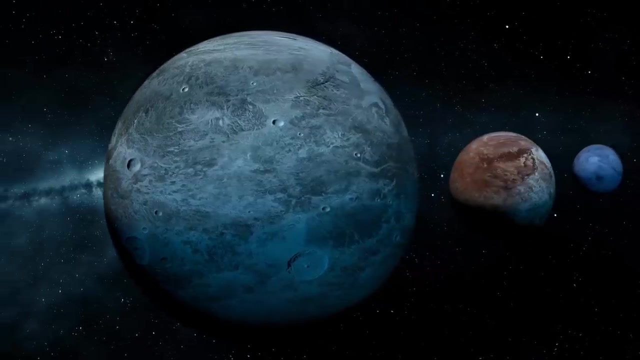 those on planets within our solar system, presenting an environment that is almost beyond comparison. Our solar system's planets orbit a stable main-sequence star, the Sun, which provides a relatively consistent source of light and heat, crucial for maintaining the conditions that 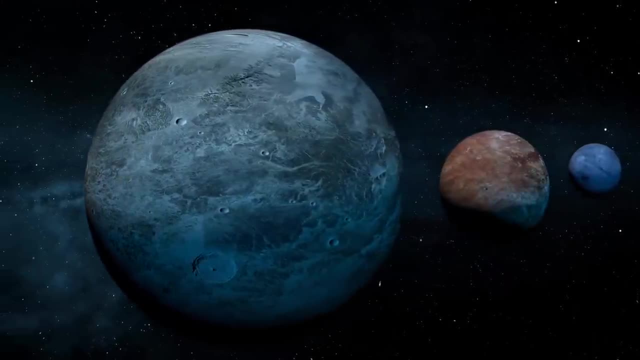 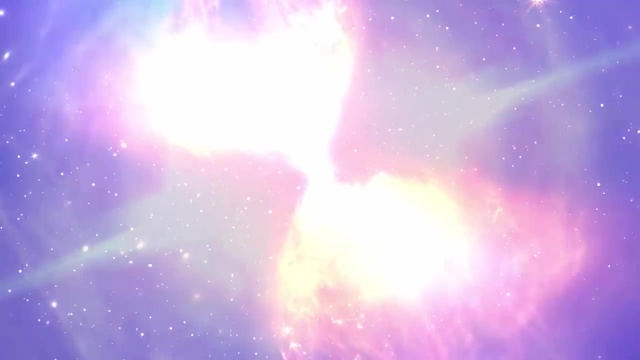 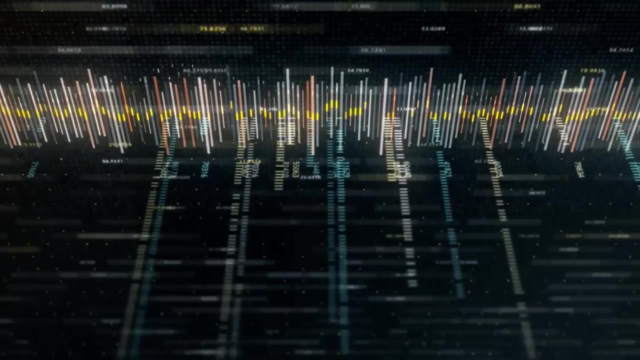 support life on Earth and influencing the climate and atmospheric dynamics on other planets. In contrast, the planets around PSR B-1257-12 orbit a pulsar, an extremely dense remnant of a supernova explosion which emits intense electromagnetic radiation and has powerful 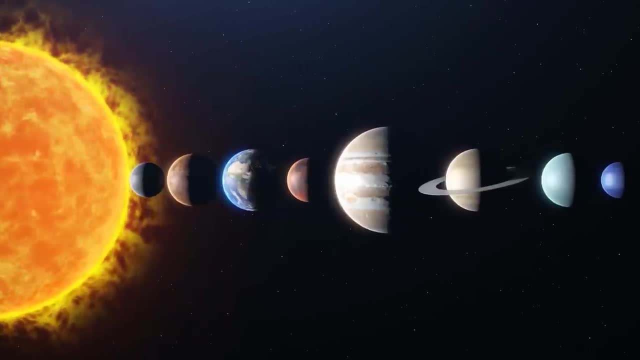 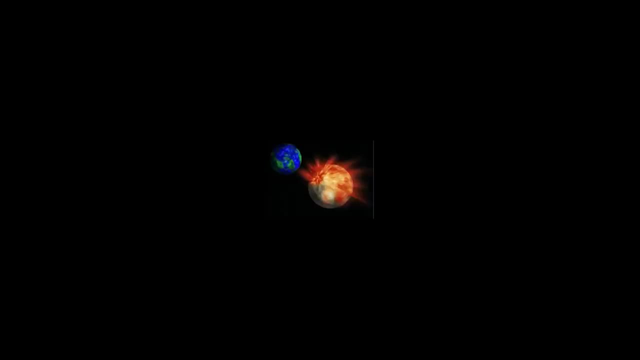 magnetic fields. The radiation environment around a pulsar is incredibly harsh compared to the sunlight that bathes our solar system. Pulsar radiation can strip away atmospheres, irradiate surfaces and cause a lot of damage. The pulsar radiation can strip away atmospheres, irradiate. 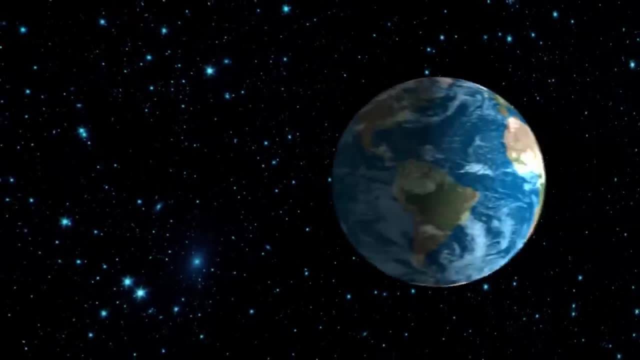 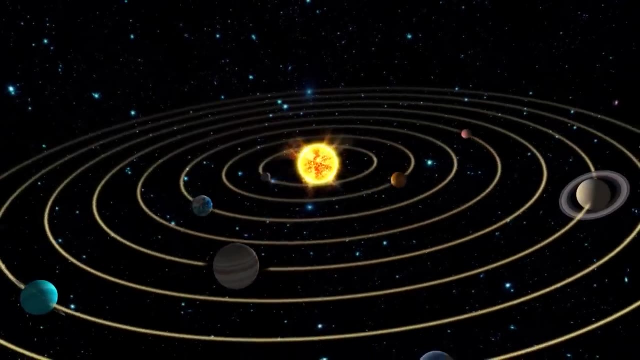 surfaces and potentially sterilize planets, making them inhospitable for life as we know it. In our solar system, planets like Earth have magnetic fields that protect them from solar wind and cosmic rays, preserving their atmospheres and enabling them to host life. 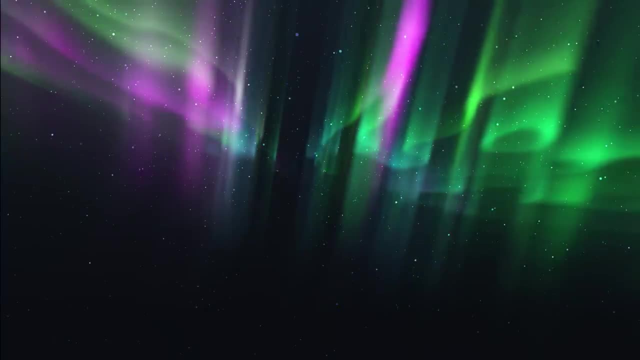 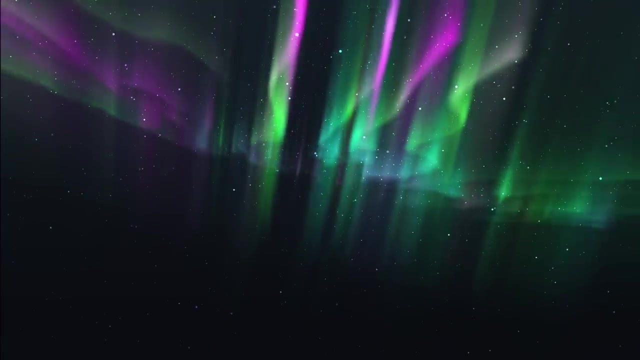 The planets around PSR B-1257-12,, however, are exposed to the pulsar's radiation with little to no protection, suggesting that any atmosphere that is exposed to the pulsar's radiation will cause a lot of damage. The pulsar radiation can strip away atmospheres, irradiate surfaces and 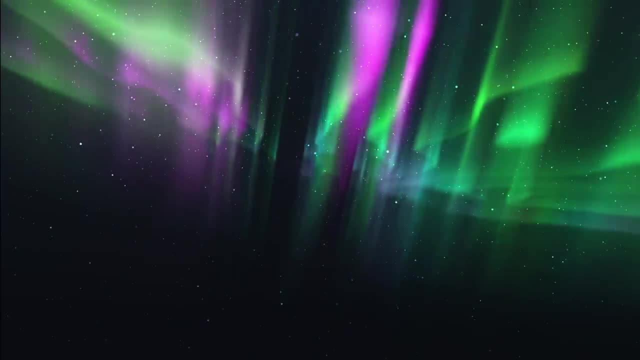 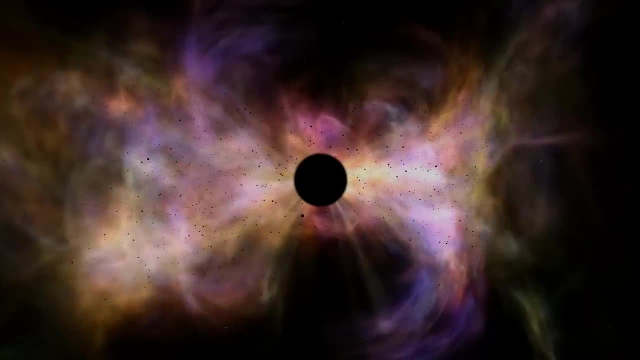 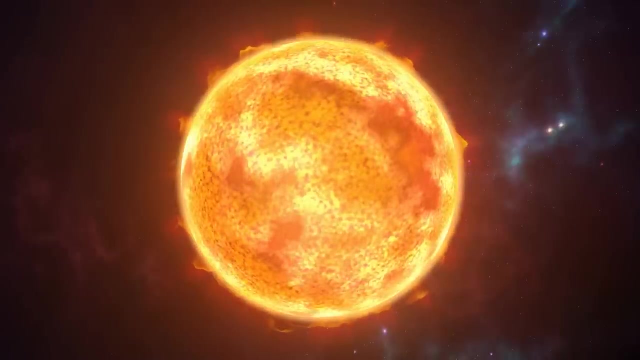 because it's essential that other planet subsides in and outside the sagen lamb� subsides in and outside the say song will make change in the way we talk about the transfer of light into light, what either people consider and special light of anything we think we have. 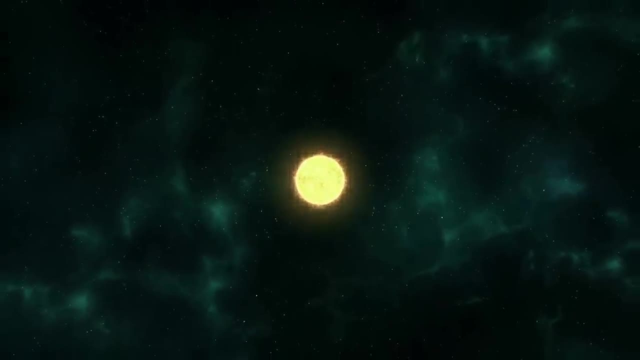 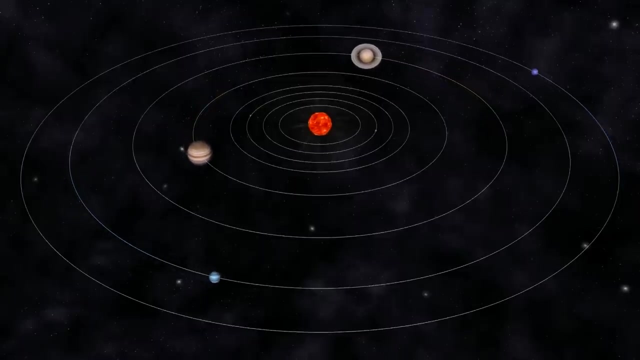 mestad compulsoris f. Antonin. Perhaps this share is more important than route of the supernova that gave birth to the pulsar. This suggests a second generation of planet formation, potentially involving different materials and processes than those that created the planets in our solar system. 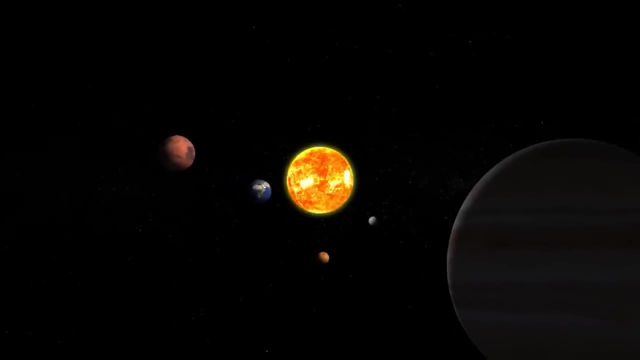 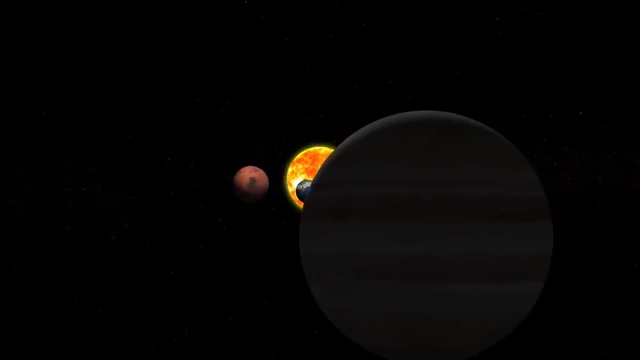 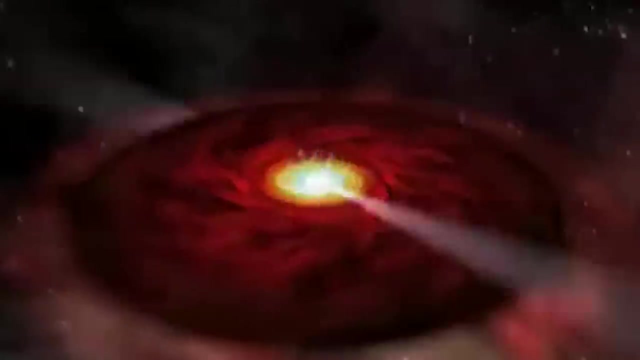 Temperature conditions also present a stark contrast. Whereas our solar system planets experience temperatures that can support liquid water on Earth and ice on the outer planets, the planets orbiting PSRB 1257 plus 12 are likely subject to extreme temperature variations, depending on their distance from the pulsar and the intensity of its emissions. 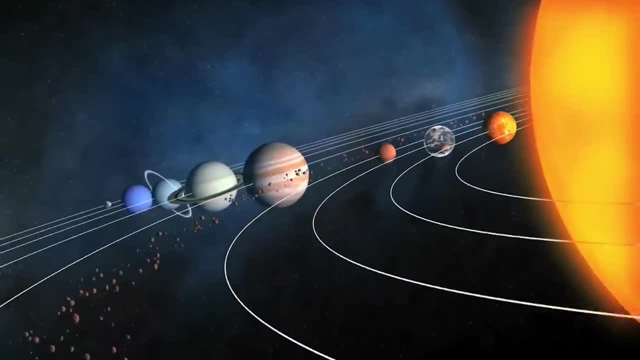 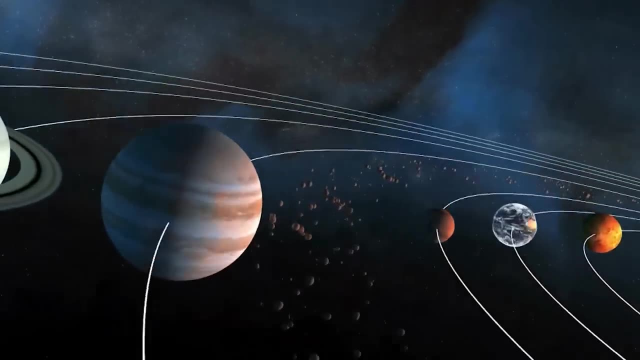 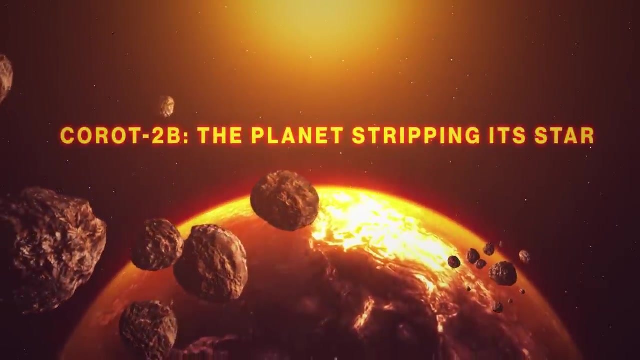 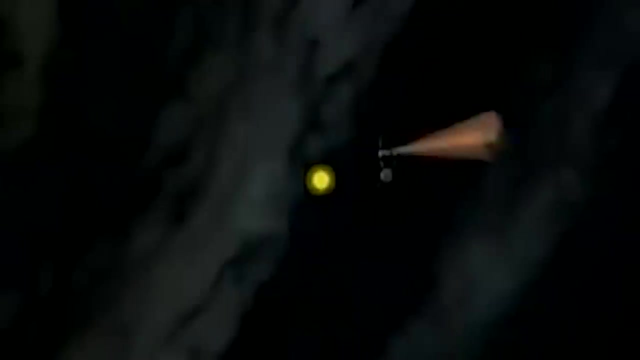 These conditions are far removed from the relatively stable environments found in our solar system, where the Sun's energy allows for a range of climates and atmospheric conditions. Corot 2B. Corot 2B, an exoplanet discovered by the Convection Rotation and Planetary Transits. 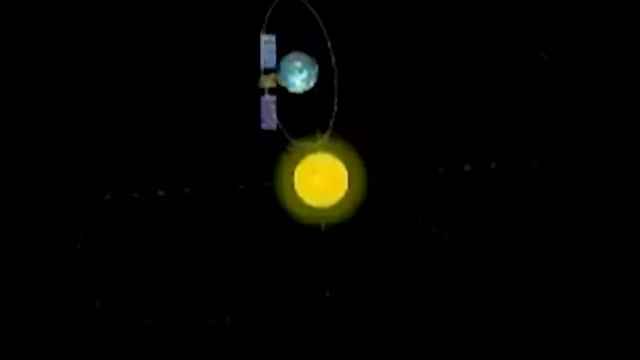 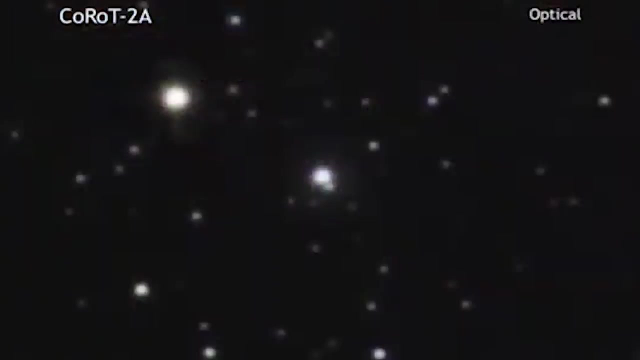 Corot space mission presents a fascinating case of a planet impacting its host star in a way that's observable from Earth, Orbiting its host star, Corot 2A, every 1.7 days. Corot 2B is a hot Jupiter. 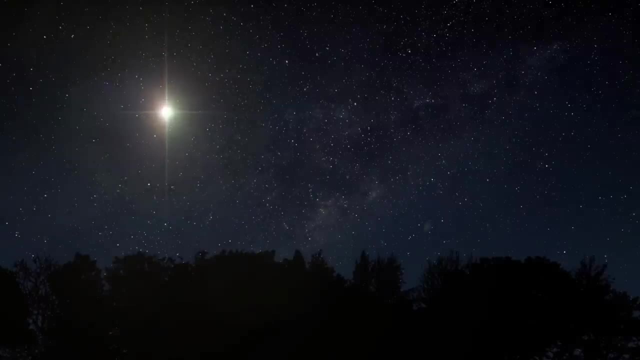 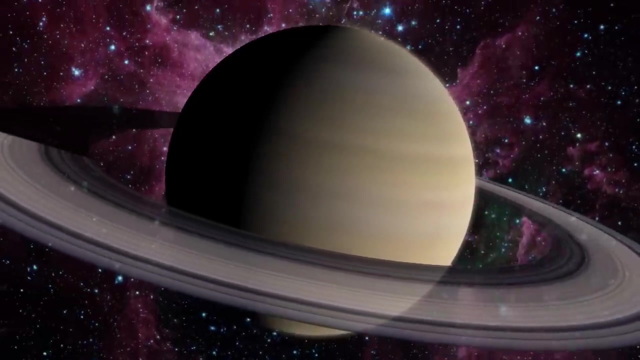 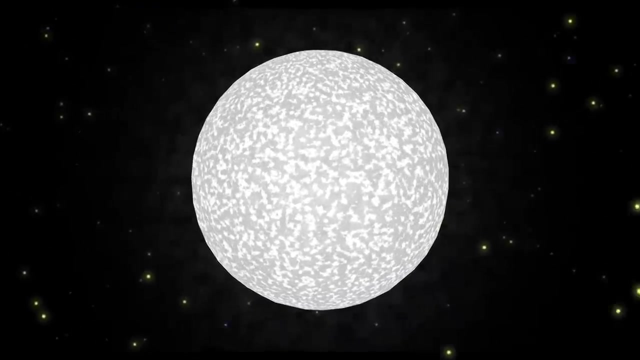 a type of gas giant that orbits very close to its star. This proximity leads to several significant effects on the star itself, showcasing the dynamic interactions that can occur between a star and its planets. One of the most striking impacts of Corot 2B on its host star. 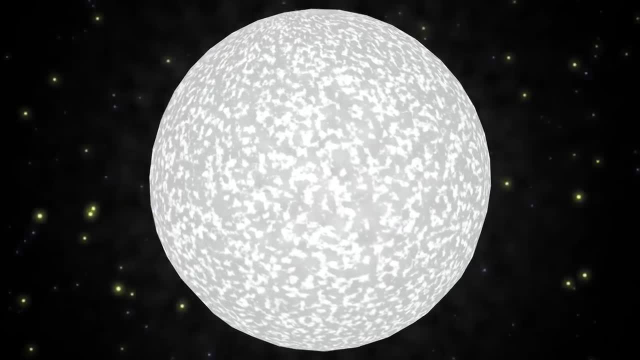 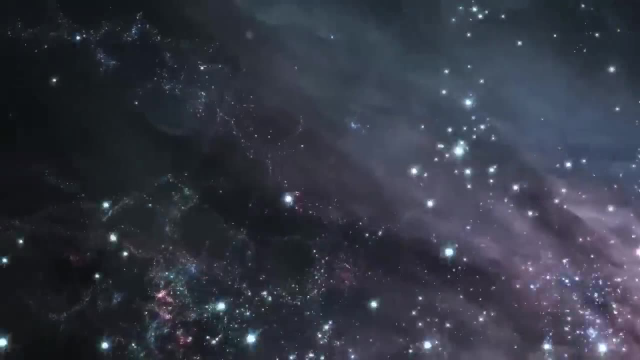 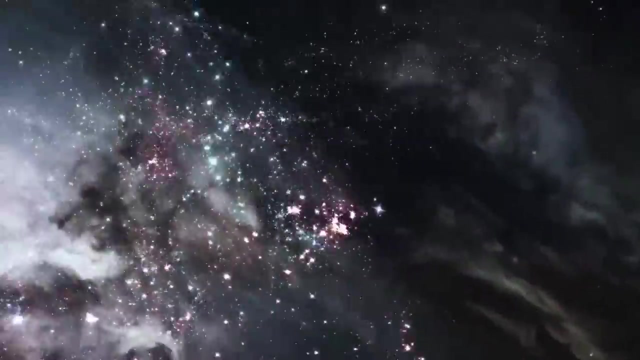 is the phenomenon known as star-planet interaction. The intense gravitational pull of Corot 2B can induce activity in the star's outer layers, potentially leading to increased magnetic activity, including star spots and flares. These effects are somewhat analogous to the way the Moon influences Earth's tides. 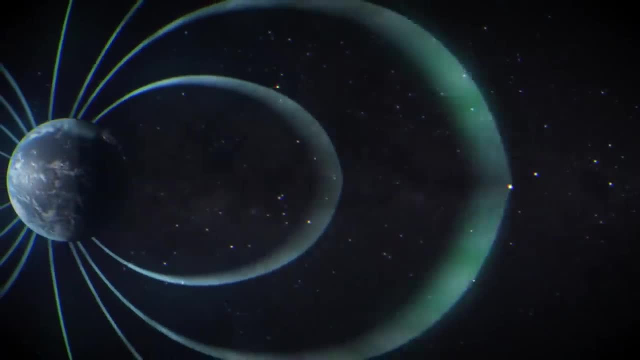 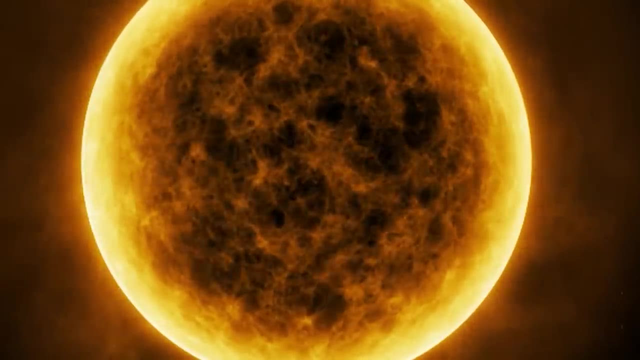 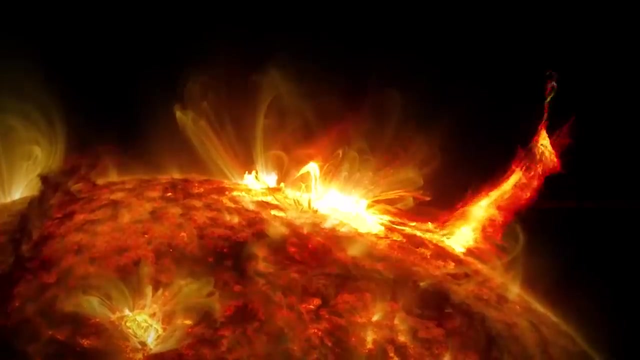 but on a much larger scale and involving magnetic fields and stellar plasma. Corot 2B's close proximity to its host star subjects it to tremendous stellar radiation, which heats the planet's atmosphere to extreme temperatures. This heating can cause the planet's atmosphere to expand and, in some cases, to escape into space. 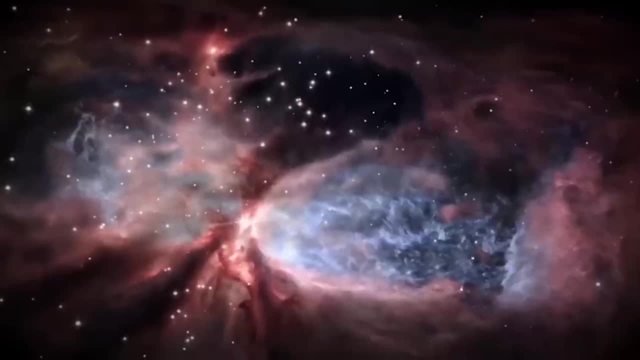 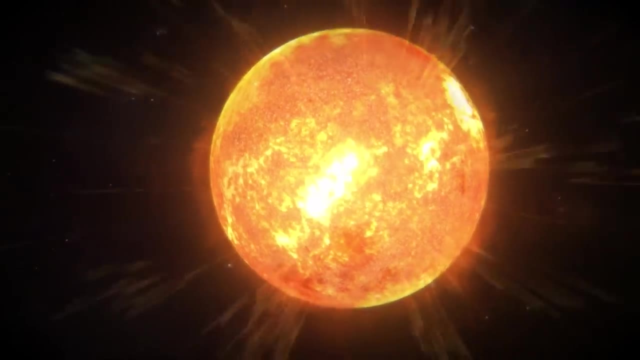 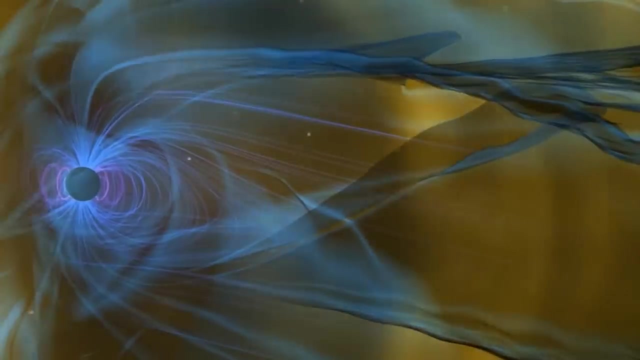 As the atmosphere bleeds off, it forms a cloud of material around the planet that can interact with the star. This interaction may lead to a transfer of angular momentum from the planet to the star, affecting the star's rotation rate and magnetic field. Another intriguing aspect of the Corot 2 system is the potential for the planet to induce chemical 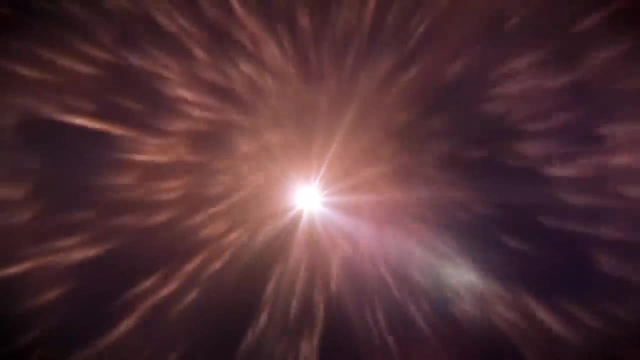 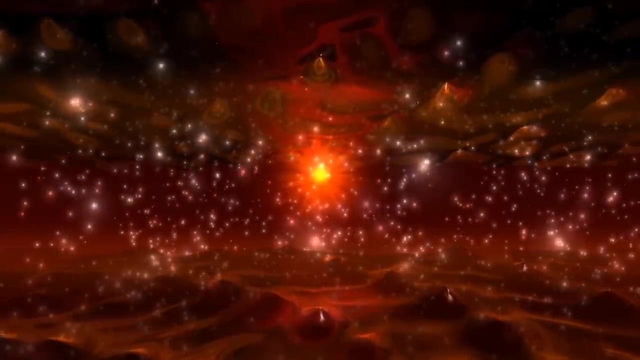 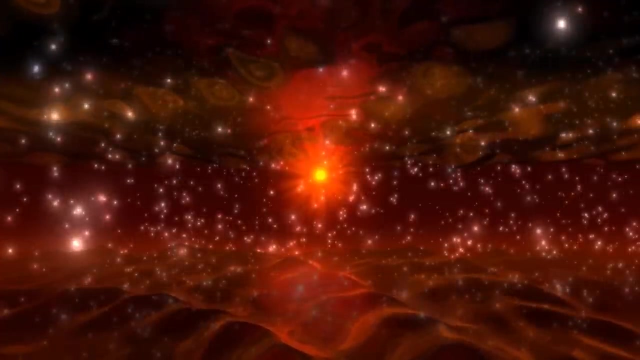 changes in the host star's outer layers, The material lost from the planet's atmosphere could fall into the star, altering its chemical composition and spectral signature. This process, known as accretion, can provide astronomers with clues about the composition of the planet's atmosphere, based on changes observed in the star's spectrum. 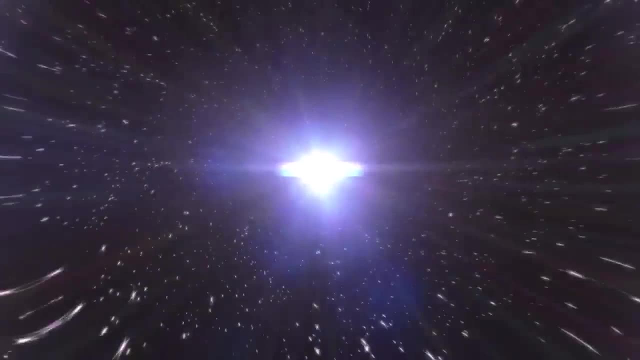 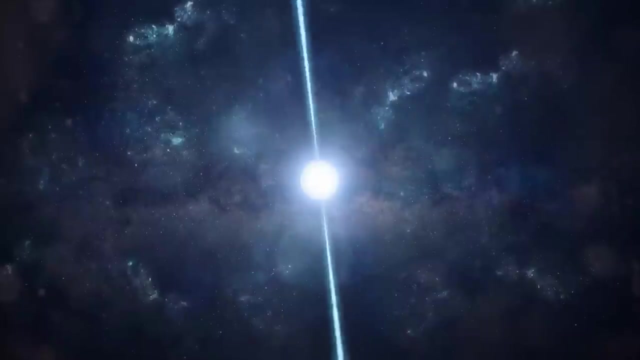 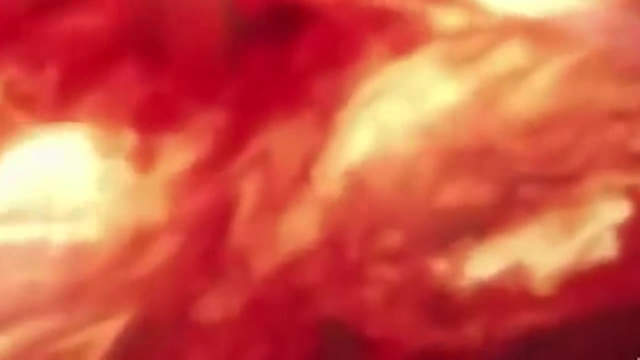 Astronomers study these interactions using various methods, including spectroscopy, which analyzes the star's light to identify chemical compositions and changes in brightness and magnetic activity. Observations of the Corot 2 system contribute to our understanding of how planets can affect their host stars, offering insights into the evolution of planetary systems. 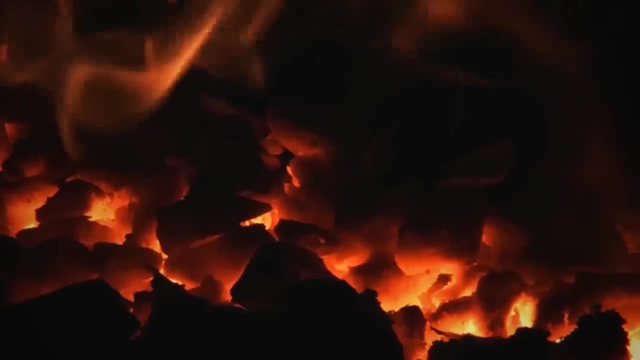 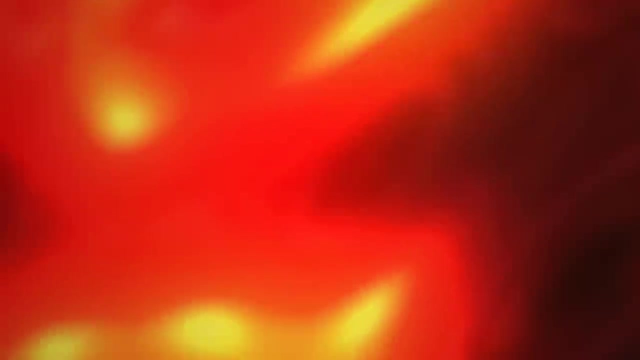 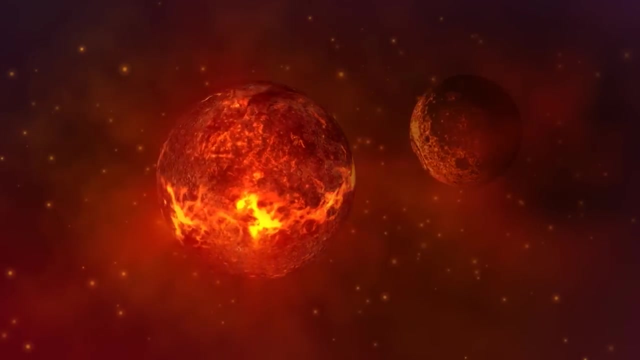 and the complex dynamics that govern their behaviour. The interaction between Corot 2b and its host star Corot 2a sheds light on the complex and dynamic relationships that can exist between stars and their planets, expanding our understanding of the cosmic ballet played out across the universe. These interactions reveal that planets 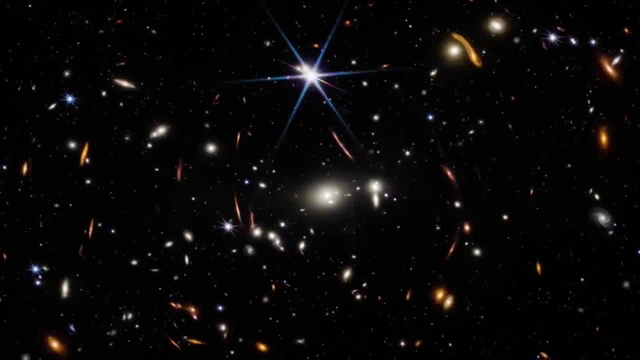 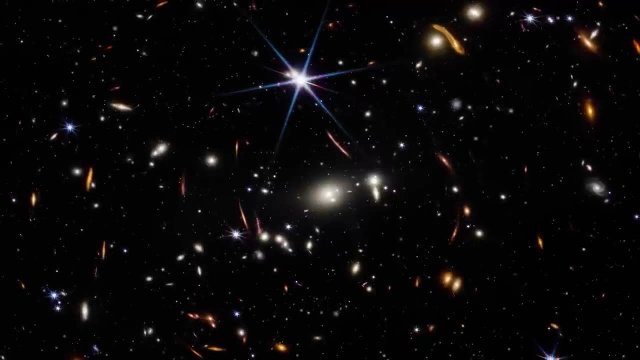 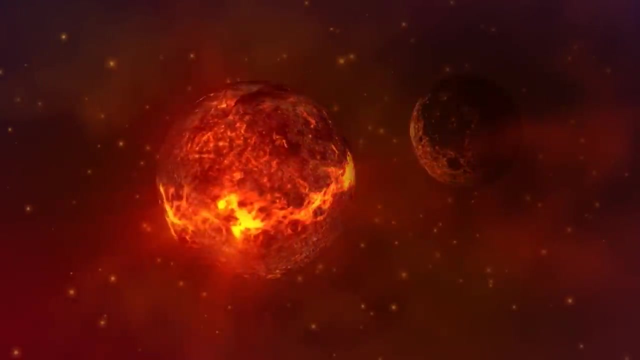 especially those in close orbits, like hot Jupiters, can have a profound impact on their stars, influencing their magnetic activity, rotation rates and even chemical compositions. This dynamic is a stark contrast to the previously held view that stars solely dictate the conditions of their orbiting planets, without any reciprocal effects. The phenomenon of star-planet- 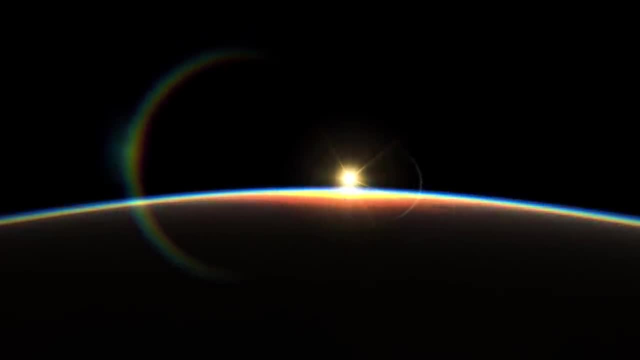 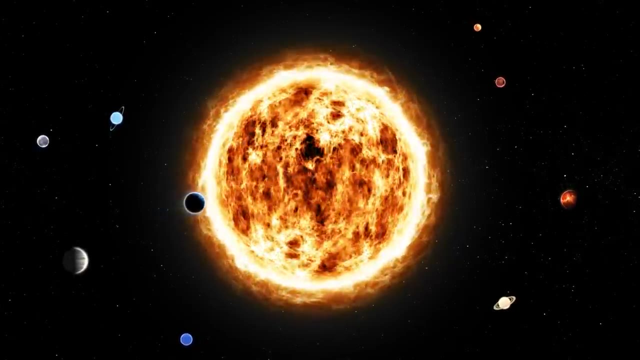 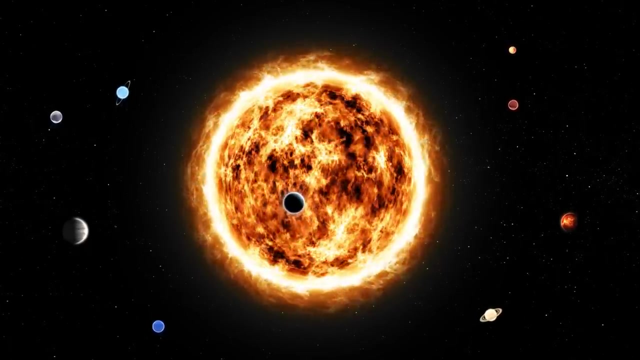 interaction exemplified by the Corot 2 system suggests that planets can induce magnetic disturbances in their host stars, leading to increased stellar activity, such as flares and spots. This is particularly significant because it implies that the presence and properties of planets can directly affect the stellar environment, altering the conditions under 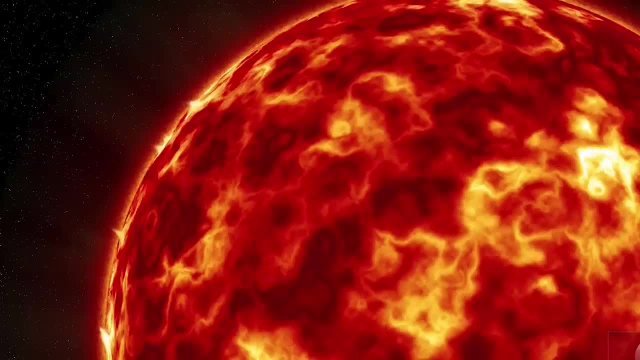 which these celestial bodies exist and evolve. In the case of Corot 2b, the close proximity to its host star and the resultant gravitational forces showcase how a planet's influence can extend beyond its own atmosphere, affecting the star it orbits. These interactions highlight: 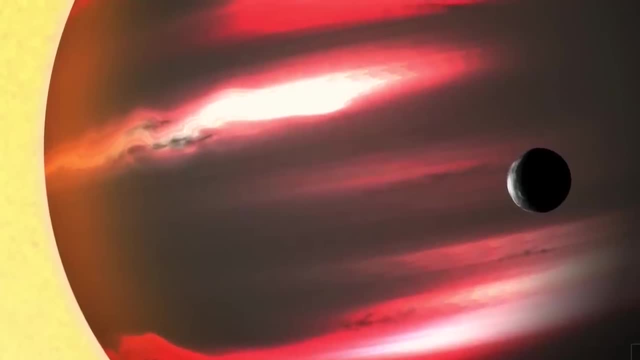 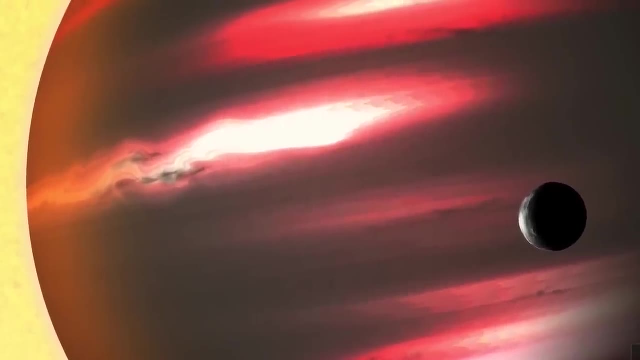 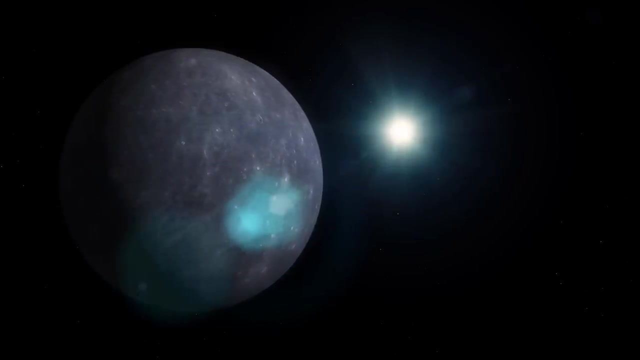 the potential for atmospheric loss from planets subjected to intense stellar radiation. The process of a planet's atmosphere being stripped away and possibly feeding into the star introduces a two-way exchange of material between stars and planets, further blurring the lines of their relationships. This material exchange can lead to changes in the chemical 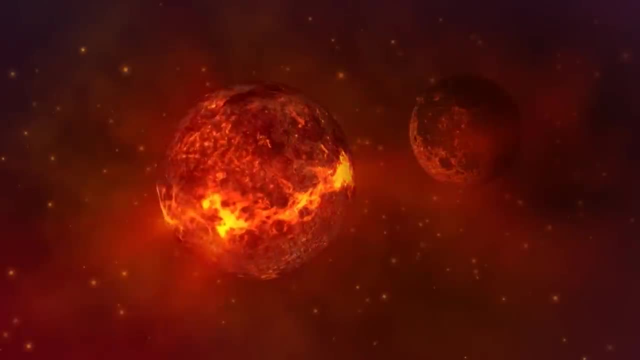 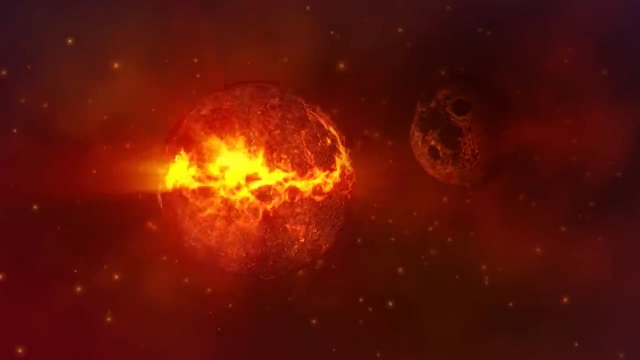 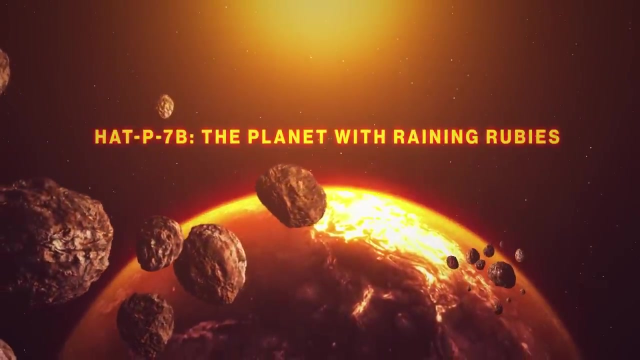 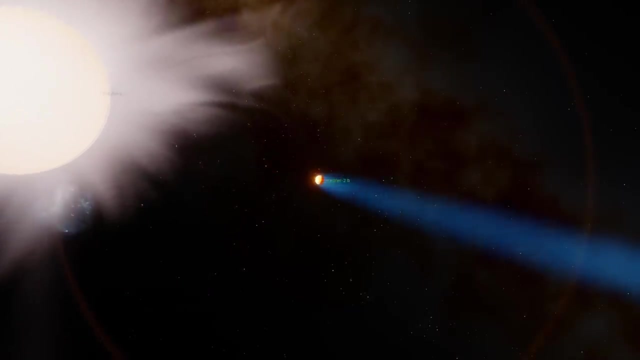 composition of a star's outer layers, providing astronomers with indirect methods to study the atmospheres of exoplanets by observing their host stars. The phenomenon of raining rubies on HAT-P7b, an exoplanet located about 1040 light-years away from Earth, is a captivating aspect of 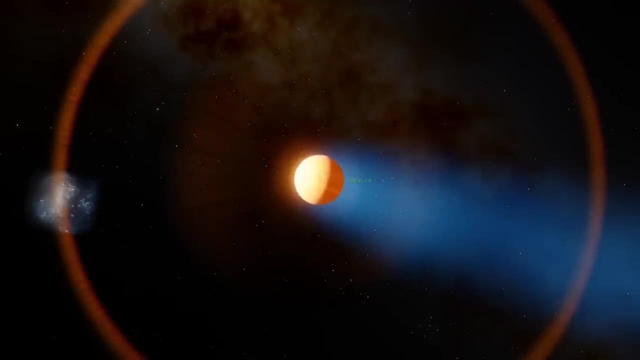 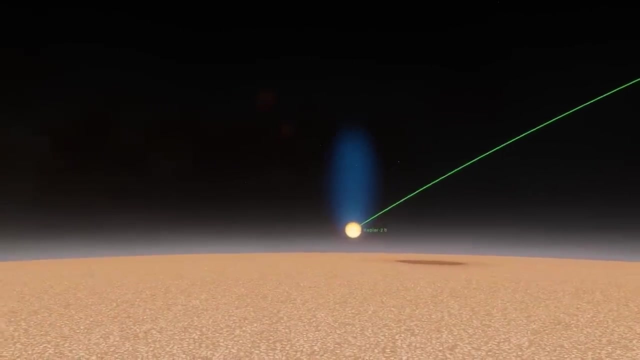 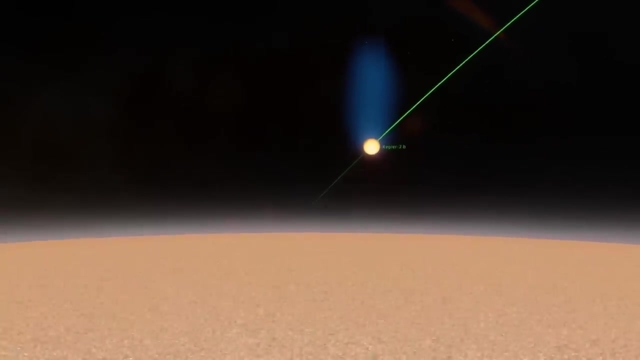 its atmospheric dynamics driven by the extreme conditions present on this gas giant. HAT-P7b is a type of exoplanet known as a hot Jupiter, due to its similar size to Jupiter, but much closer proximity to its host star, leading to significantly higher temperatures. 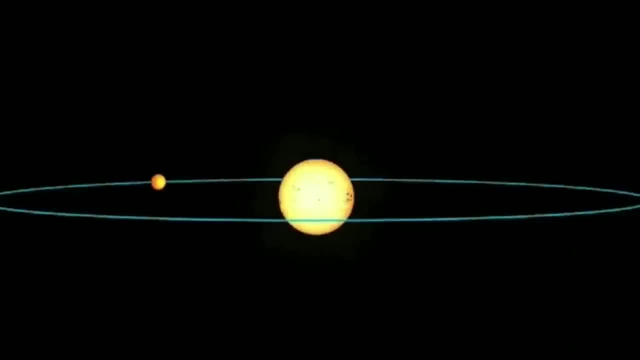 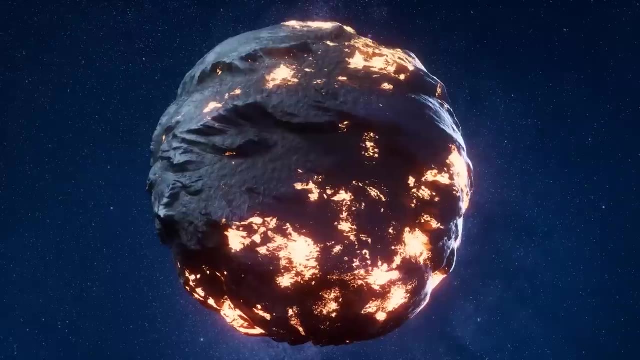 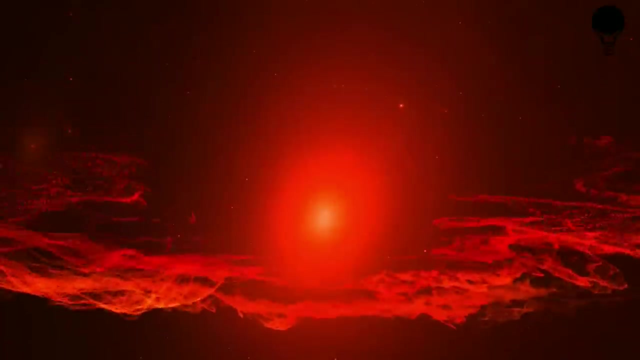 The unique weather pattern, including the precipitation of materials like rubies and sapphires, is attributed to the presence of aluminum oxide in the planet's atmosphere. In Earth's conditions, aluminum oxide crystallizes to form corundum, the base mineral for gems such as rubies and sapphires, depending on the type of trace impurities it. 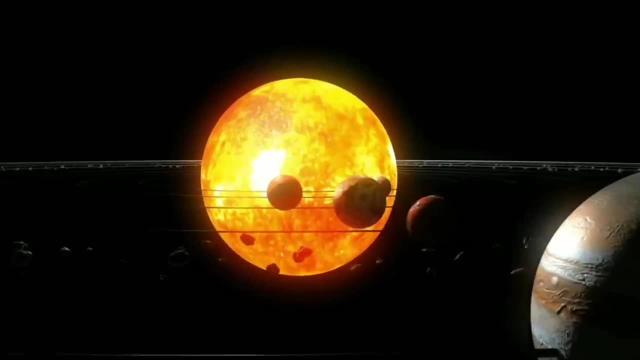 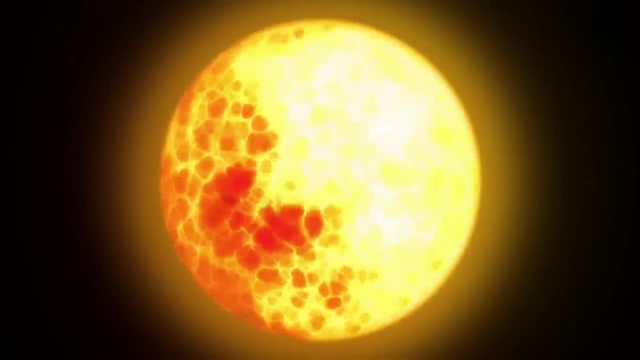 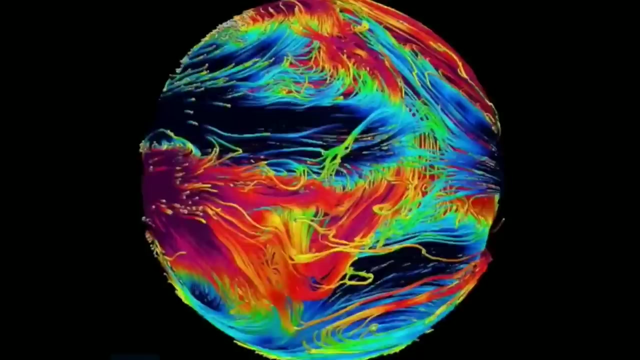 contains. The high temperatures on the day side of HAT-P7b allow for the formation of aluminum oxide vapor within the atmosphere. The planet's close orbit around its host star projects it to intense stellar radiation heating the atmosphere to temperatures where 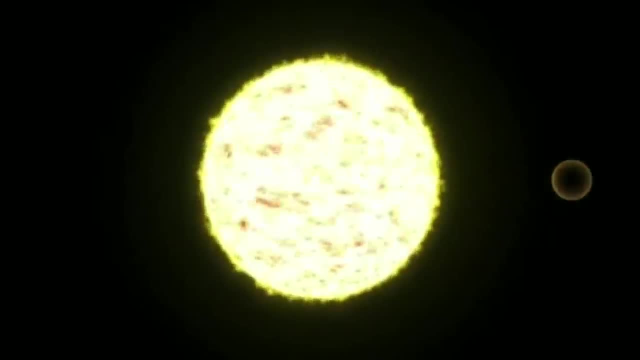 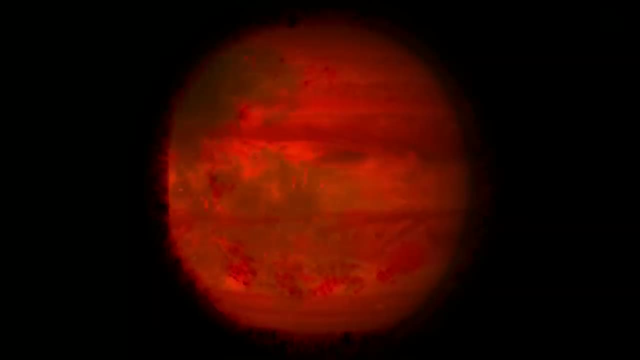 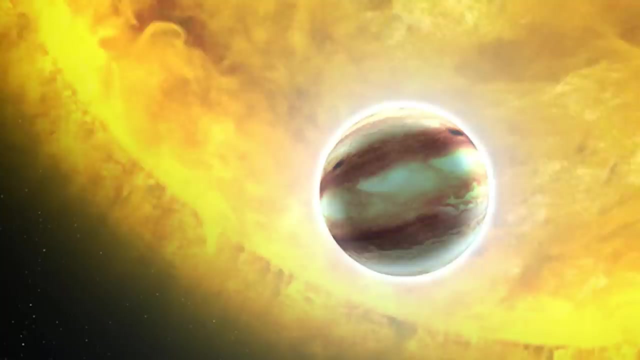 metals can vaporize and complex chemical reactions can occur. As the vapor is carried by strong winds to the cooler night side of the planet, the drop in temperature allows the aluminum oxide to condense and form clouds. Further cooling may lead to the precipitation of corundum crystals. 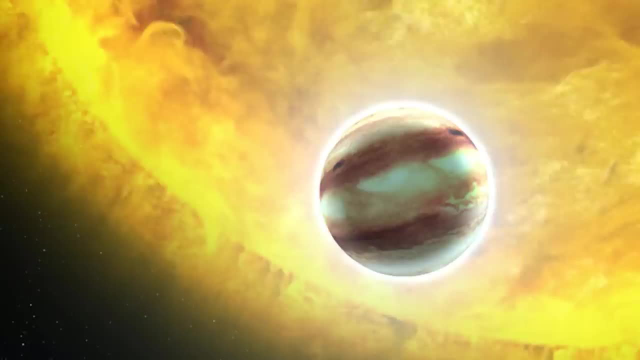 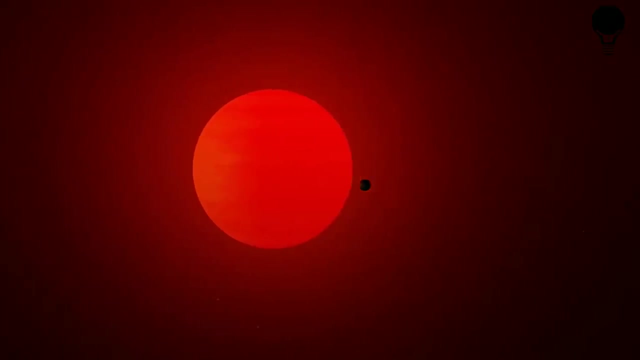 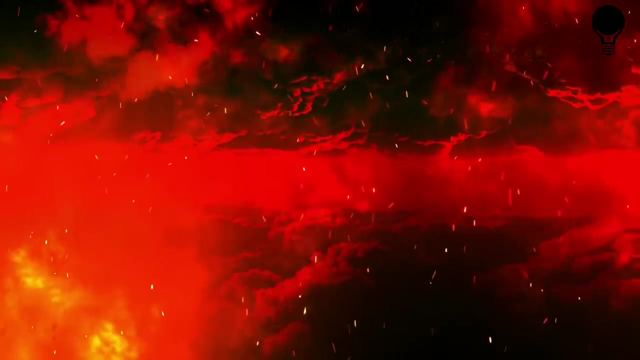 falling as rain in the planet's atmosphere. Depending on specific local conditions, such as trace elements like chromium or iron, these corundum crystals could theoretically resemble rubies and sapphires, hence the poetic description of it: raining gems on HAT-P7b. 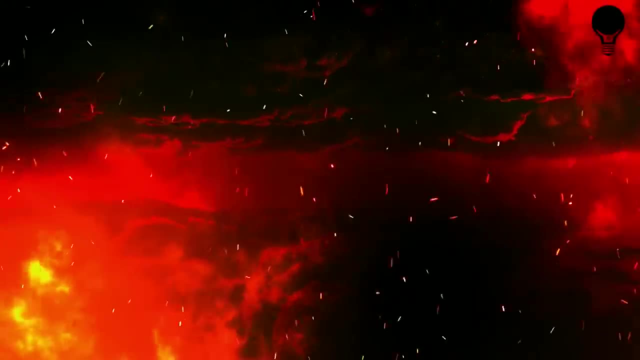 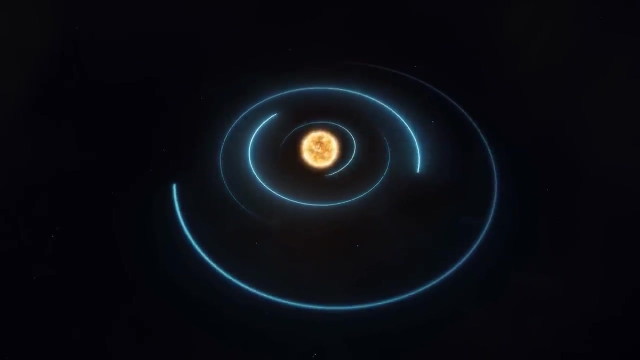 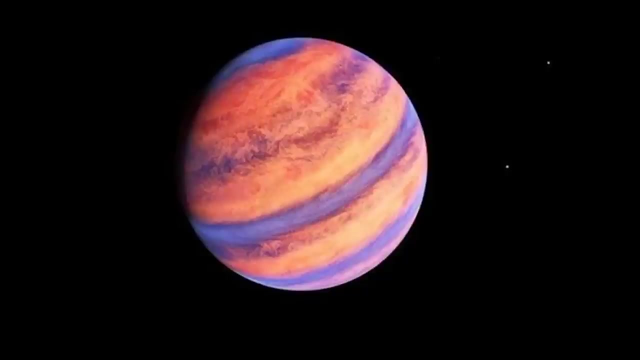 This extraordinary weather phenomenon is part of what makes studying exoplanets so fascinating, offering a glimpse into the vast range of environmental conditions that can exist beyond our solar system. The dynamics of HAT-P7b's atmosphere, the formation of gemstone rain, are studied through observations of the planet's brightness. 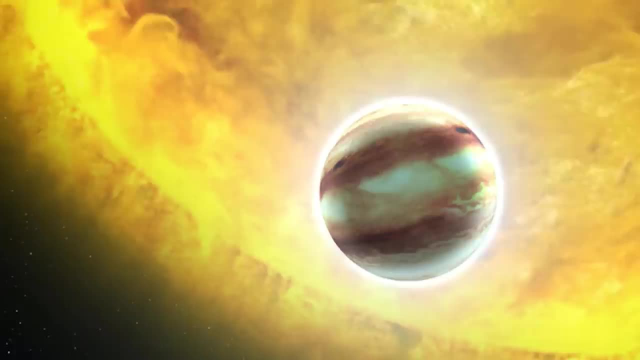 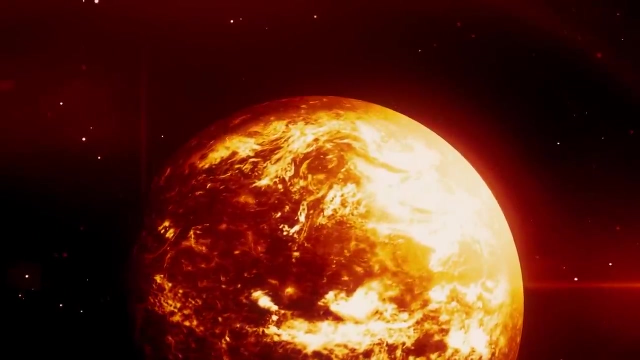 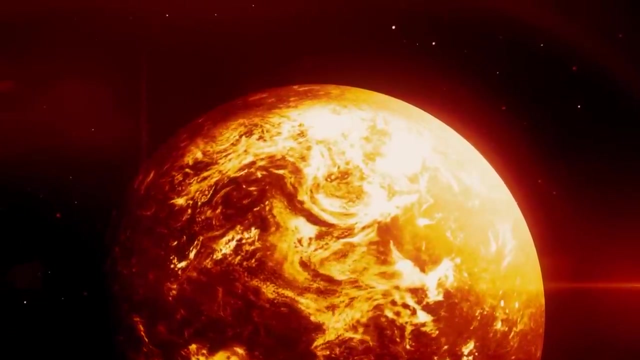 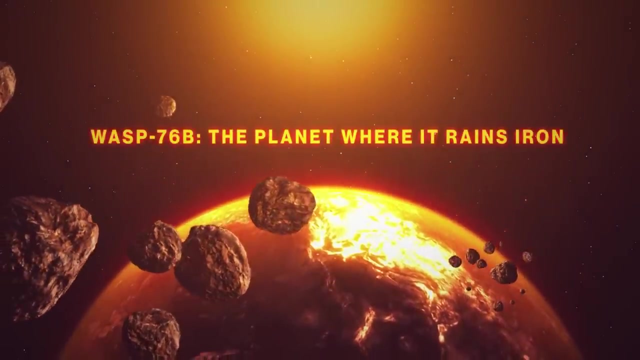 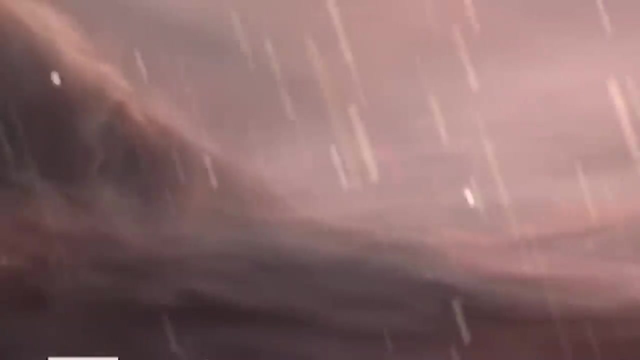 variations and spectral analysis which reveal information about its atmospheric composition and temperature distribution. Such studies provide crucial insights into the atmospheric chemistry and climatic processes of hot Jupiters, expanding our understanding of planetary science. The extraordinary phenomenon of iron rain on WASP-76b, a planet located about 640 light-years away. 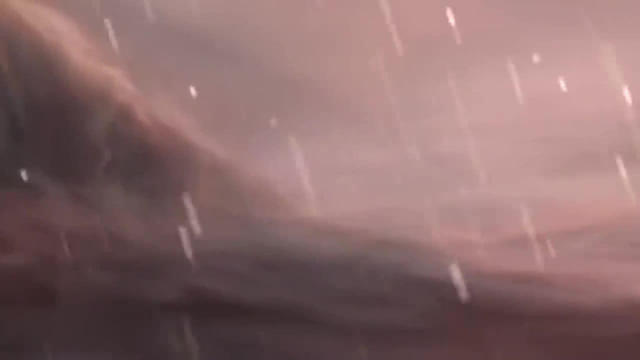 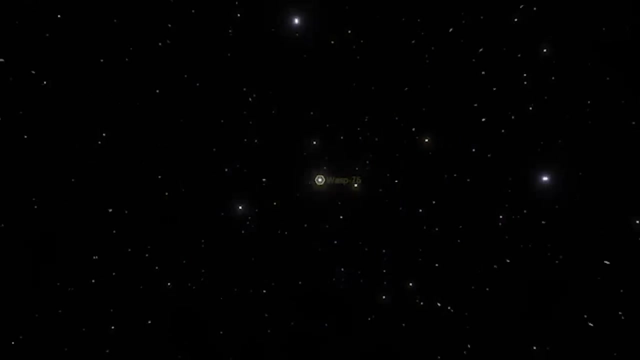 in the constellation of Pisces is a direct consequence of the extreme temperature differences and unique atmospheric dynamics of this ultra-hot Jupiter. WASP-76b orbits very close to its host star, completing one orbit in approximately one-third of the Earth's atmosphere. 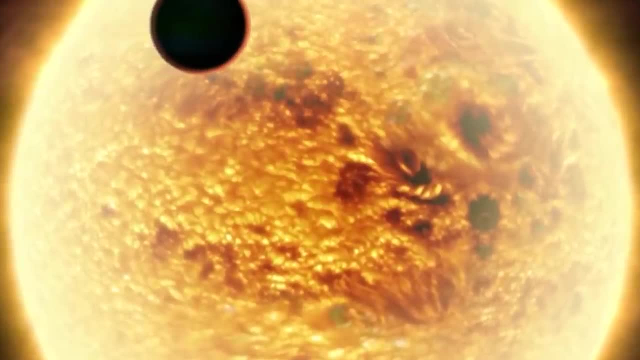 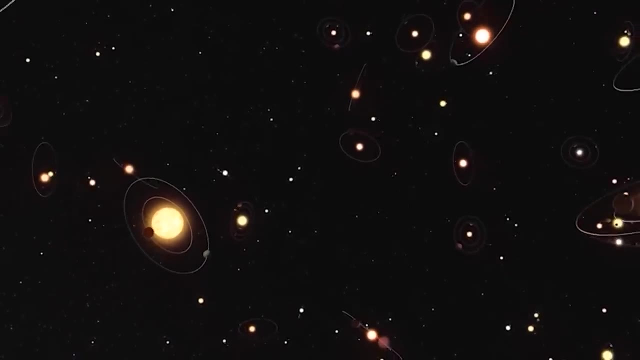 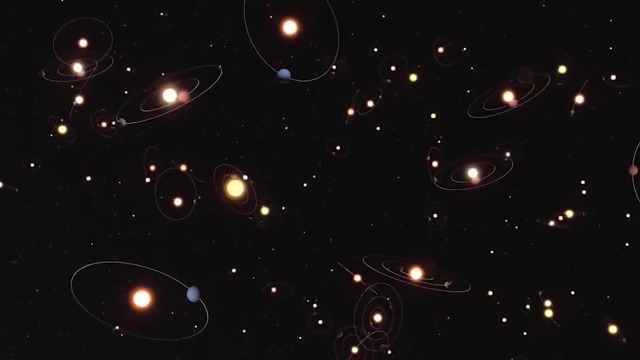 and one-third of the Earth's atmosphere. Wasp-76b orbits in approximately 1.8 Earth days, which subjects one side of the planet, the day side, to intense stellar radiation. This proximity to its star results in daytime temperatures soaring above 2,400 degrees Celsius, approximately 4,350 degrees Fahrenheit. 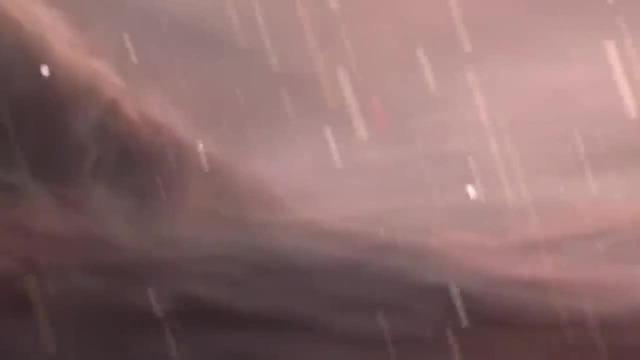 hot enough to vaporize metals, including iron. The mechanism behind the iron rain involves the vaporized iron being carried from the day side to the cooler night side of the planet. As the iron-laden atmospheric currents move to the night side, where temperatures are significantly. 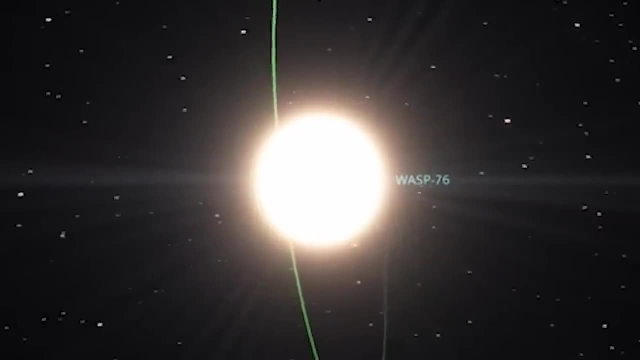 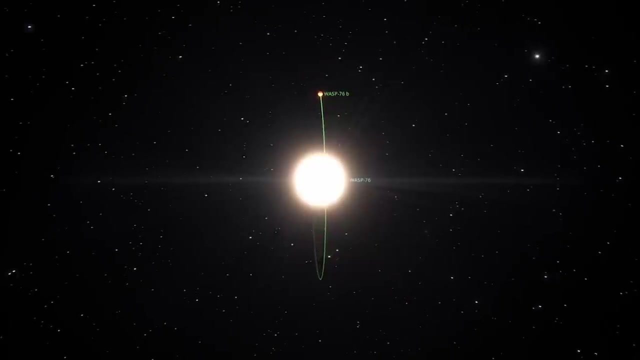 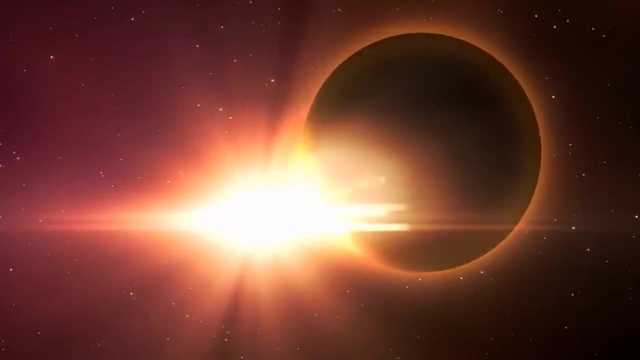 lower, the vaporized iron cools down and condenses into droplets, forming clouds that precipitate as iron rain. This stark contrast in temperature between the planet's day and night sides, combined with the efficiency of atmospheric heat distribution, creates the conditions necessary for 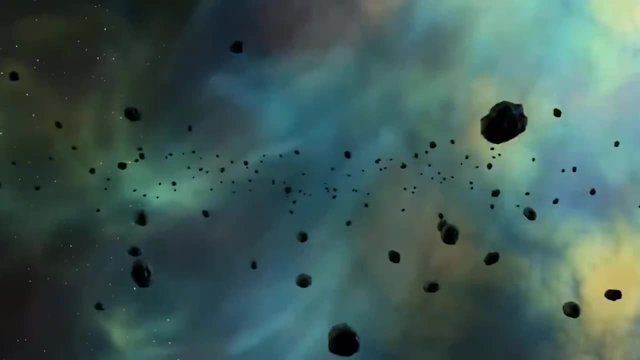 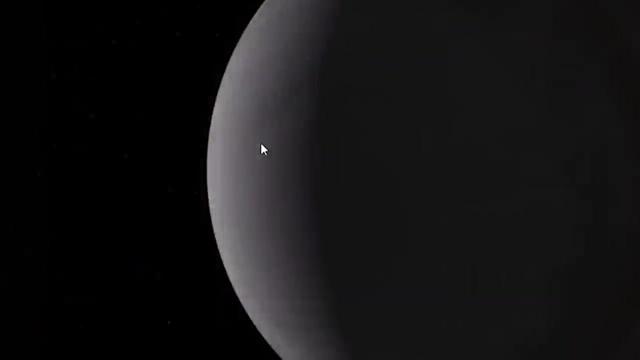 this metallic precipitation. Observations and studies have shown that the ion-laden atmospheric currents can be used to detect the chemical signatures of elements in the planet's atmosphere by analyzing the starlight that filters through it. The presence of iron vapor on the day side. 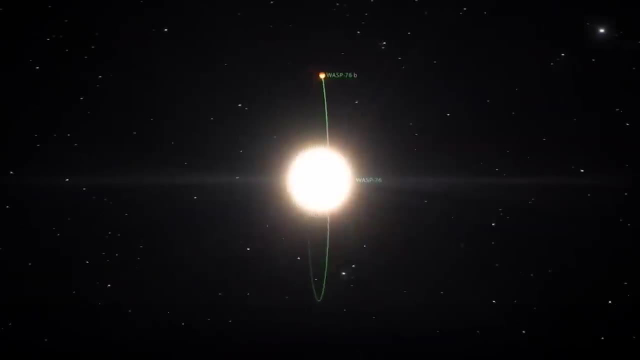 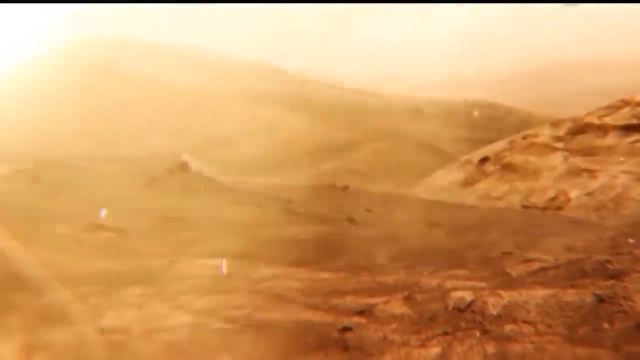 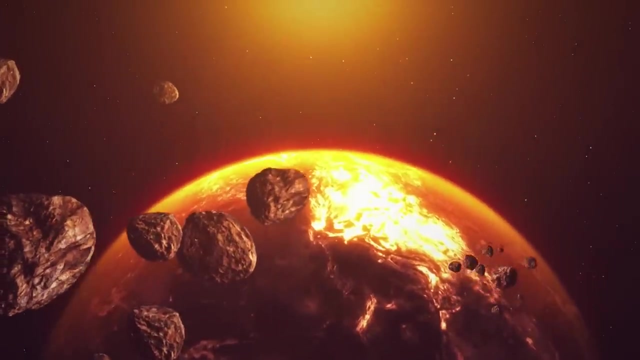 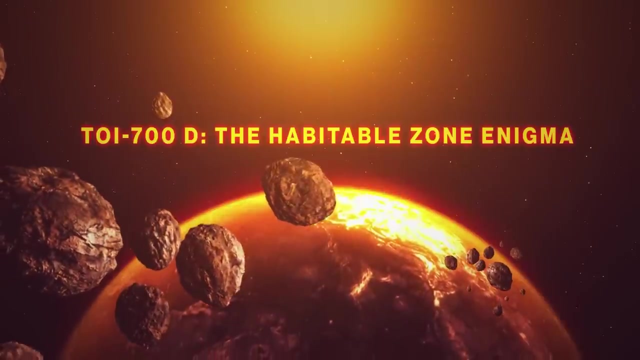 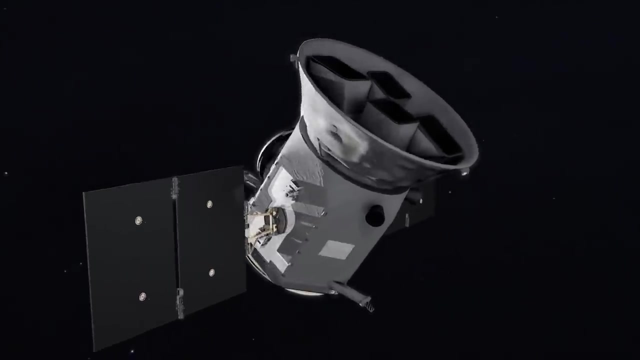 but not on the night side, suggests that the iron condenses and rains down, likely before it can circulate back to the day side. Tau I-700d, an exoplanet discovered by NASA's Transiting Exoplanet Survey Satellite, has captured the attention of scientists and space enthusiasts alike. 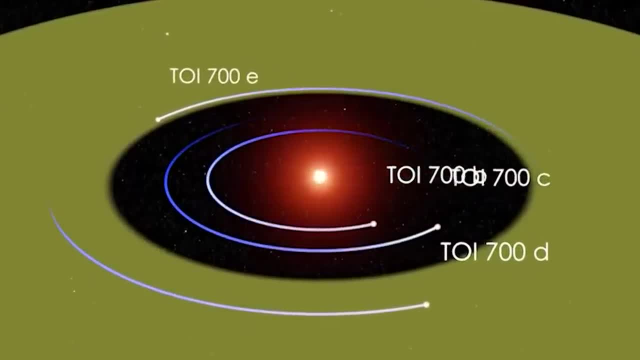 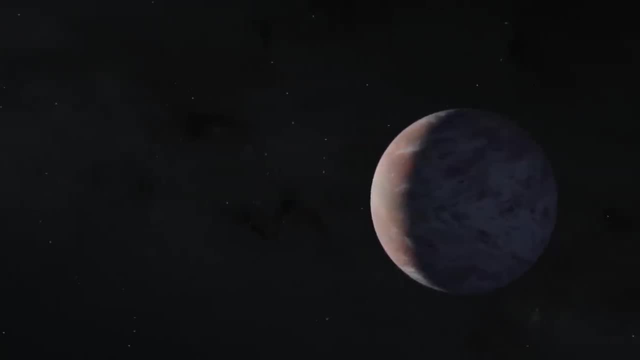 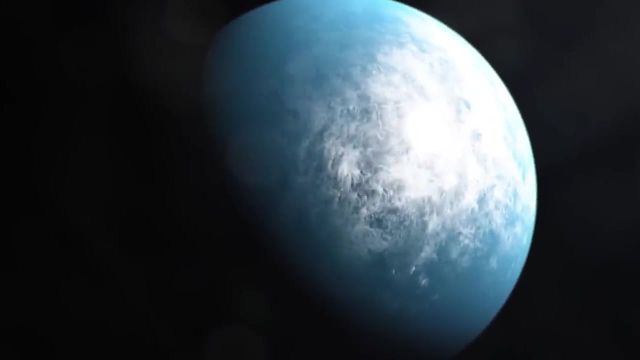 due to its potential habitability. Located about 100 light-years away in the constellation Dorado, Tau I-700d is the outermost planet in its star system, Orbiting a small, cool M-dwarf star. What makes Tau I-700d particularly intriguing as a candidate for habitability? 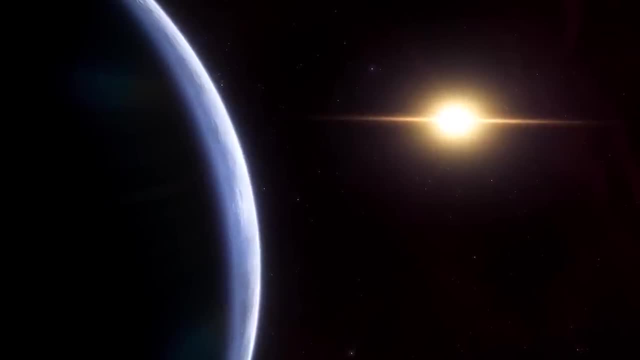 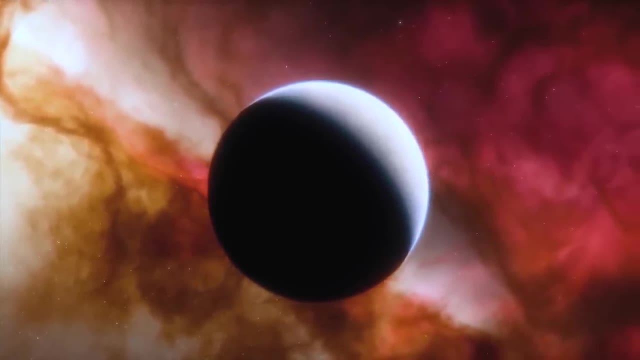 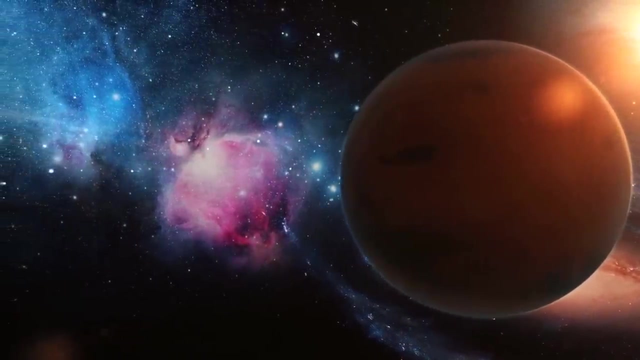 are several key characteristics that differentiate it from many other exoplanets. Tau I-700d resides in its star's habitable zone, the region around a star where conditions could be just right for liquid water to exist on a planet's surface, a crucial ingredient for life. 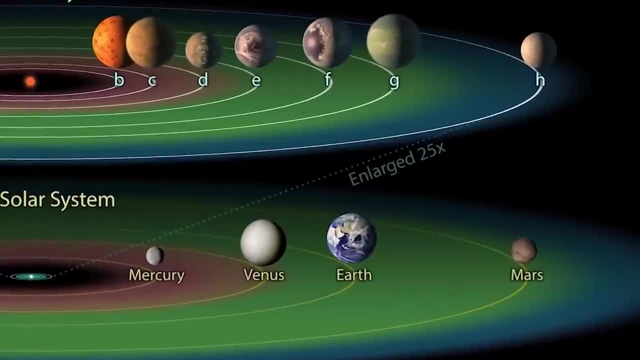 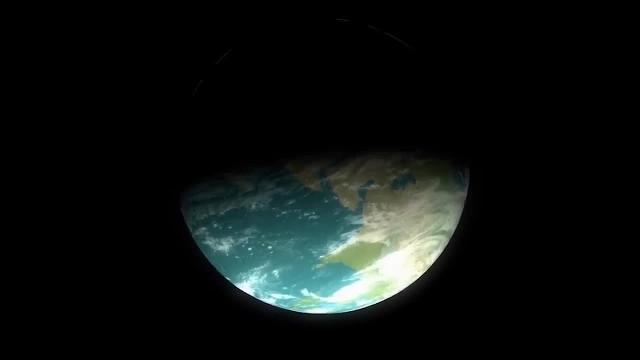 as we know it, Tau I-700d is the outermost planet in its star system. The planet's orbit places it at a distance where it receives approximately the same amount of stellar energy from its star as Earth does from the Sun. This equilibrium suggests that 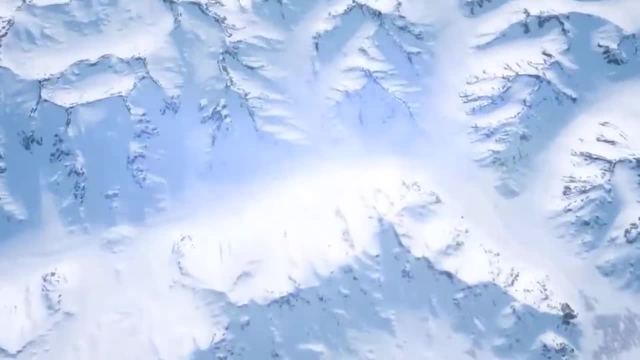 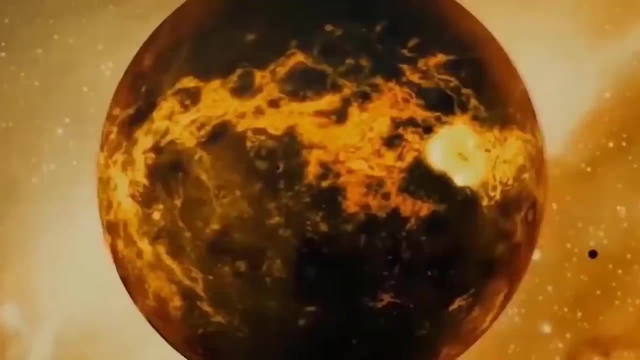 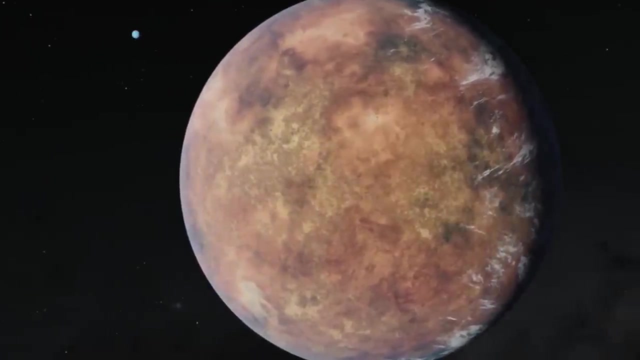 the temperatures on Tau I-700d could allow for the presence of liquid water, provided it has a suitable atmosphere. Tau I-700d is roughly Earth-sized, with estimates suggesting it has a radius about 1.2 times that of Earth. This size indicates that the planet could have a rocky. 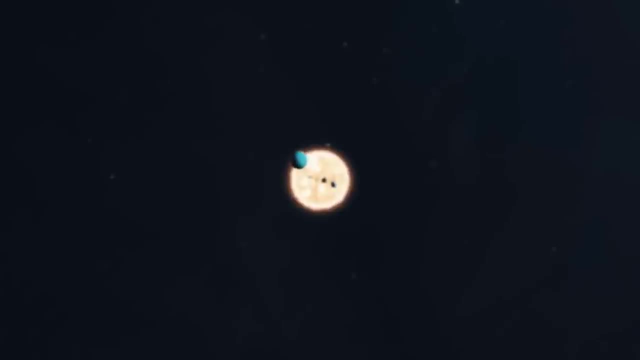 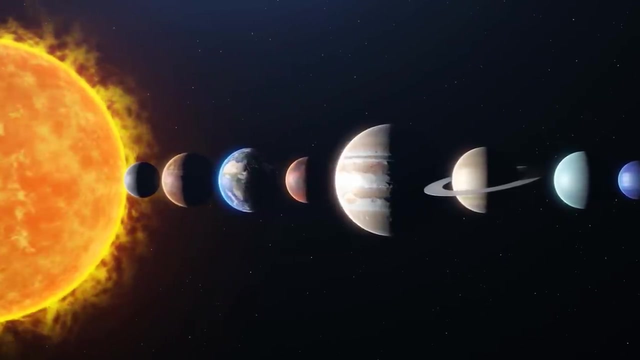 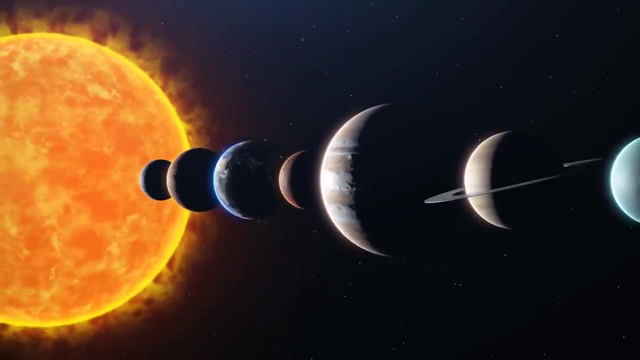 composition similar to that of Earth, Mars and Venus. Planets of this size are more likely to maintain a stable atmosphere, which is another critical component for potential habitability. An atmosphere could not only provide the necessary gases for life, but also regulate the planet's temperature by trapping heat through the greenhouse effect. 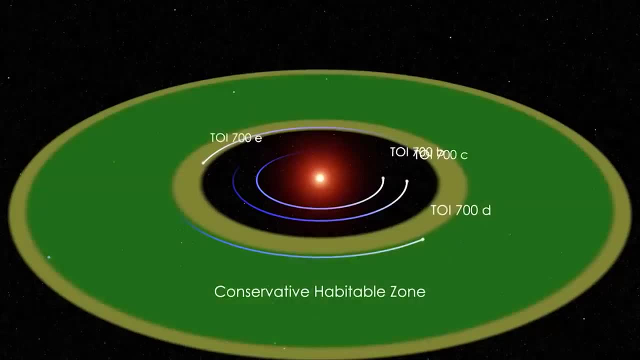 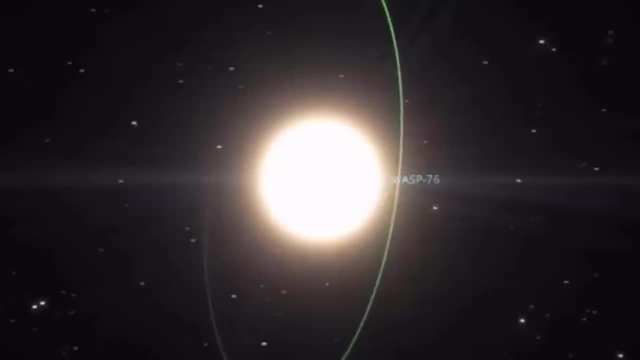 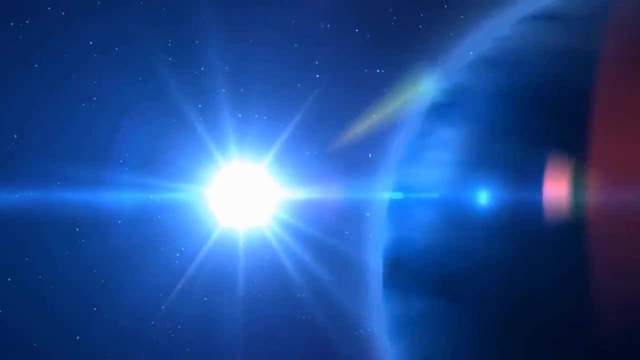 The orbit of Tau I-700d is also tidally locked to its star, meaning one side of the planet is perpetually day, facing the star, while the other side remains in constant night, While this could lead to extreme temperature variations between the day and night sides. 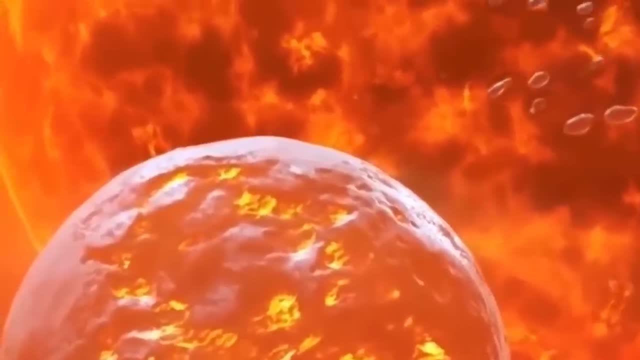 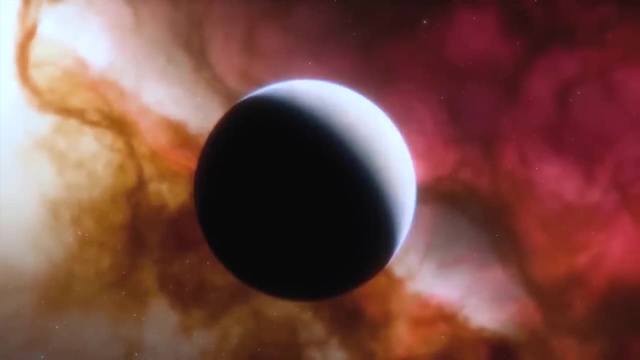 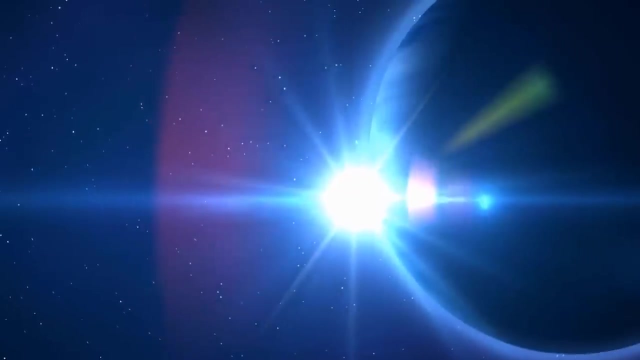 the presence of an atmosphere could help to distribute heat around the planet more evenly, potentially stabilising the climate enough to support liquid water and, by extension, life. The host star, Tau I-700d, is a quiet M-dwarf exhibiting fewer flares than many other stars of. 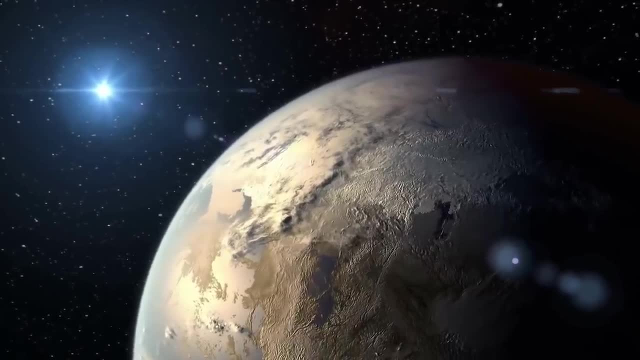 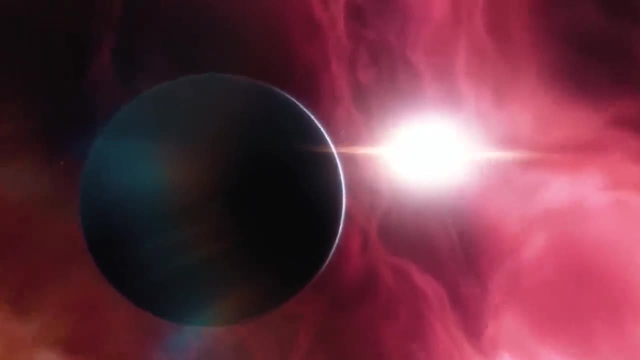 its type. This is the reason why Tau I-700d is known as the M-dwarf, as it is known for its stellar flares. Stellar flares can strip away a planet's atmosphere and bombard its surface with harmful radiation, both of which are detrimental to habitability. The relatively calm nature of 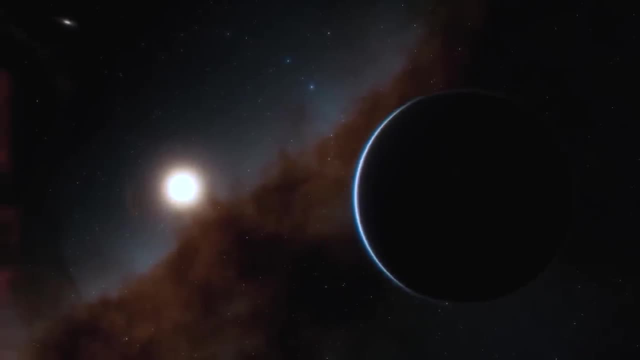 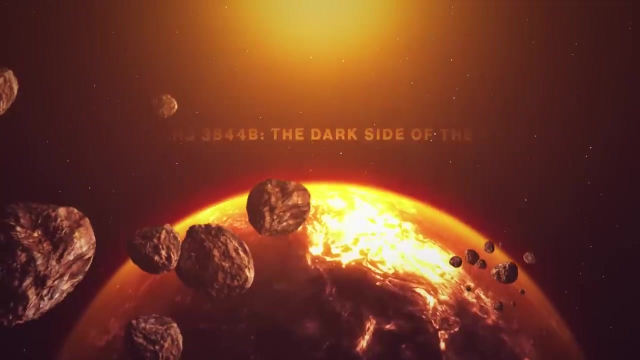 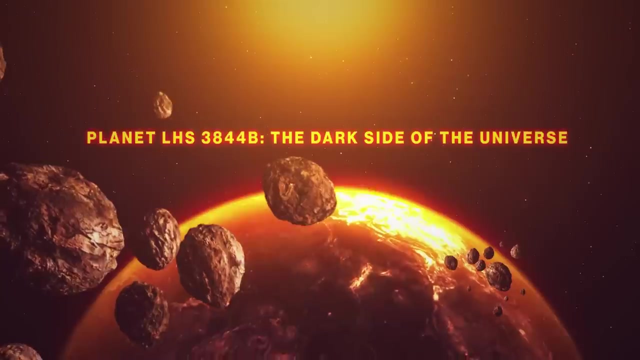 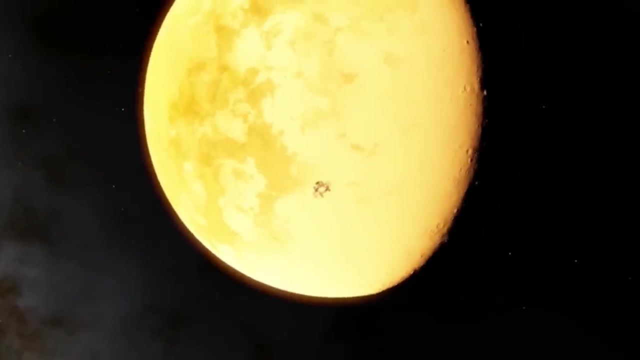 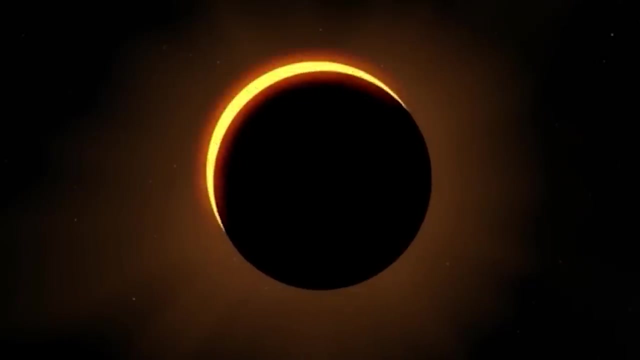 Tau I-700 enhances the prospects for Tau I-700d's habitability by minimising these risks. LHS 3844 b, An exoplanet orbiting a red dwarf star approximately 48.6 light-years away in the constellation of Indus, showcases extreme temperature differences between its day and 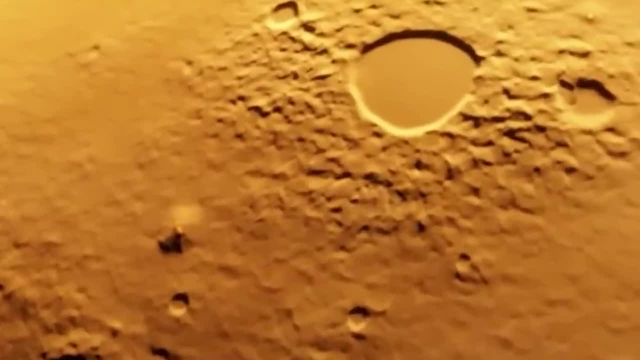 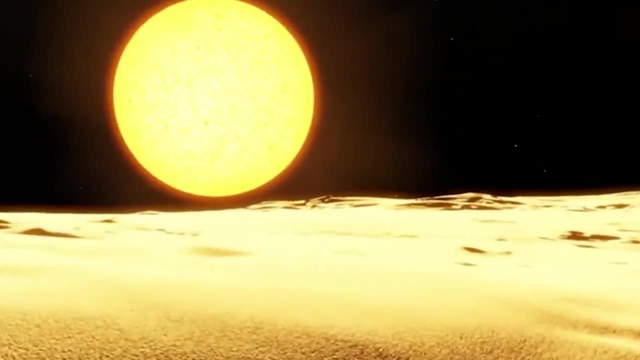 night sides due to a combination of its close proximity to the star's atmosphere. LHS 3844 b: This exoplanet is known for its close proximity to its host star and its likely lack of a significant atmosphere. This terrestrial planet completes an orbit around its star in just 11. 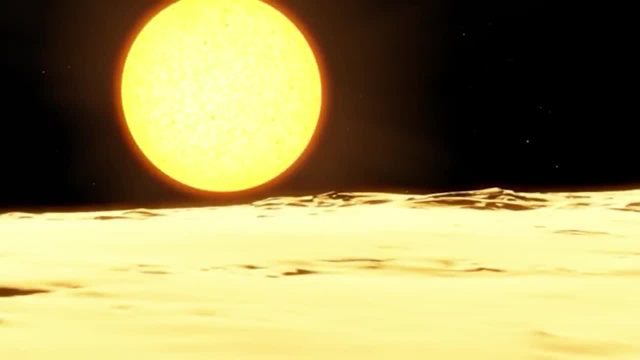 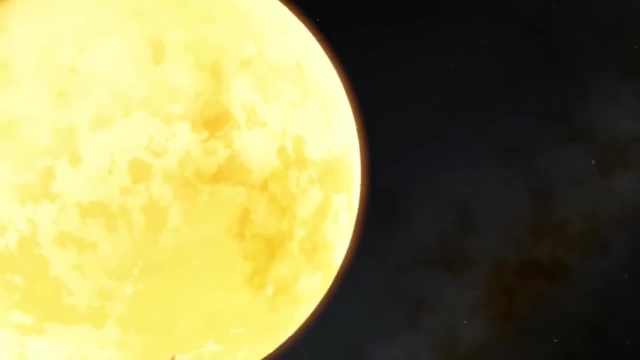 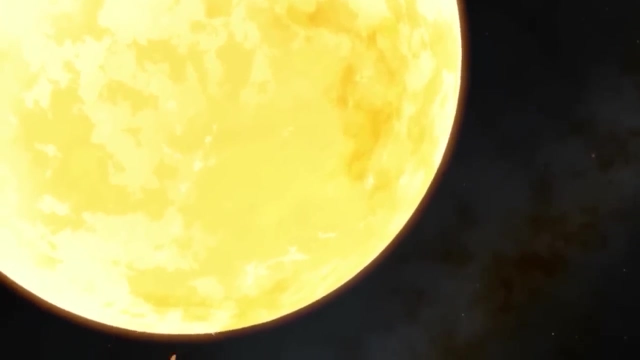 hours, placing it much closer to its star than Earth is to the Sun. Such a tight orbit results in the planet receiving a high amount of stellar radiation on its dayside, leading to extremely high temperatures, The significant factor contributing to the stark temperature contrast between the day. 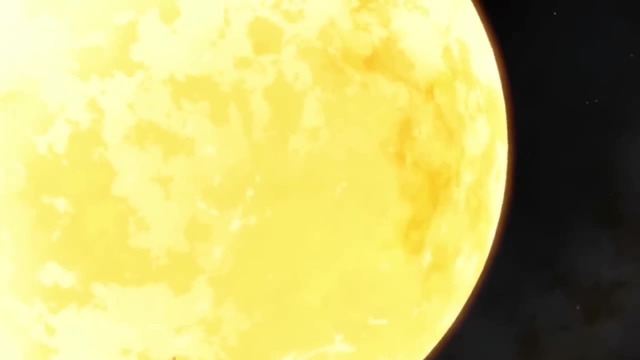 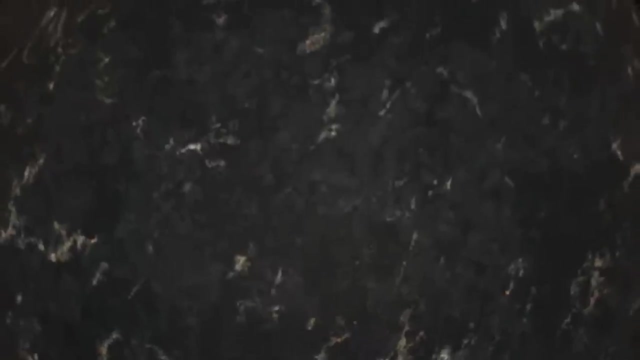 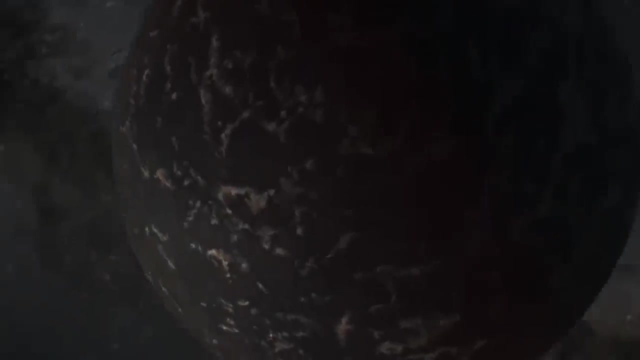 sides of LHS 3844 b is its tidally locked nature. Being tidally locked means the same side of the planet always faces the star, receiving constant daylight, while the opposite side remains in perpetual darkness, Without an atmosphere to redistribute heat around the planet. the 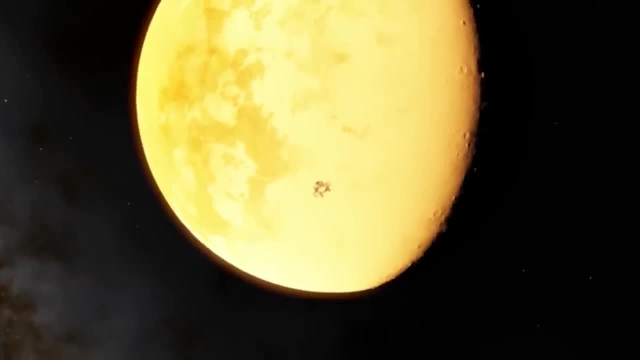 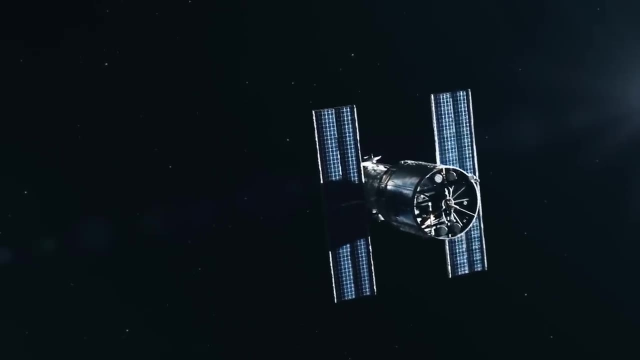 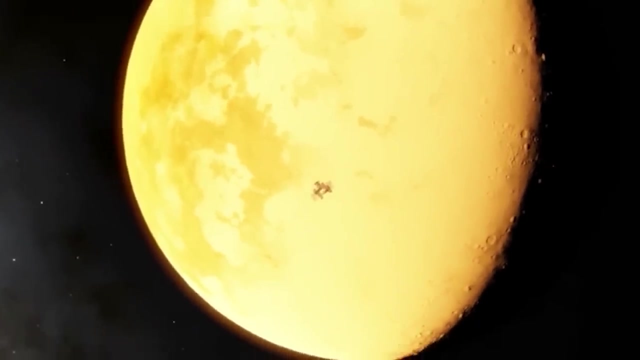 temperature on the day side can soar, while the night side remains much cooler due to the lack of direct stellar heating. Observations and studies, including those using NASA's Spitzer Space Telescope, have provided evidence suggesting that LHS 3844 b has little to no atmosphere. An atmosphere plays a crucial role in a planet's 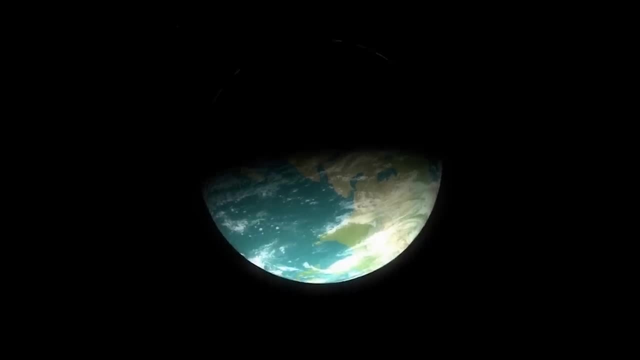 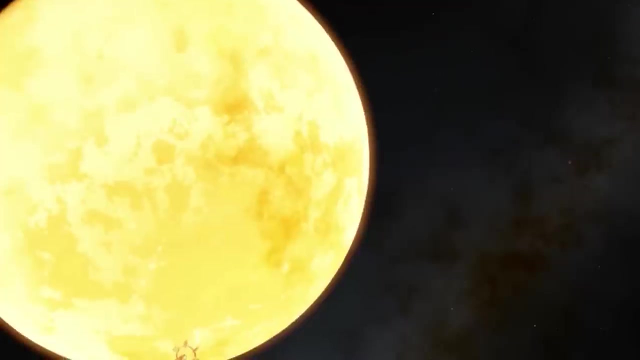 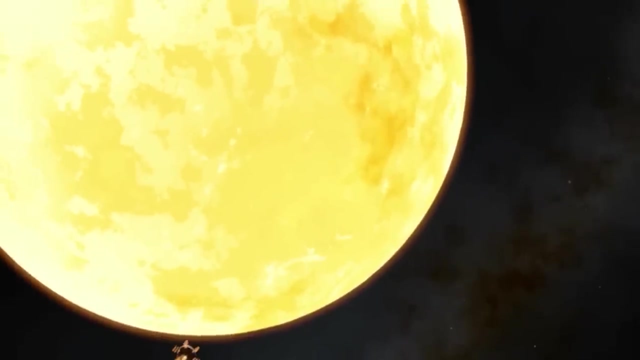 climate by circulating heat On Earth, for example. the atmosphere helps to moderate temperatures across the globe by distributing heat from the equator toward the poles. The apparent absence of an atmosphere on LHS 3844 b means that heat from its star is not efficiently spread across the planet. As a result, 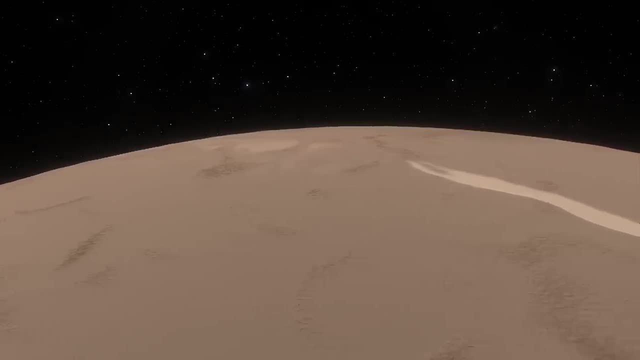 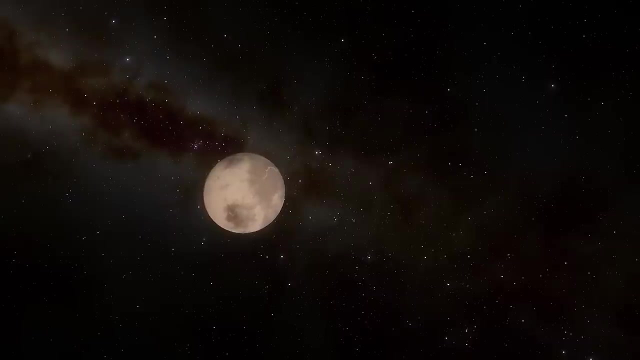 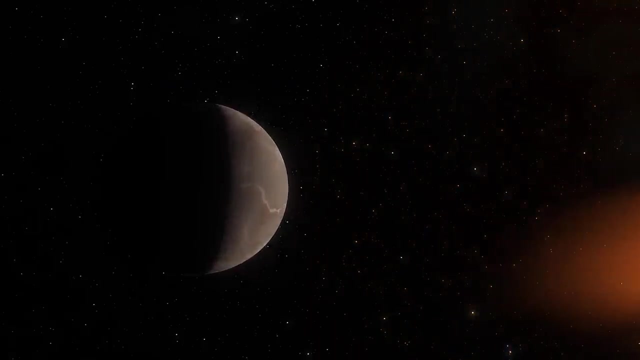 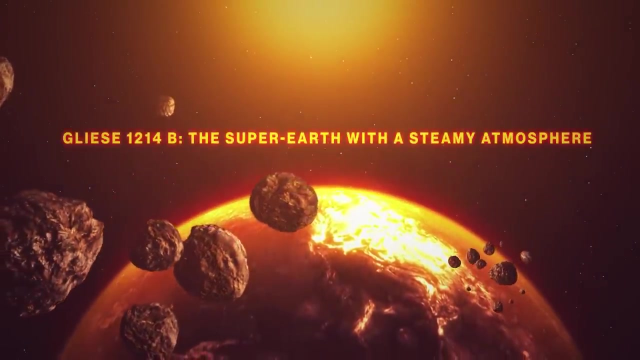 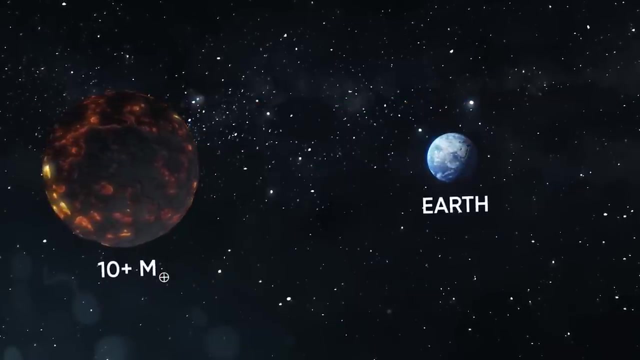 the temperature on the side of LHS 3844 b facing its star can reach up to approximately 800 degrees Celsius, while the night side can be drastically cooler, with a significant temperature drop. LHS 3844 b is considered a super-Earth because it is an exoplanet that is larger than Earth. 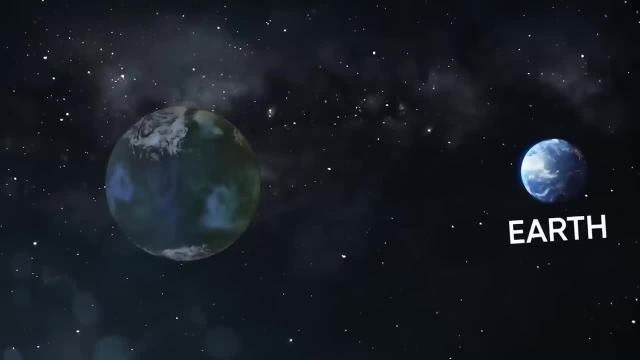 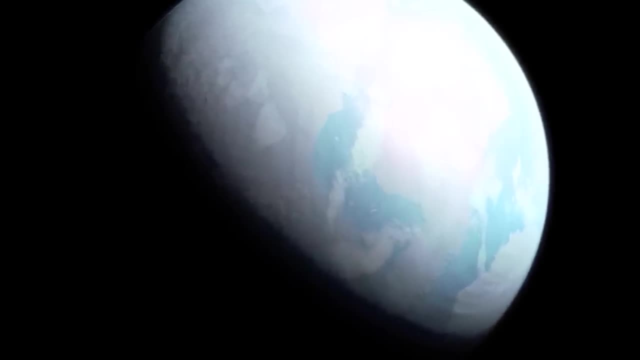 but smaller than the ice giants Uranus and Neptune, with a mass and radius that suggest a composition different from that of the rocky planets in our solar system. Specifically, LHS 3844 b has about 6.5 times the Earth's mass. 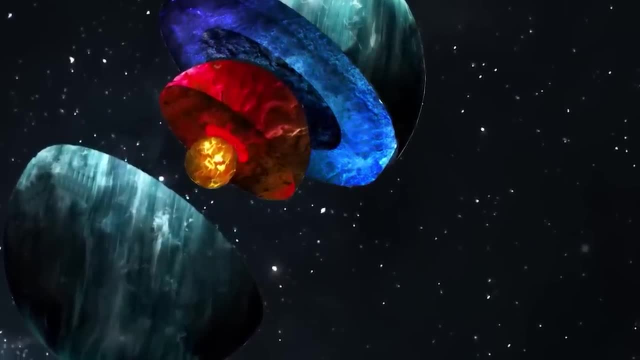 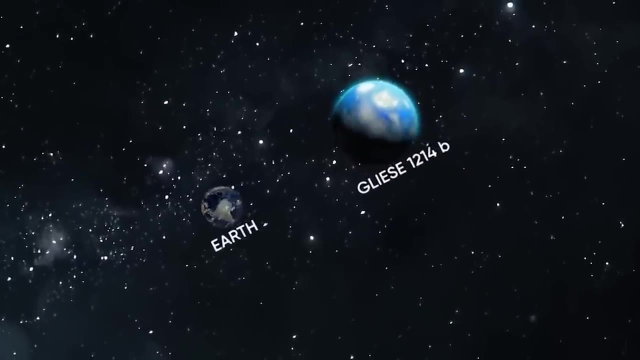 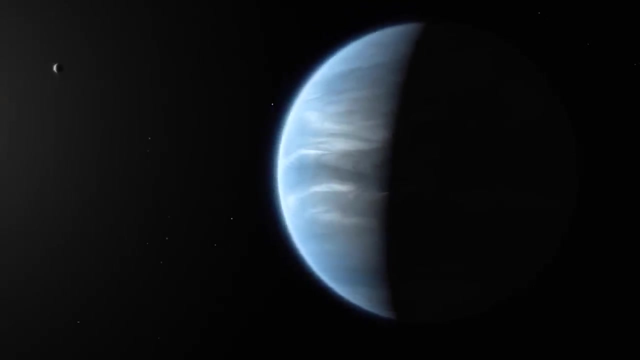 and a radius approximately 2.7 times larger than Earth's, placing it in the category of super-Earths due to its size and mass. This classification is significant because it indicates that LHS 3844 b could have a variety of characteristics, including a dense atmosphere, a possibility of liquid water or even an ocean. 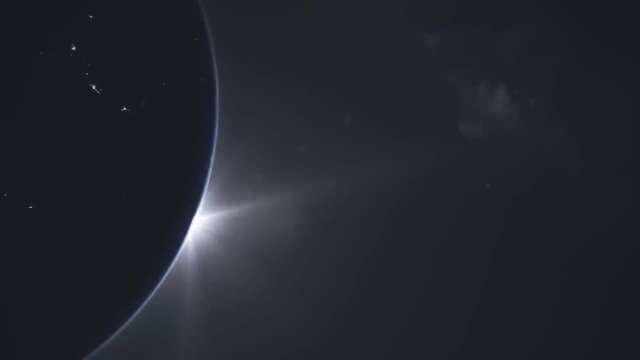 covered world depending on its composition and the conditions present in its atmosphere. LHS 3844 b represents the earth's density and temperature, which are the same as the Earth's temperature and temperature. LHS 3844 b represents the Earth's velocity and temperature. The term super-Earth 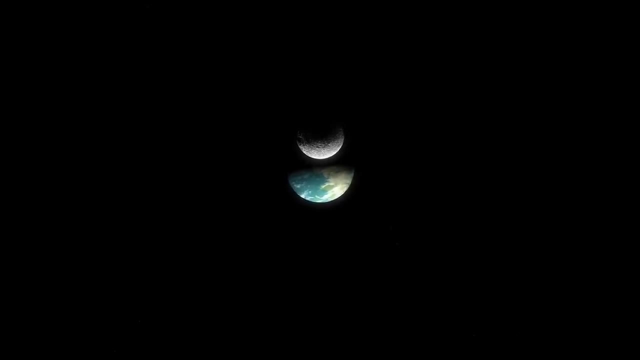 but still, the extra-tendency of the Earth, thus becoming a surface, is considered an issue of interest in the future, But we're often faced with concerns about these types of issues such as: the unique diversity of the environment does not necessarily imply that the planet is habitable. 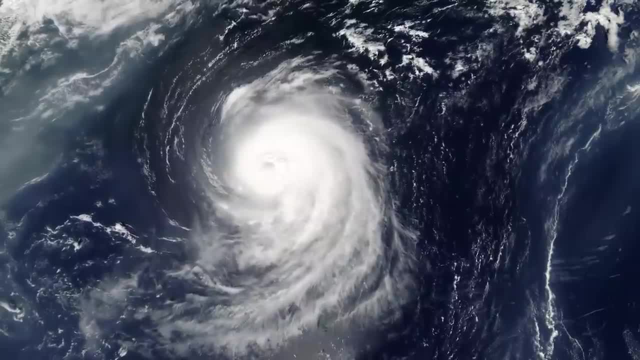 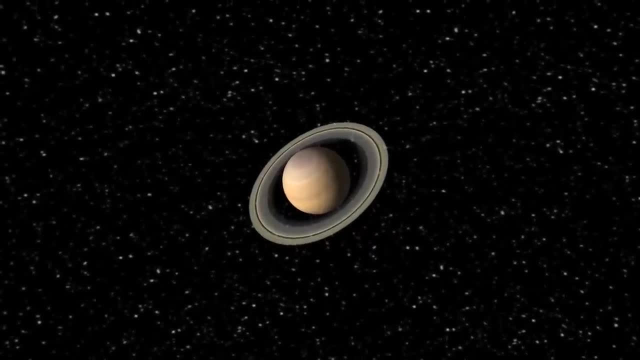 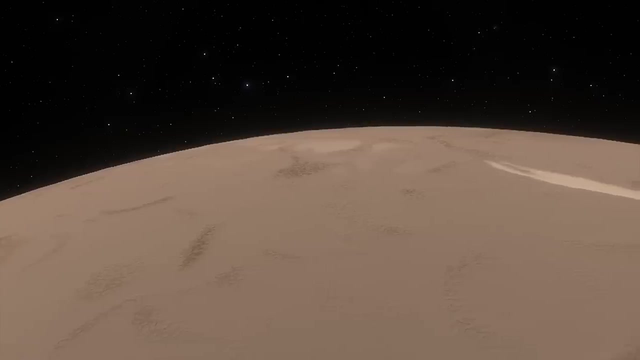 or Earth-like in terms of climate and conditions. Instead, it refers to the planet's size as being between that of Earth and Neptune, and suggests a diversity in the types of planets that exist beyond our solar system. Super-Earths like Gliese 1214 b are of particular interest to astronomers. 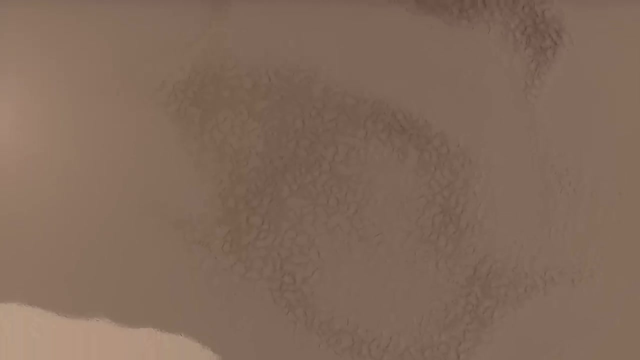 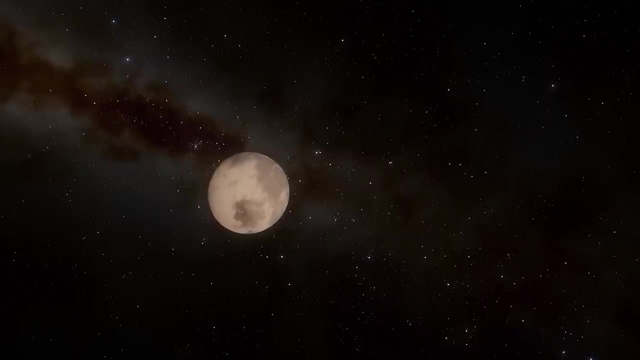 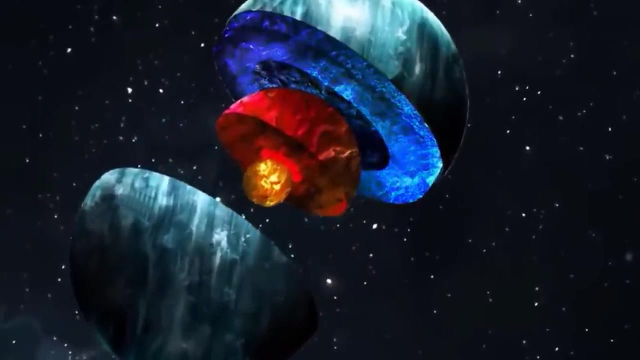 because they represent a class of planets not found in our solar system, offering unique opportunities to study planetary formation, evolution and the potential for life in conditions different from those on Earth. Gliese 1214 b orbits a red dwarf star located about 48 light-years away. 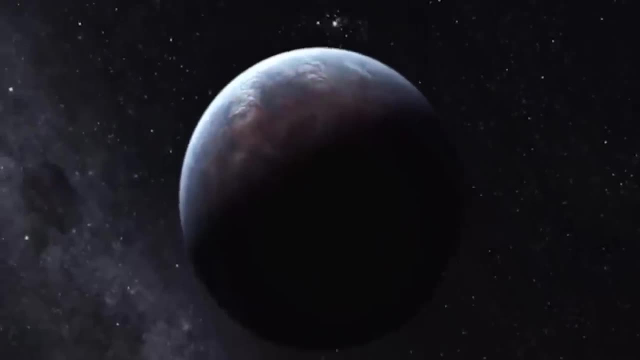 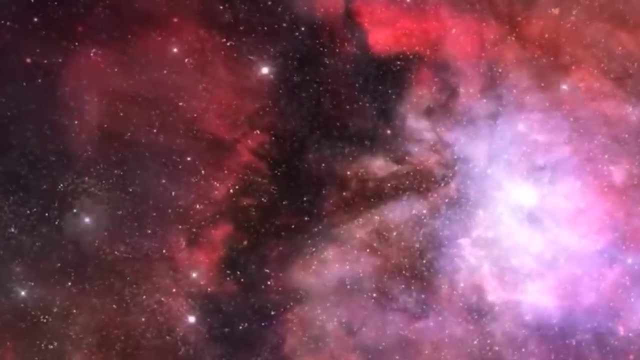 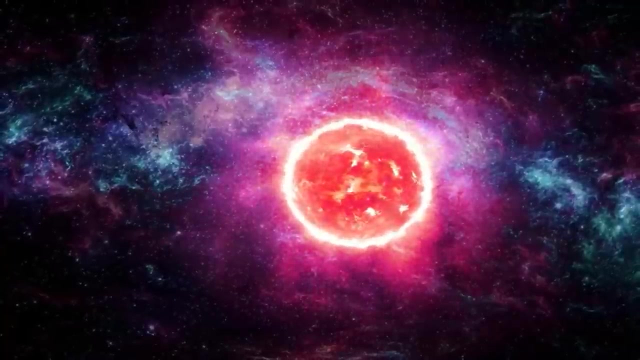 in the constellation Ophiuchus. Its relatively short orbital period of about 38 hours means that it is very close to its host star, which influences the planet's temperature and atmospheric conditions. Observations suggest that Gliese 1214 b has a thick atmosphere. 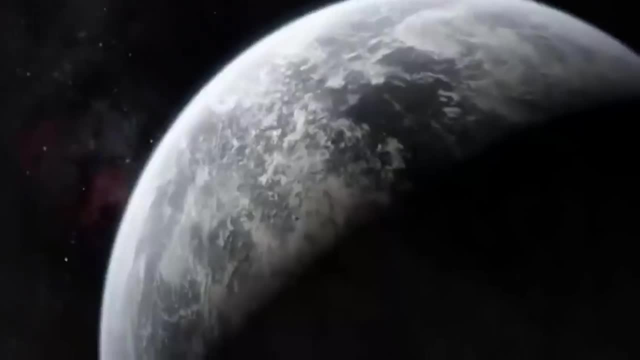 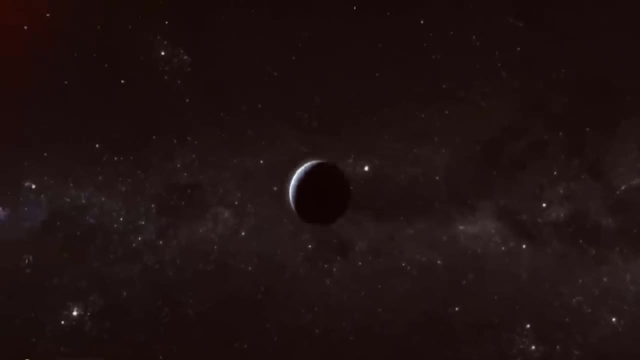 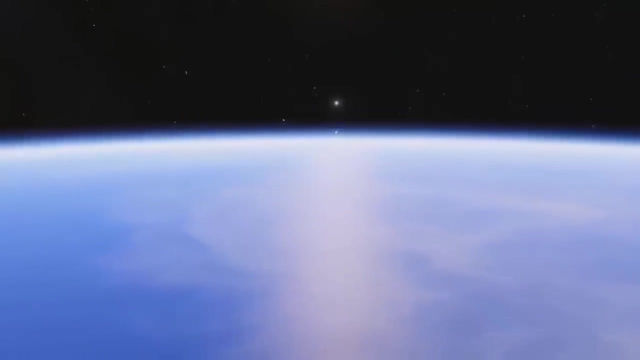 which could be composed of water, vapour or other heavy molecules, leading to speculations about its surface conditions and the potential for an exotic form of water under high pressure and temperature known as a water world. The study of Gliese 1214 b and other super-Earths. 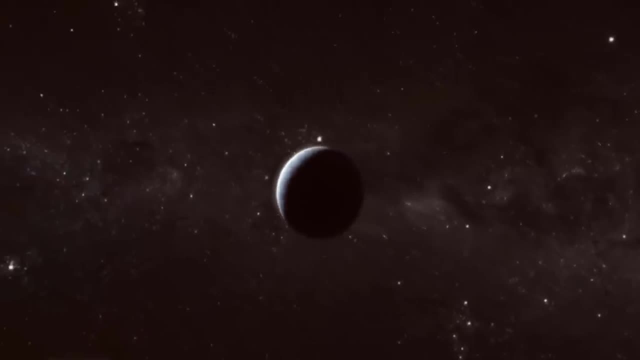 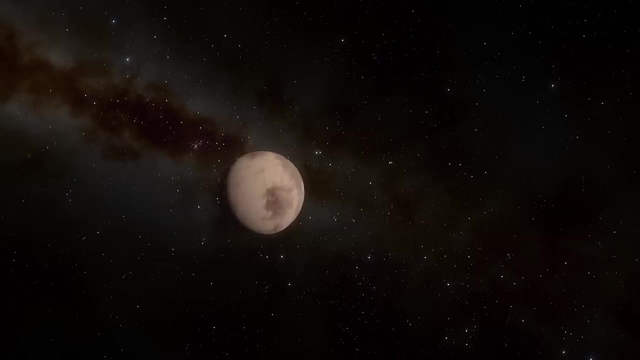 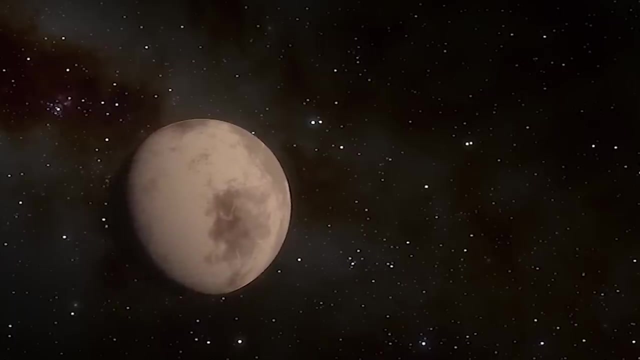 is crucial for advancing our understanding of planetary diversity across the Universe. By analysing the atmospheres of these planets through techniques such as transit spectroscopy, scientists can gain insights into their chemical compositions, weather patterns and, potentially, their capacity to support life. 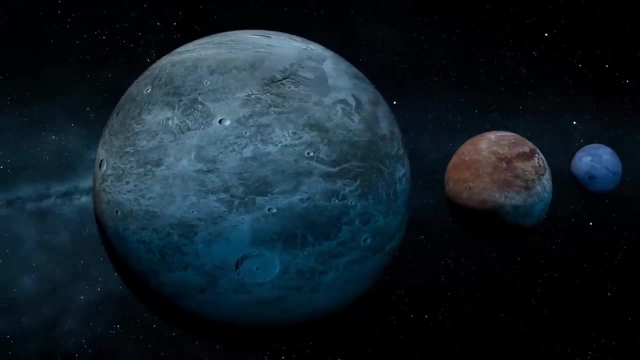 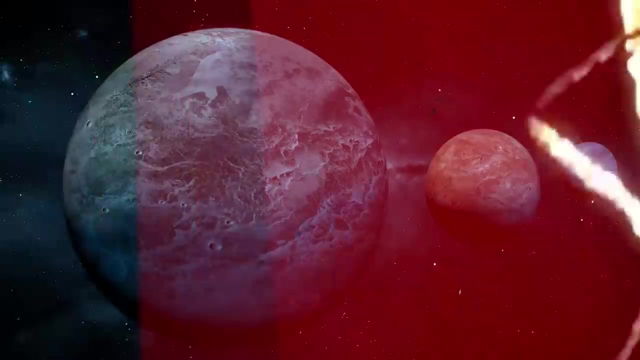 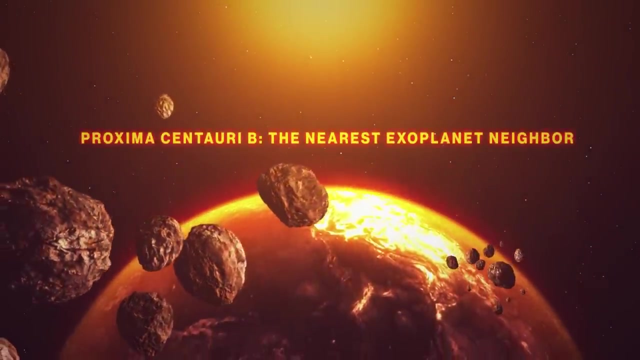 This research not only broadens our knowledge of exoplanets, but also helps refine models of planetary systems and the formation of planets under varying conditions. The study of Gliese 1214 b is a very interesting one. The study of Gliese 1214 b is a very interesting one. 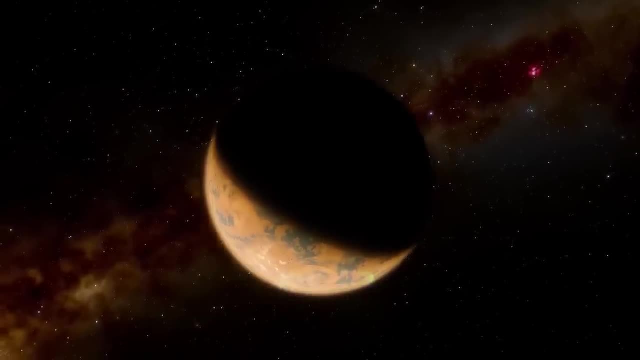 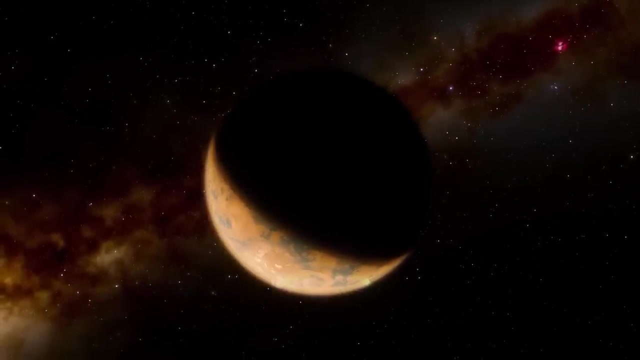 Proxima Centauri b. orbiting the closest star to the Sun, Proxima Centauri, approximately 4.2 light-years away in the constellation of Centaurus, emerges as a prime candidate in the search for extraterrestrial life due to several compelling characteristics. 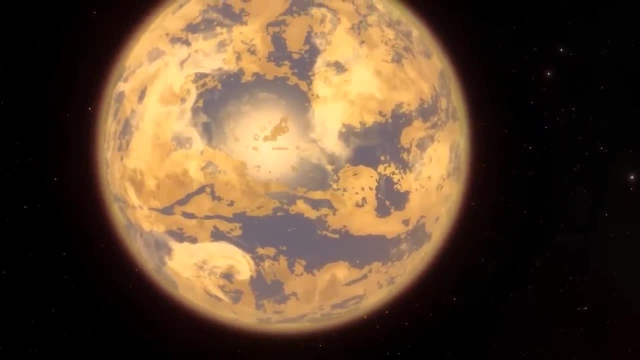 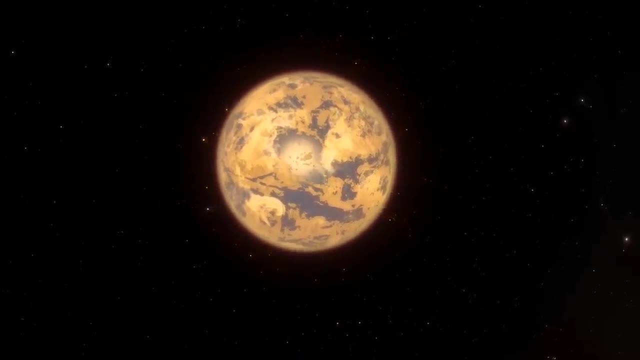 First and foremost, its location within the habitable zone of its star is a critical factor. This zone, often referred to as the Goldilocks zone, is the range of distances from a star where conditions might be just right for liquid water to exist on a planet's surface. 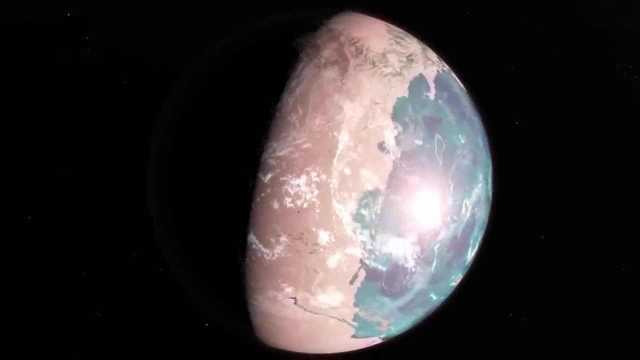 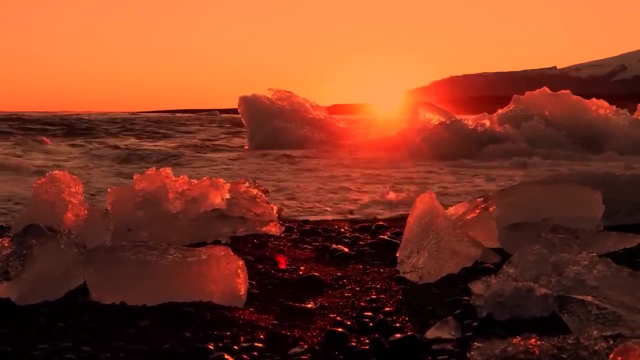 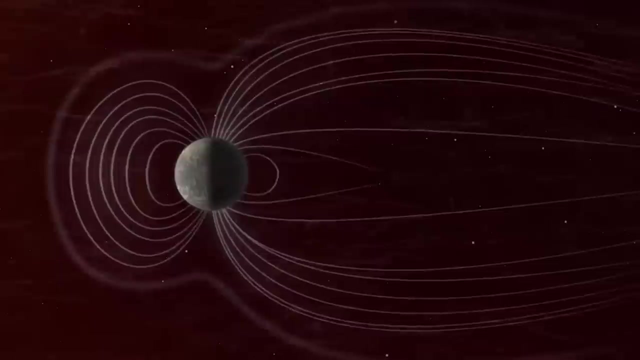 an essential ingredient for life as we understand it. Proxima Centauri b's orbit within this zone suggests that it has the potential to maintain surface temperatures that could support liquid water, assuming it has a suitable atmosphere. Another factor that bolsters the case for Proxima Centauri b: 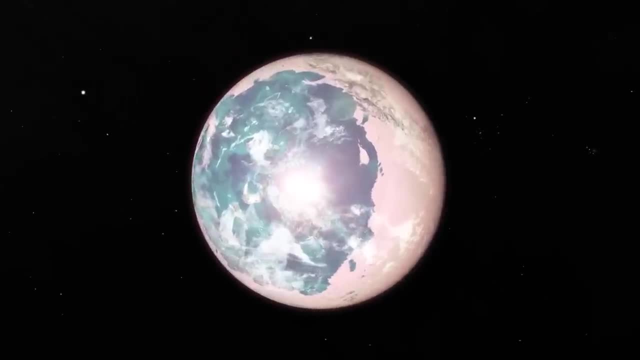 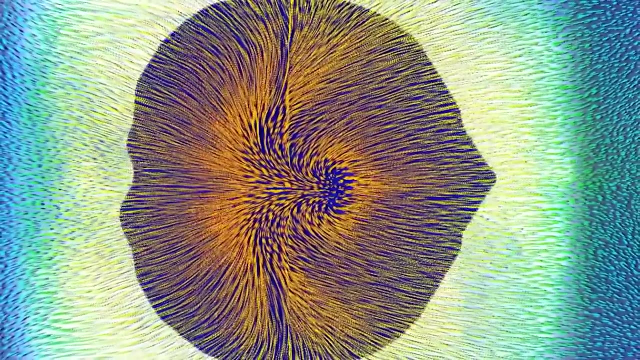 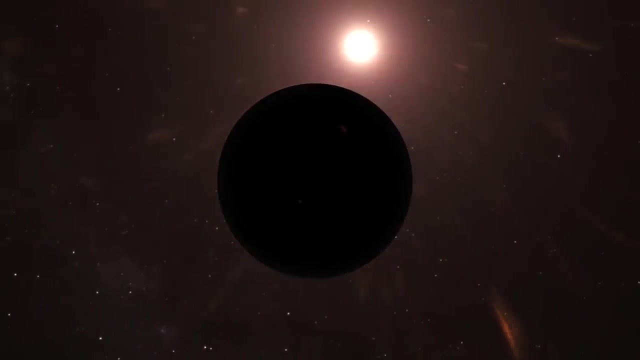 as a candidate for hosting life is its Earth-like size. Estimates of the planet's mass indicate that it is at least 1.17 times that of Earth, pointing to a rocky composition rather than a gaseous one. This similarity in size and implied composition to Earth. 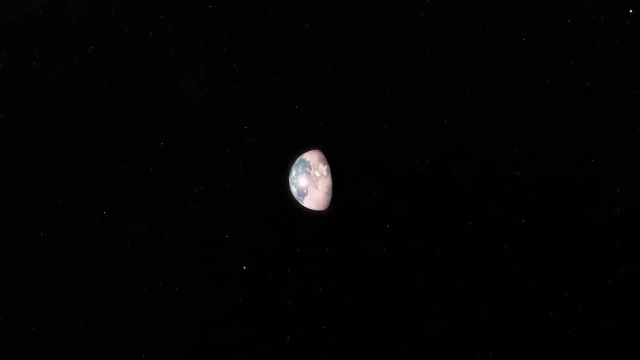 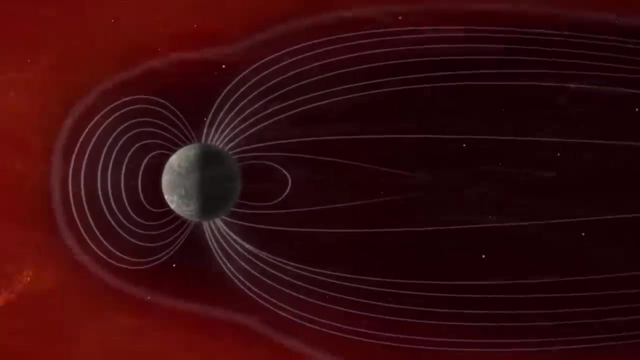 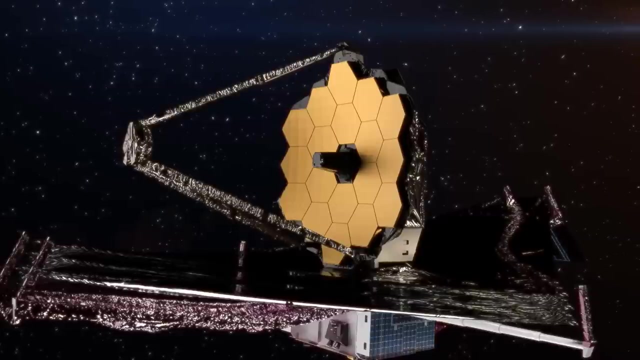 increases the likelihood that Proxima Centauri b could have Earth-like environmental conditions, further supporting the potential for habitability. The proximity of Proxima Centauri b to Earth offers a unique advantage for astronomical observation and study, Being the closest known exoplanet. 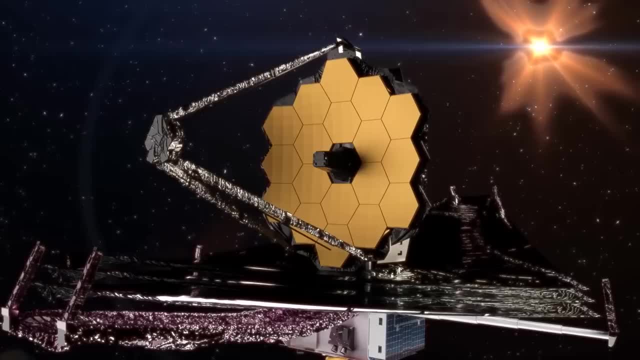 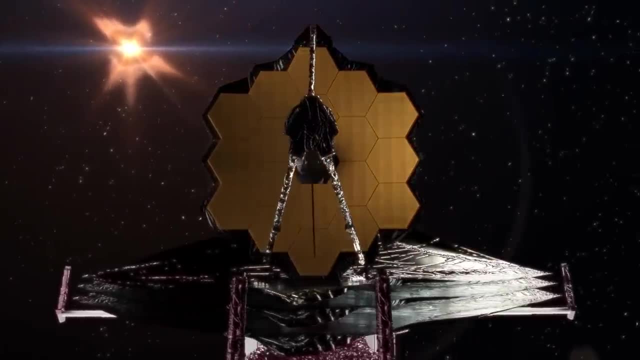 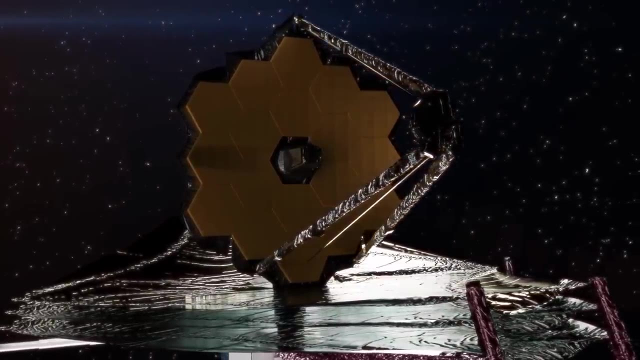 it is a prime target for future missions and telescopes designed to study exoplanetary atmospheres, surface conditions and possible biosignatures. Advanced technologies and telescopes, such as the James Webb Space Telescope, could provide the capability to analyze the chemical makeup of the planet's atmosphere. 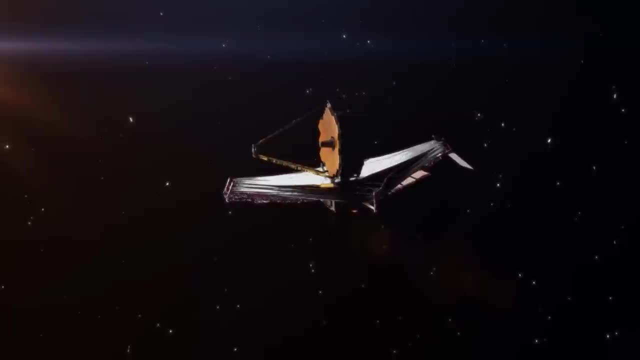 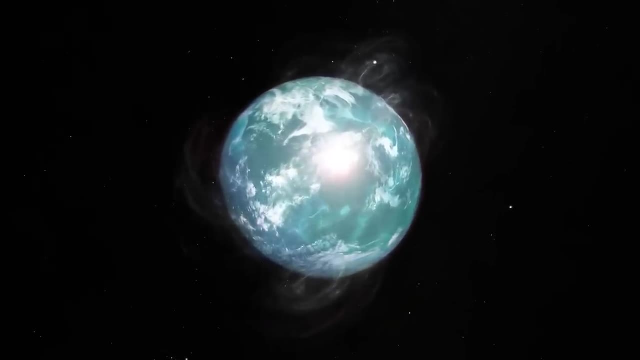 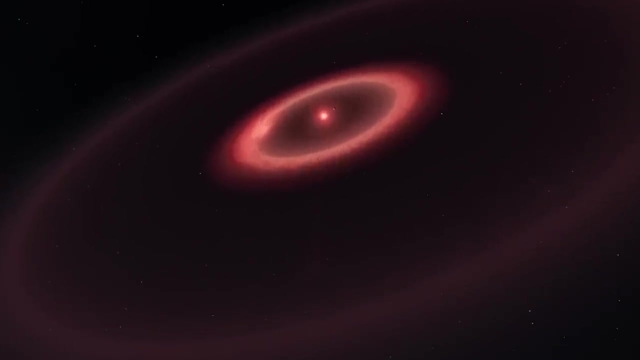 search for signs of water and detect molecules that could indicate biological processes. However, there are challenges associated with Proxima Centauri b's potential habitability. Proxima Centauri is a red dwarf star known for its stellar flares and high levels of stellar activity. 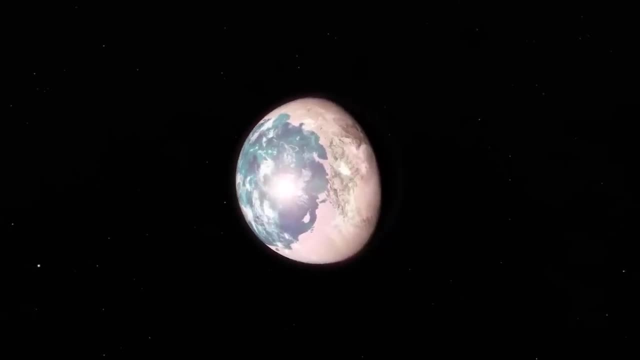 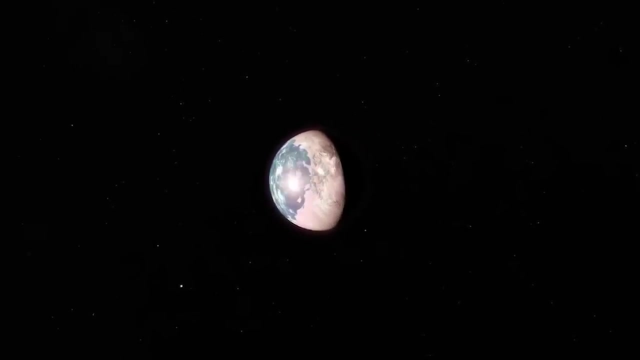 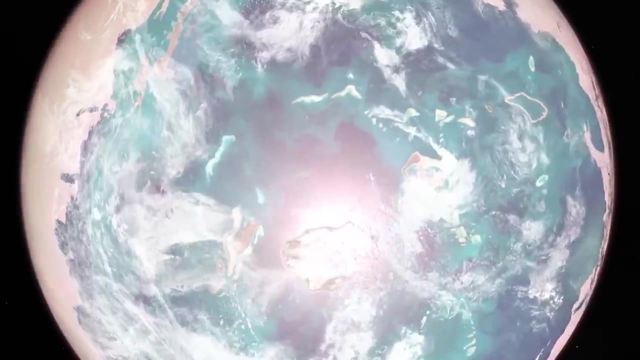 which could pose a threat to the atmosphere and surface conditions of Proxima Centauri b. For life as we know it to exist, the planet would need a robust magnetic field to protect it from the star's radiation and preserve its atmosphere. Proxima Centauri b's status as a prime candidate in the search for extraterrestrial life. 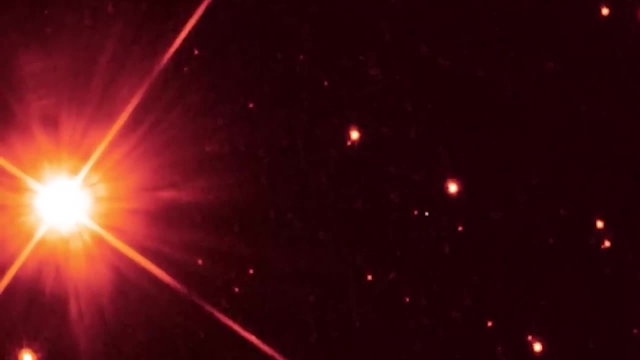 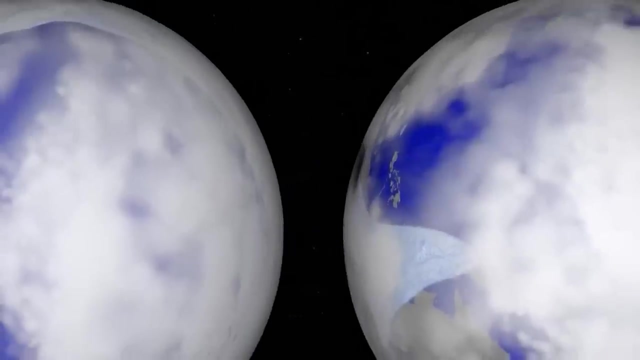 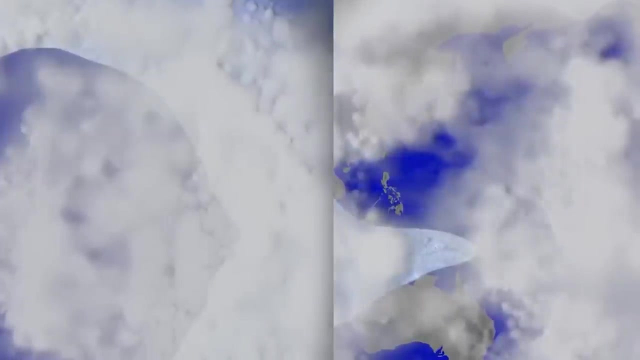 is underpinned by its orbit within the habitable zone of its star, its Earth-like size and its position as the nearest exoplanet to our solar system. These factors, combined with the potential for future direct observations, make Proxima Centauri b a focal point of interest. 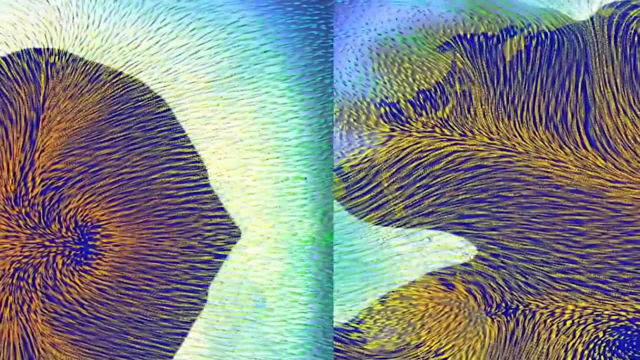 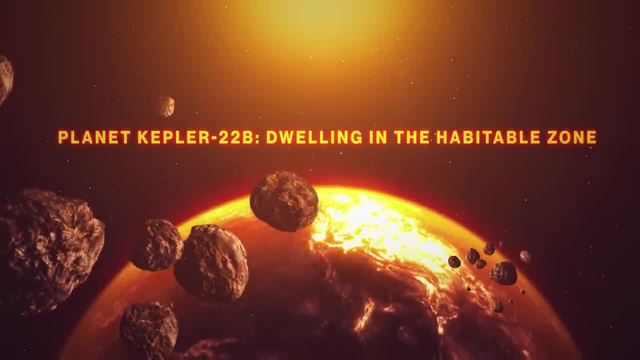 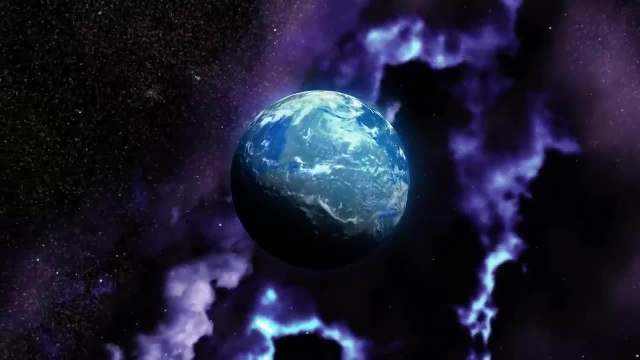 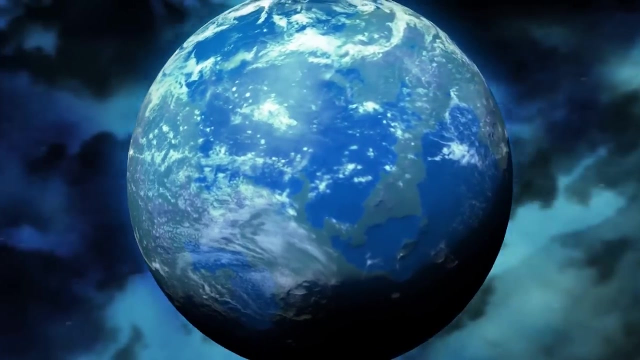 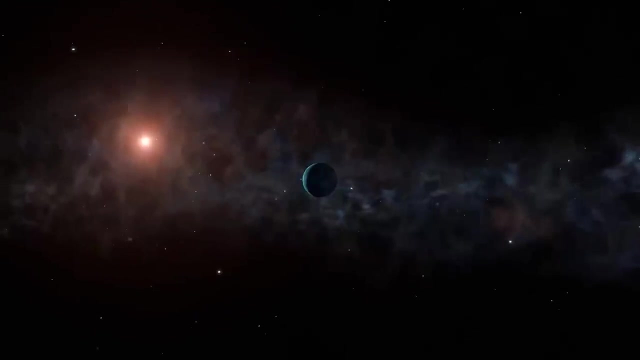 for scientists aiming to discover signs of life beyond Earth. Kepler-22b, an exoplanet discovered by NASA's Kepler Space Telescope, has sparked considerable interest in the scientific community due to several features that suggest it might be capable of supporting life Located about 620 light-years away in the constellation of Cygnus. 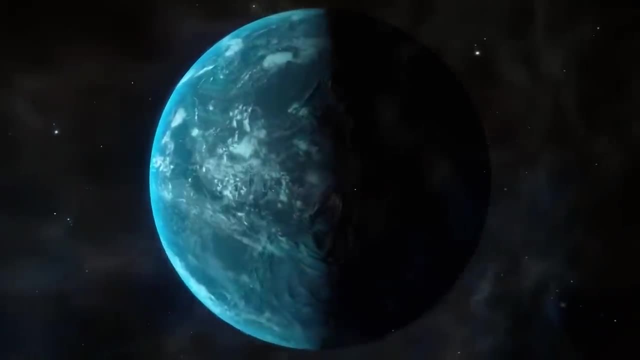 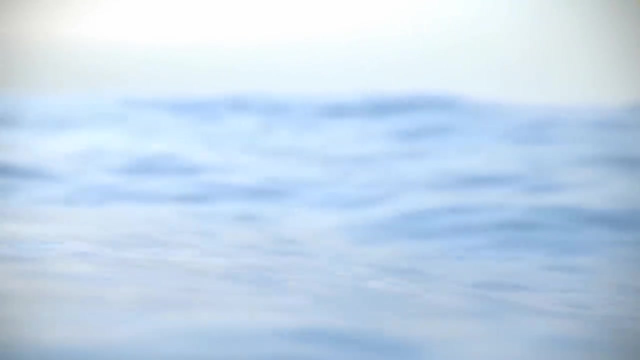 this planet orbits within the habitable zone of its star Kepler-22,, a region where conditions may allow for liquid water to exist, a fundamental requirement for life as we know it. One of the primary reasons for the interest in Kepler-22b. 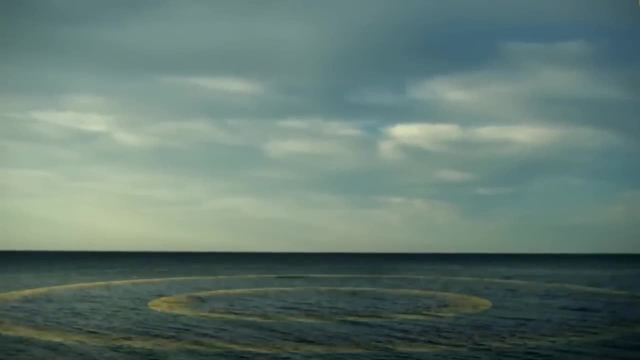 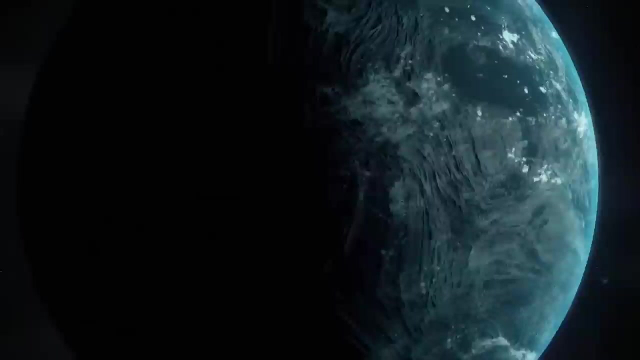 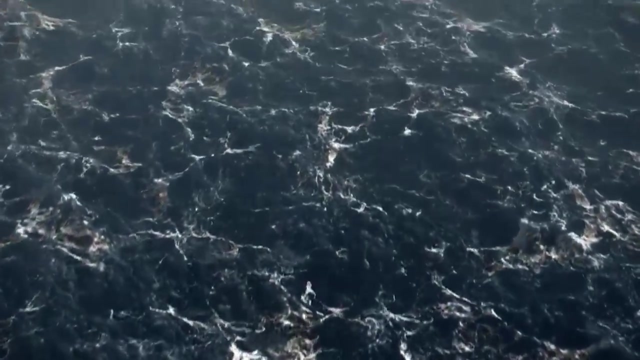 is its position in the habitable zone. This placement means the planet receives a similar amount of stellar radiation to what Earth gets from the Sun, potentially allowing for a climate that could support water in liquid form on its surface. The importance of liquid water cannot be overstated. 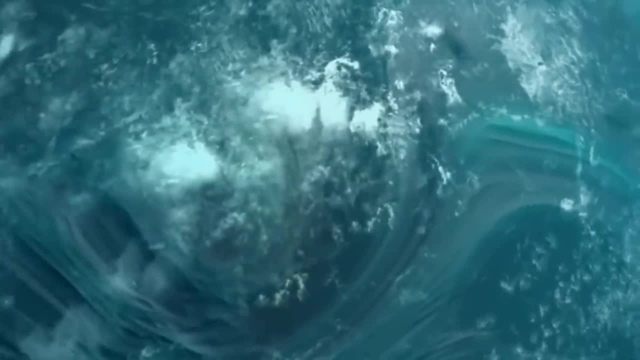 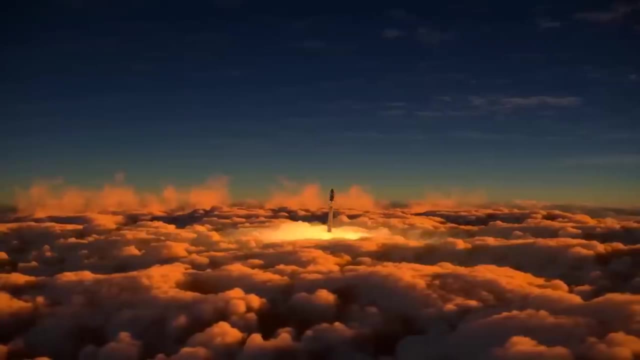 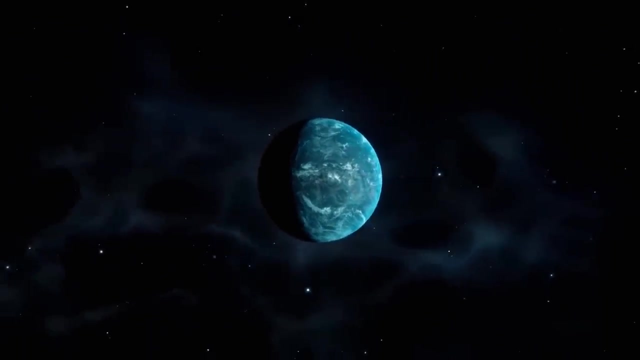 It is considered a critical ingredient for the biochemical processes known to sustain life. Furthermore, Kepler-22b is approximately 2.4 times the radius of Earth, Categorising it as a super-Earth, While its mass and composition remain uncertain due to the limitations of current observational techniques. 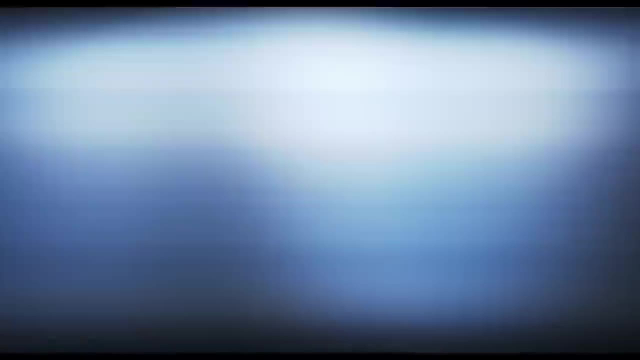 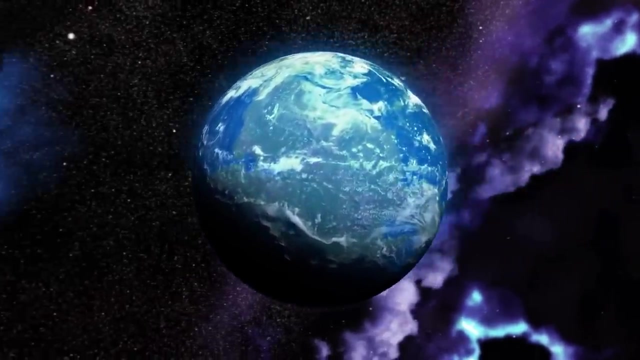 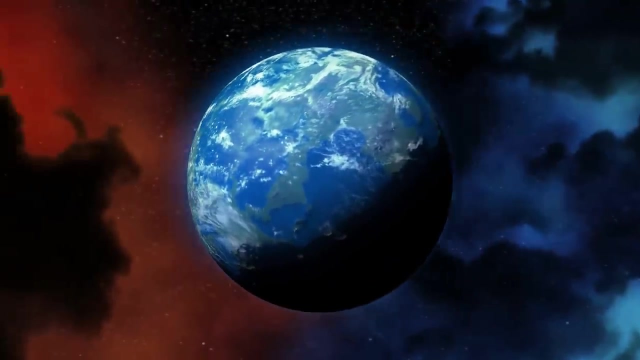 the possibility exists that Kepler-22b has a rocky surface or a surface covered by a global ocean, a scenario that could be conducive to life. The concept of a planet covered in liquid water without any land breaking the surface opens up intriguing possibilities for aquatic life forms. 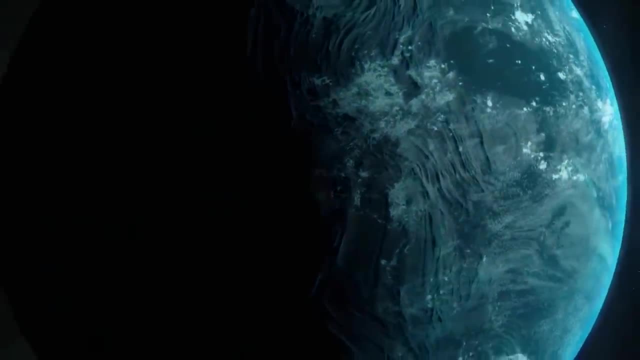 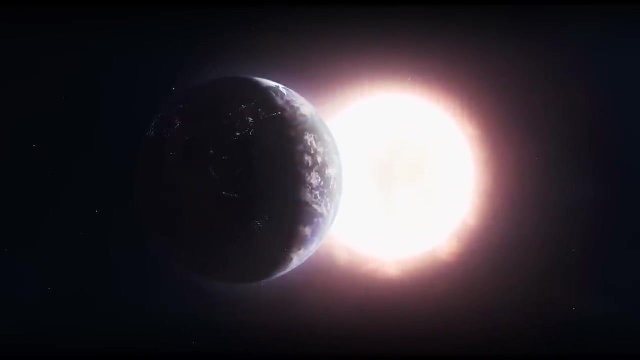 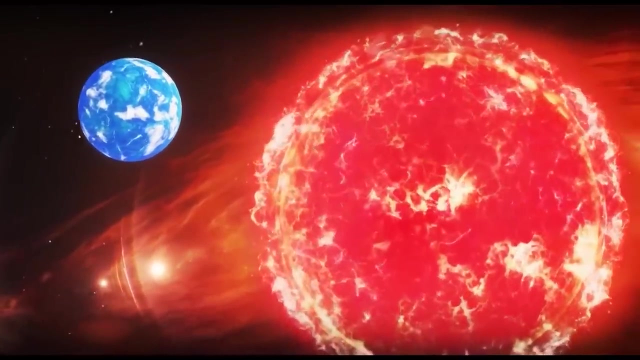 The star Kepler-22 itself also plays a role in the potential habitability of Kepler-22b. It is a G-type star, similar to the Sun, though slightly smaller and cooler. The stability and characteristics of G-type stars are thought to be conducive to the development of life. 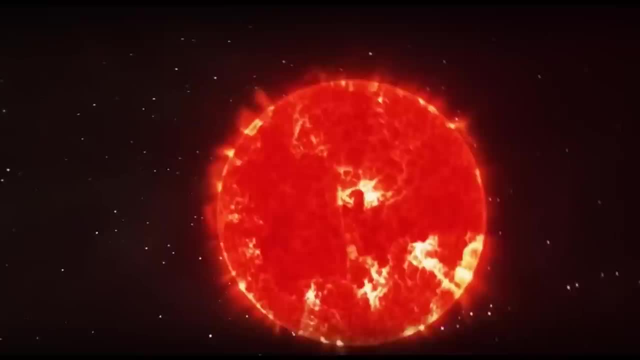 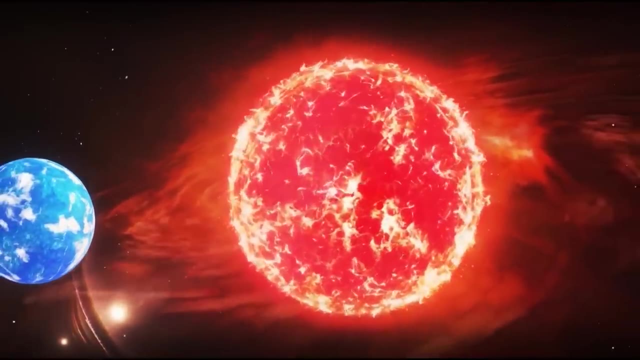 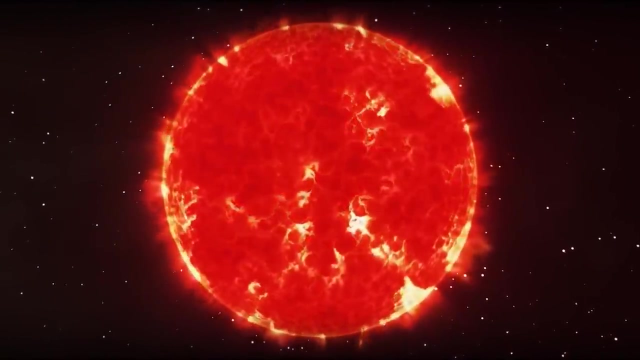 given that they provide a consistent and long-lasting source of energy. The relatively gentle stellar environment compared to more volatile star types such as red dwarfs, known for their powerful flares, suggests that Kepler-22b could maintain a stable atmosphere. However, the capacity of Kepler-22b to support life 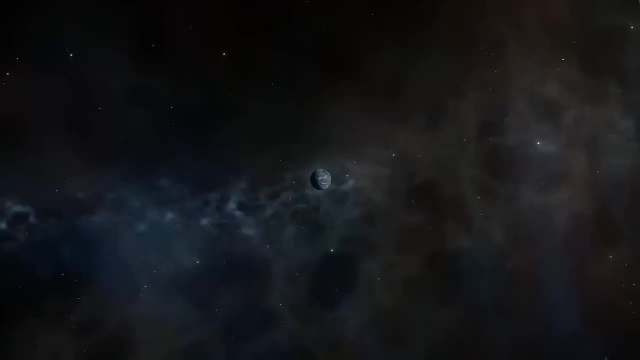 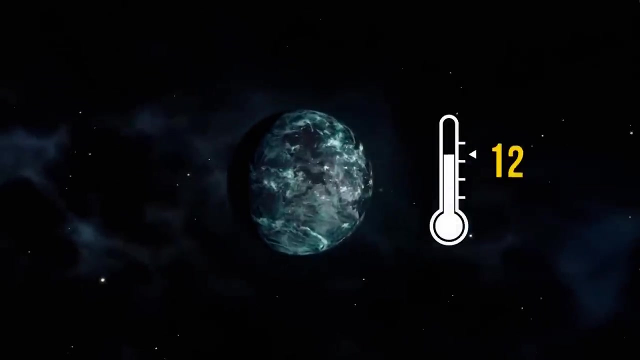 hinges not only on its location within the habitable zone and the nature of its host star, but also on its atmospheric composition, which remains unknown: An atmosphere thick enough to retain heat through a greenhouse effect, yet not so thick as to trigger runaway heating. 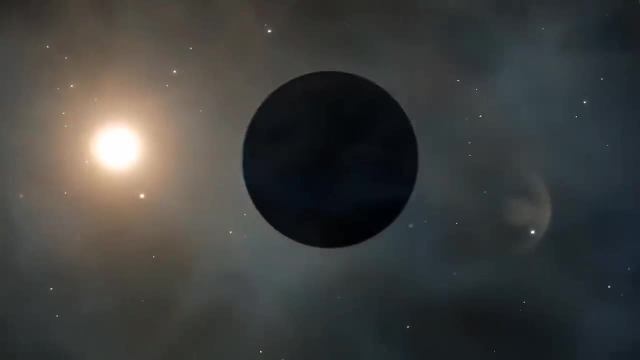 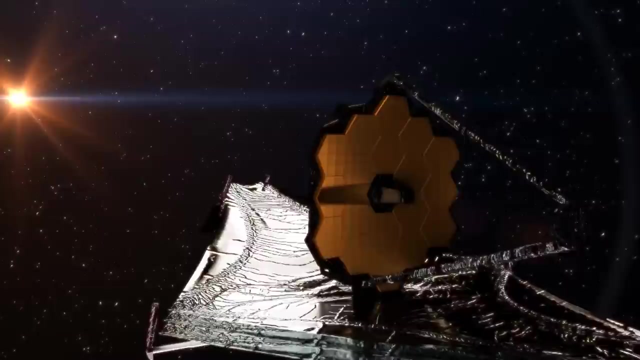 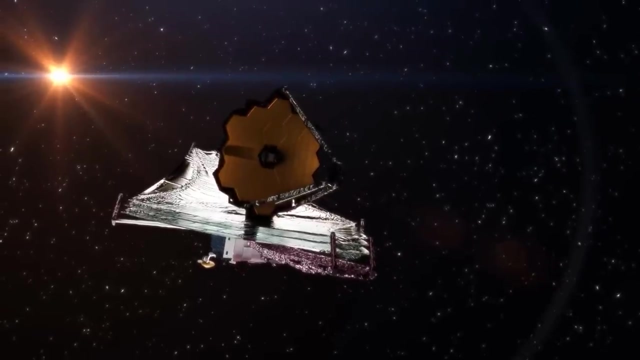 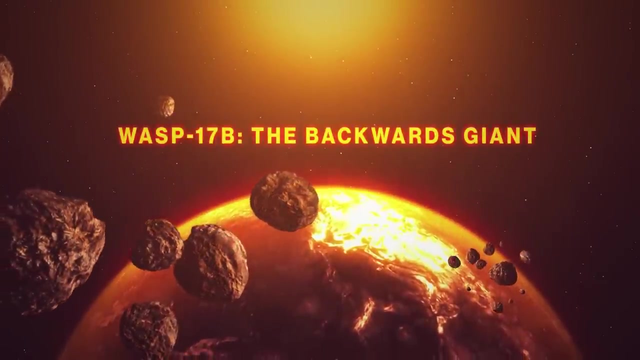 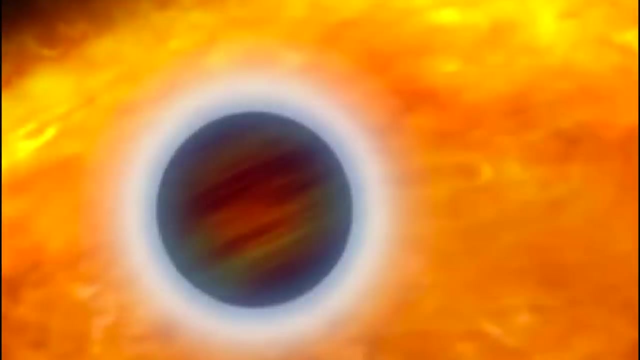 or be hostile to life would be ideal. Future observations with more advanced telescopes, like the James Webb Space Telescope, may provide insights into the atmosphere of Kepler-22b, including the presence of gases that could indicate biological activity. Planet WASP-17b, discovered in 2009,. 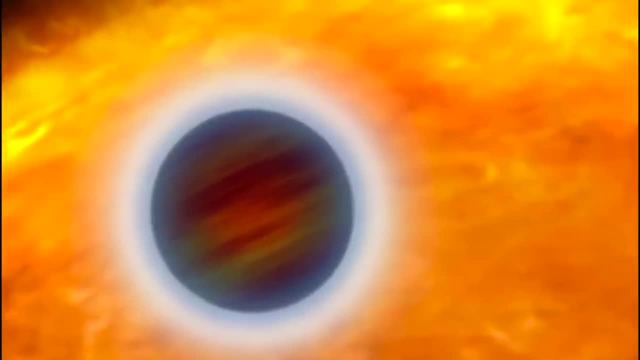 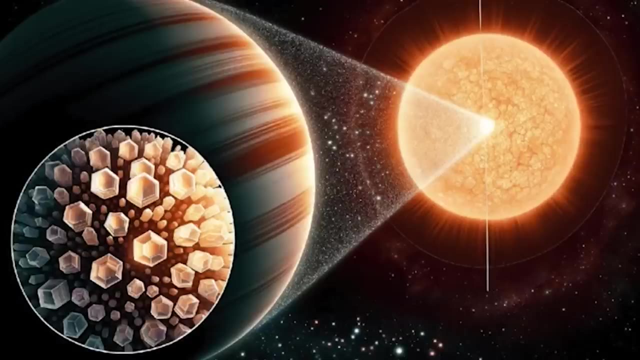 defies conventional planetary behaviour with its unique and intriguing characteristics, earning the nickname the Backwards Giant. This gas giant is located about 1,000 light-years away in the constellation Scorpius and is one of the largest exoplanets discovered, with a radius nearly twice that of Jupiter. 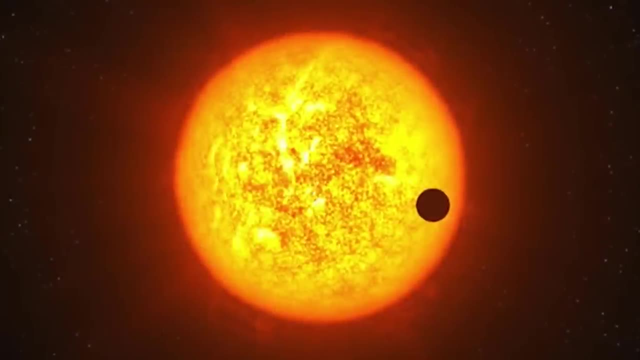 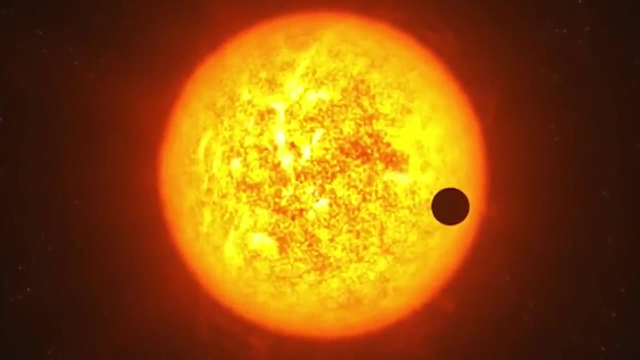 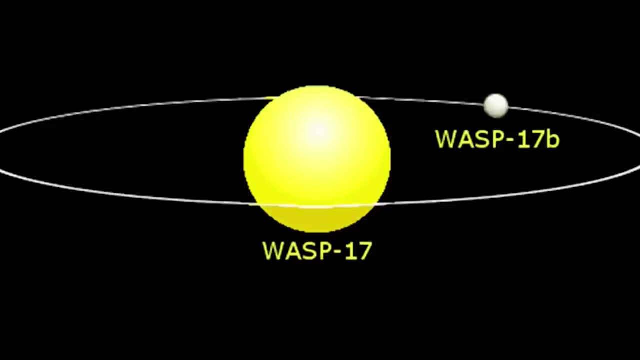 yet it has only half Jupiter's mass. This results in an exceptionally low density, likening it to a celestial puffball in space. However, what sets WASP-17b apart most distinctly is its retrograde orbit. It moves in the opposite direction to the rotation of its host star. 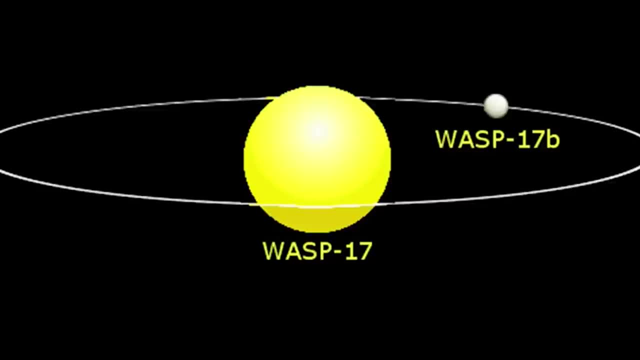 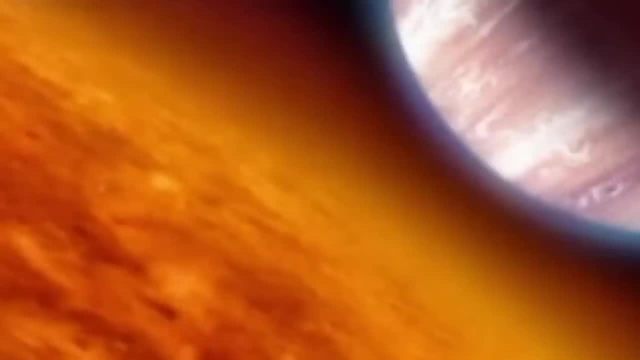 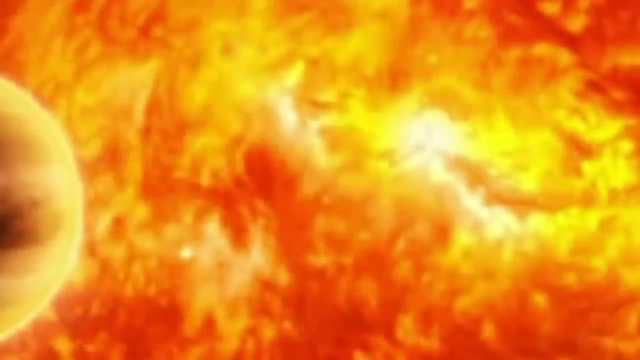 which is a rare phenomenon among the planets discovered outside our solar system. The retrograde motion of WASP-17b challenges traditional models of planetary formation and migration. According to these models, planets form from a circumstellar disk of gas and dust, and their orbits initially align with the rotation of the parent star. 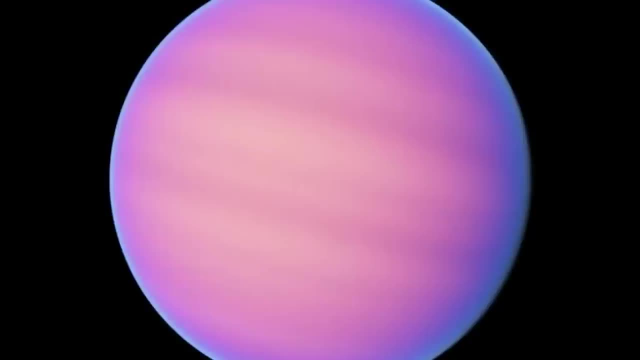 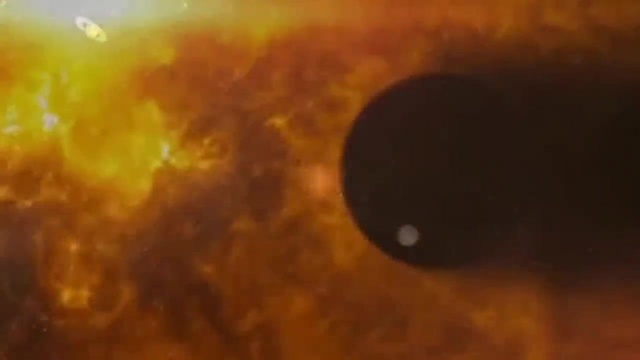 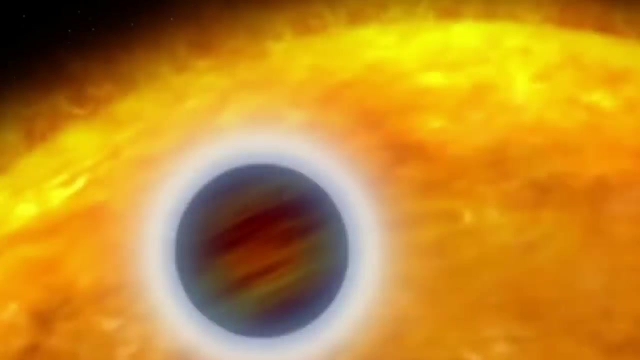 The backward orbit of WASP-17b suggests a turbulent past involving gravitational interactions with other planetary bodies or a nearby star which could have dramatically altered its original path. This might include scenarios such as close encounters with other planets leading to gravitational slingshots. 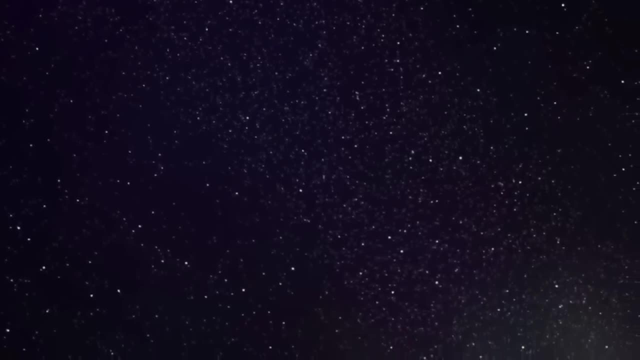 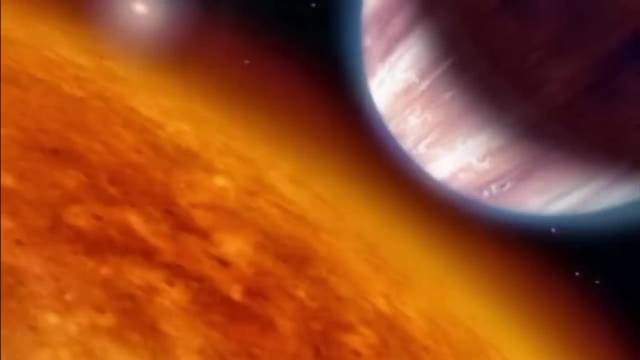 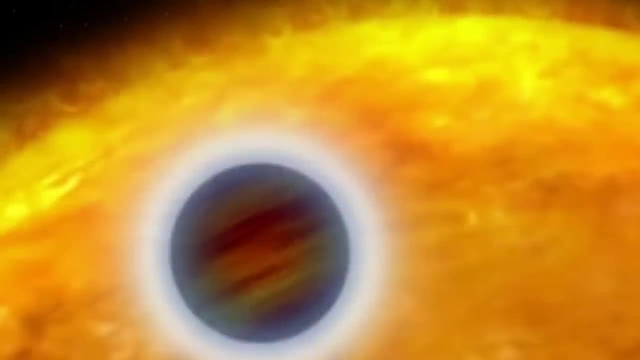 or a more gradual process known as cosi-cycles, which can exchange a planet's orbital inclination for eccentricity over time, potentially flipping its orbit in relation to the star's rotation. Another fascinating aspect of WASP-17b is its atmospheric properties. 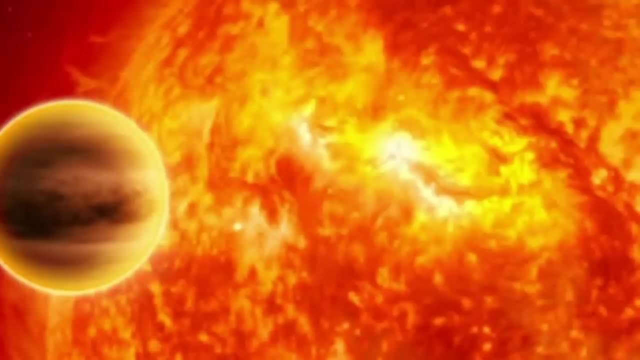 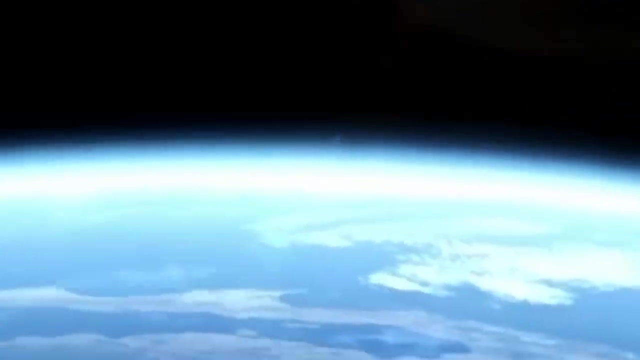 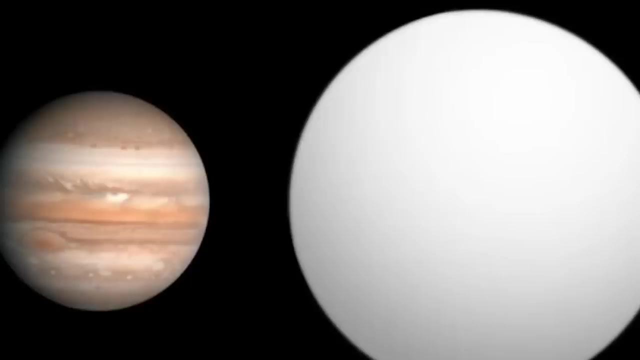 Observations indicate the presence of water vapor and possibly even carbon monoxide, but the planet's extended atmosphere and low density raise questions about its composition and the dynamics of its weather patterns. The intense radiation it receives from its close proximity to its host star could drive extreme atmospheric phenomena. 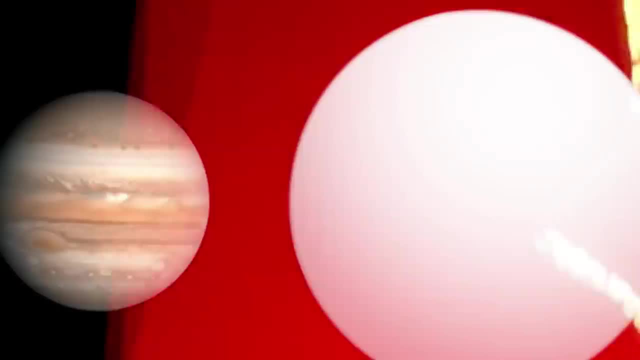 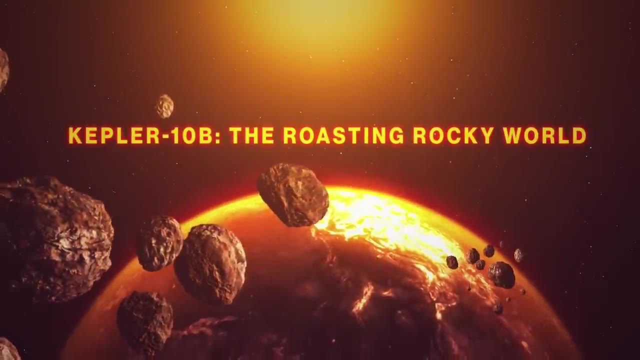 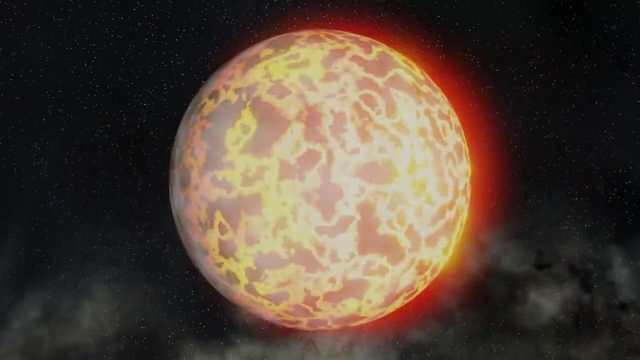 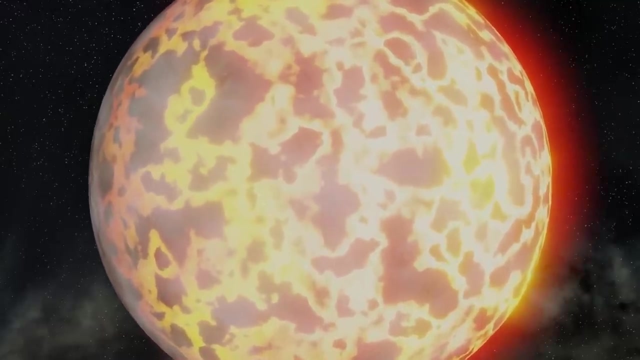 unlike anything observed in our solar system, This is the first time that a planet has been able to orbit its host star Kepler-10,. outside our solar system, Situated about 560 light-years away in the constellation Draco, this planet orbits its host star Kepler-10,. 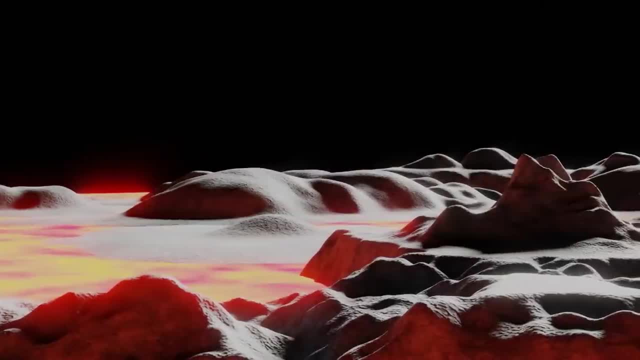 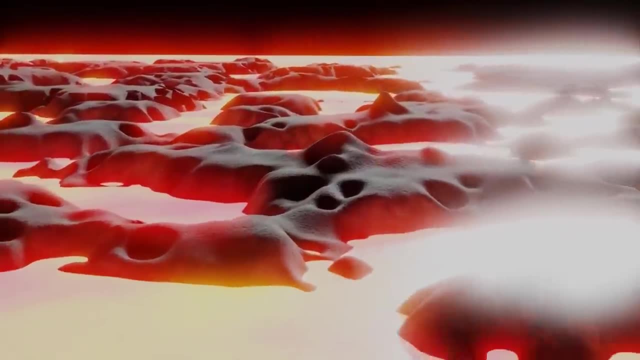 at a remarkably close distance to its star subjects Kepler-10b to extreme temperatures, earning it the nickname the Roasting Rocky World. The intense radiation from its host star heats the surface of Kepler-10b to more than 1,300 degrees Celsius. 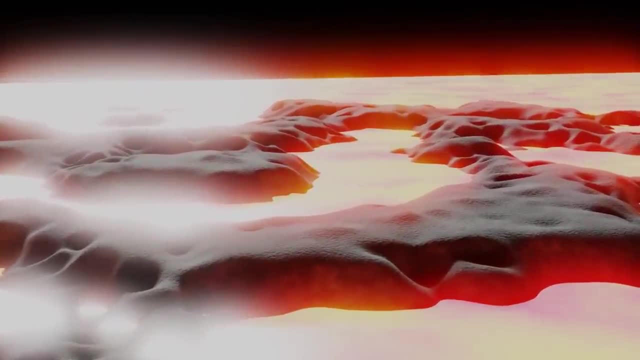 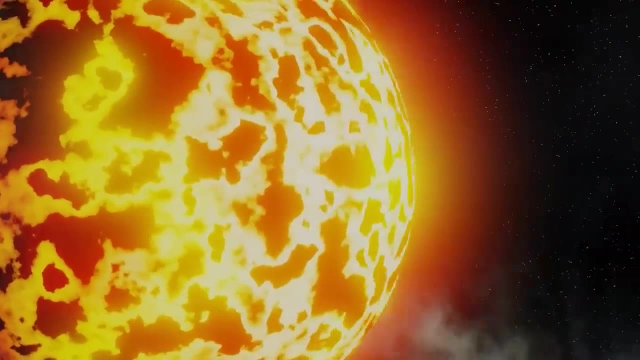 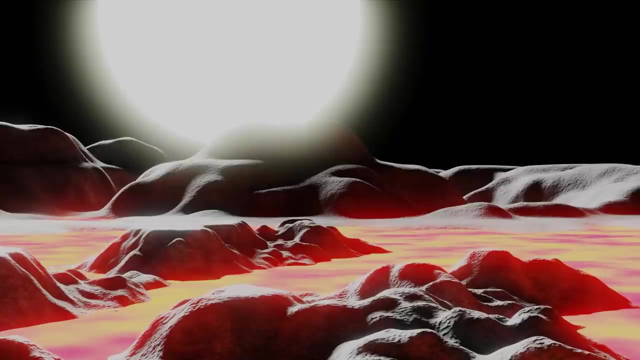 about 2,372 degrees Fahrenheit, a temperature that can melt iron and rock, creating a lava-covered landscape. This extreme heat makes Kepler-10b an unlikely candidate for hosting life as we know it, but it provides a unique laboratory for studying the compositions. 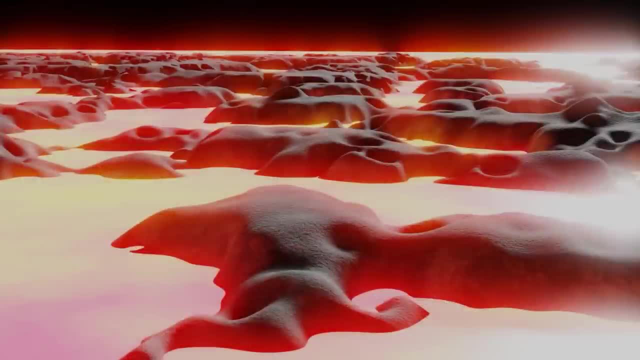 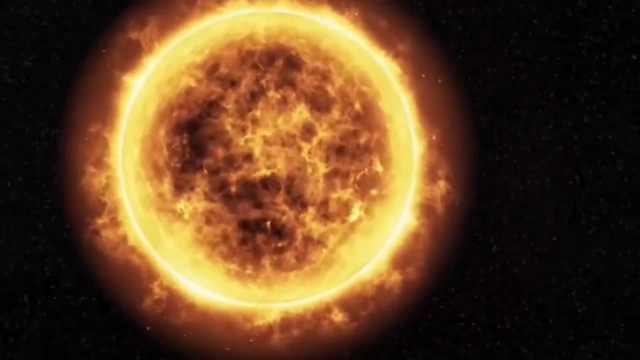 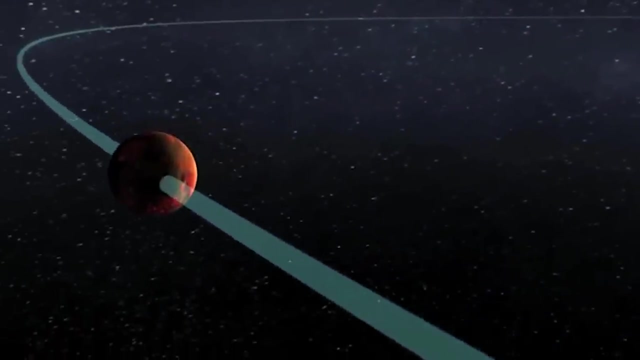 and atmospheres of rocky exoplanets, as well as the conditions under which they form and evolve. Kepler-10b's composition is primarily silicate rock, with a mass about 3.3 times that of Earth, and it has a radius 1.47 times larger. 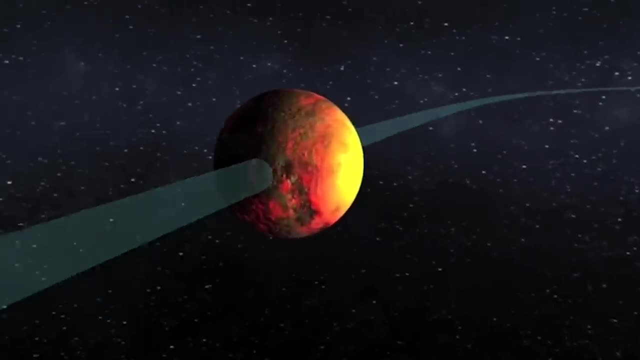 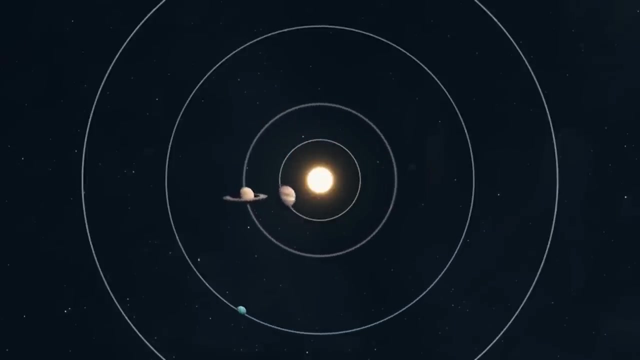 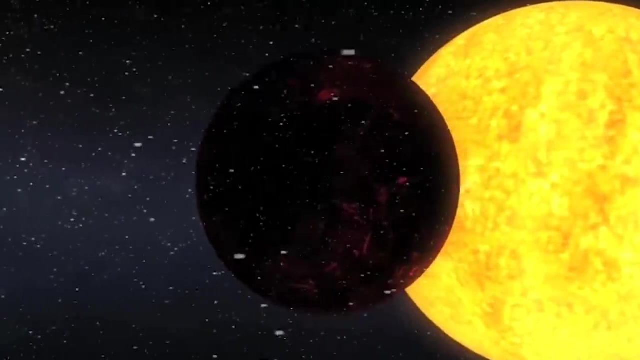 than our planet's. These characteristics confirm its status as a terrestrial or rocky planet, similar in composition to Earth, Venus, Mars and Mercury in our solar system. However, unlike the rocky planets orbiting our Sun, Kepler-10b's close orbit. 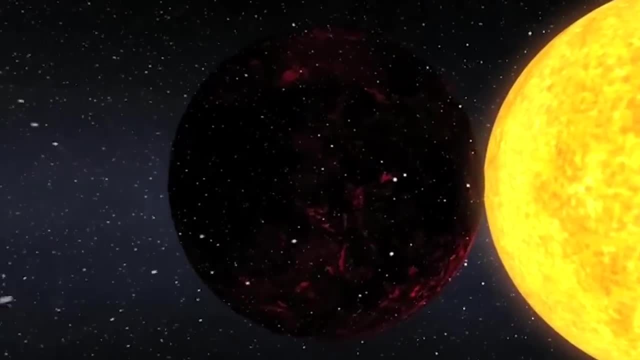 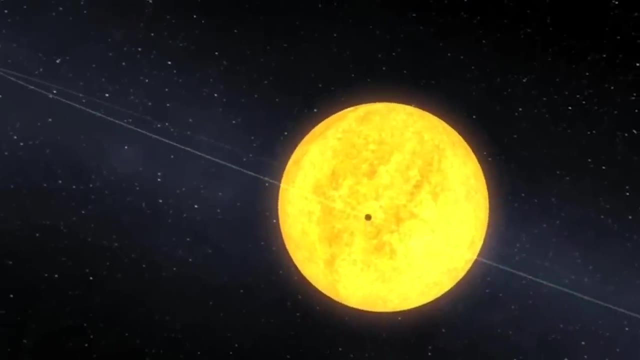 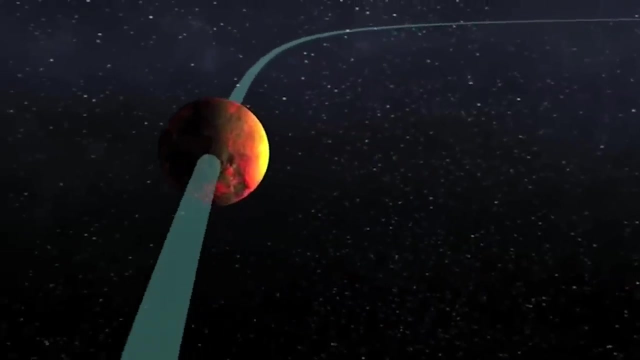 and the resulting high surface temperatures highlight the diversity of planetary environments that exist in the galaxy. The discovery of Kepler-10b was significant not only for confirming the existence of rocky exoplanets, but also for demonstrating the capabilities of the Kepler telescope and the transit method of detecting exoplanets. 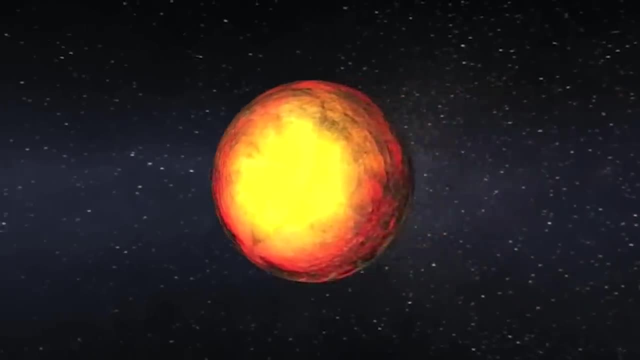 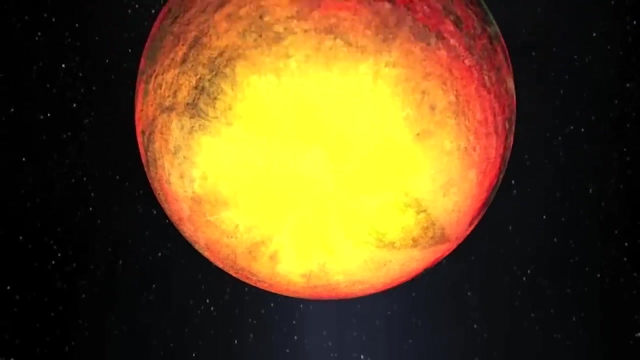 By monitoring the slight dimming of a star's light as a planet passes in front of it, astronomers can gather critical information about the planet's size, density and orbital period. In the case of Kepler-10b, these observations have provided valuable data. 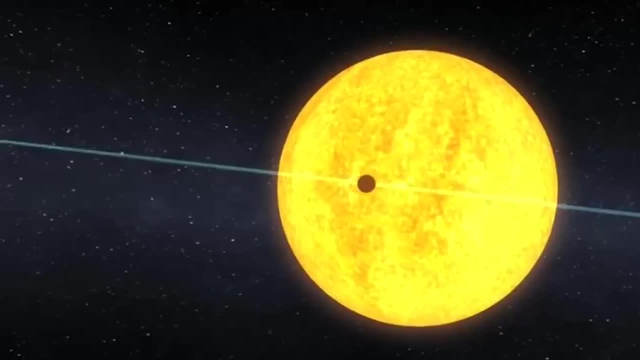 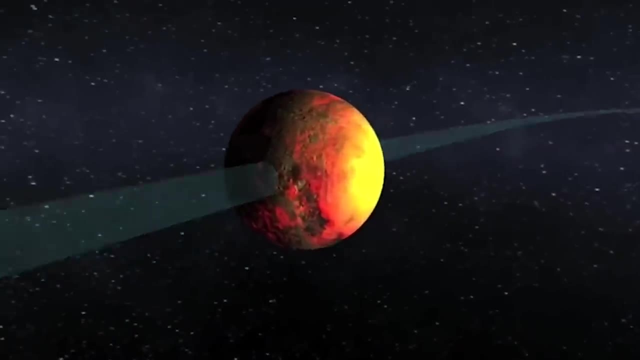 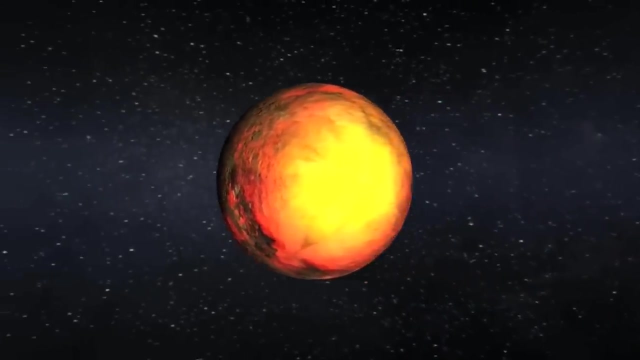 on the properties of rocky planets, including their densities, which in turn offer clues about their compositions and structures. Kepler-10b's extreme proximity to its host star also raises questions about its formation and history. It is likely that the planet formed farther out in its solar system. 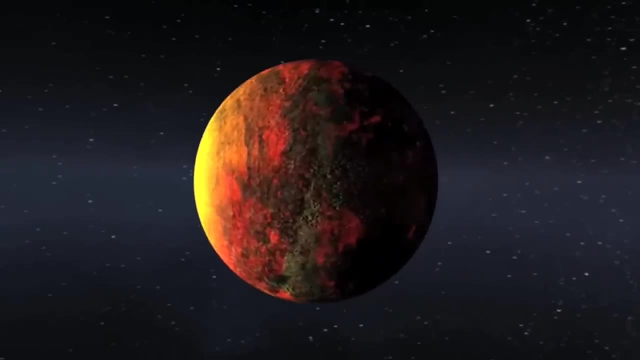 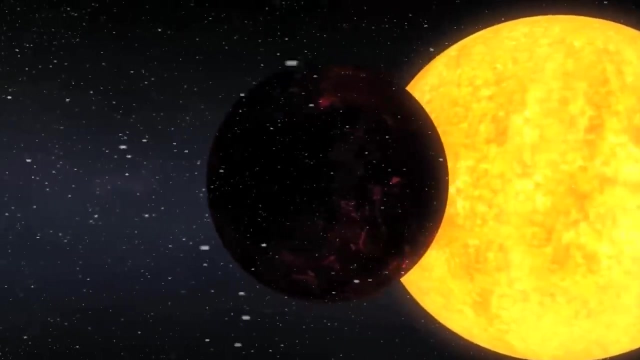 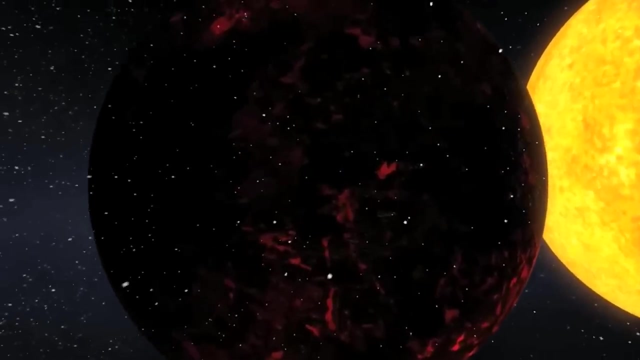 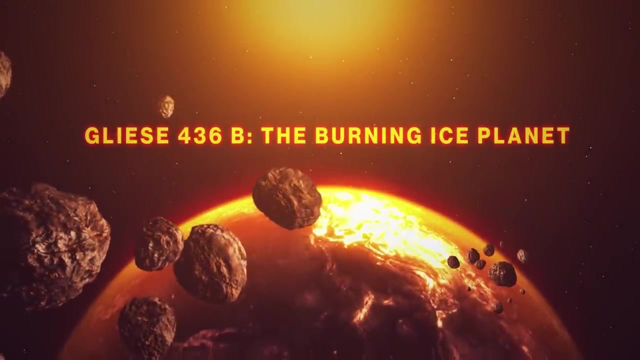 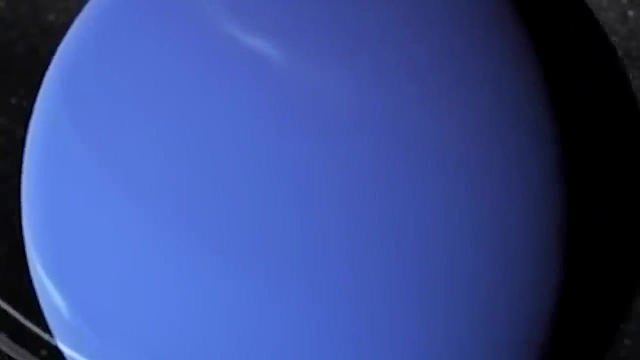 and migrated inward over time, a process that could have involved interactions with other planets or the protoplanetary disk from which it originated. Understanding these dynamic processes is crucial for piecing together the story of planetary systems, including our own. Gliese 436b. 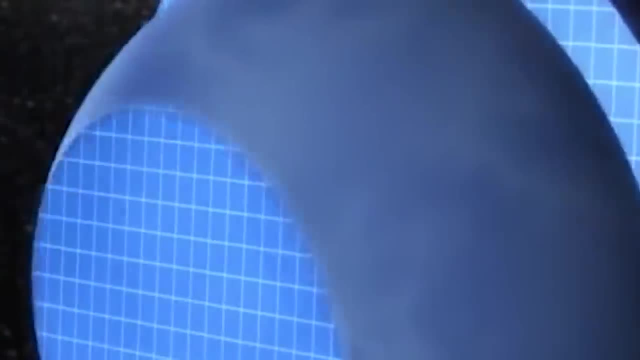 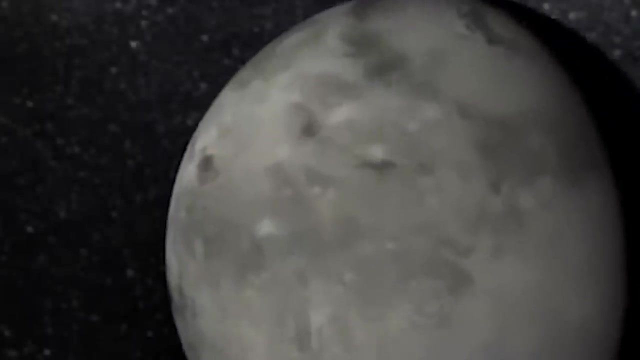 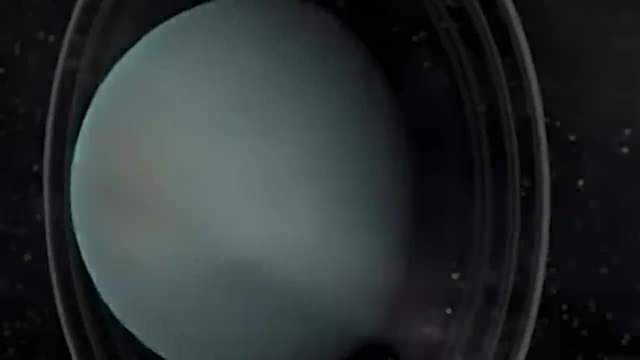 an exoplanet located about 33 light-years away in the constellation Leo, presents a paradoxical phenomenon that has intrigued astronomers since its discovery. Known as the Burning Ice Planet, this world defies traditional expectations about planetary conditions and composition, Despite orbiting very close. 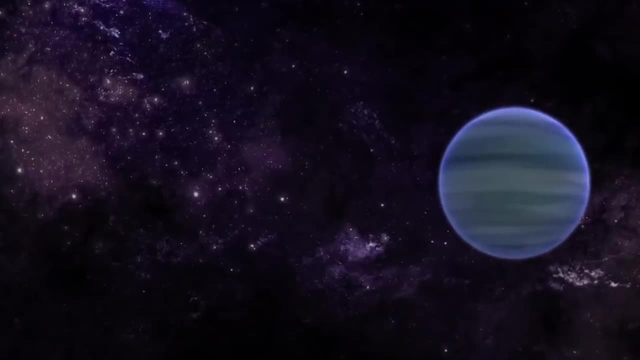 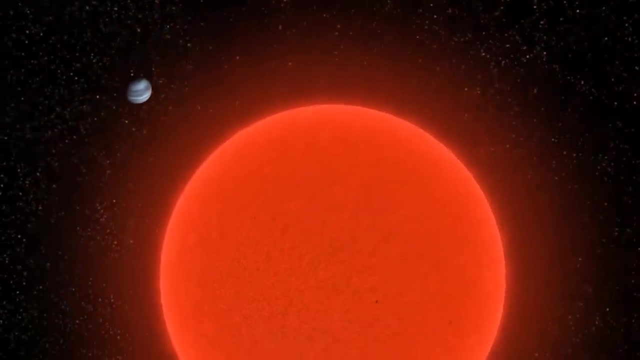 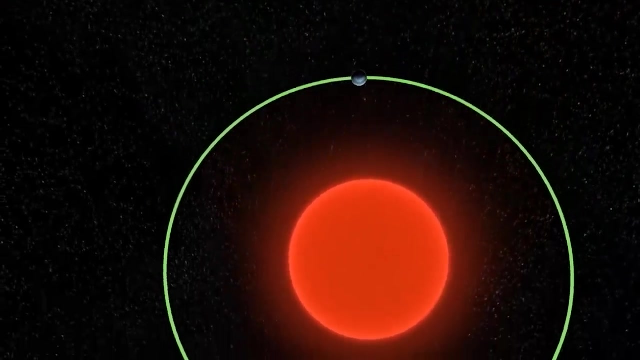 to its host star Gliese 436, with a scorchingly short orbital period of just over two days. the planet is covered in what is known as hot ice, a state of water that exists under extreme pressure and high temperature. The surface temperature of Gliese 436b. 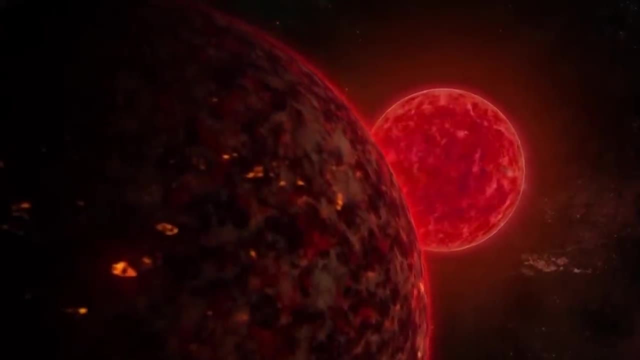 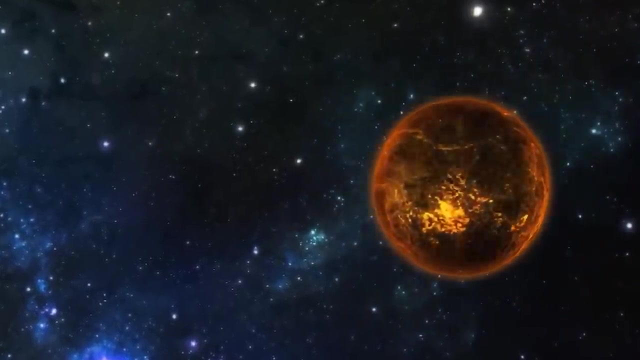 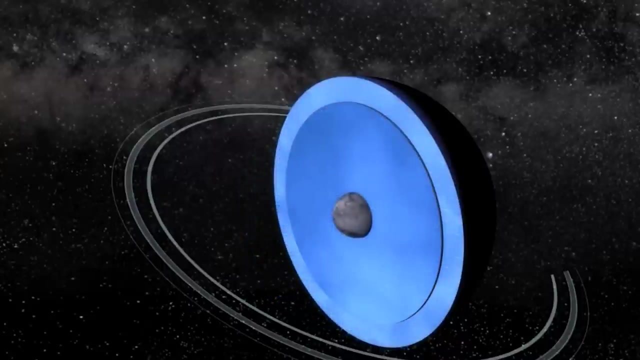 exceeds 400 degrees Celsius, 750 degrees Fahrenheit, conditions under which water would normally be expected to exist as steam. However, the immense gravitational pressure on Gliese 436b is so great that it forces the water into an exotic form of ice known as Ice X. 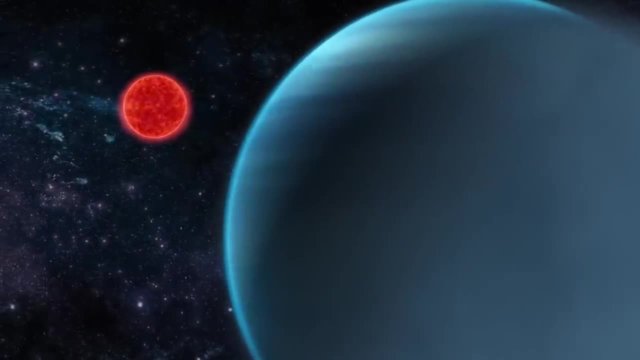 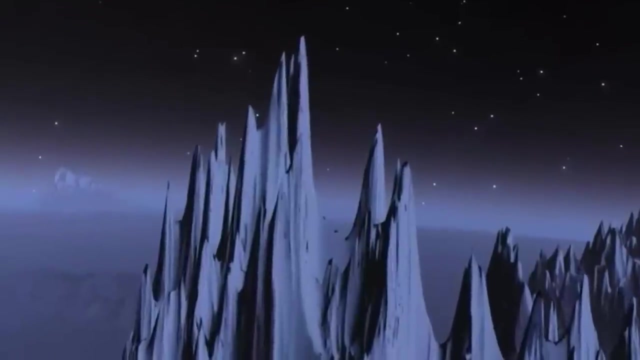 This form of ice does not melt into liquid water at higher temperatures, but remains solid due to the pressure exerted upon it, creating a scenario where ice can exist in a near-stellar environment. This peculiar state of matter on Gliese 436b. 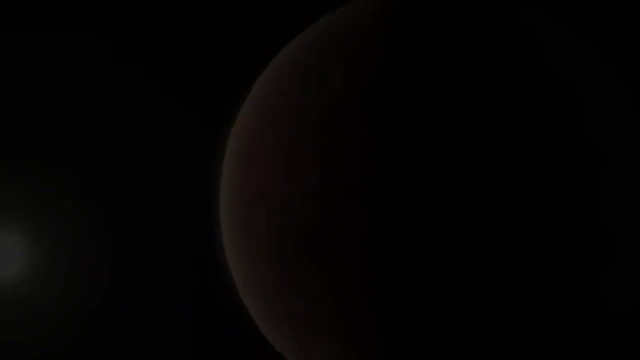 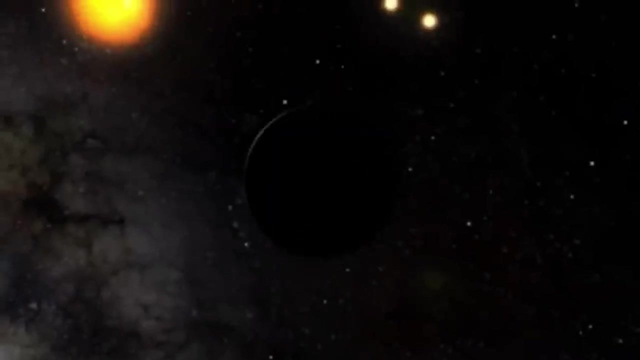 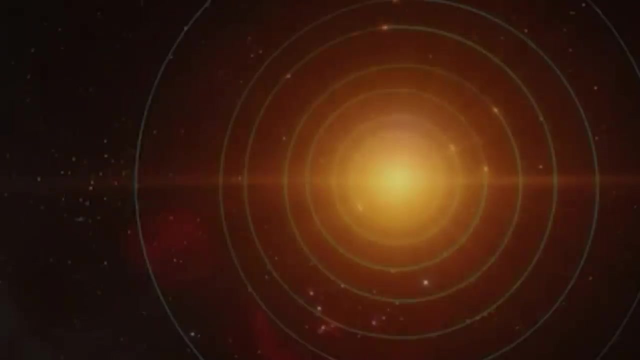 is a result of its unique atmospheric and physical characteristics. The planet's atmosphere is rich in hydrogen and helium, with traces of water vapour, which suggests that there is water present on the planet. However, due to the extreme conditions, this water does not exist in familiar states. Instead, the high temperatures and pressures transform it into hot ice and supercritical fluid, a state of matter that exhibits properties of both liquids and gases. The discovery of Gliese 436b has significantly expanded our understanding of the diversity of exoplanets and the range of conditions. 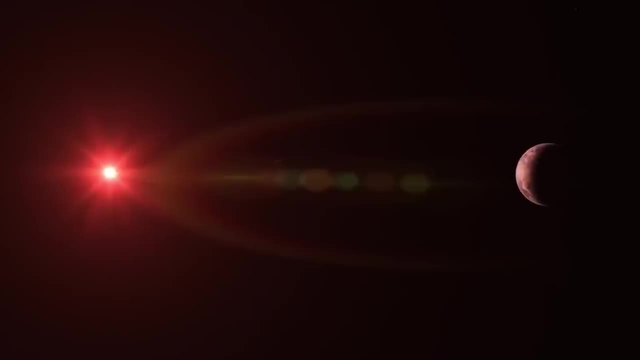 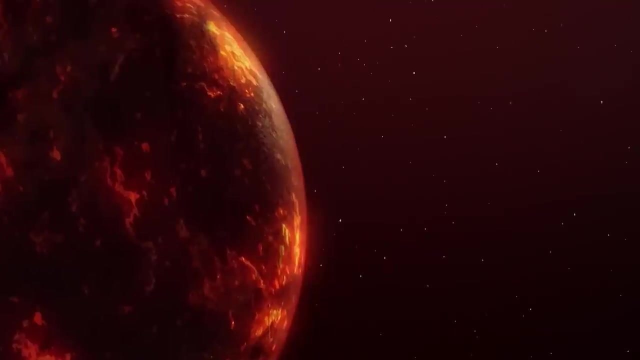 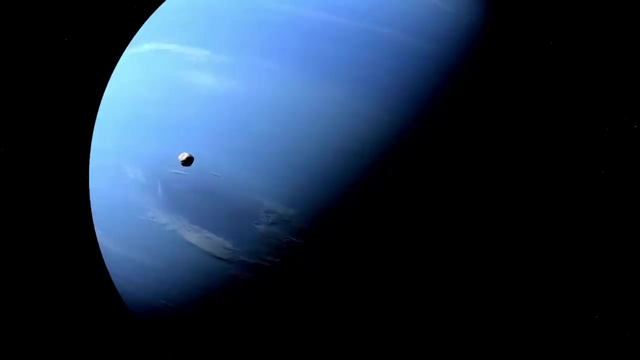 under which they can exist. It challenges preconceived notions about the behaviour of water and the conditions necessary for different states of matter to form. The existence of hot ice on Gliese 436b suggests that there may be many more planets with similarly exotic conditions. 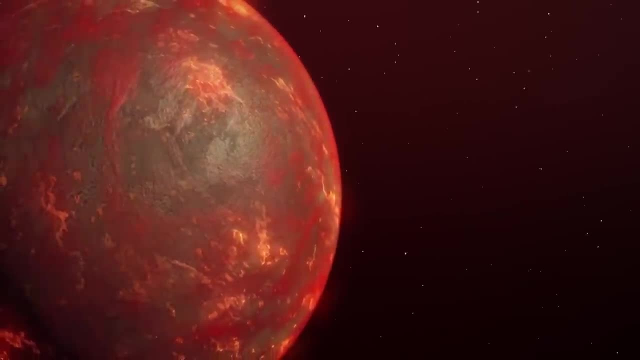 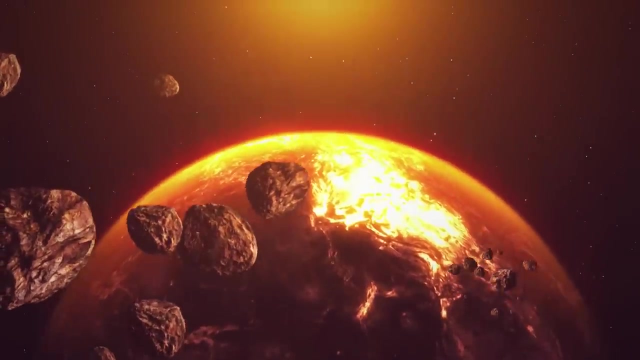 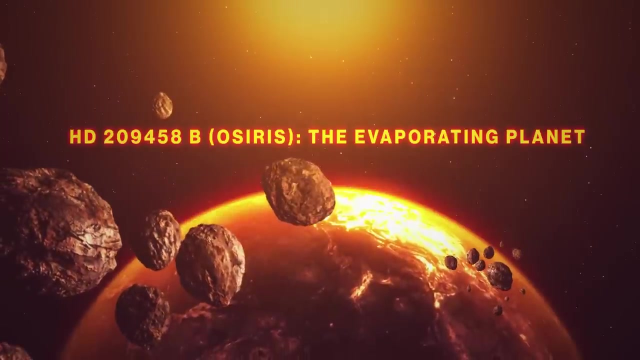 defying easy categorisation and expanding the possibilities for what conditions planets in the Universe may exhibit. Gliese 436b, also known as OSIRIS, stands out in the pantheon of exoplanets for its dramatic and visible process of evaporation. 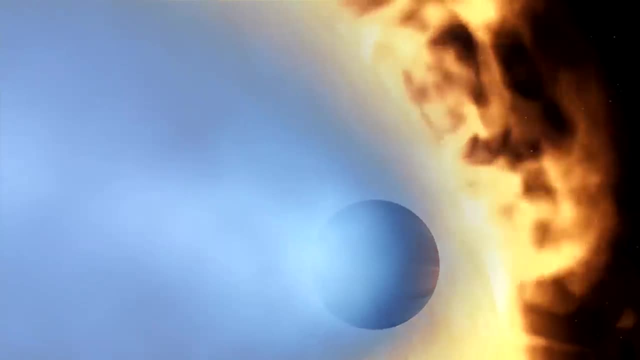 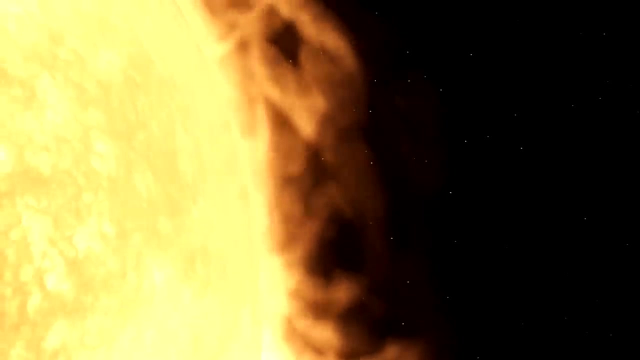 Located about 150 light-years away in the constellation Pegasus. this gas giant orbits its host star at a distance of 1,000 light-years. Gliese 436b, also known as OSIRIS, stands out in the pantheon of exoplanets. 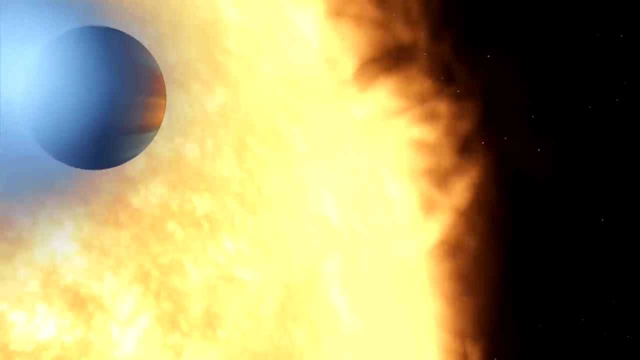 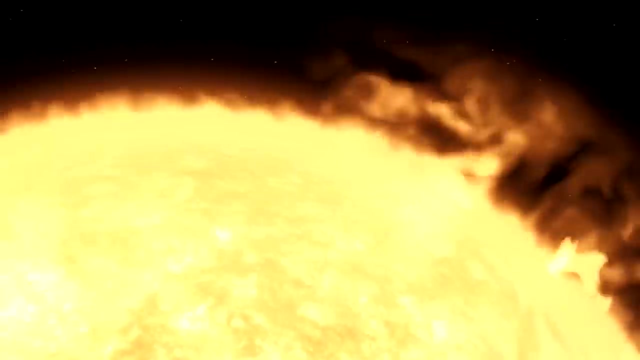 for its dramatic and visible process of evaporation. Located about 150 light-years away in the constellation Pegasus, this gas giant orbits its host star at a mere eighth of the distance that separates Earth from the Sun, leading to extremely high surface temperatures, exceeding 1,000 degrees Celsius. 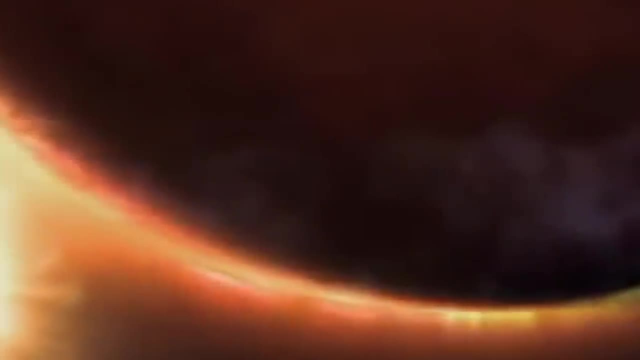 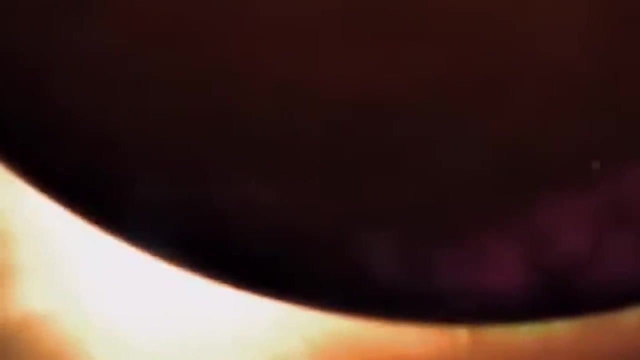 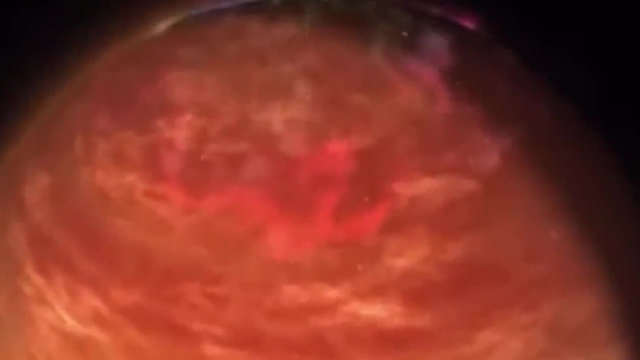 about 1,832 degrees Fahrenheit. This close proximity to its star subjects, HD 209458b, to intense stellar radiation, causing its atmosphere to heat up and expand to the point where it starts to escape into space. The phenomenon of atmospheric escape in the constellation HD 209458b. 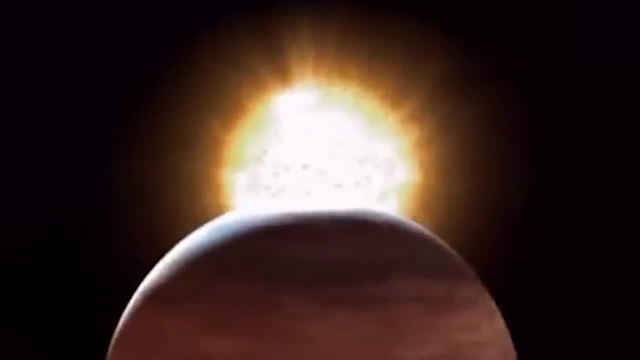 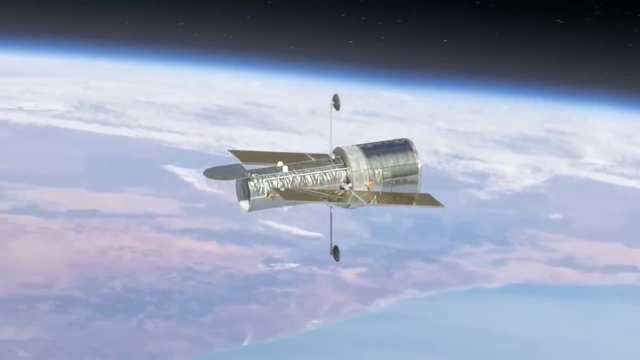 was among the first of its kind to be observed directly Using the Hubble Space Telescope. astronomers detected hydrogen, carbon and oxygen being blown off the planet at speeds of thousands of kilometers per hour, creating a vast tail of material trailing behind the planet. 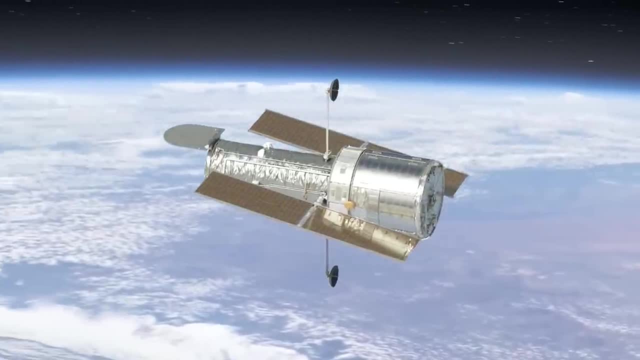 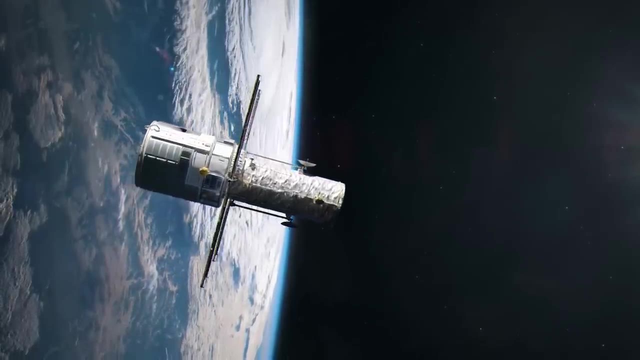 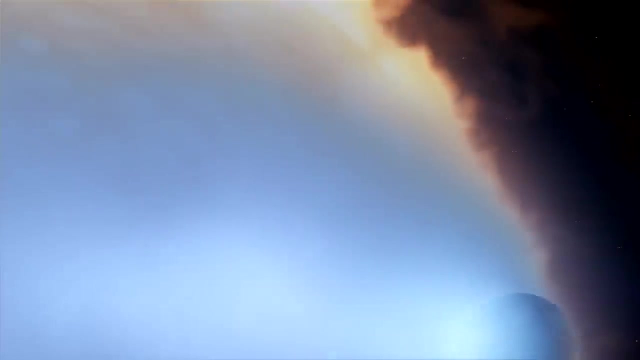 much like a comet. This escape process is so significant that it is estimated the planet may lose about 100 million to 500 million kilograms of mass. The evaporation of HD 209458b provides critical insights into the interactions between exoplanets and their host stars. 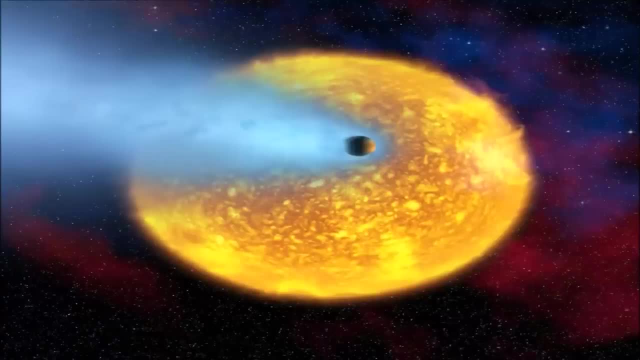 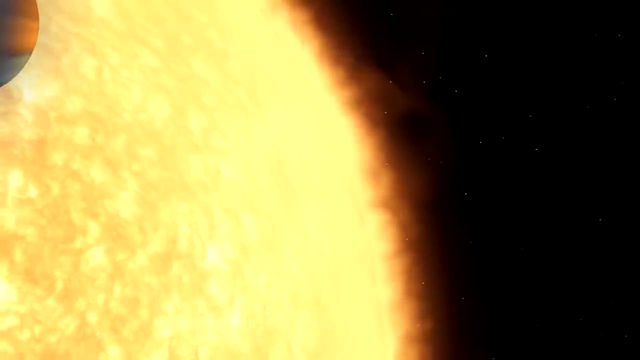 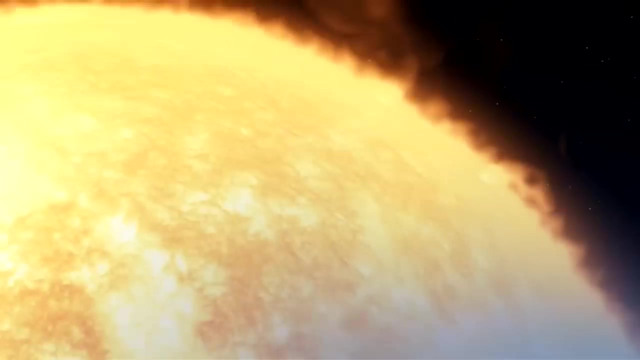 particularly in cases where planets are located in close orbits. The intense radiation that drives the atmospheric escape on OSIRIS is also responsible for ionizing the escaping gases, which then interact with the star's light to produce the observable signatures that led to the detection of this phenomenon. 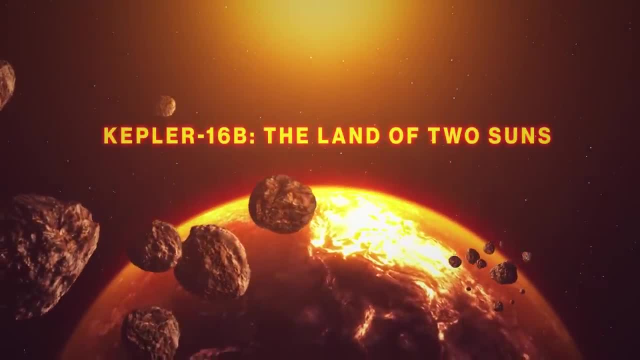 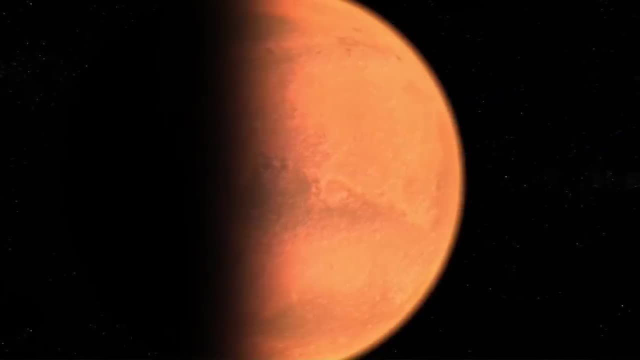 The Hubble Space Telescope is the world's largest observable satellite. It is the world's largest observable satellite. It is the world's largest observable satellite- Kepler-16b, an exoplanet located about 200 light years away in the constellation Cygnus. 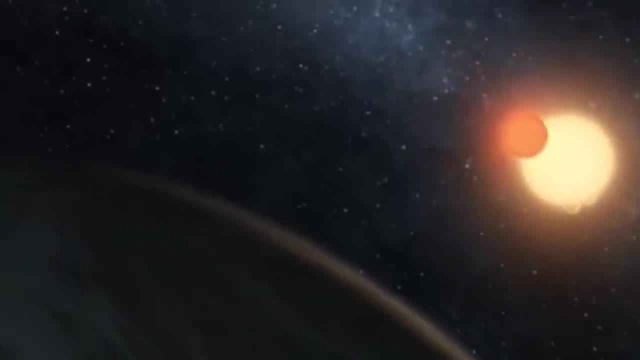 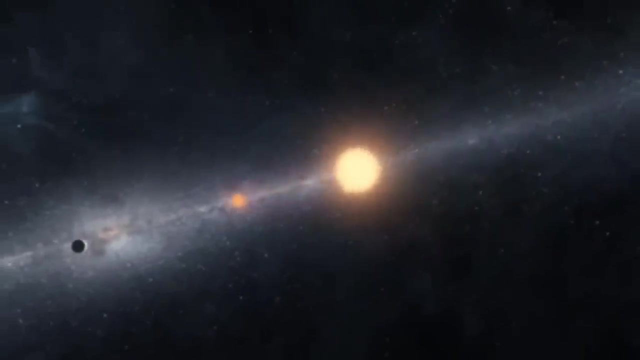 offers a glimpse into a world that seems as though it was plucked from the realms of science fiction. Known as the Land of Two Suns, this planet is distinguished by its orbit around a binary star system, making it the first confirmed circumbinary planet. a planet that orbits two stars instead of just one. This unique celestial configuration results in Kepler-16b experiencing a double sunset and sunrise, reminiscent of iconic scenes from the Star Wars saga. The discovery of Kepler-16b was made possible by NASA's Kepler Space Telescope. 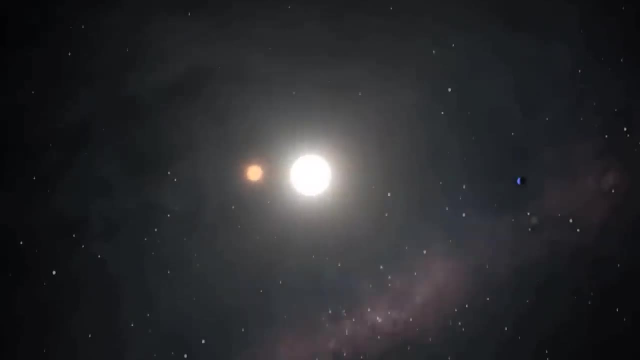 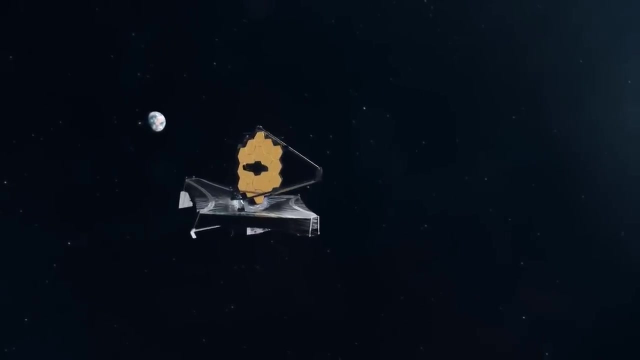 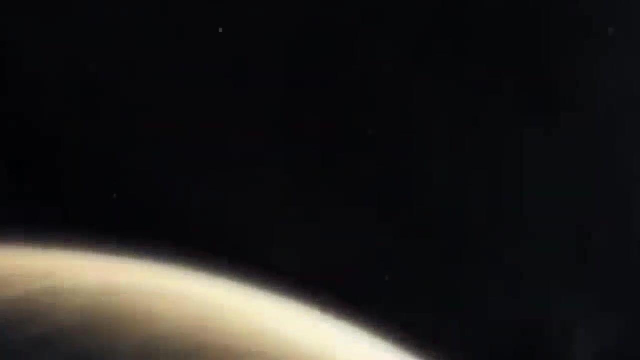 which detected the planet using the transit method. This method involves observing the dimming of starlight as a planet passes in front of its host stars from the perspective of the telescope. Kepler-16b's transits revealed not only its existence: 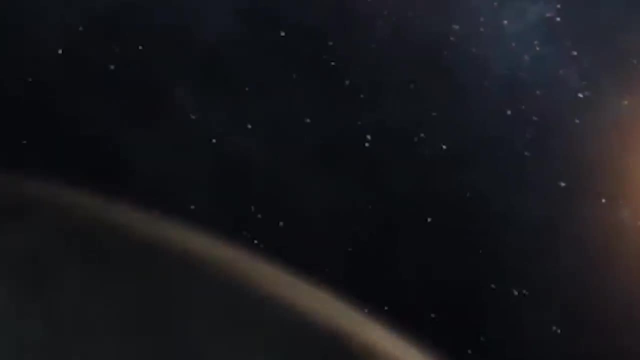 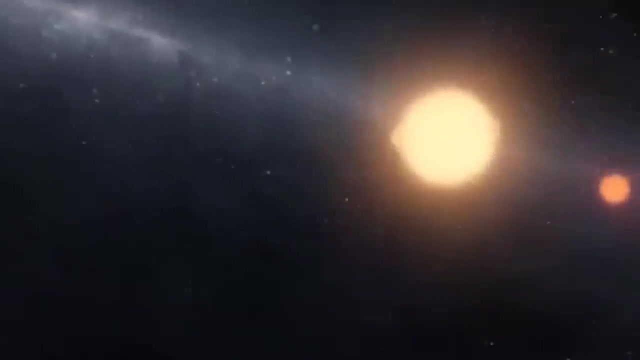 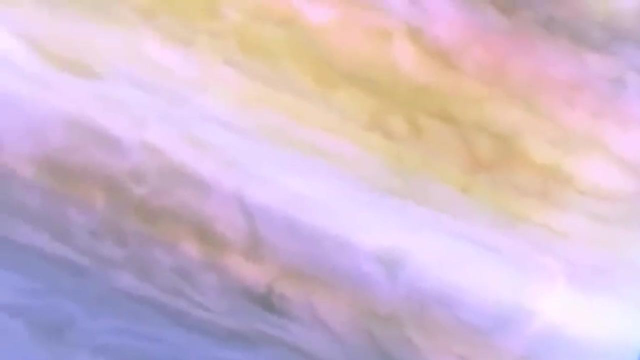 but also its remarkable orbit around both members of a closely orbiting pair of stars, one slightly smaller than the Sun and the other much smaller, cooler and redder. Kepler-16b is approximately the size of Saturn, a radius that suggests a composition of gas. 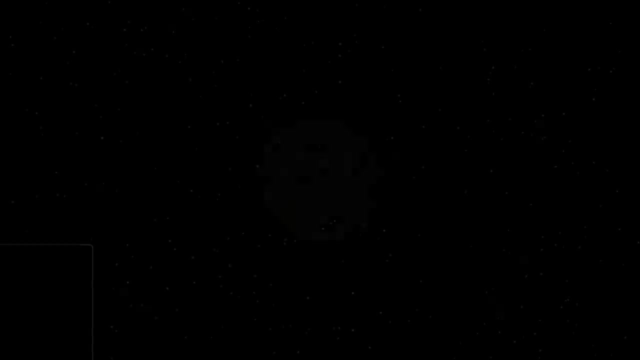 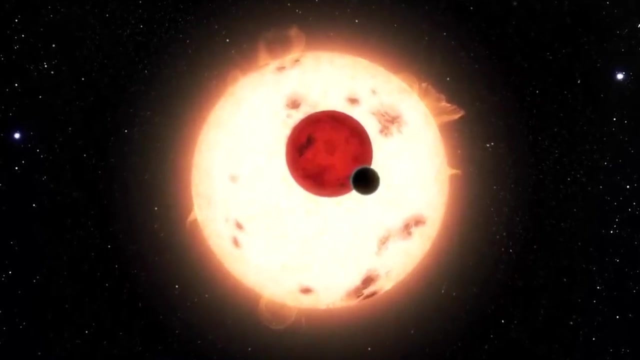 possibly with a rocky core. Its orbit around the binary stars takes about 229 days, a distance that places it outside the habitable zone of its star system, suggesting that temperatures on Kepler-16b are likely too cold for liquid water to exist on its surface. 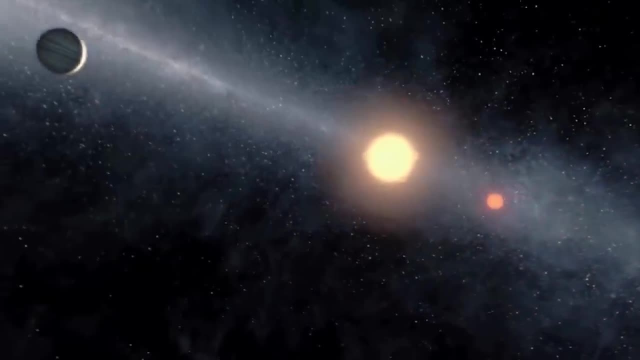 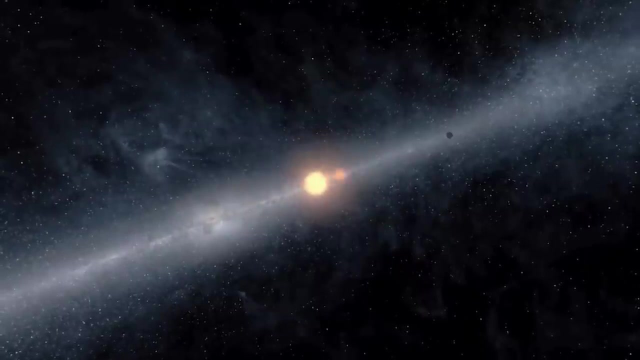 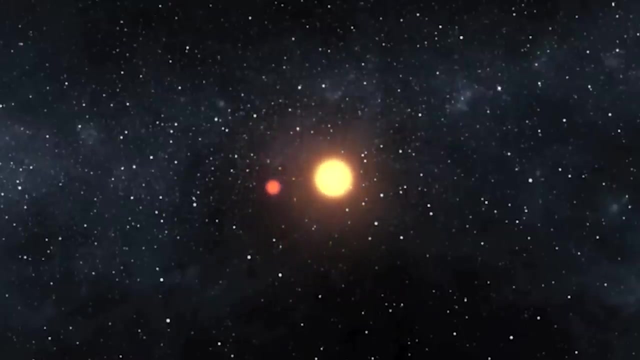 Despite this, the planet's discovery has significant implications for our understanding of the formation and dynamics of planetary systems of binary stars. The existence of Kepler-16b challenges previous assumptions about planet formation, indicating that planets can form and maintain stable orbits even in the complex gravitational fields. 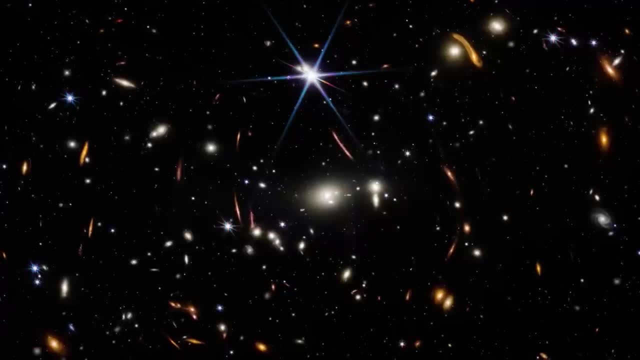 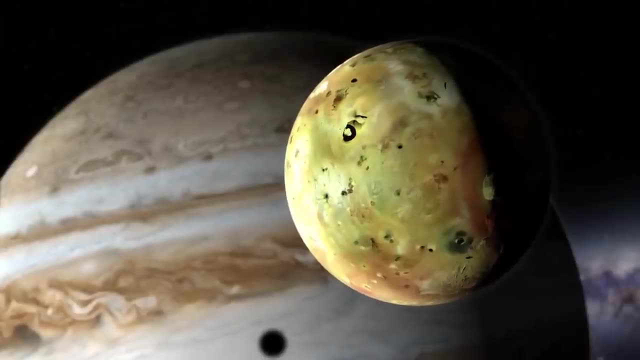 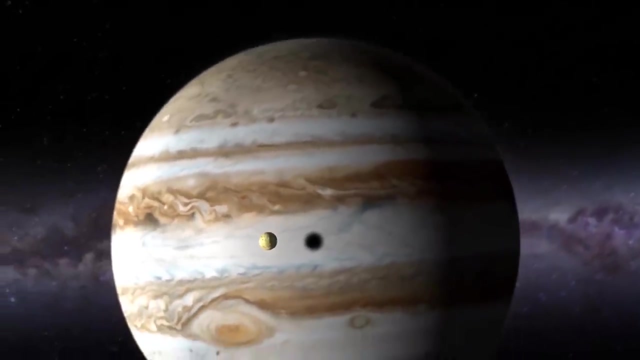 generated by two stars. This has broadened astronomers' search for exoplanets to include binary and multiple star systems which are common in our galaxy. Moreover, the study of Kepler-16b and similar circumbinary planets helps scientists to refine models of planetary formation. 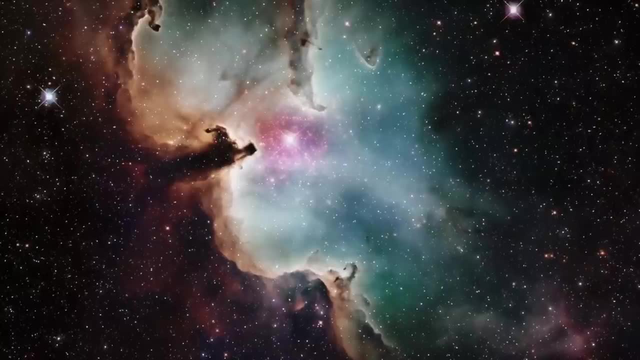 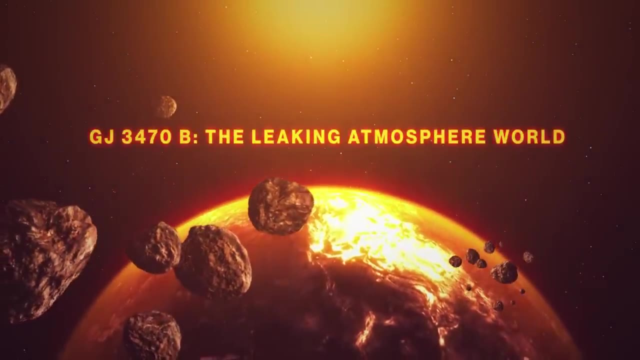 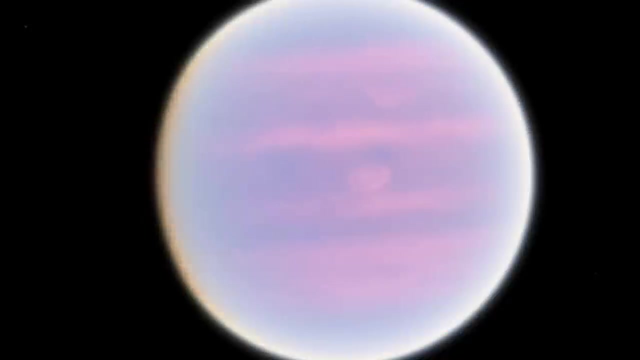 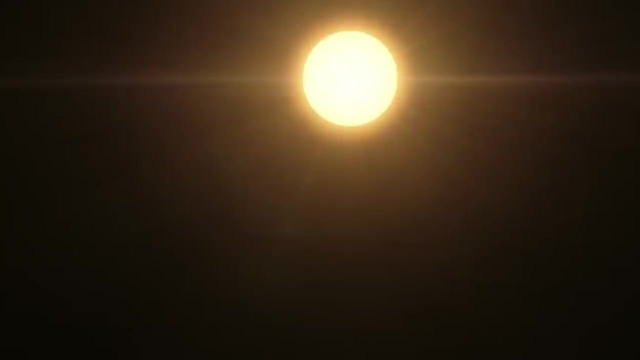 and migration, offering insights into the diversity of worlds that exist in the Universe. GJ 3470 b, an exoplanet situated about 100 light-years away in the constellation of Cancer, has caught the scientific community's attention Due to its significantly. 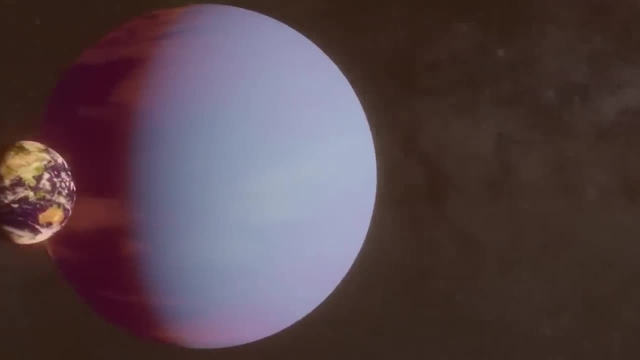 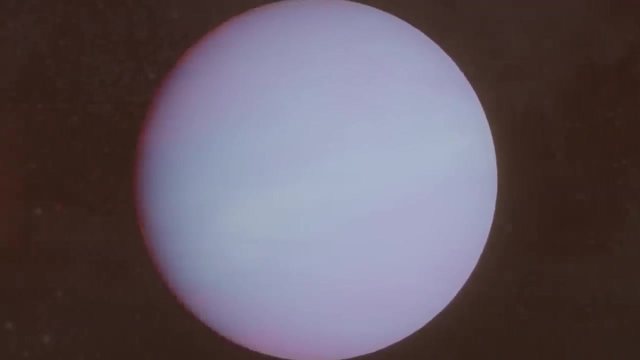 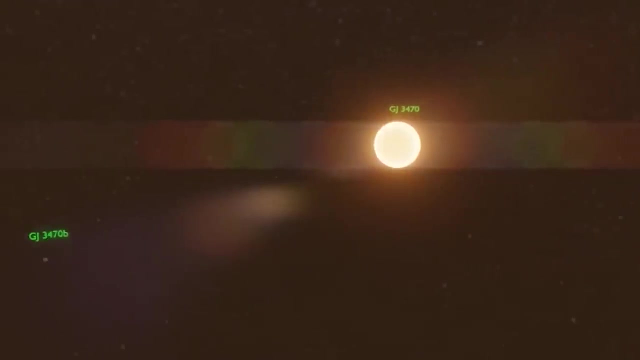 leaking atmosphere. this Neptune-sized world orbits a red dwarf star, GJ 3470,, and is classified as a warm Neptune because of its size and the higher temperatures it experiences compared to Neptune in our solar system. The phenomenon of its leaking atmosphere presents a rare opportunity. 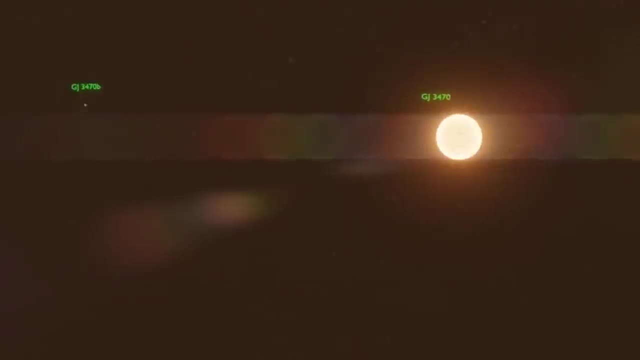 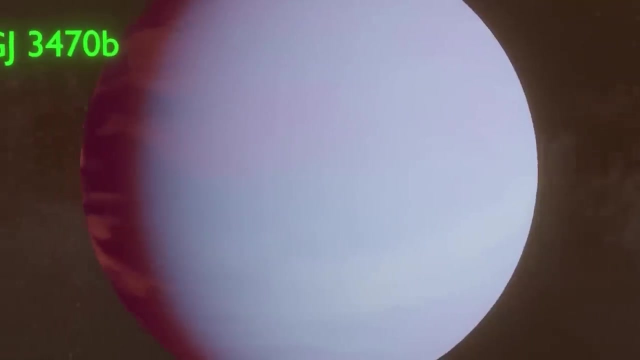 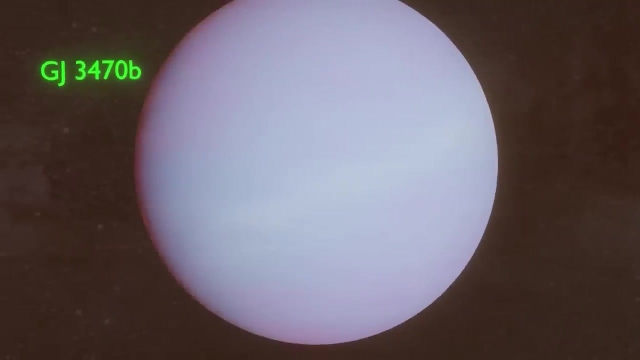 for astronomers to study atmospheric loss processes in exoplanets, which can provide insights into the evolution and the factors influencing habitability. The atmosphere of GJ 3470 b is escaping into space at an astonishing rate, a process that has been directly observed by astronomers. 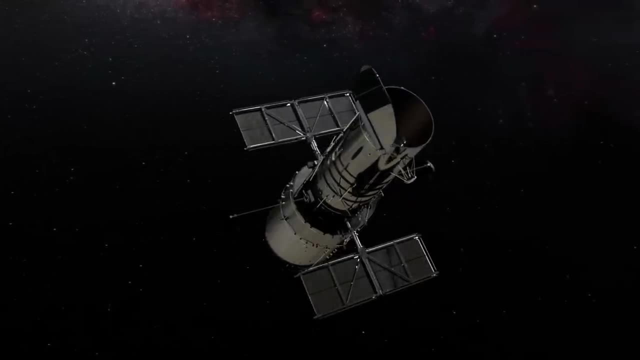 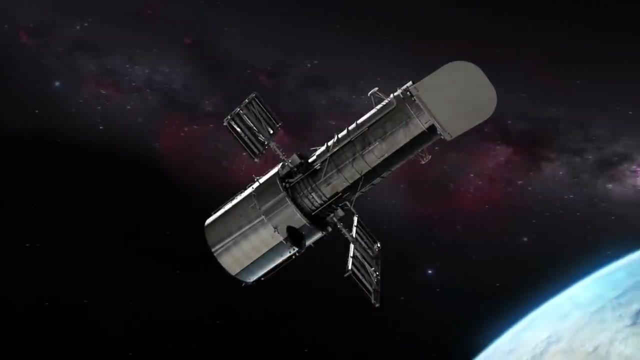 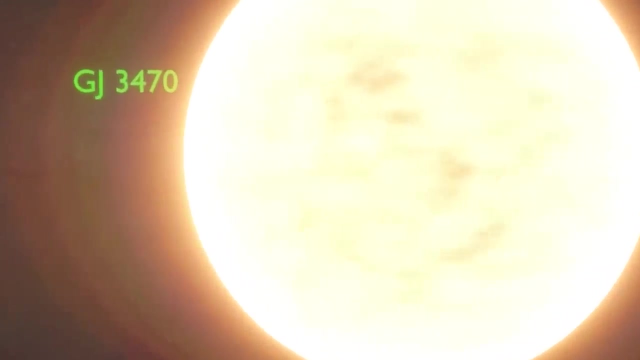 using the Hubble Space Telescope and other observatories. The planet's proximity to its host star exposes it to intense ultraviolet and X-ray radiation, which heats the upper layers of the atmosphere to the point where hydrogen and other gases can achieve escape velocity and break free. 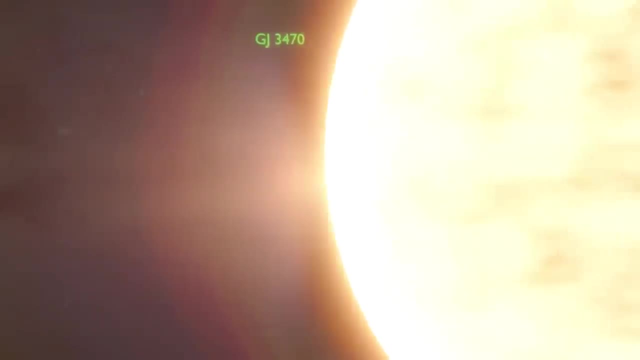 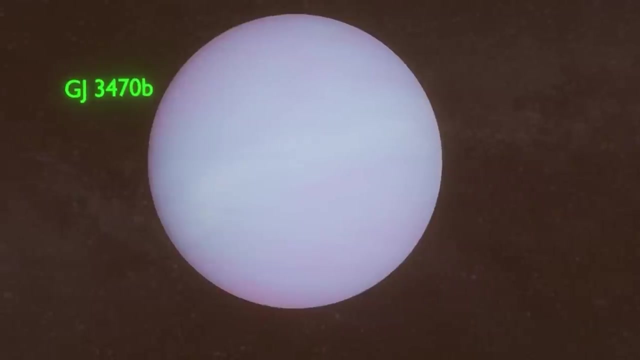 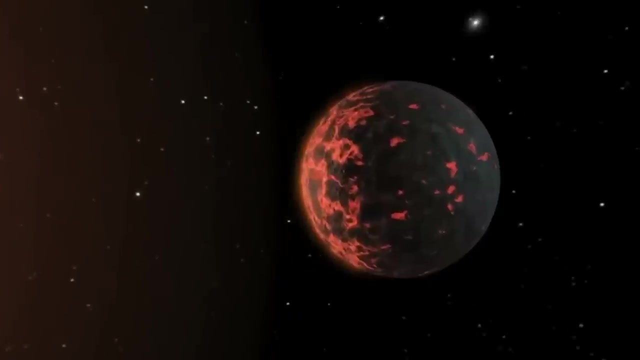 from the planet's gravitational pull. This atmospheric escape is particularly significant in GJ 3470 b's case, with estimates suggesting it may be losing up to 100 times more mass per year than a similar exoplanet GJ 436 b. 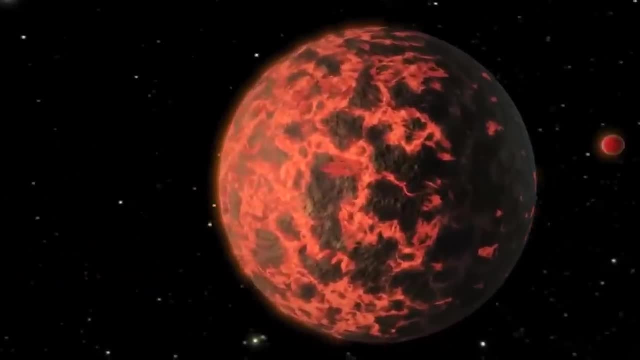 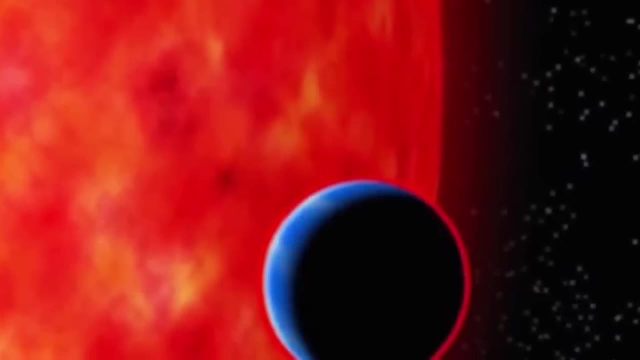 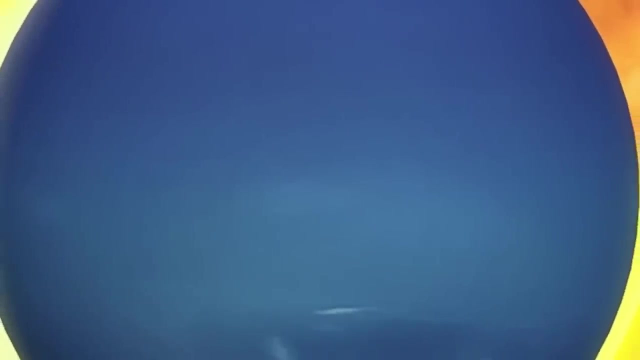 another warm Neptune in the atmosphere. The rapid loss of atmosphere on GJ 3470 b raises questions about the planet's future and what it might tell us about the life cycles of similar exoplanets Over time. the continuous loss of atmospheric gases. 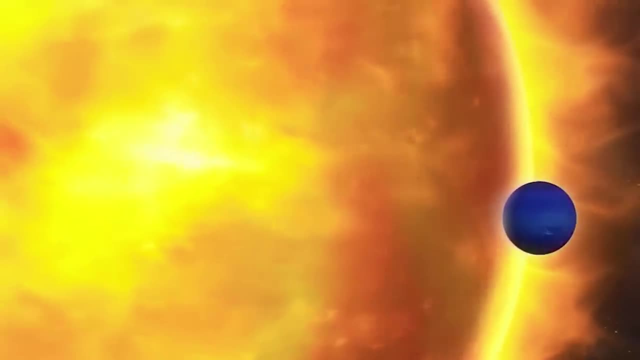 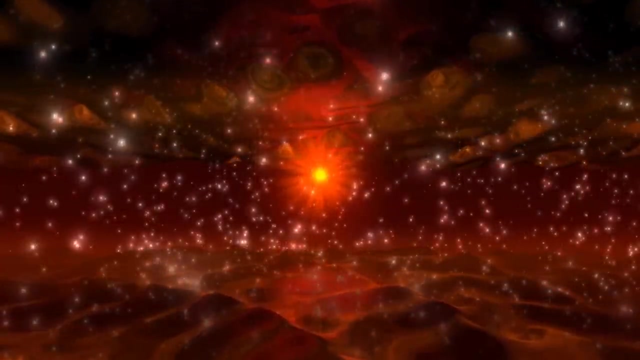 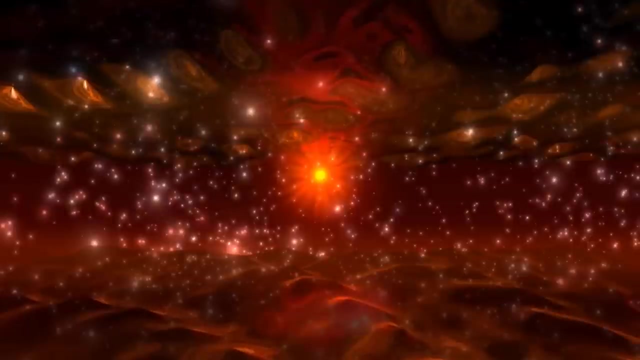 could significantly alter the planet's composition, potentially transforming it from a gas-dominated world to a red dwarf star. This transformation process, while taking billions of years, offers a glimpse into the dynamic nature of planetary systems and the various end states that planets can achieve. 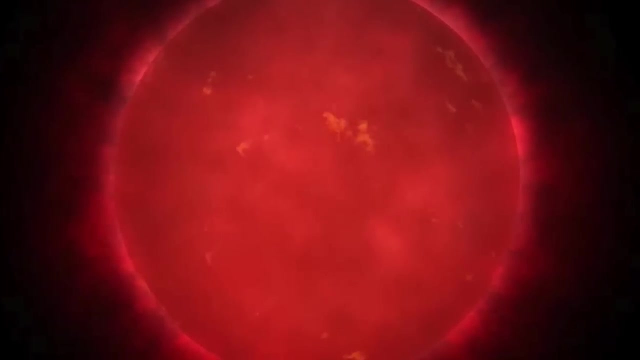 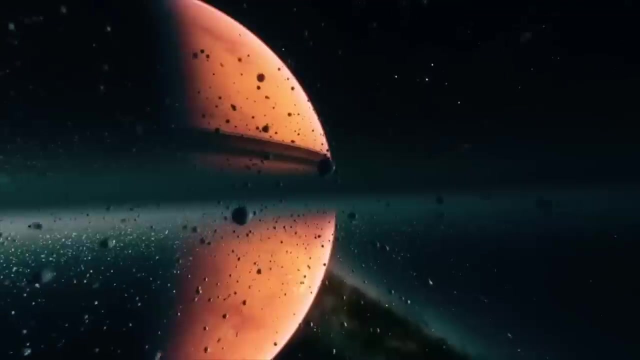 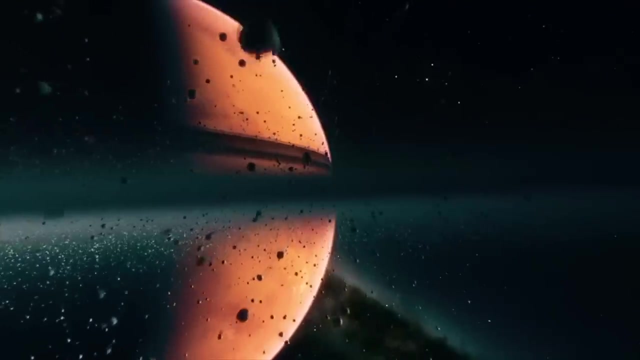 K 218 b, an exoplanet that orbits within the habitable zone of K 218,, located about 124 light-years away in the constellation Leo, has piqued the interest of astronomers and astrobiologists alike. This planet is classified. 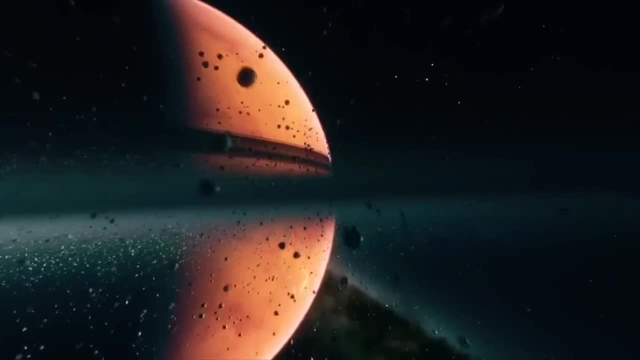 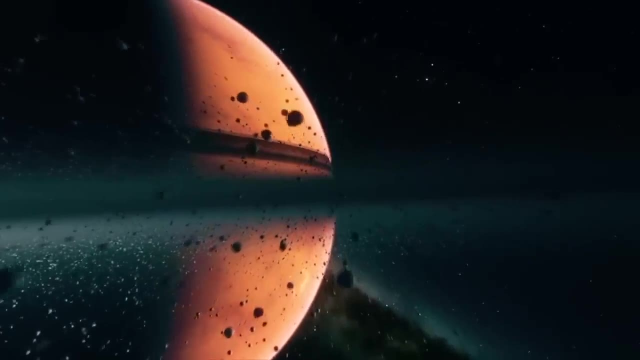 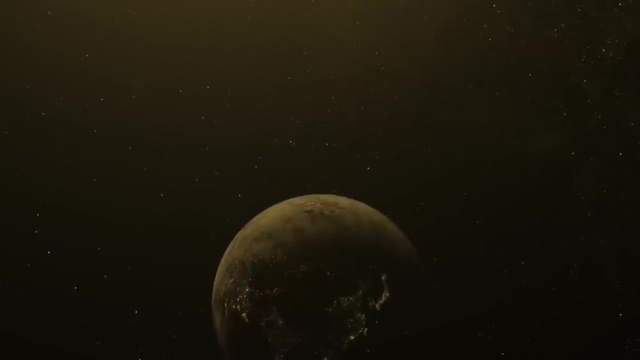 as a super-Earth due to its size and mass, which are several times that of Earth, making it larger than typical rocky planets, but smaller than gas giants like Neptune or Jupiter. What sets K 218 b apart from other planets is the detection of water vapour. 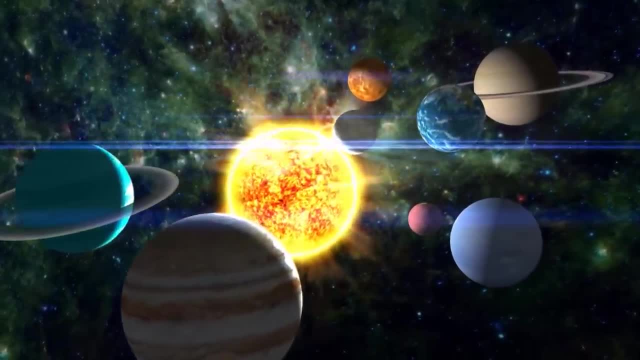 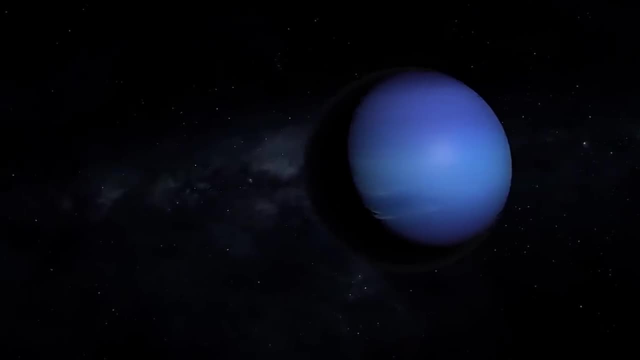 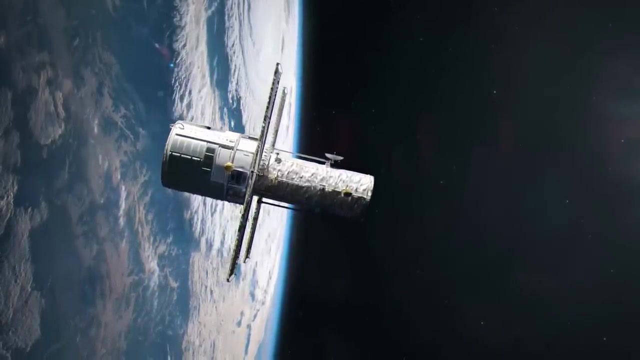 in its atmosphere, a finding that marks a significant milestone in the search for habitable worlds beyond our solar system. The presence of water vapour in the atmosphere of K 218 b was confirmed through observations made by the Hubble Space Telescope utilising a technique. 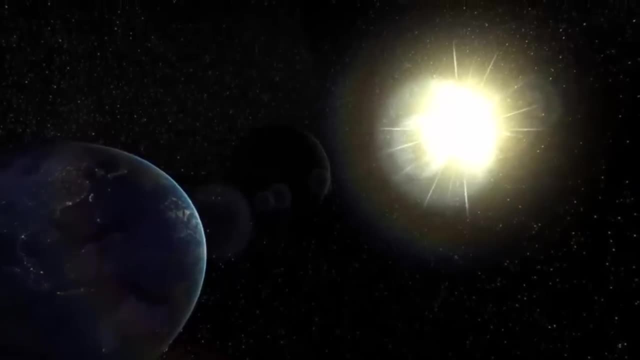 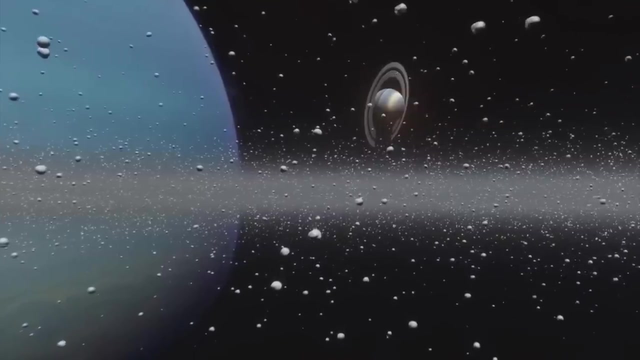 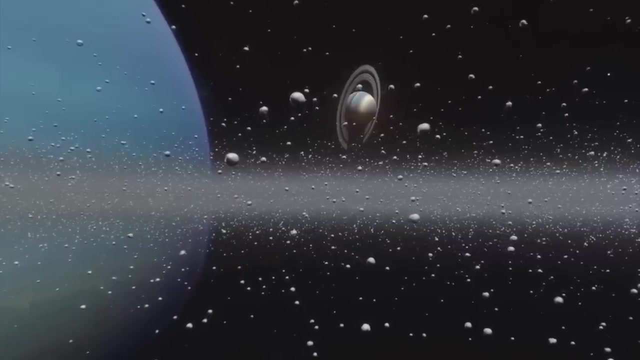 known as transit spectroscopy. As the planet passes, it filters through its atmosphere, allowing scientists to analyse the light and identify the chemical signatures of various molecules, including water vapour. This method provides valuable insights into the composition of exoplanet atmospheres and the conditions present. 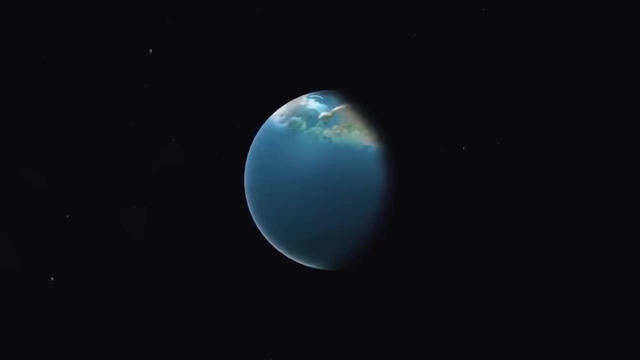 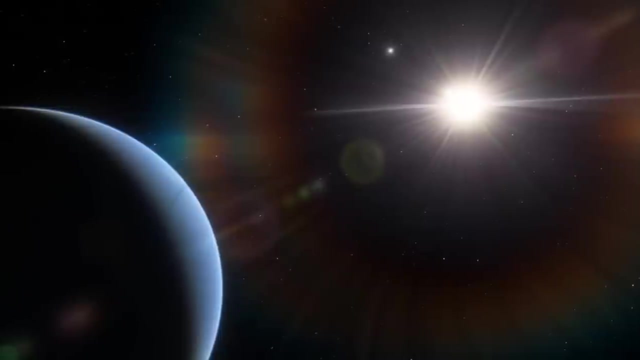 on these distant worlds. K 218 b's orbit lies within the habitable zone of its star, a region where temperatures could allow for liquid water on its surface, provided the planet has a suitable atmosphere. The discovery of water vapour in the atmosphere of K 218 b. 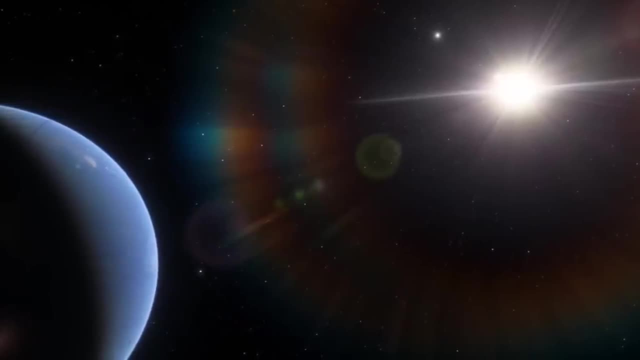 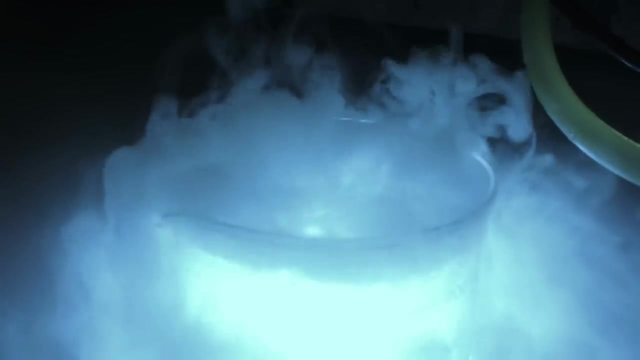 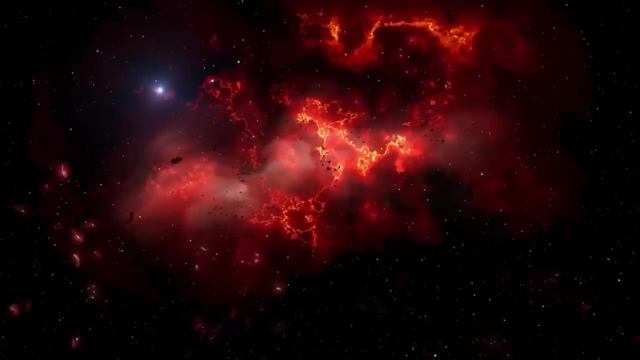 suggests that, under the right conditions, this planet could potentially have liquid water, a crucial ingredient for life as we know it. However, it's important to note that the existence of water vapour in the atmosphere does not guarantee the presence of liquid water on the surface. 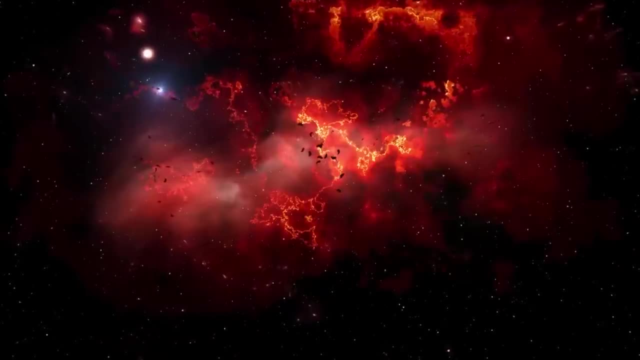 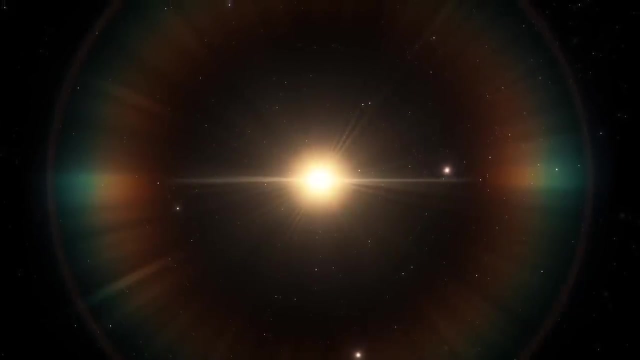 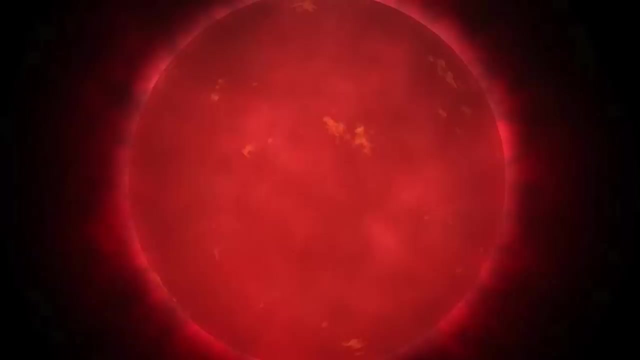 and that temperature and other environmental conditions play significant roles in determining whether water can exist in liquid form. The star K 218 is a red dwarf smaller and cooler than our Sun, and red dwarfs are known for their stellar activity, which can impact the habitability. 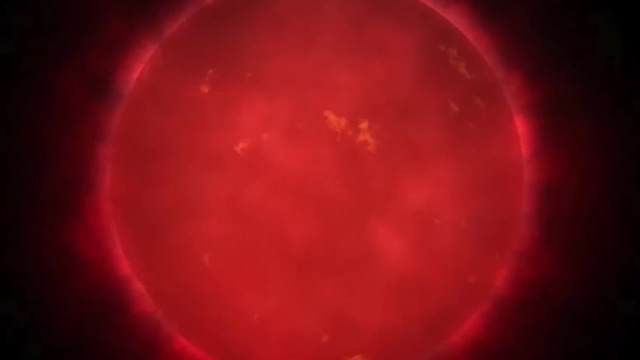 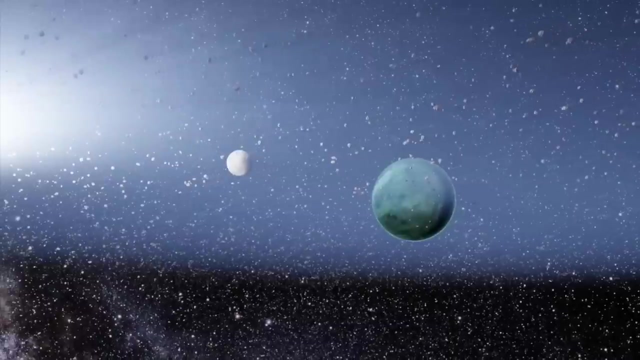 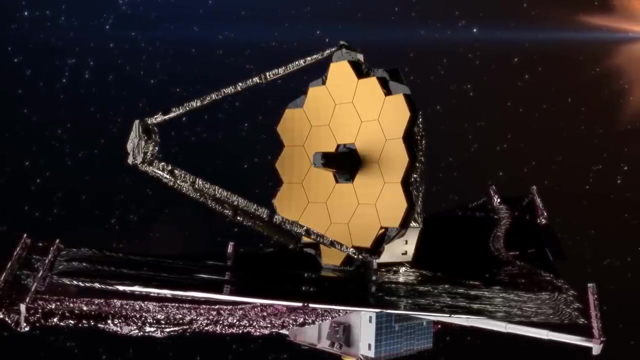 of orbiting planets. Despite this, the specific conditions of K 218 b's orbit make it one of the most intriguing targets for further study in the quest to find potentially habitable exoplanets. Future observations with more advanced telescopes such as the James Webb Space Telescope. 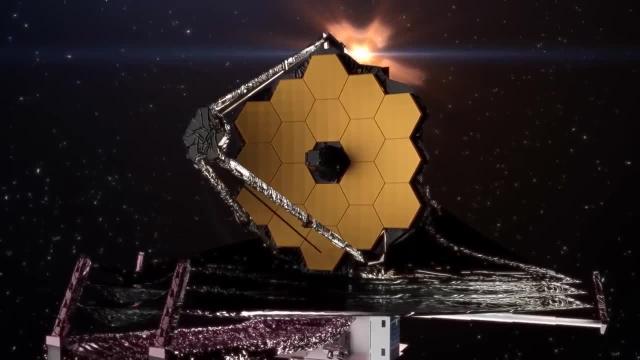 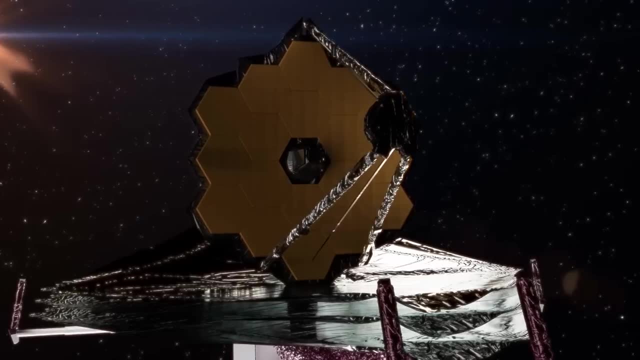 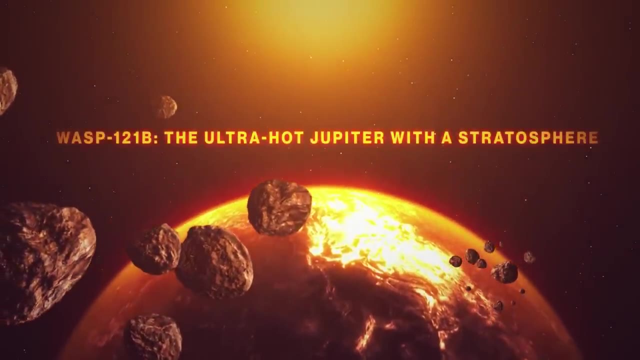 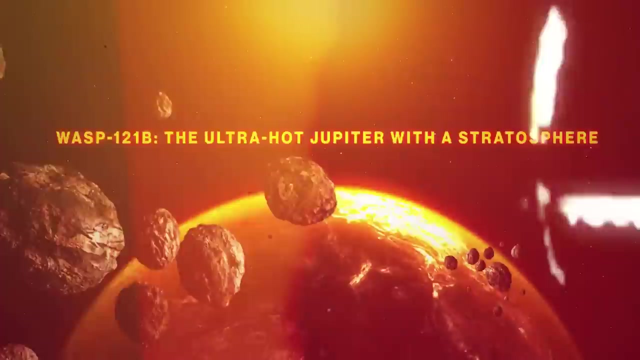 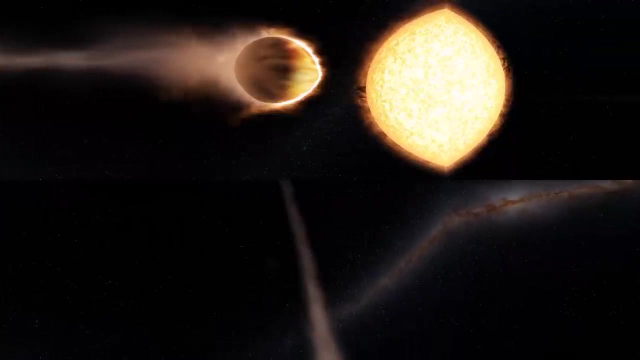 will aim to provide a more detailed understanding of K 218 b's atmosphere, including the possibility of other gases that might support a habitable environment, such as nitrogen and oxygen Wasp. K 218 b's orbit is known for its very unique atmospheric characteristics. 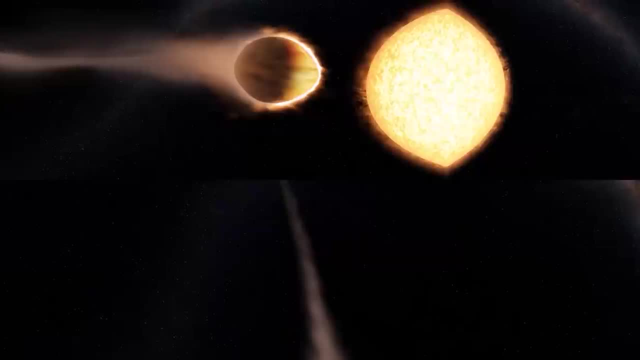 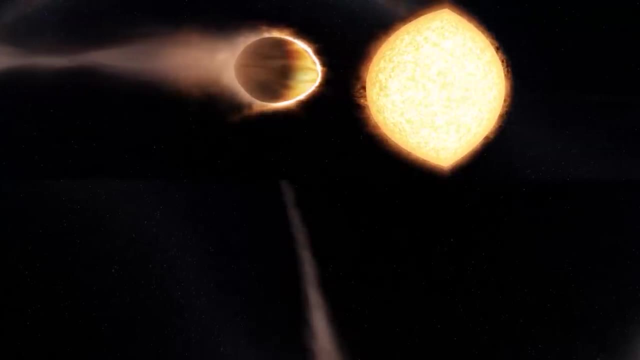 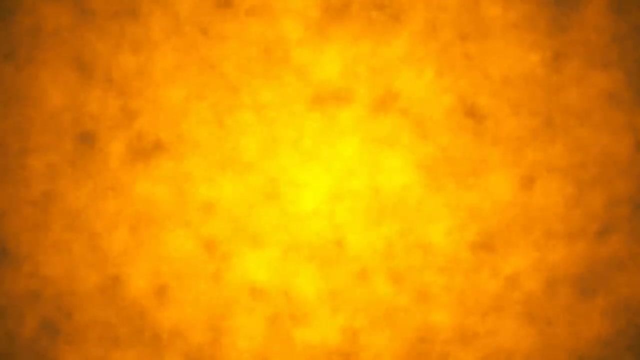 K 218 b's orbit is classified as an ultra-hot Jupiter, a gas giant that is more massive than Jupiter, its host star, leading to extremely high temperatures. One of the most striking features of WASP-121b is the presence of a stratosphere, a layer. 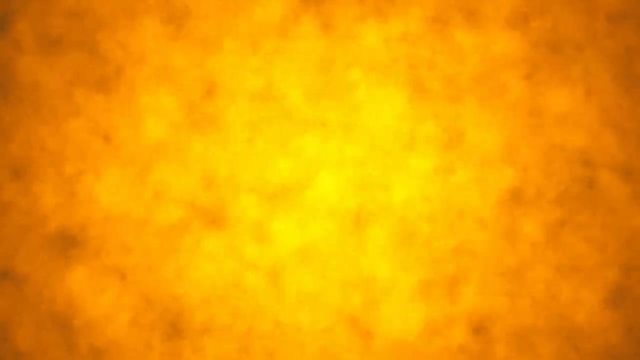 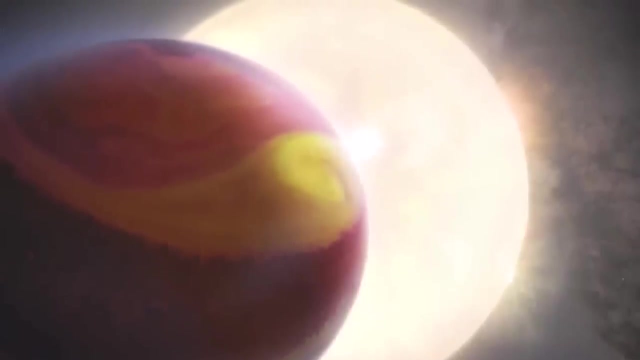 in its atmosphere, where temperature increases with altitude similar to the stratosphere of Earth. This discovery marks a significant step forward in our understanding of the atmospheric dynamics of exoplanets. The existence of a stratosphere on WASP-121b was confirmed through observations made by